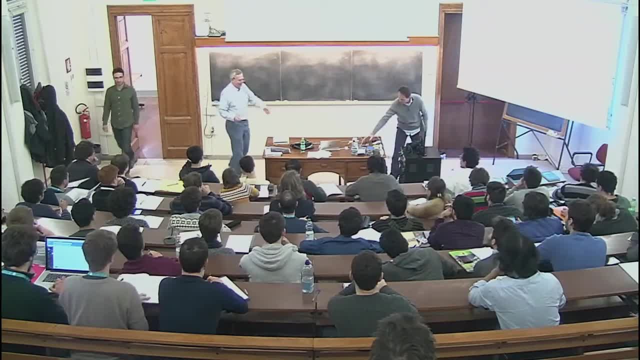 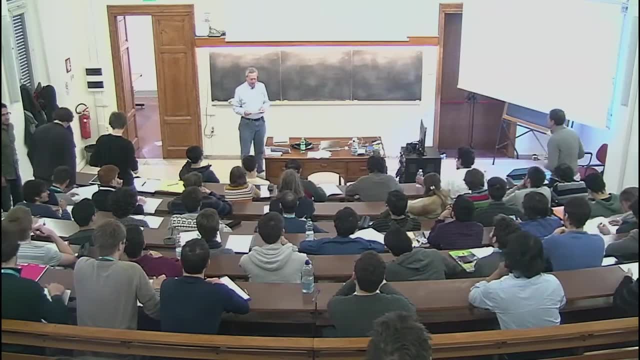 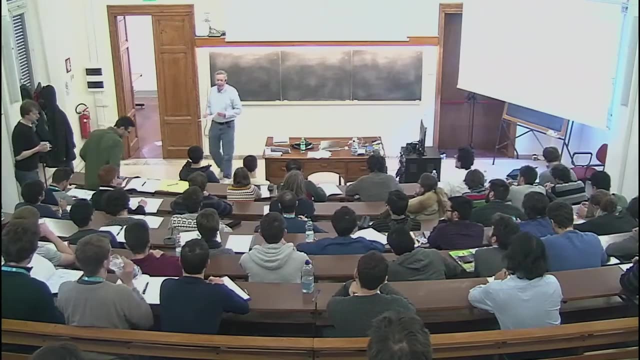 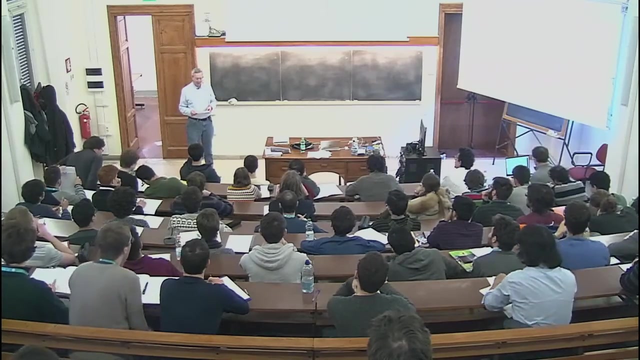 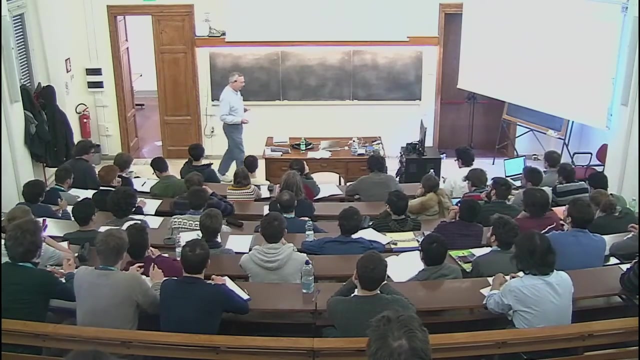 Okay, thanks, very much Thanks to the organizers for inviting me to this school. I love these schools, especially. this is such a nice environment. So I look forward to three days of interesting discussions with you all. I do a lot of these schools, but I do very few of them where the audience is primarily theorists. I've done this before, but it's rare, And so I think the angle that you come at the topic of statistical data analysis is going to be a little bit different from what I usually do with an experimental crowd. 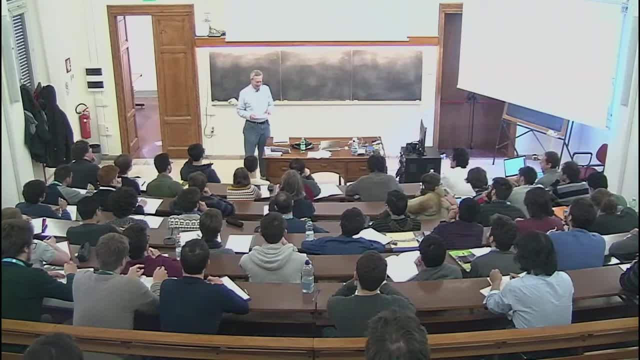 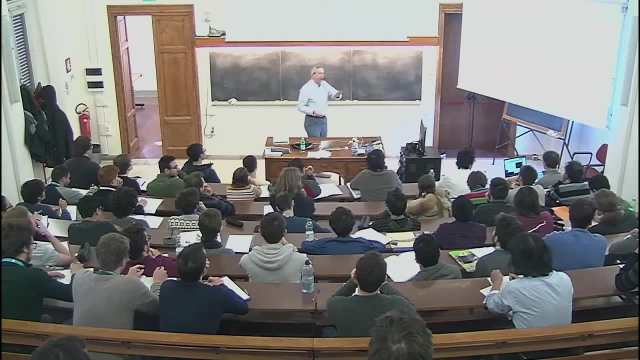 But we'll just feel our way through that, And so let me start. No, sorry, before I start on the board, I should mention a couple of things. I like the suggestion very much of using mainly the blackboard, but I'm just going to mention a few things that we have on the web. 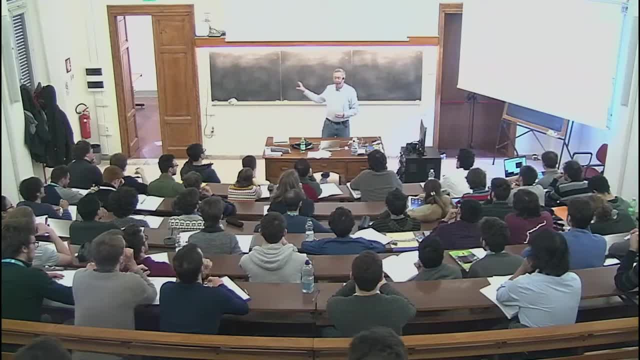 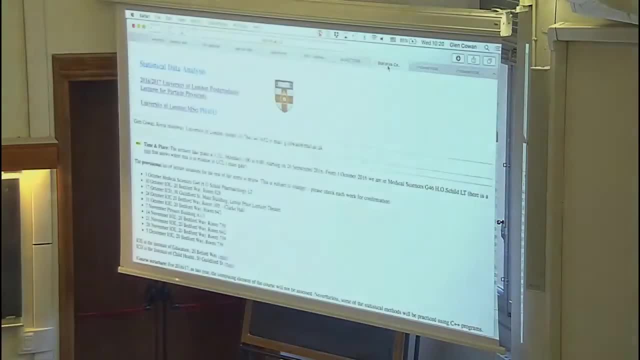 And a lot of the things that I'm going to show in the next three days. essentially, everything is a subset of the course that I give in London, And you all received an email with the link to this course, And so, if you take a look at that, there are down here some problem sheets. 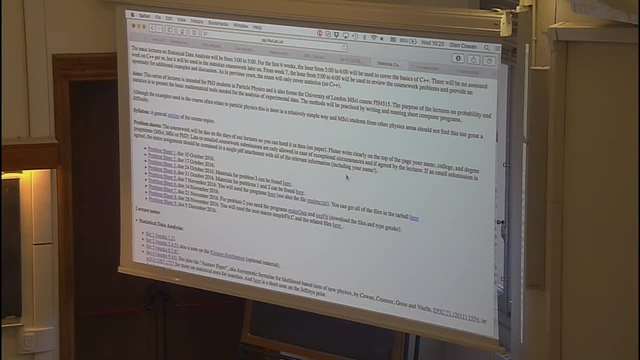 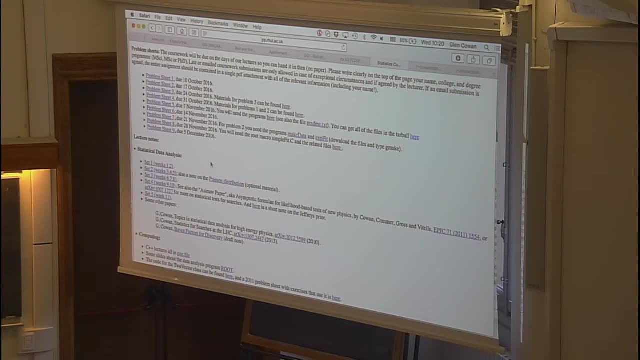 And I've also selected a subset of these problems for us to discuss in the afternoons. And then There are some slides. these various slides here and almost all of the material- if you want to refer back to some formulas- are somewhere in those slides. 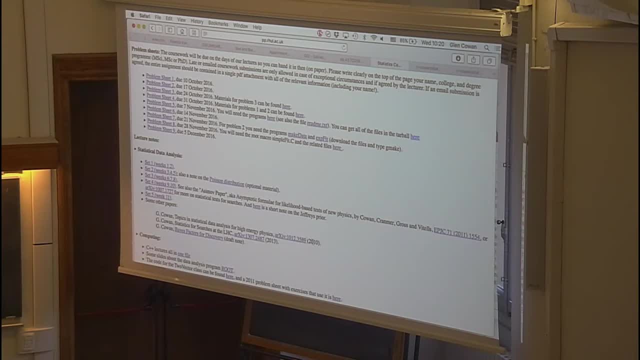 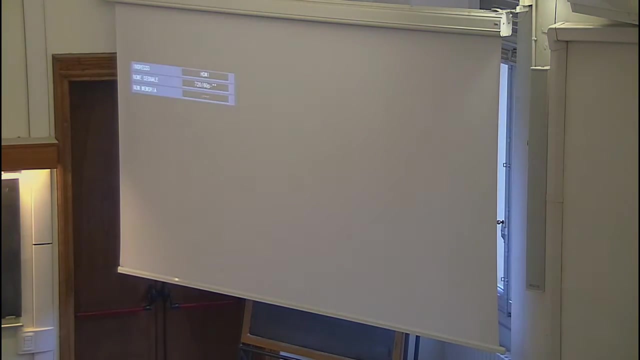 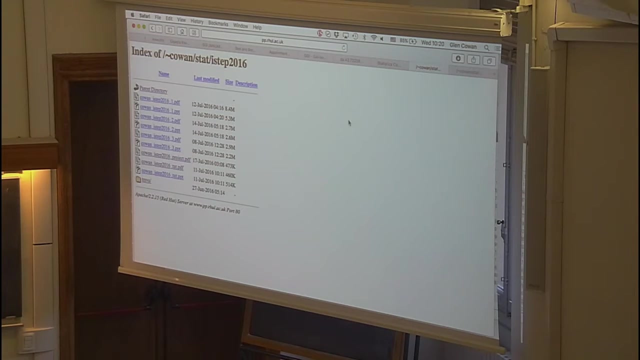 There are also some papers that I've written as the result of some CERN summer schools that discuss these things in slightly greater detail, And so you could look at those as well. So from where you sit? a slightly more advanced, Largely empty web page, but this is just the place where I'm going to collect together all of the files that are specific to you. 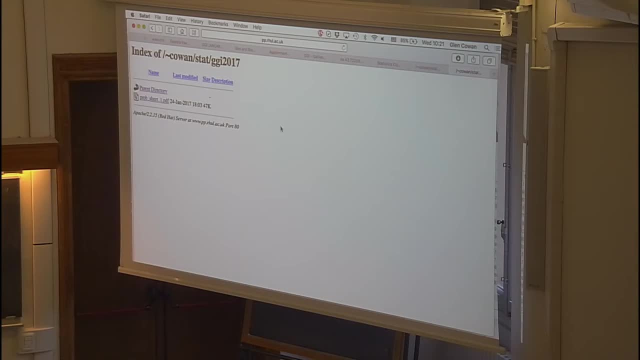 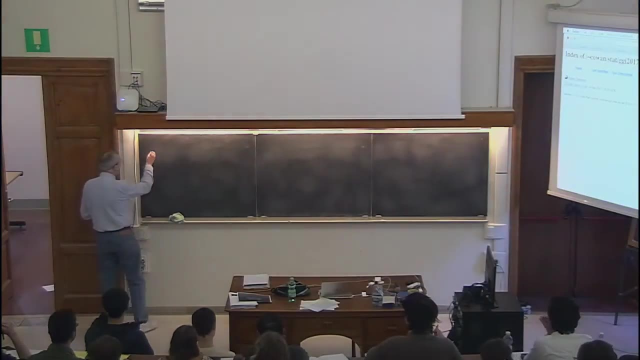 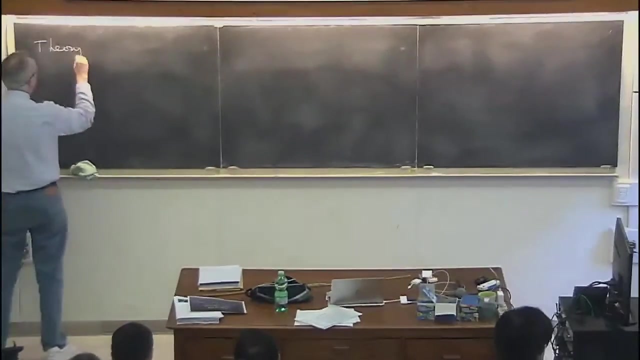 So the problem sheets, for example, that we'll be discussing in the afternoons. Okay, so, having said that, let's start with the main topic, And that is in the landscape of particle physics. I think that statistics lives, And so you're over here with theory. 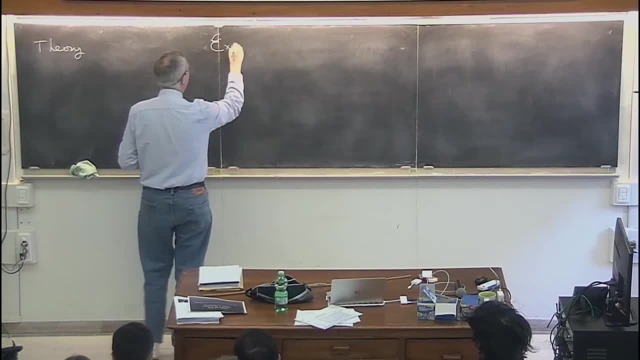 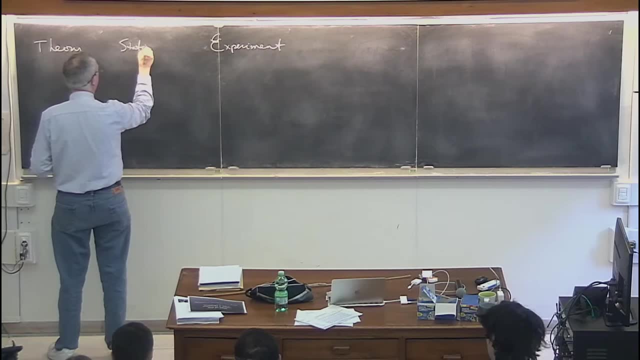 And then over here we have some sort of experiments, And statistics is right in the middle, And statistics is right in the middle, And statistics is right in the middle, And it is, And it is in some sense the place by which the two can be compared. 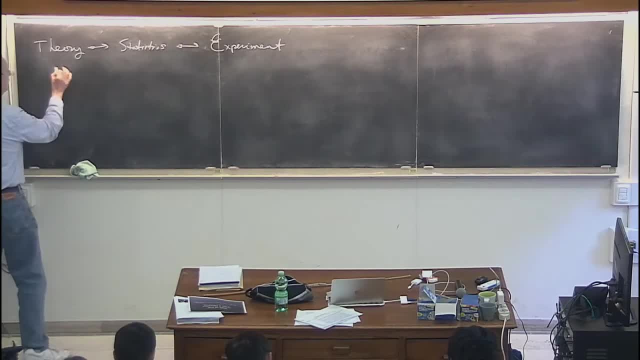 It is the language by which you can say whether or not a certain theory stands in agreement with what we see in observation. Can the theory be rejected or not? And so what do you do? in your theories, You make predictions for some observable, And so two comments on how that works. 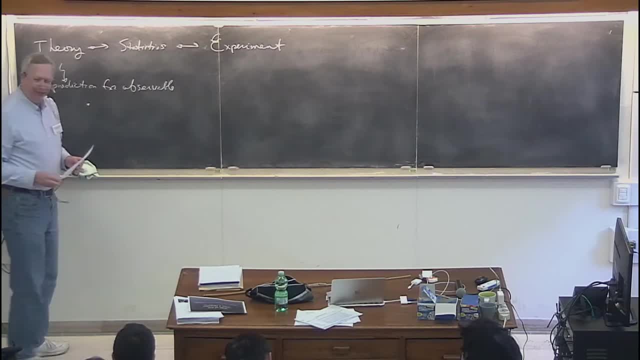 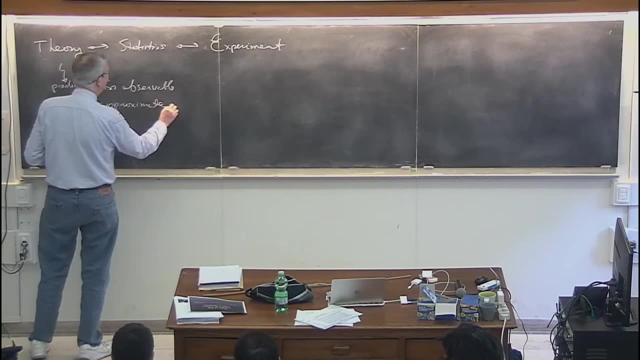 One is: although I'm sure you're very good theorists, I'm still convinced that every time you make a prediction there are going to be a certain number of approximations involved. You calculate perturbation theory to some fixed order or to some limited order. 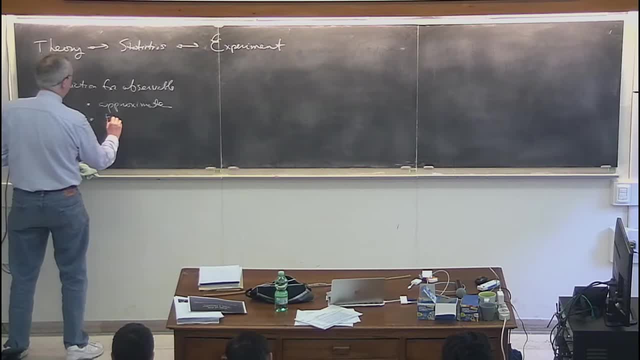 Furthermore, the theoretical predictions very often are not really specific predictions, but they include some adjustable parameters, some free parameters, And so both of those aspects are very relevant when it comes to trying to test a theory: The fact that you're not even in a situation where you can make an accurate prediction from the theory in all cases. 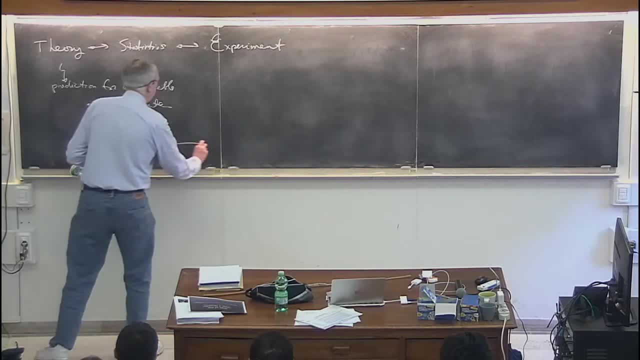 So what does that result in? That results in some prediction of some quantity y sometimes versus some other quantity x, And that's the output of your work. You make a prediction of some quantity y sometimes versus some other quantity x, And that's the output of your work. 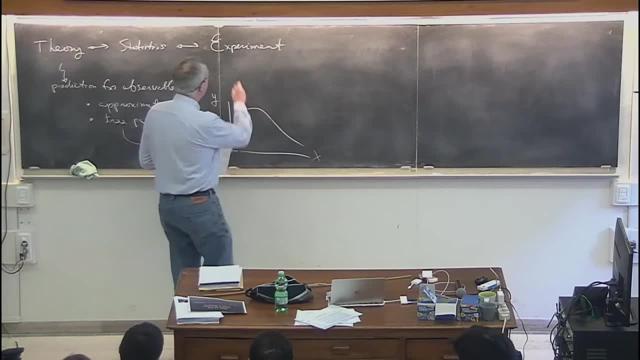 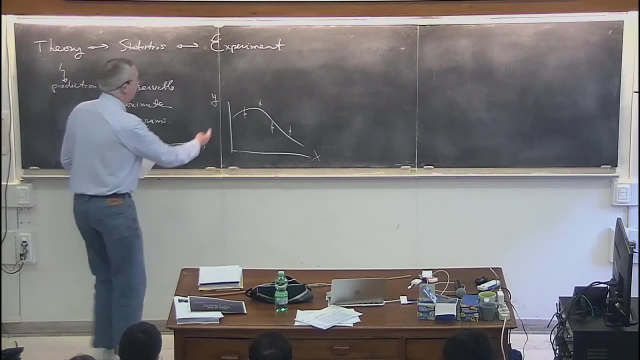 You make a prediction. So then some guys over here on Atlas or CMS or whatever They come in and they fill in some measured values, maybe with some error bars, And we would like to now make a quantitative statement as to whether or not the theory can be excluded. 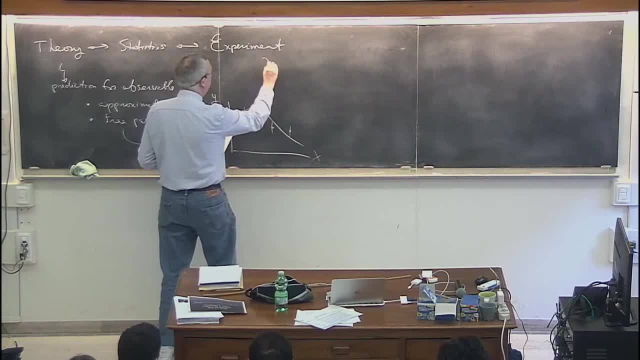 One of the important points to make about the measurements. So measurement is that they inevitably have that little error bar there, at least as a consequence of the random fluctuations due to the finite size of the data. So I'll say measurement with random fluctuations. 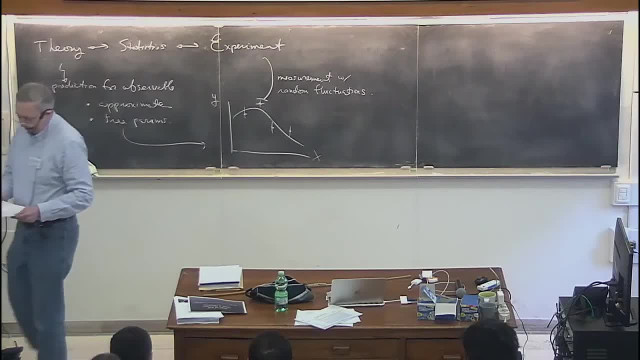 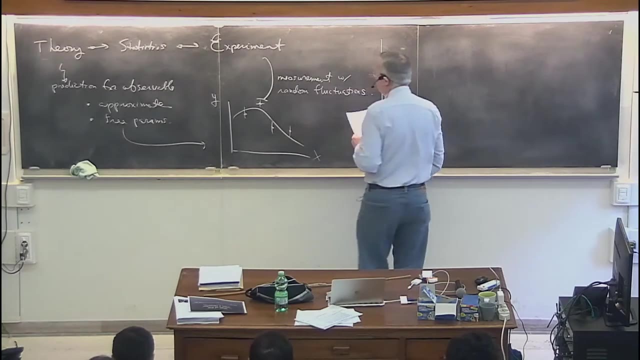 Typically we would count a number of events. That number of events that we count will be distributed according to some probability distribution. If you were to repeat the experiment, you might see a different number of events. So that's the basic setup. And now what we want to do in that middle blob in statistics. 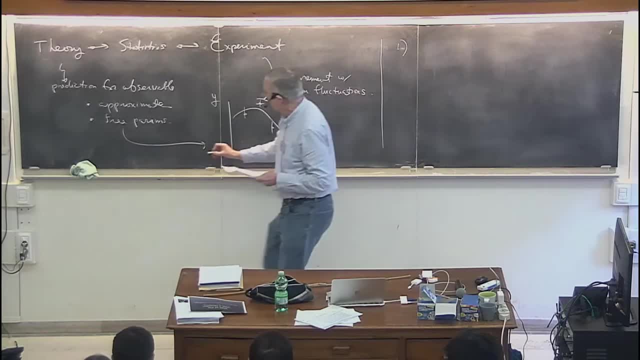 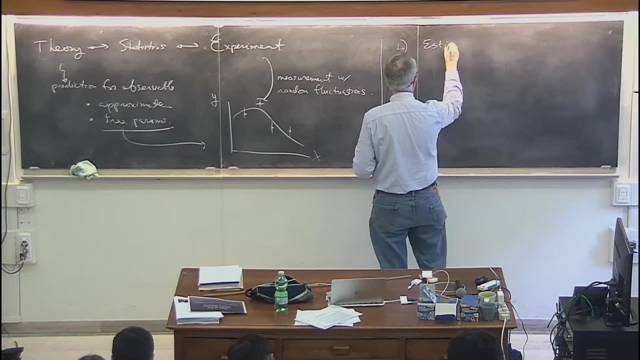 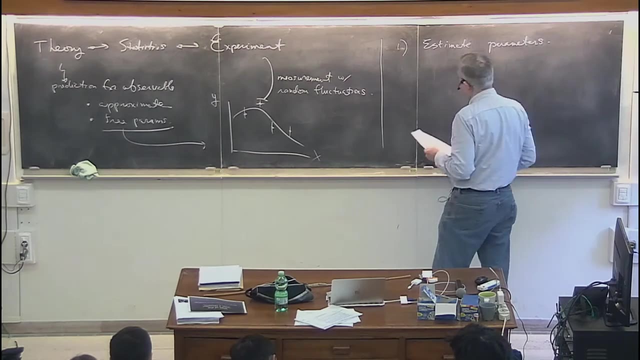 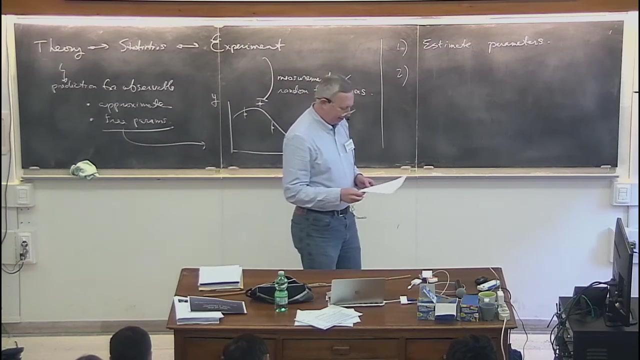 is, first of all, we need to estimate the values of the parameters, And that's what I want to concentrate on for the most of today: Estimate the parameters. Beyond that, you want to know whether or not the Well, sorry, before I go there. 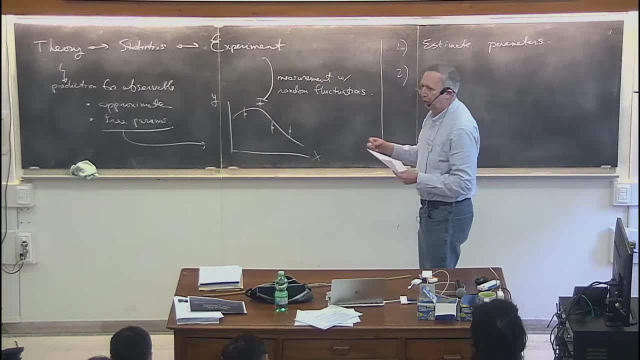 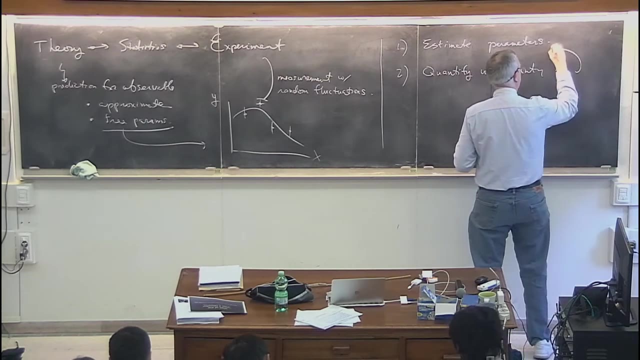 you can estimate the parameters, but then you also have to quantify the uncertainty in the parameter estimates. So let me write that first. So quantify uncertainty in the parameter estimates, And then three- sorry, the thing that I think is probably most interesting. 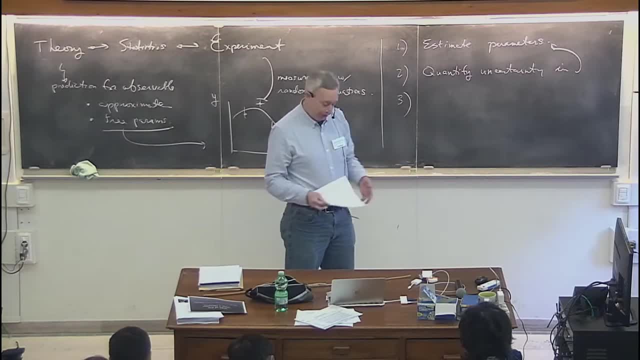 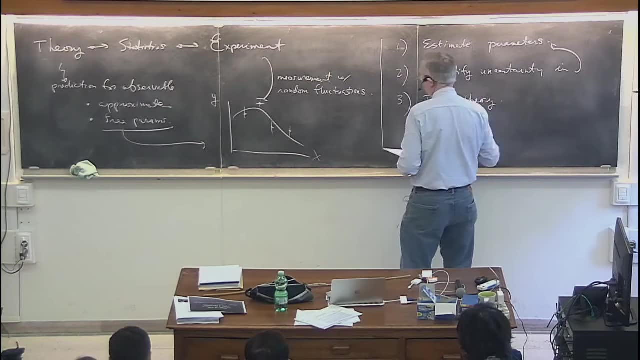 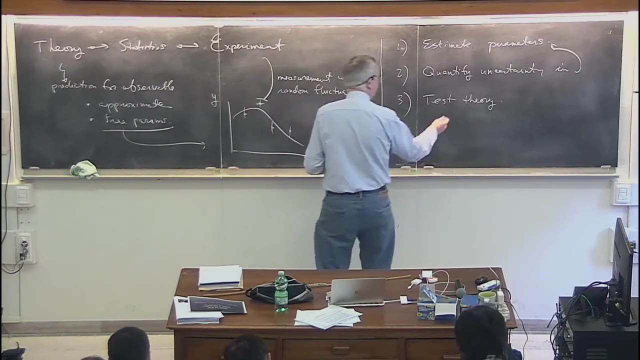 and will be occupying most of the second and third days, is that we want to test the theory. We really want to be able to say: is this theory completely excluded, perhaps for any of the points in its parameter space? I should say that the theory 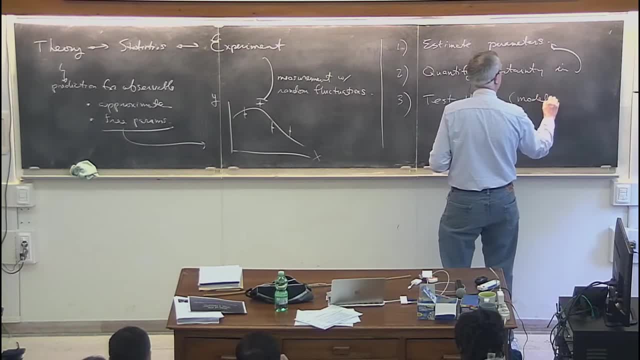 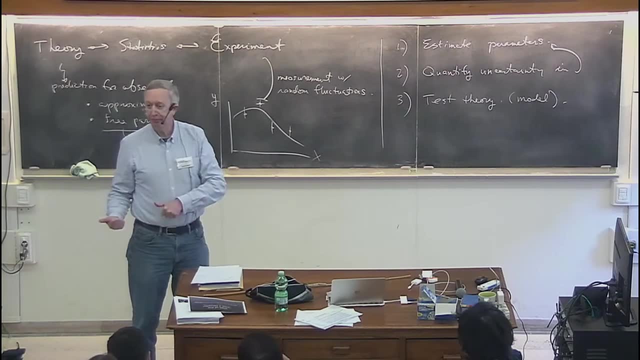 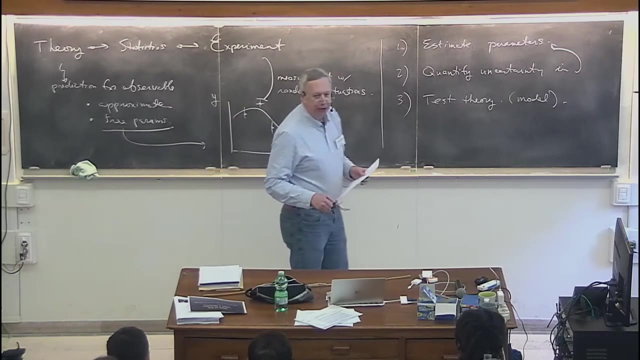 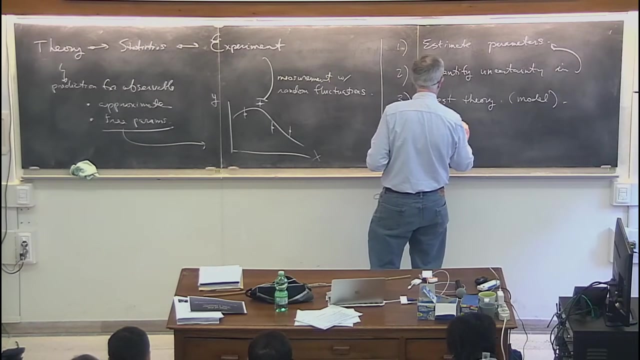 I'm going to use the words theory and model interchangeably in these lectures. For me, either of those two words means a rule that makes predictions for data All right. So there are various elements of uncertainty that enter into this game, And a lot of that is related to the randomness that I mentioned. 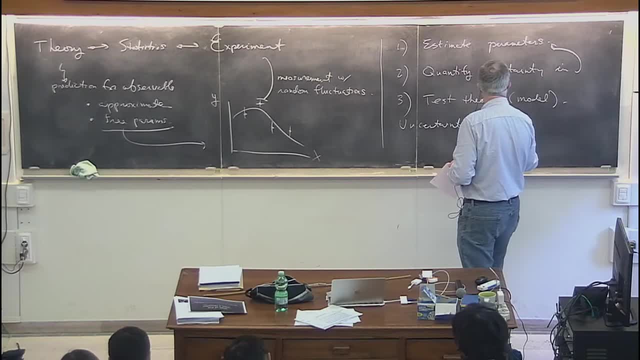 All right. so randomness- And the randomness, of course, is inherent in the types of theories that we deal with- that you have a quantum mechanical theory. It's not a deterministic theory, It has to. It only predicts probabilities, And there I've said the magic word. 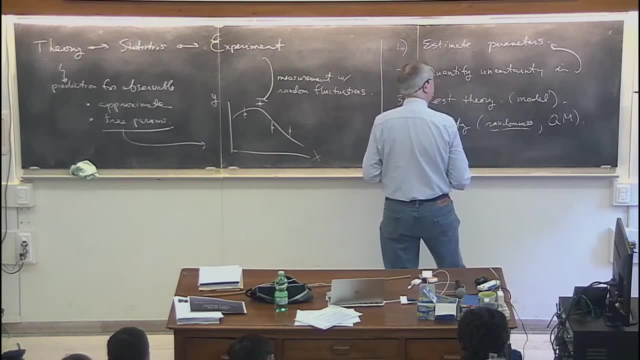 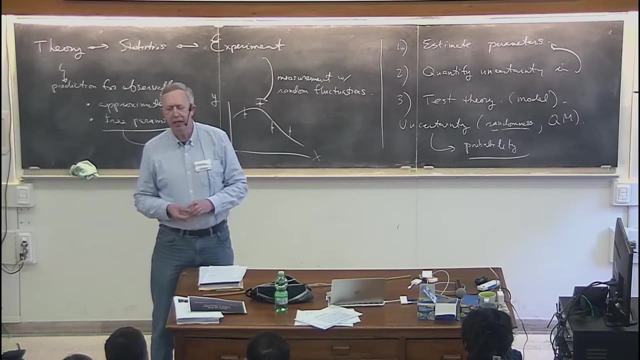 that to quantify these various sorts of uncertainties we're going to have to introduce probability. So even if we lived in a deterministic environment- there's no quantum mechanics- you would still have to deal with random uncertainty for any real observations made in real experiments. 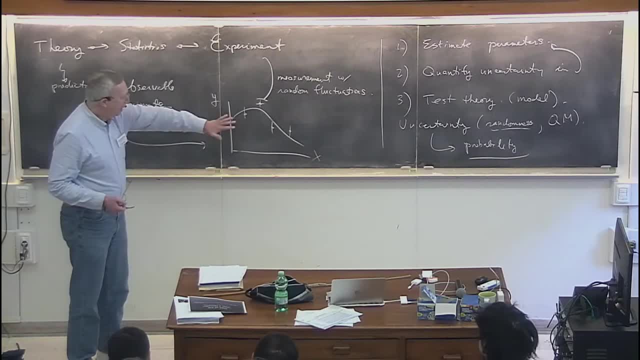 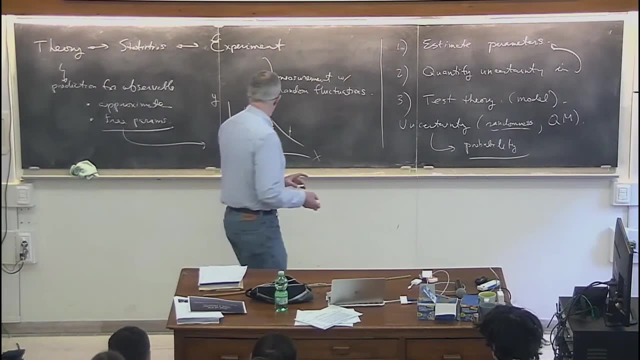 and carried out with a finite budget. So the fact that we have quantum mechanical theories absolutely ensures that we have to talk about probability, but we would have to anyway. Okay, so let's see what. Ah, so here's the eraser right. 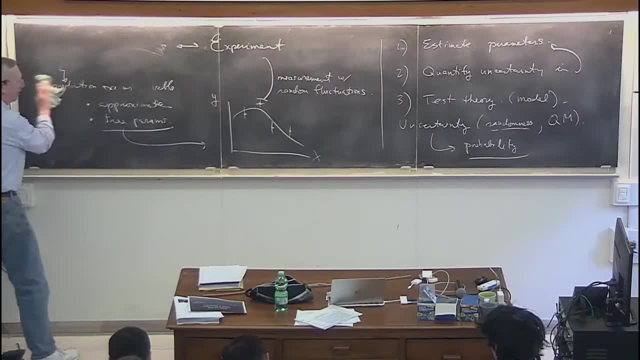 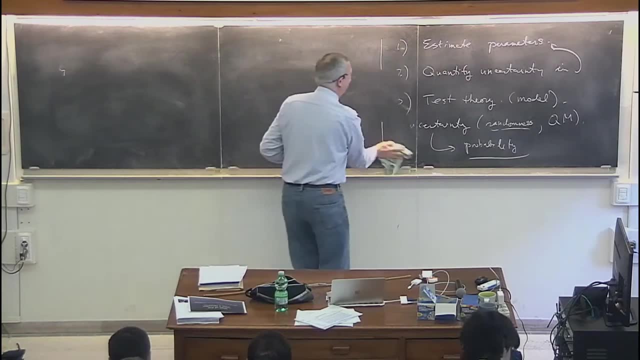 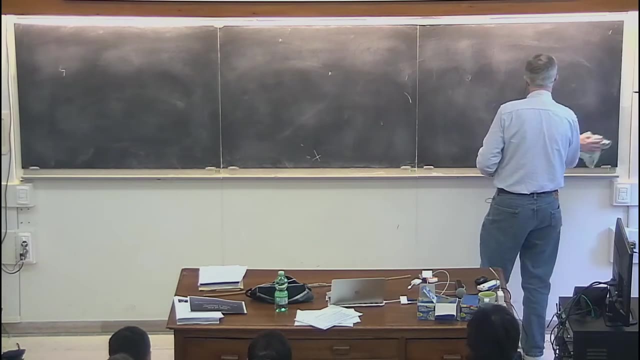 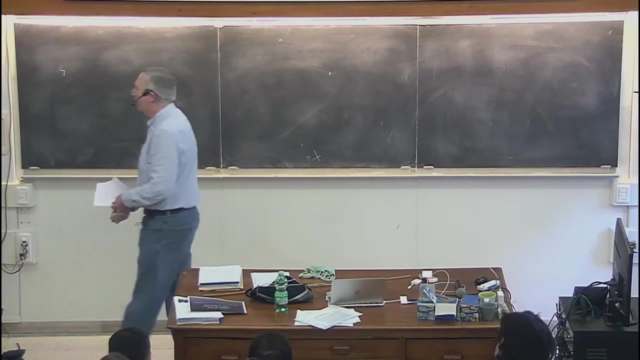 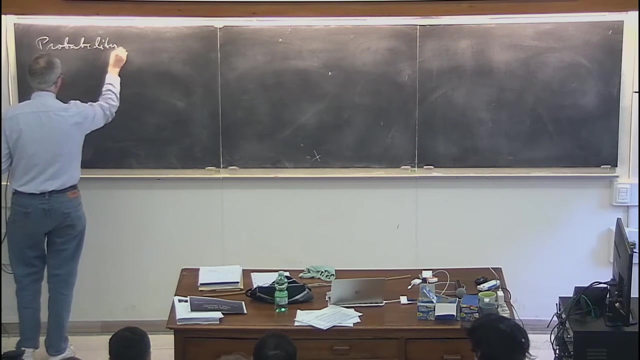 Okay, Unfortunately, I tend to be very spread out when I write on the board. I seem to have to do a lot of erasing, but that's okay. So let's start with probability. Probability: This is one of these topics that everybody sort of has. 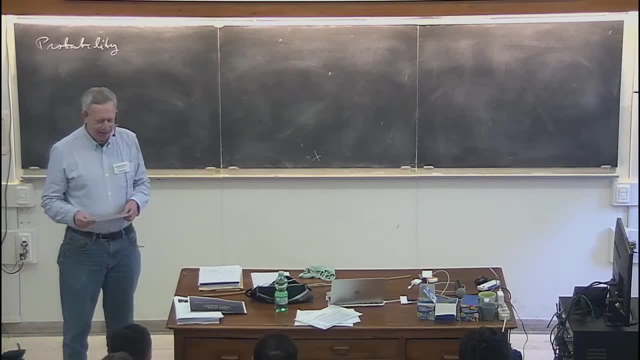 an intuitive notion for probability and I think even cavemen or primates had some notion of probability. But to define it mathematically it's actually a bit slippery, And so the way that this was done by Kolmogorov in the 1930s. 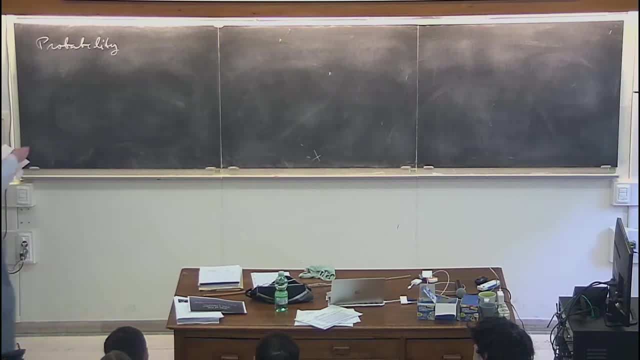 was in the language of set theory. So you have a set S called the sample space, And you have subsets- I'll call them A and B and so forth- And I can write down in this language's set theory some axioms of probability. 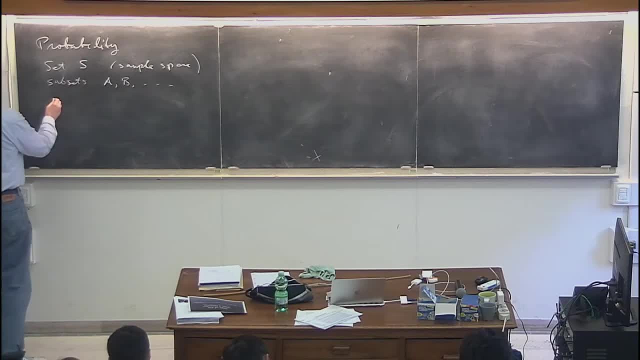 And I can write down in this language's set theory. In fact, it's so easy, I'm just going to do this right away For every subset. How should I write this? For all subsets A in S, I define a real-valued function called the probability. 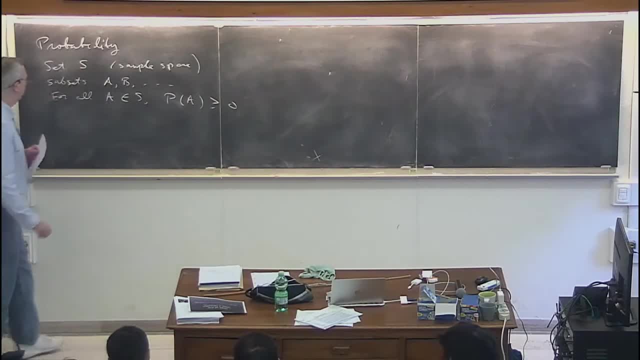 which is greater than or equal to zero. Okay, So that's axiom one. So the sample space is of course one of the subsets, And I assign, for the probability of the sample space, the value one, And then the third one I say is that if I have two subsets, 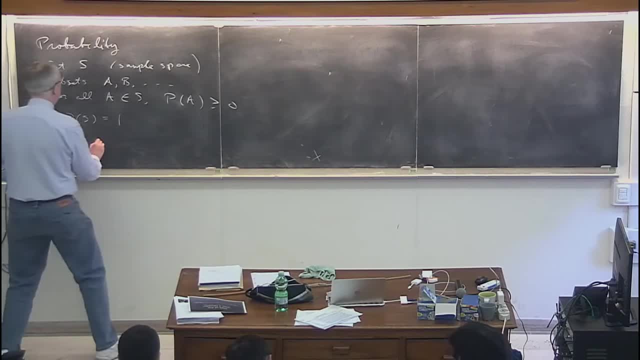 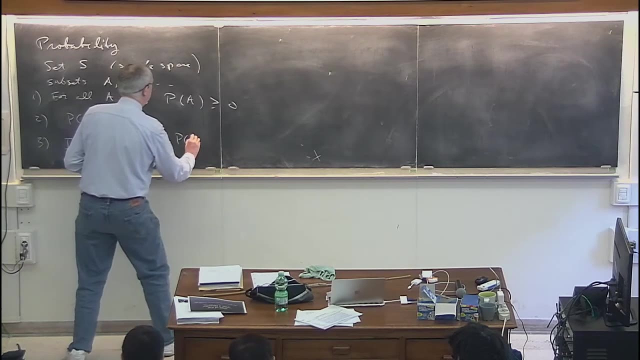 that are disjoint, which is to say so that if the intersection of A and B is equal to the null set- okay, so that means that they're disjoint- then the probability that you associate with the union of those two subsets is simply equal to the sum. 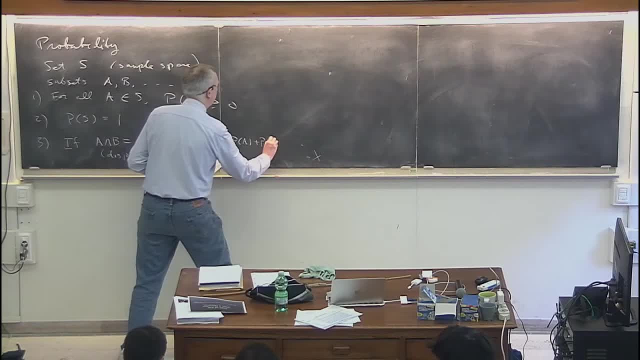 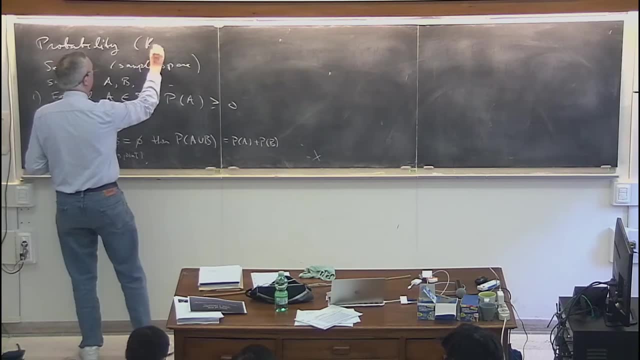 of the two corresponding probabilities. All right, I hope I said that right. So this is Kolmogorov- Kolmogorov, 1930-something. So actually, the first mathematical definitions of probability were from the 1600s. 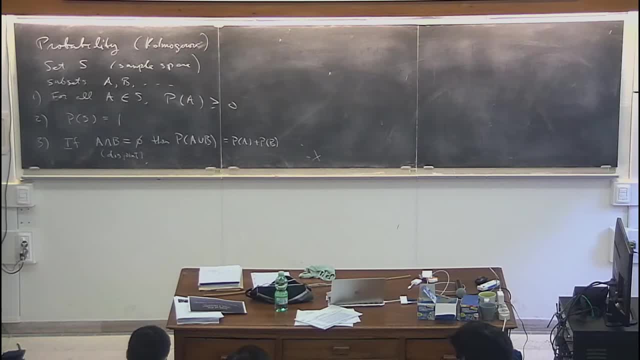 in the context of gambling. In fact it was the first major application. But anyway, the formal definition of mathematical interpretation in terms of- sorry, the axiomatic definition, wasn't until the 20th century. So these axioms are very useful. 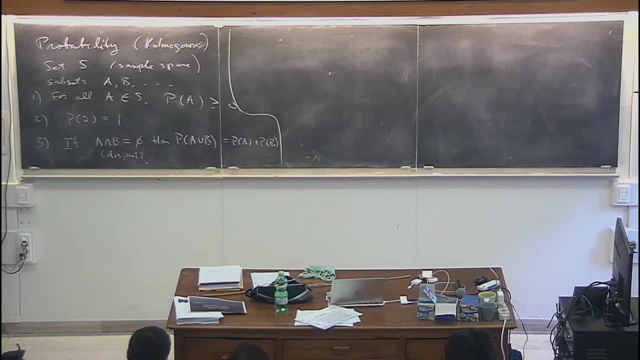 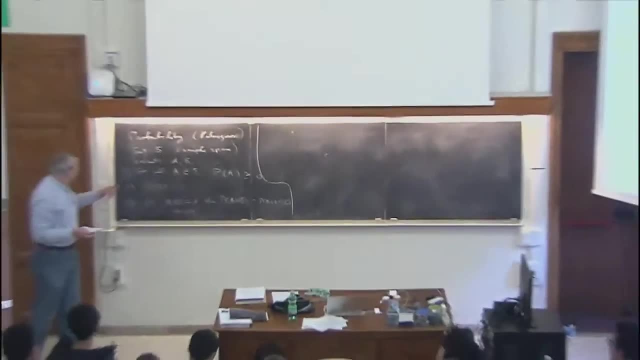 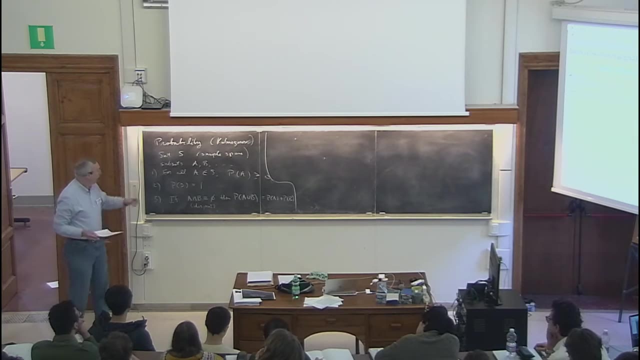 but that may not have been what you would think we would grab for. when we need to work with probability, What we need is a way to interpret the elements of the subsets and a recipe for actually assigning numerical values to the probabilities. So, in this very abstract language of set theory, 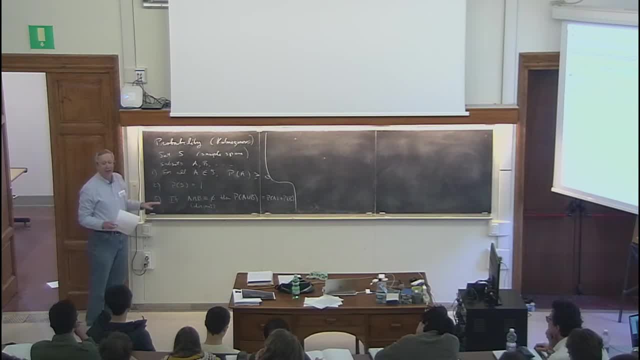 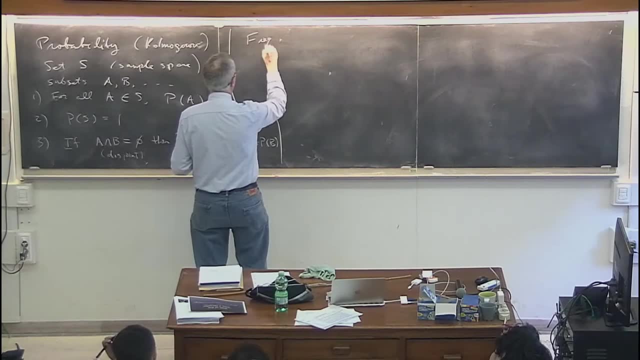 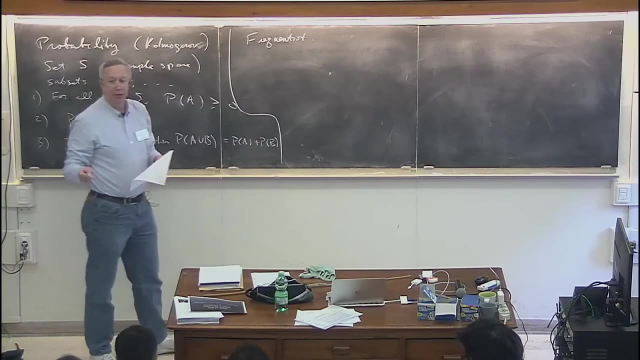 I don't even have to say what the elements represent, But there are two important interpretations of probability, And so one is what I will call frequentist, And in this interpretation of probability, the elements of the sample space represent possible outcomes of a repeatable experiment. 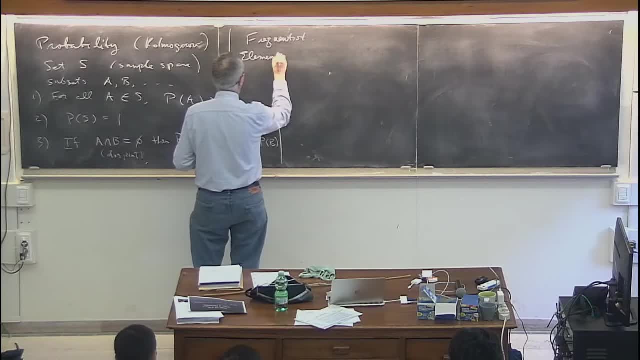 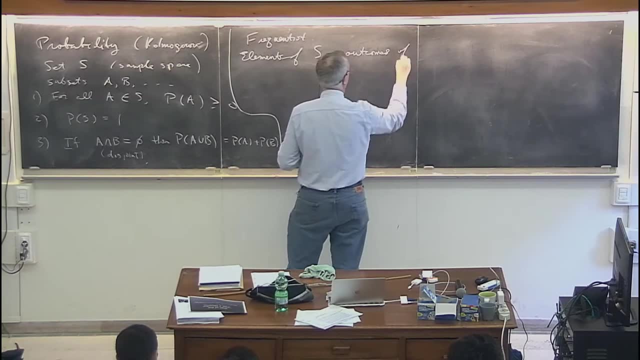 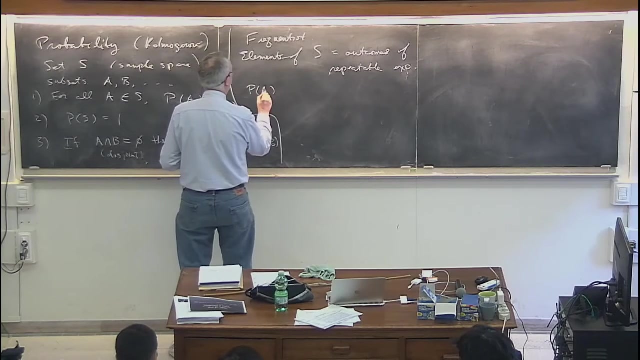 Okay, So I'll say elements of S are outcomes of a repeatable experiment or observation, All right, And we simply say that the probability that you would assign to some subset of those outcomes, so A could here represent an individual outcome or a subset of the outcomes. 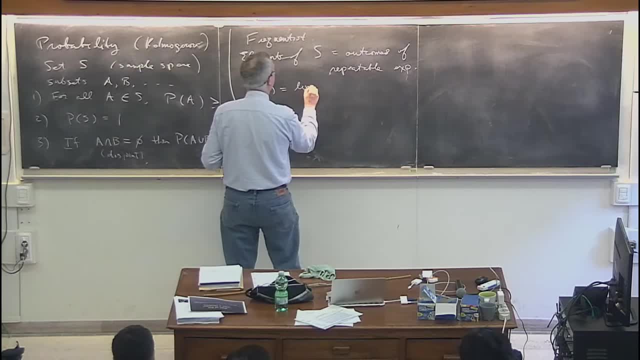 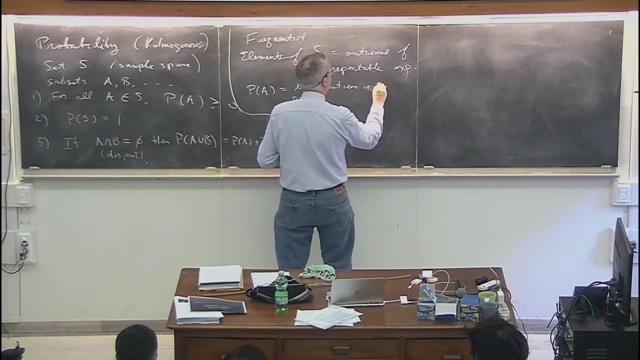 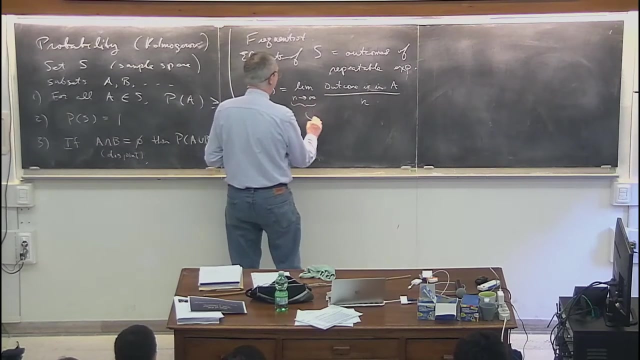 and you simply say that it's the limit, as you repeat the experiment a large number of times, or an infinite number of times in the limit that you repeat the experiment an infinite number of times. What is this supposed to mean? Limit, Limit as N goes to infinity. 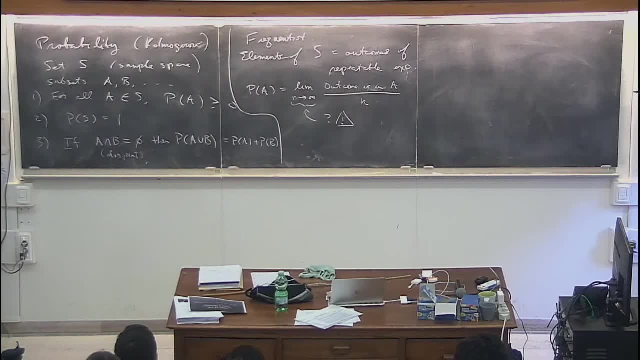 of repetition of an experiment. That's not a mathematical limit in the sense that you would define it rigorously, But nevertheless, this is the notion that we have in mind when you interpret probabilities in the frequentist sense, And it's the interpretation of probability. 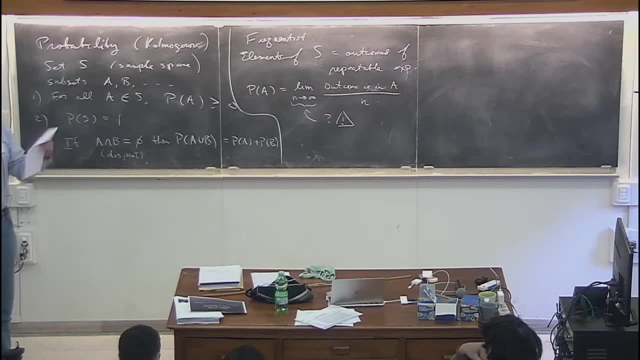 that you would have in mind in the ordinary- I'm going to put that word ordinary in quotes- Copenhagen interpretation of quantum mechanics: All right. So it's also very natural for particle mechanics, but it's also very natural for particle physics because we have this notion. 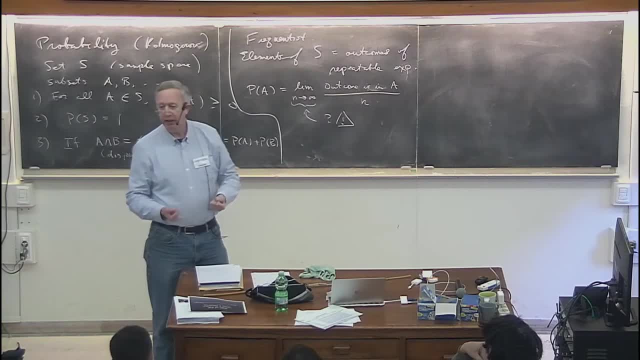 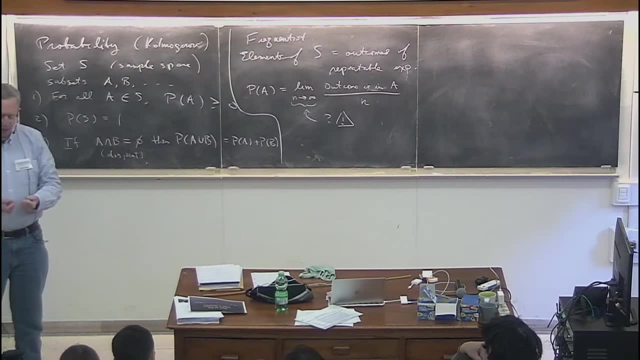 that we can say collide together protons an arbitrarily large number of times. There seems to be no particular limit to the number of times that we could repeat an experiment And furthermore there's no reason to believe that it should be any different, So it's an identical experiment. 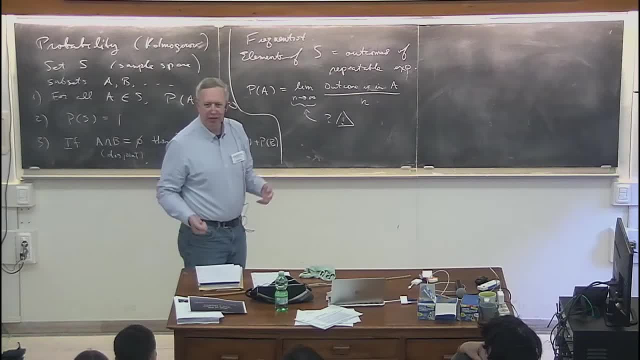 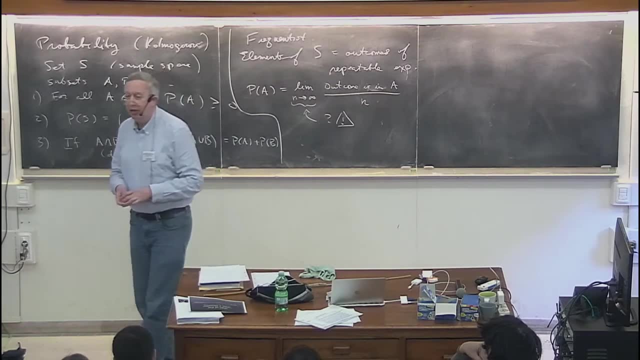 every time we collide together two protons at the center of mass energy of 13 TeV Right. On the other hand, there are many areas where you would naturally want to use something like, say, probability, but where this frequentist interpretation. 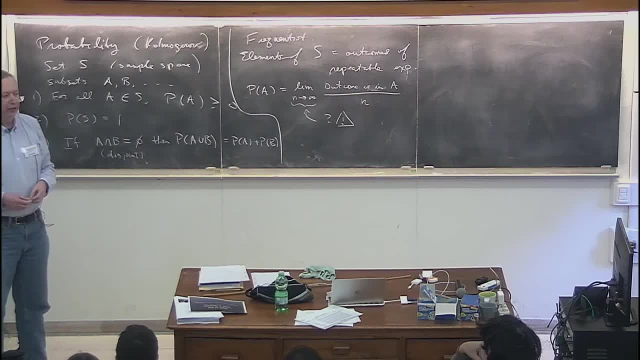 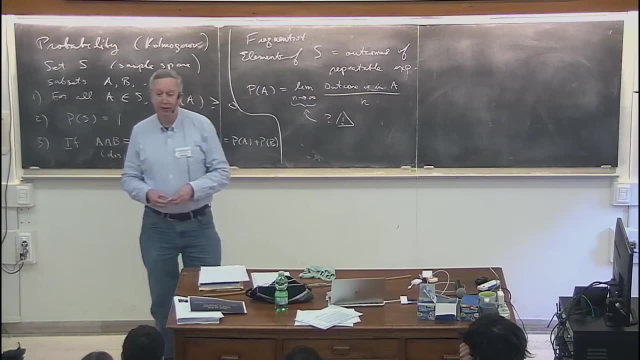 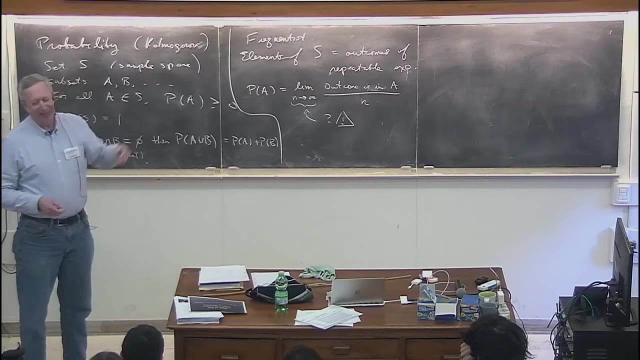 seems completely inappropriate. So suppose you wanted to use probability to quantify whether you thought that some theory like supersymmetry is correct. What's the probability that Susie is true, Or what is the? I have to change my example that I used in my course last fall. 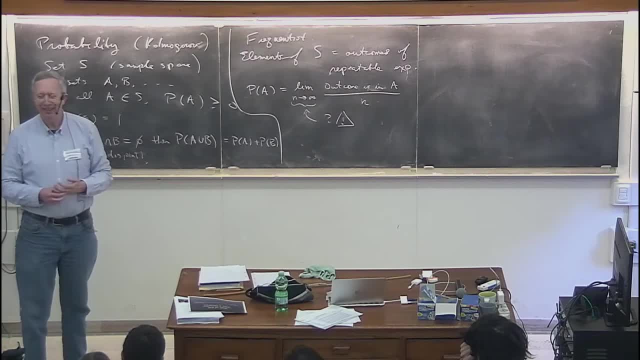 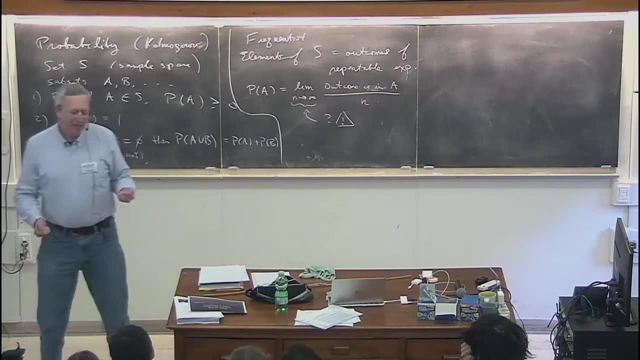 I said what is the probability that Donald Trump will be elected. So I'll say what is the probability that Donald Trump will be elected to a second term, or So you see that probabilities can be updated as more evidence is acquired. Susie will either be true or not. 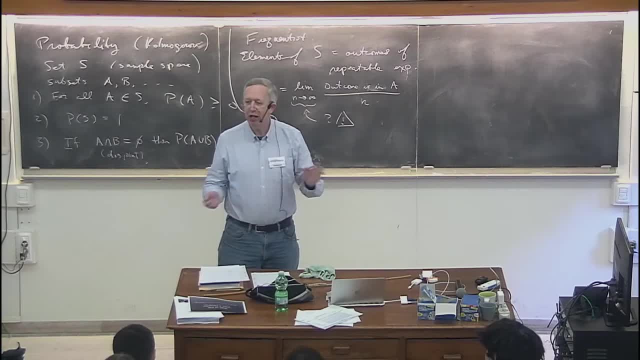 And no repetition of any experiment is going to change that. So, therefore, the fraction of times that Susie would be true upon repetition of any observation would either be 0 or 1.. But we don't know which. But nevertheless we would like to use probability. 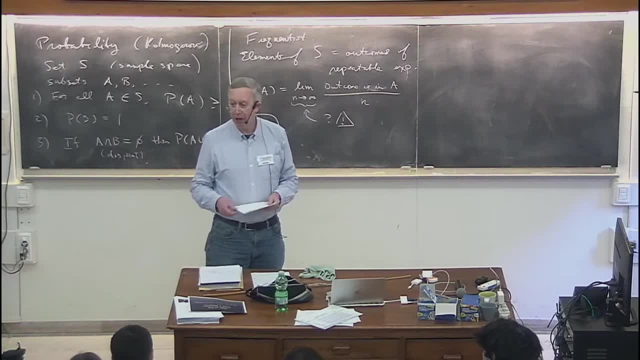 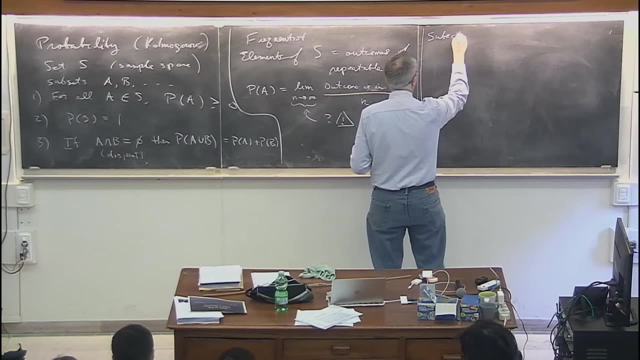 to quantify our degree of belief that certain hypotheses are true. And so that leads us to our second important interpretation of probability, which I'll call subjective. It's also called Bayesian for reasons which will become clear, And so there we say that the elements of S 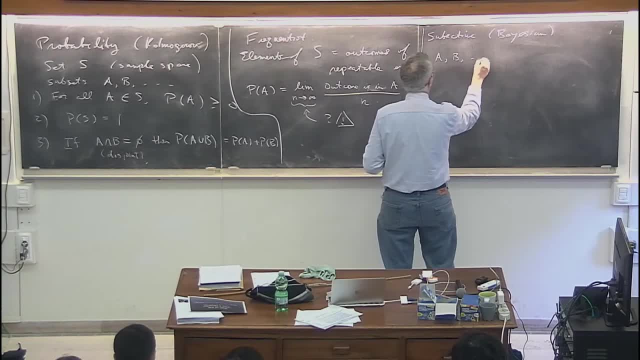 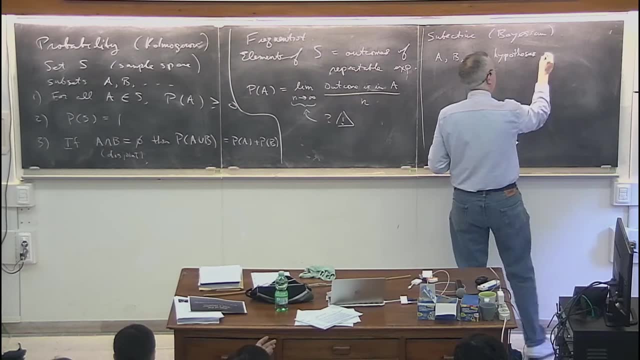 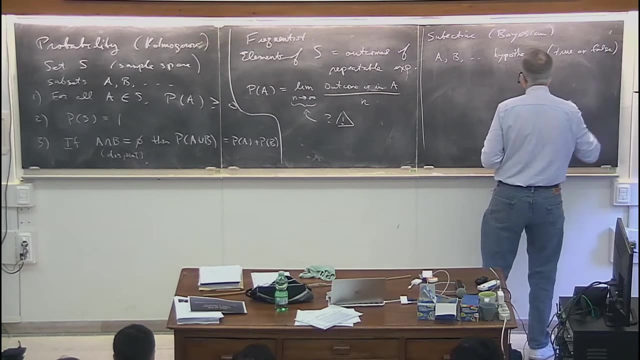 so A- B are hypotheses. For now I'm just going to say that a hypothesis is a statement that is either true or false. I need to refine that a little bit later, And then I'm going to interpret the probability that I assign. 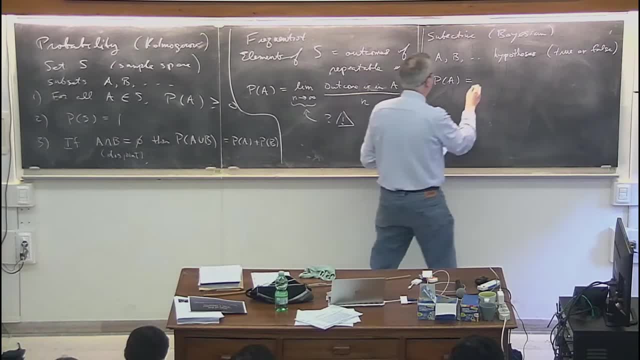 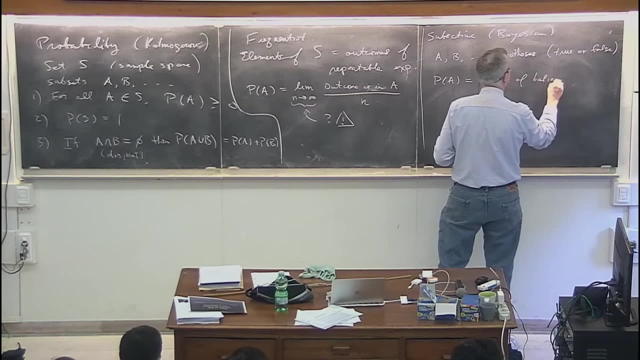 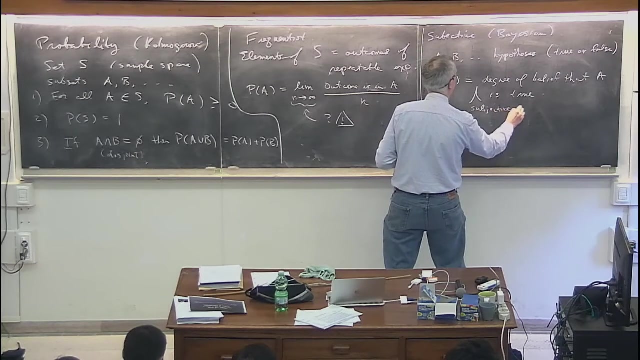 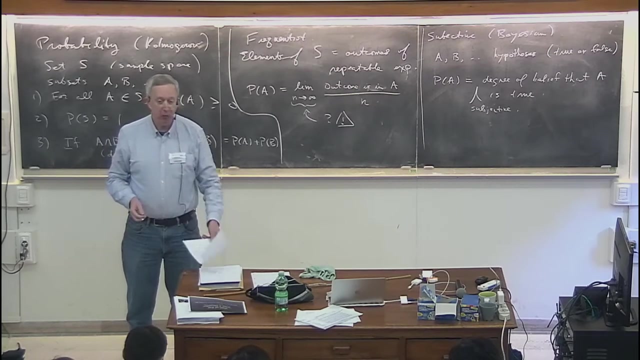 to a particular hypothesis or subset of hypotheses, is my degree of belief that it is true, And this is necessarily, let me insert here the word subjective. And so you might initially wonder whether or not that could be useful in a scientific discussion, And it is. 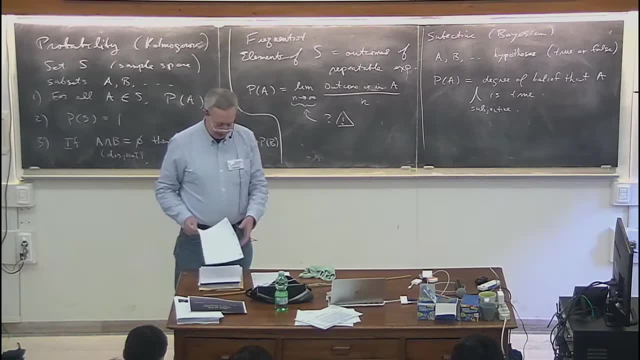 It turns out to be very useful, in fact. Okay, so those are. that's some sort of axiomatic definition of probability, where we don't insist on what the elements mean And then, to make it useful, we can either interpret probability as a limiting, 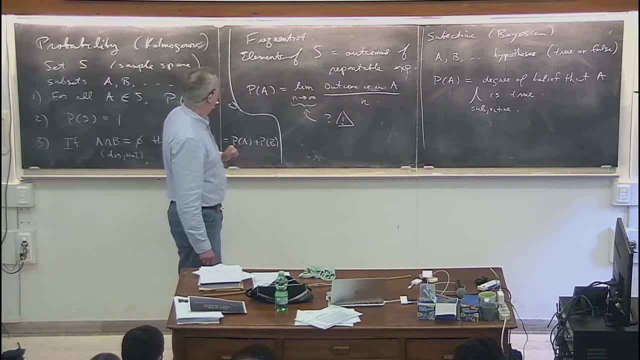 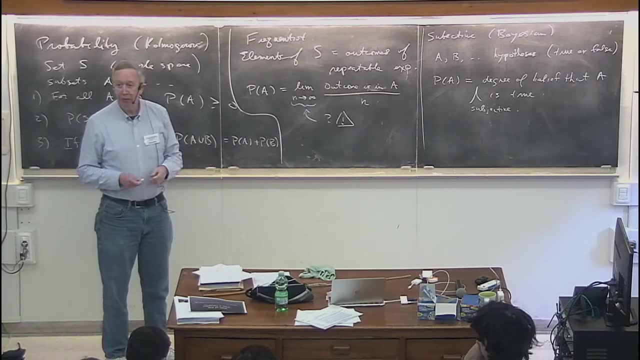 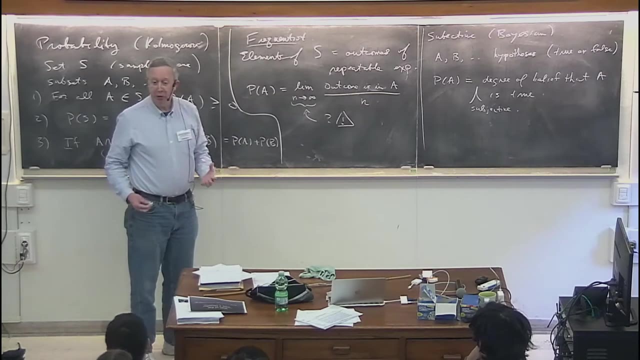 frequency or as a degree of belief, And I think it's fair to say that the vast majority of statistical tools that we really use in analysis of particle physics data is mainly frequentist. But this seems to preclude addressing some of the really important questions, like 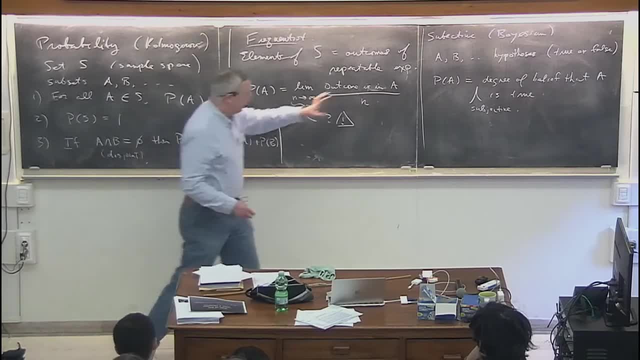 do? I believe that my theory is true And to address those sorts of questions, we need to have subjective or Bayesian probability. Okay, so let me erase that. I have to say, if you want to somehow discuss or debate or ask questions, we can either. 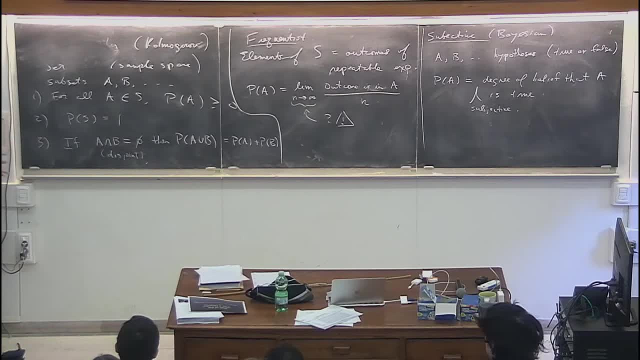 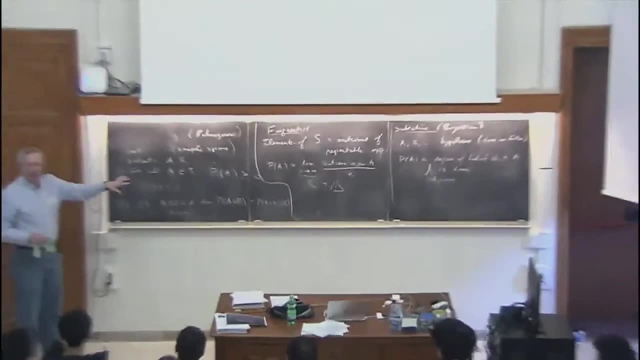 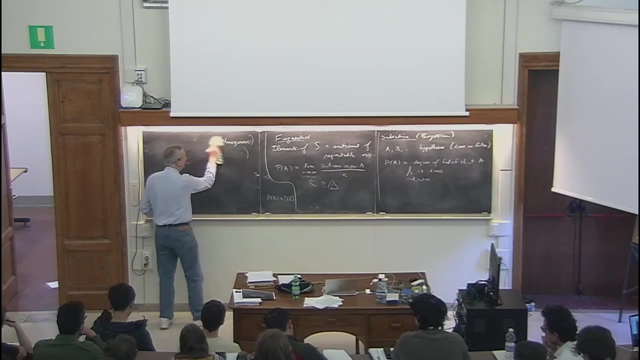 do that in the afternoon, but I presume we have time during the lectures as well. Alright, so this is usually a point in the discussion that people like to debate. So you know the utility or meaningfulness of various stages. Yes, 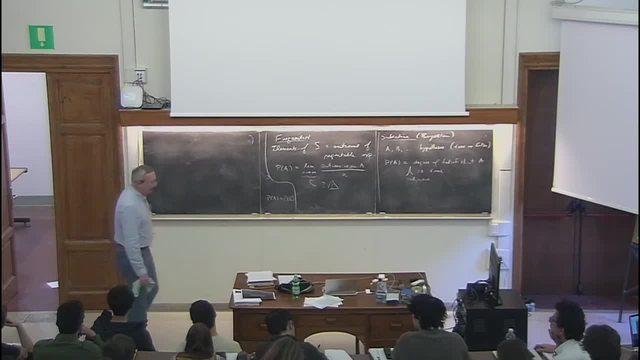 Yes, yes, So there's many others, but most of them boil down to different flavors of these. Alright, So you can get somehow probability based on the idea of some sort of symmetry, that if you have entities that you deem to be equivalent in some sense, 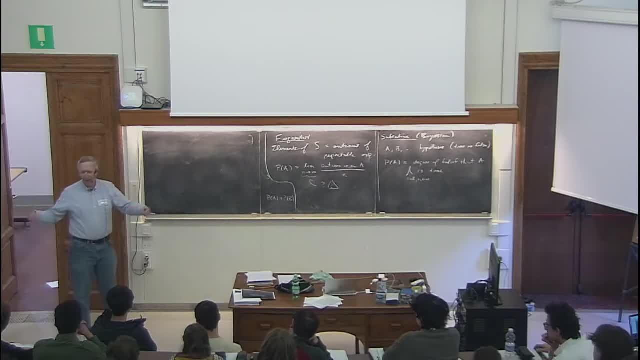 you could assign an equal probability to one. based on that sort of symmetry, You could also talk about a type of subjective probability that, Okay, here's a good one. What's the probability that the billionth digit of pi is a seven? What do you think? 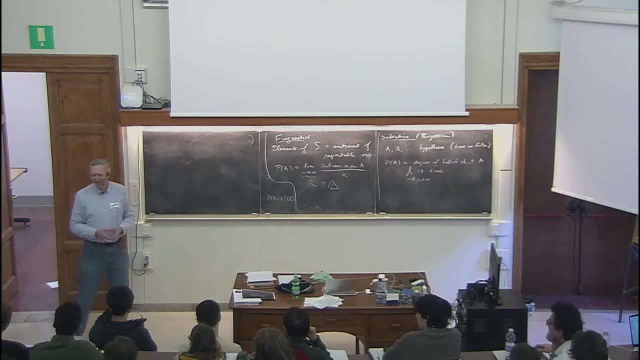 Okay, But it either is or it isn't right. So, furthermore, once you define what pi means, then whether or not the billionth digit is seven or not can be deduced from logic. Alright, So you could have a version of subjective probability. 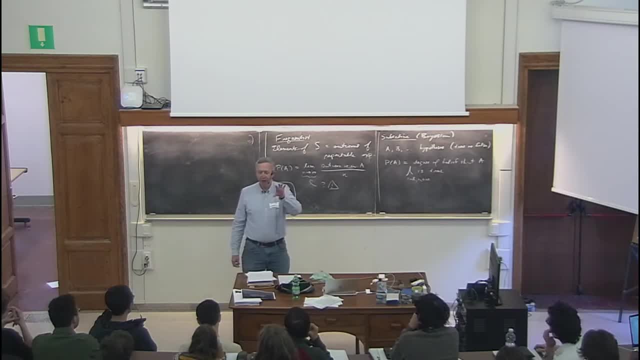 that if something is true, if something has a certain probability, then anything that logically follows from that must have the same probability. Alright, And so then you would get into trouble. So there are different flavors of these different types of probability. Yeah, 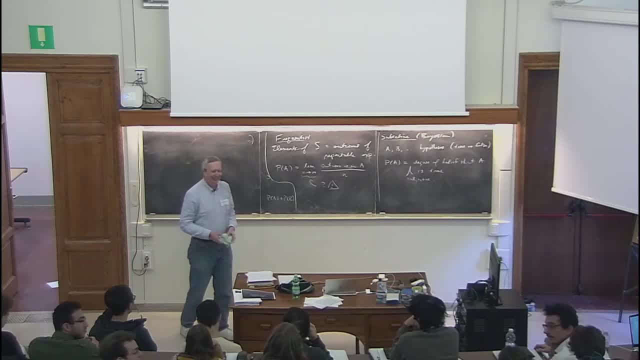 Right, More, uh, yes, So in general, the two interpretations are going to lead to two really distinct schools of statistical inference using different tools, So what's called the frequentist statistical school and Bayesian statistics. And uh, there are certain. 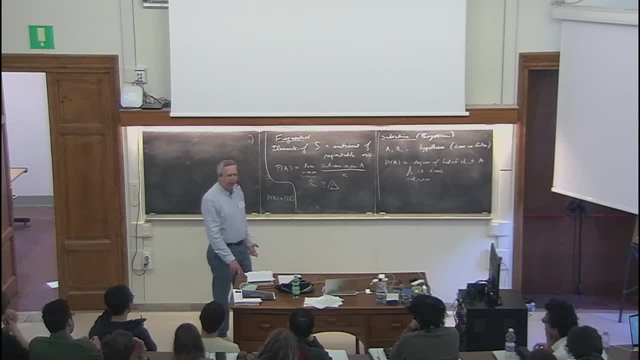 there are cases, I would even say many cases, in which numerically the results of the two schools are the same. They lead to the same set of numbers, But they would be interpreted in different ways. And there are other cases where the two 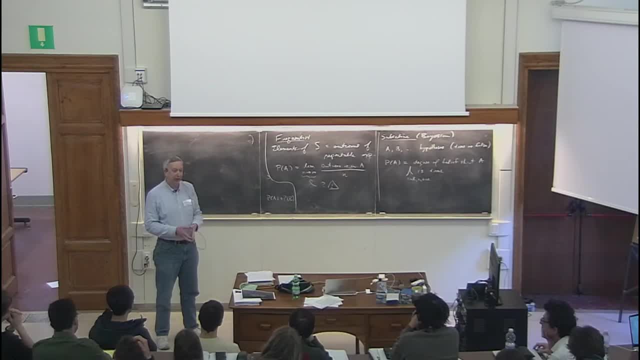 approaches actually lead to completely different numbers. So uh, and that would be in an analysis of the same underlying theory. So, in other words, if you wanted to say uh, do an analysis where you tried to compare the predictions of a particular 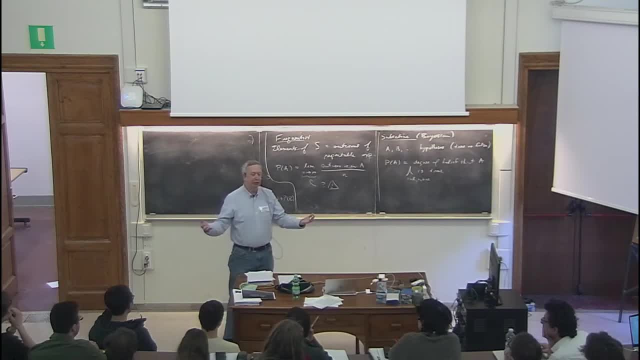 supersymmetric model to the data emerging from ATLAS. you could do it in either of the two schools And you could come to different conclusions. In the limit that the data sample becomes very large, they converge, But we'll see why, And that is that this Bayesian. 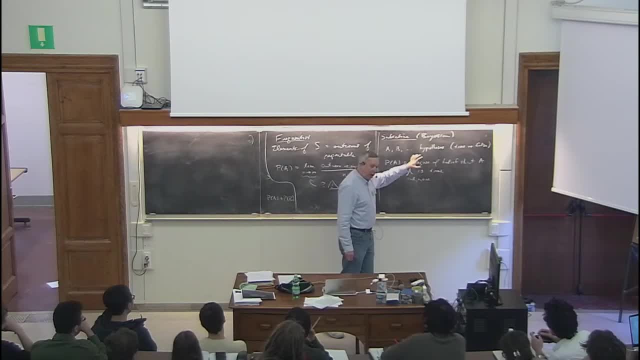 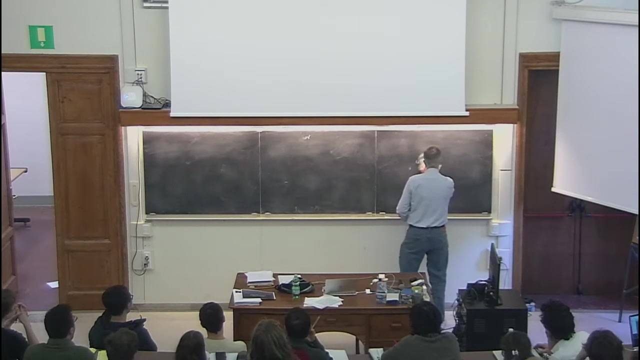 approach is necessarily going to require subjective input And depending on how you adjust that subjective input, you could get different results. We'll see this in just a second. Okay, good, I just want to mention quickly a few more things about probability And I 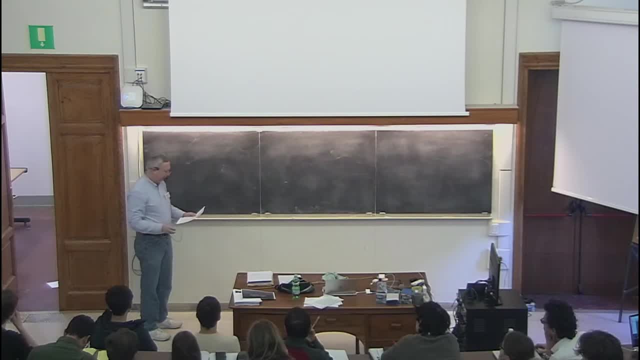 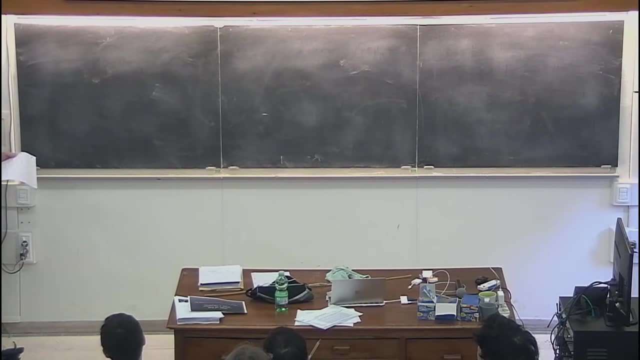 apologize that this is just a review of things that you probably know. I had those Kolmogorov axioms, but there's essentially a fourth axiom that I need to put down and that is to define what is called conditional probability. So here, 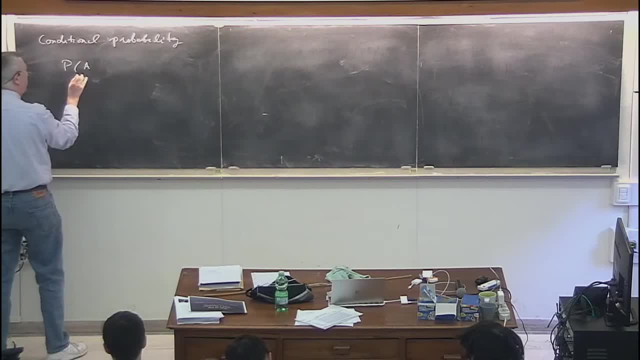 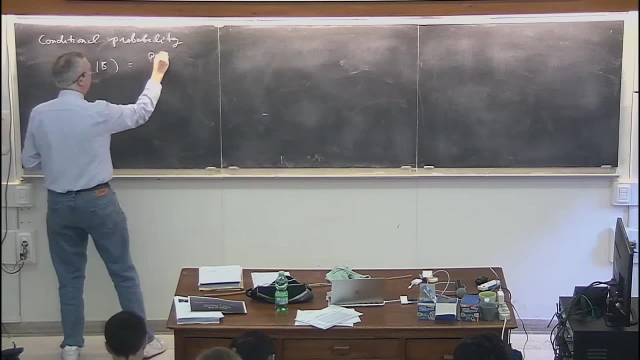 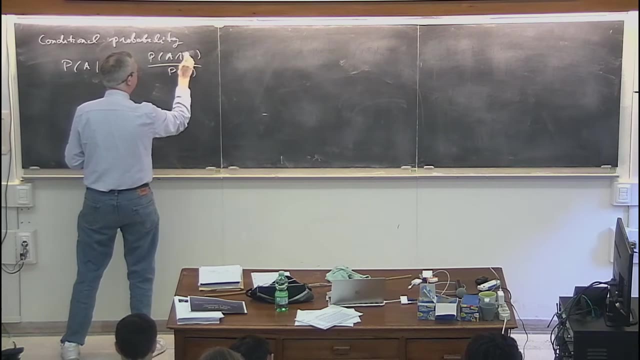 if I have two subsets, A and B, I will write the probability for A given B, so the conditional probability of A given B. This is defined as the probability of the intersection of A and B divided by the probability of B. So the idea here: 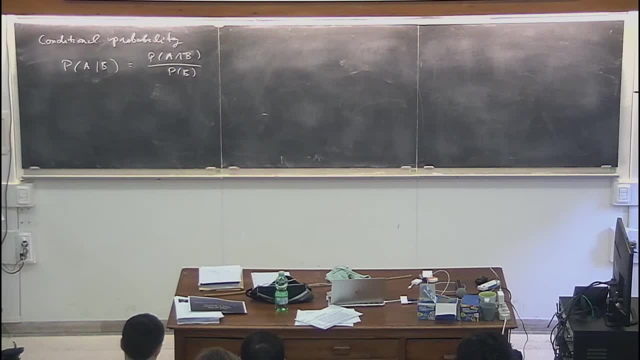 is the following: is that if you start out with some sample space S, some set of all possible outcomes, but then suppose somebody comes along and says: no, actually I want you to restrict that sample space to some smaller subset B, So this is a restriction. 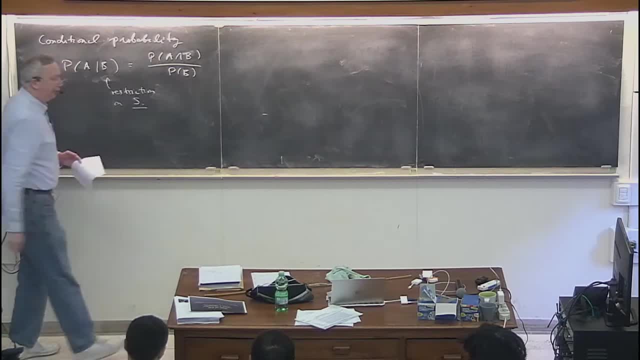 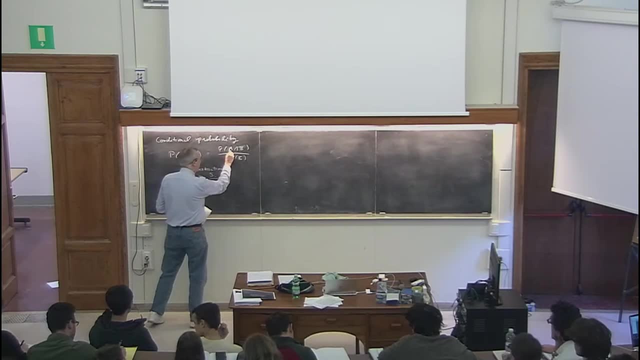 on the sample space S. So what that says? this is defined to be the probability of the intersection of A and B. This intersection operation can be understood as the logical AND. So, in other words, suppose you're rolling a die and you want to know what's the 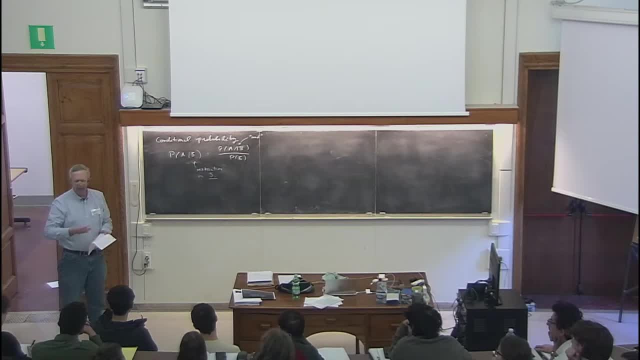 probability of getting a number less than three And you, then somebody says, oh, but by the way, I know it's an even number. So what's the probability of getting a number less than three, given that you know that the outcome is even? You would work that out. 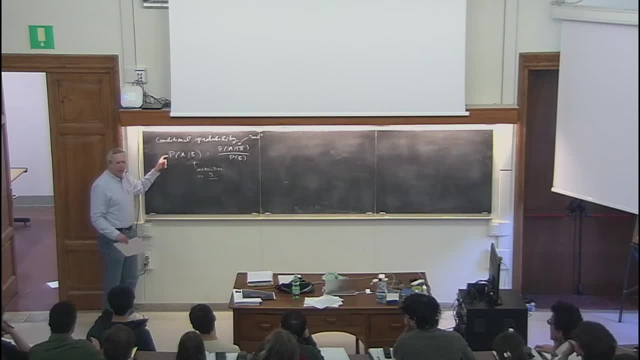 with this formula. That cannot be derived from the Kolmogorov axioms. That has to be taken essentially as a fourth axiom. It's a definition, Alright, Just a further thing on that. I want to say that two subsets A. 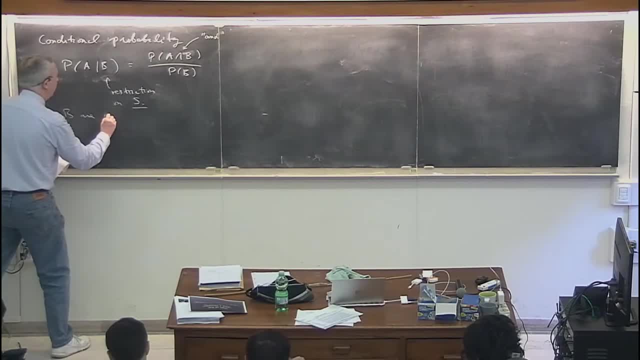 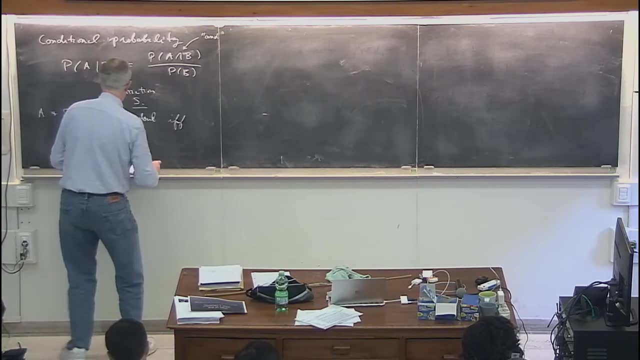 and B are independent if, and only if, the probability for both of them occurring, which is to say the intersection, factorizes into the probability of A times the probability of B. So that's also just a definition of what I mean by the word independent. 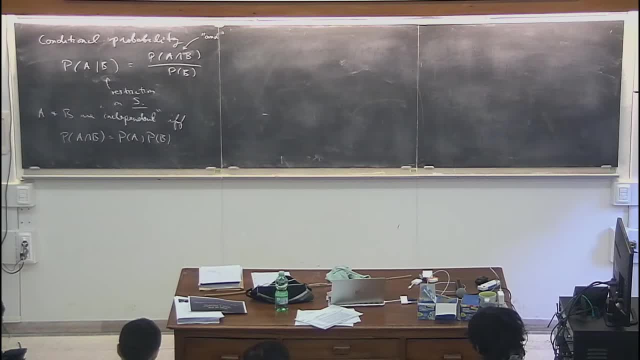 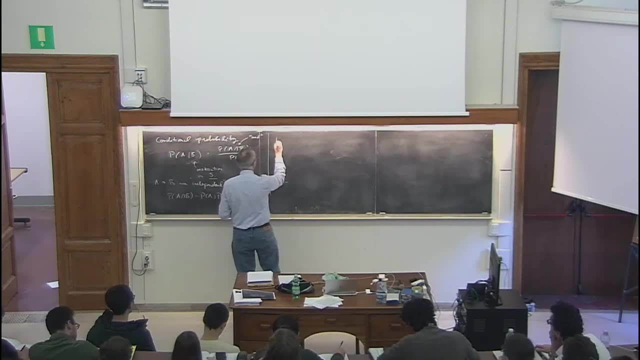 And you might say, why do they call that independent? Why don't they call that factorizability or something like that? But it makes sense if you think about this in the context of conditional probability, Because if you have two subsets that are independent, so let's say 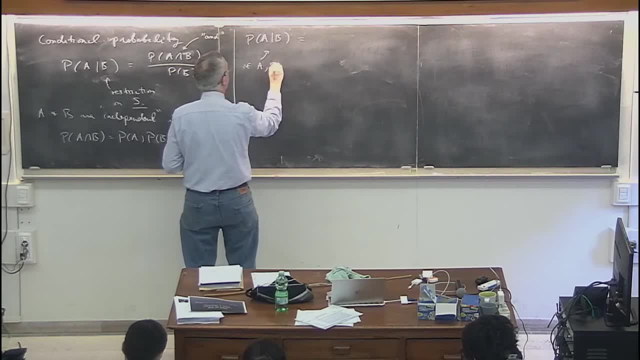 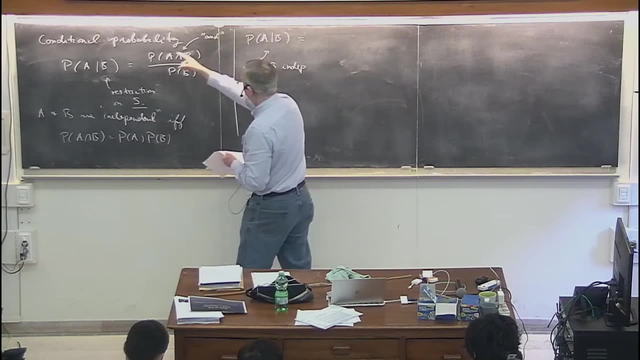 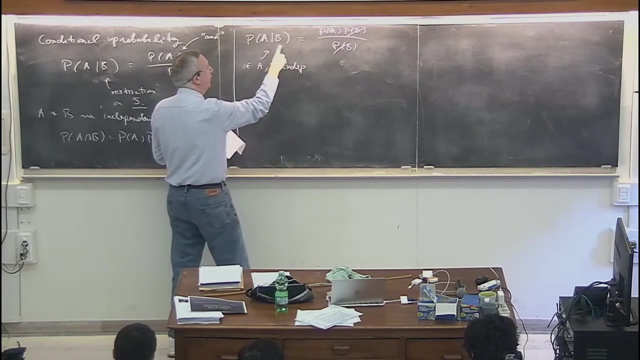 if A and B independent, then what is this? The intersection is just going to be the product. The probability of the intersection is just the product of the two probabilities, And so what that means is that imposing the restriction of B has no influence on the probability. 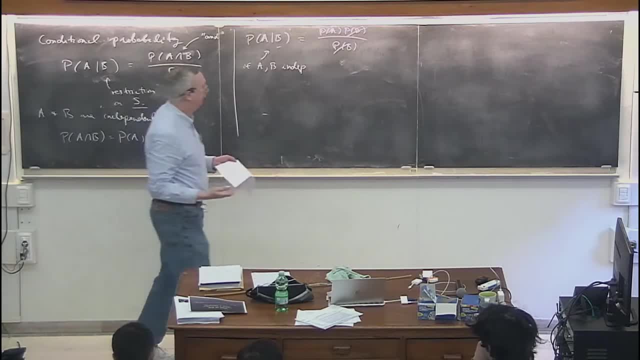 for A, So in that sense this word independent makes sense. Imposing the restriction of B didn't change the probability for A, So this is for A and B independent And it would work equally well the other way. So I mention that because 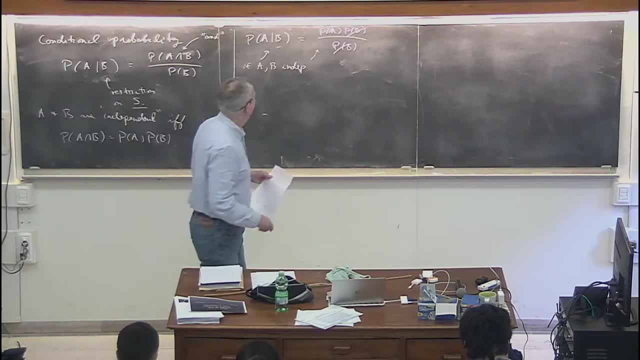 that's going to come up Now. next, Bayes' Theorem, An important theorem that is satisfied by anything that you deem to call a probability, regardless of whether you interpret it as a frequency or a degree of belief or anything else. 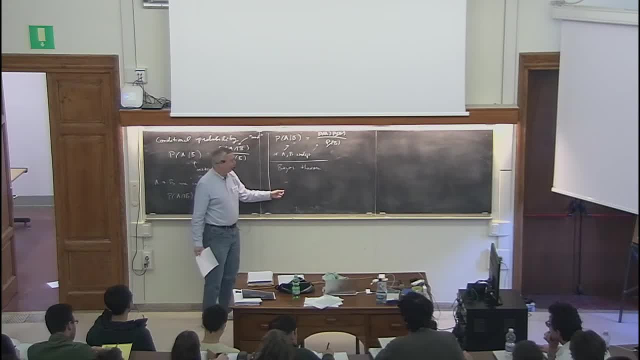 it has to satisfy what's called Bayes' Theorem. Now you may have heard that there's a some sort of controversy and rivalry between the two main schools of statistics, the frequentist school and the Bayesian school, And you may think, ah well, surely that has 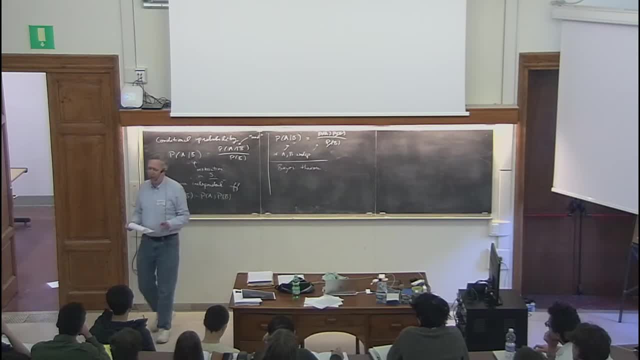 to do with some disagreement about Bayes' Theorem, And that's not true. Bayes' Theorem is a theorem And we can derive it in less than 60 seconds, So let's do that. So I have here that P of. 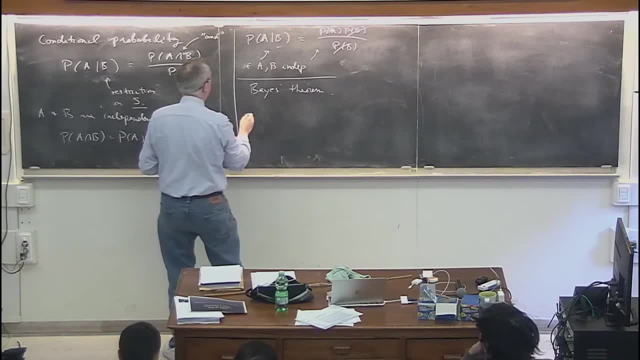 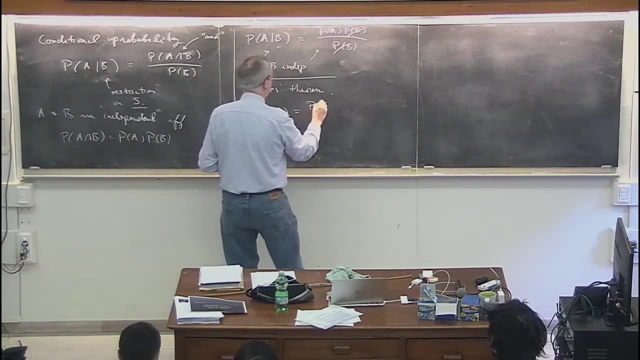 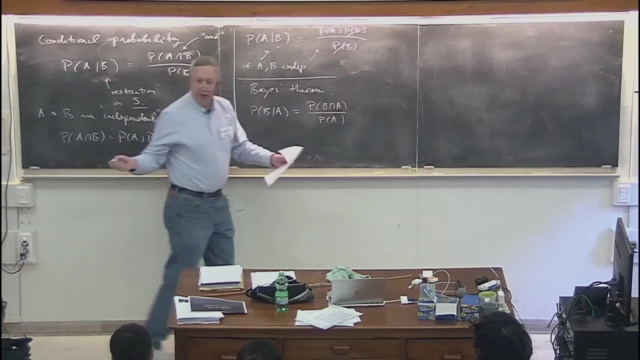 A, given B is defined to be that, And so therefore, if I switch the labels, I have that P of B given A is equal to the probability of the intersection of B and A divided by the probability of A. I've just switched. the labels Must also 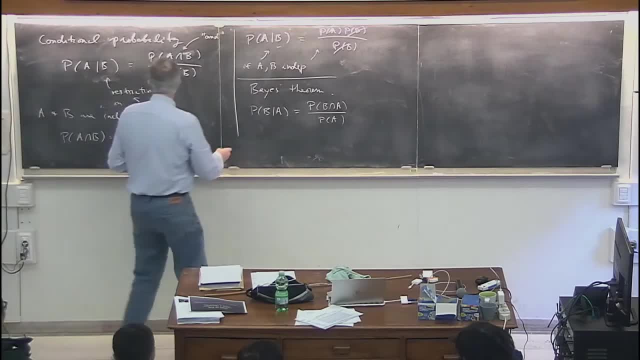 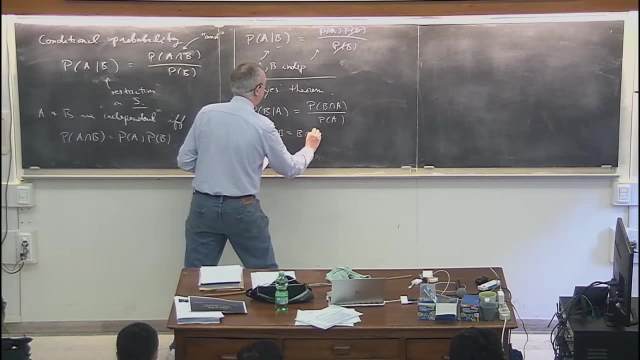 hold. But if you think about how set theory works, the intersection of A and B is the same subset as the intersection of B and A, Right? I mean, if there's A and there's B, it's that guy in both cases. 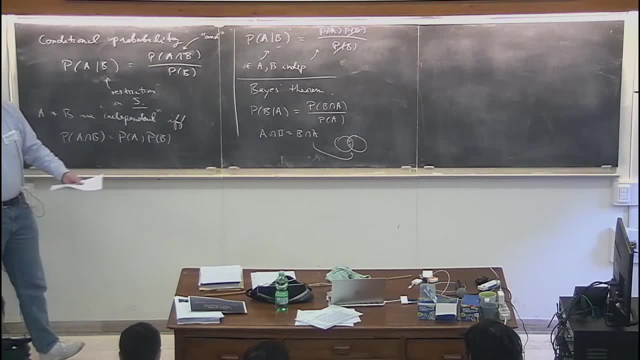 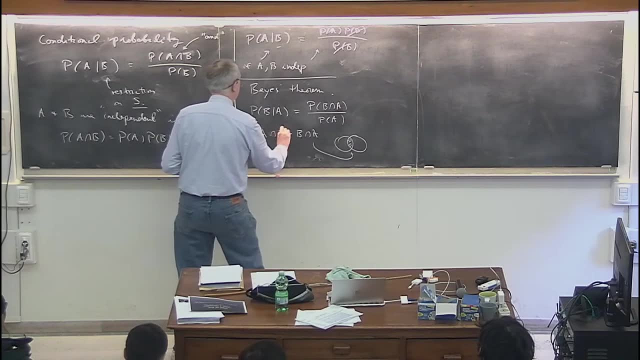 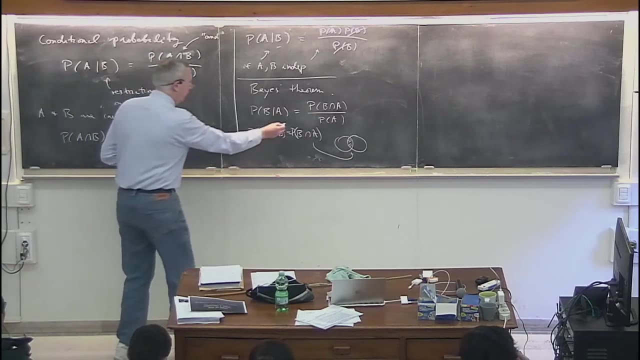 As so therefore, if it's the same subset, the probabilities of these two things must also be the same. So therefore I can say that the probability of that has to be equal to the probability of that in either order, And so what I can do is I can solve this equation. 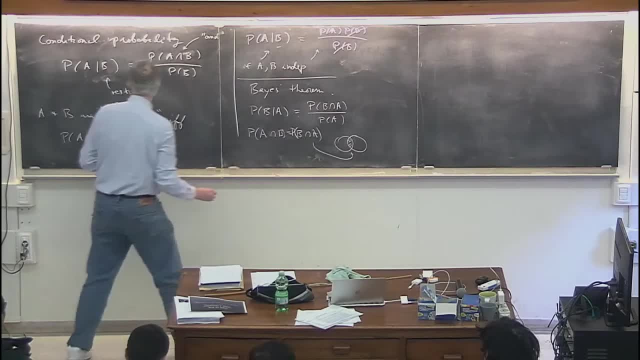 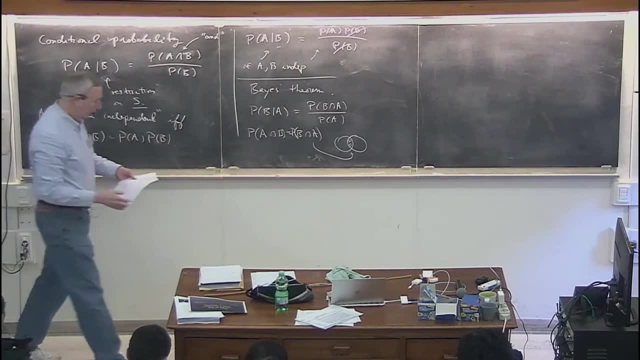 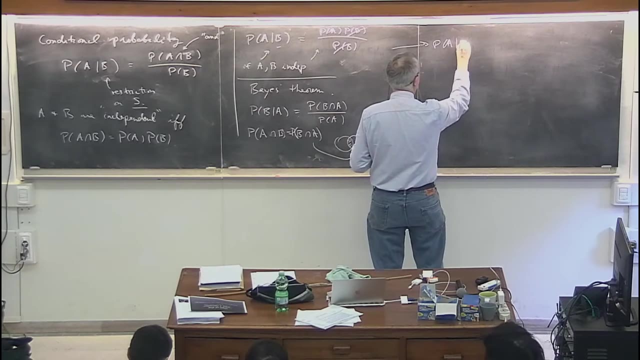 for the probability of B intersect A and this one for the probability of A intersect B, and set them equal, because they must be equal, And then I'm going to rearrange the result, and the result is that the probability of A given B 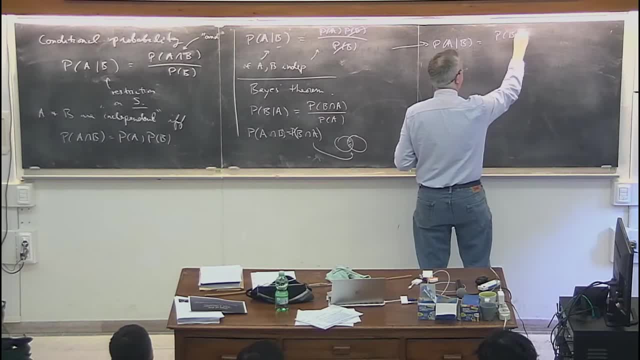 is equal to the probability of B, given A times the probability of A divided by the probability of B, And that's Bayes' theorem. And like I say, that's a theorem, There's no real disagreement about it. You can read it in: 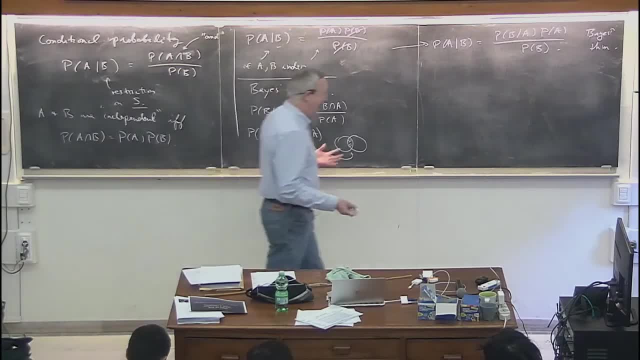 this article by paper by Bayes that was written in 1763, and you can Google for the original paper. It's actually fun to look at. just because the language has changed so much, You'd hardly know what you were reading actually. 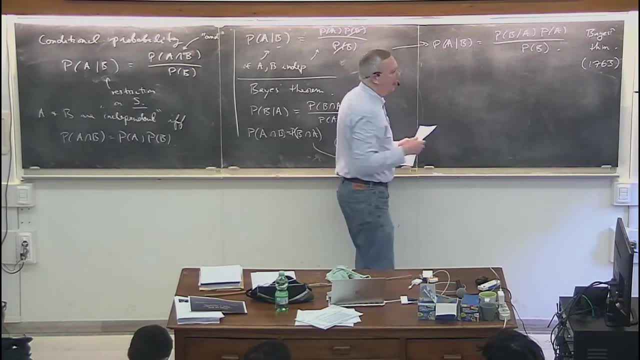 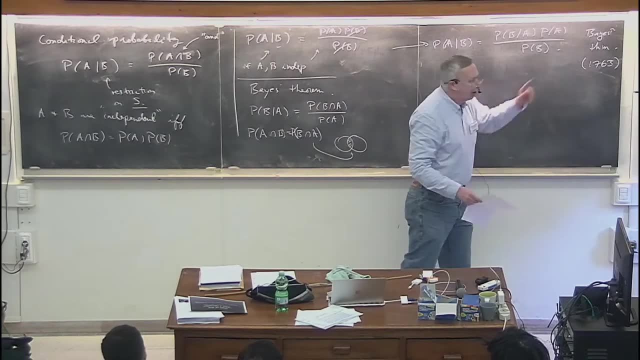 And Bayes' theorem will turn out to be essentially the fundamental equation from which we get Bayesian statistics. But the real controversy doesn't have to do with Bayes' theorem. It has to do with whether or not you deem the subjective interpretation of probability. 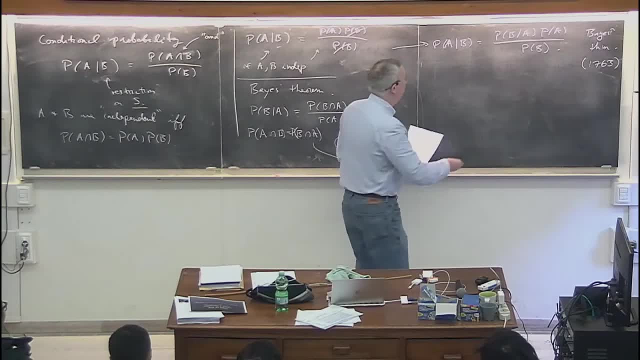 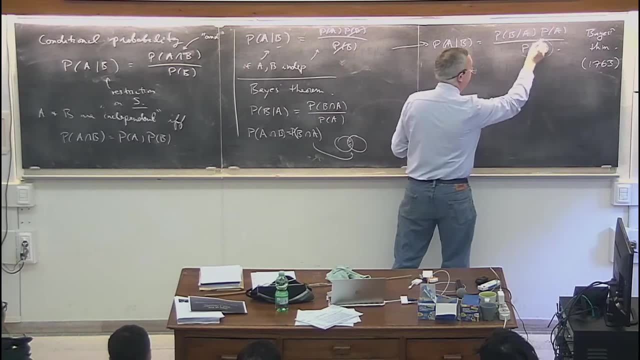 as being meaningful. I want to mention just really quickly before we go on, that this Bayes' theorem is very often combined with another theorem that can be used to rephrase this P of B, And so let me explain how that works. Suppose that we start off. 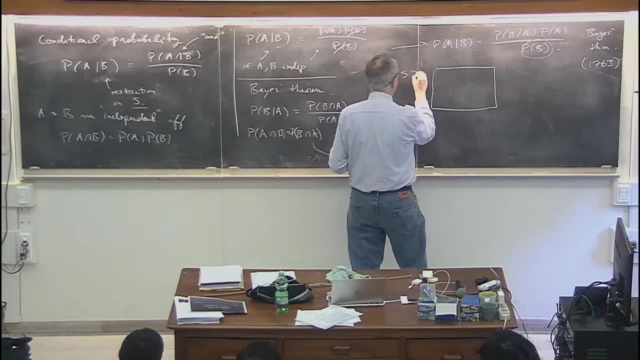 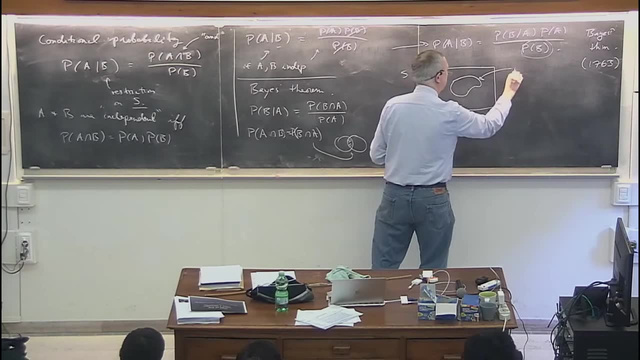 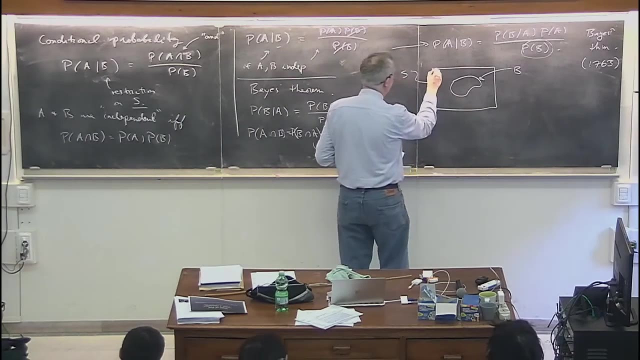 with the sample space. so here's S, and I restrict that sample space with this smaller subset B. So that's the restriction that you're going to impose. Now, very often it is possible to decompose the sample space into a number of. 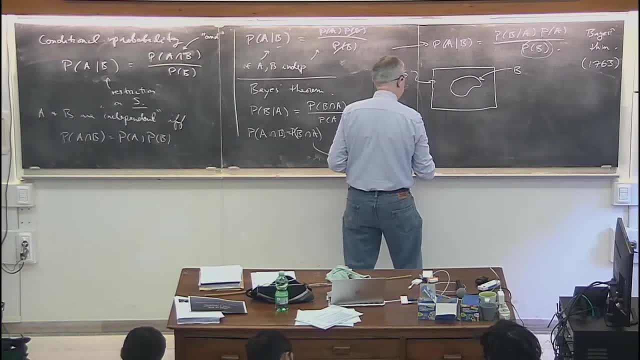 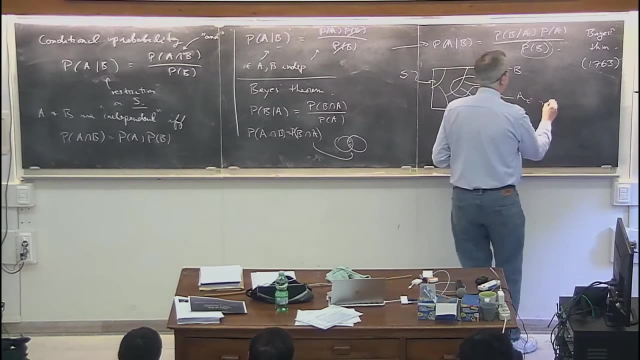 disjoint subsets And so I'll just draw those. Do I have colored chalk even? Yeah, good, Let's draw those like that. I don't know what to say. Okay, so suppose this is A sub i and I would have that the. 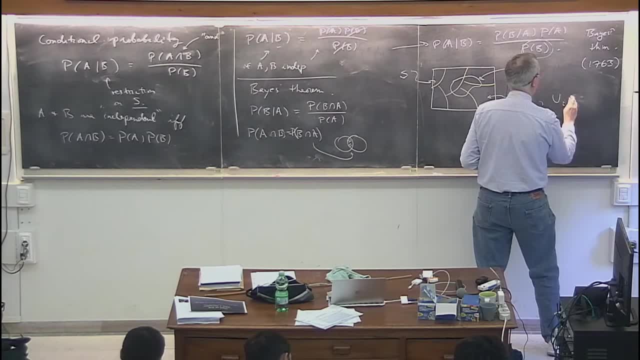 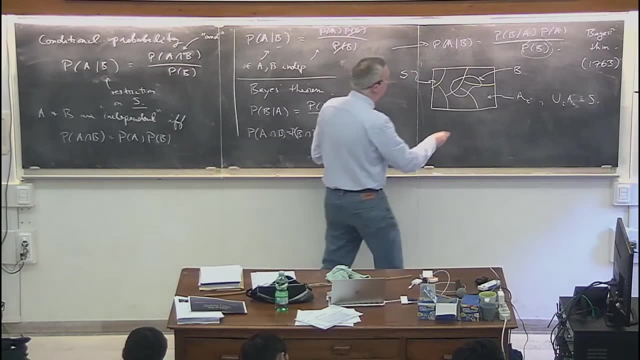 union of all of those A sub i's gives me back the sample space. What I want to do is to write down an expression for P of B, this kidney shaped thing in the middle. Let me just do that graphically without bothering with the formal mathematics. 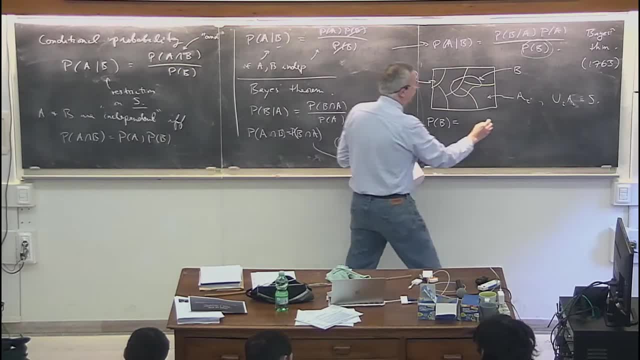 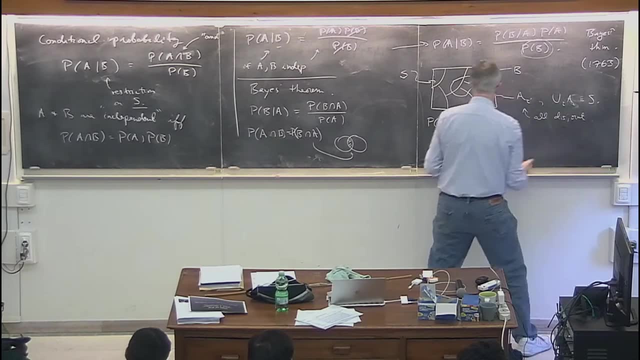 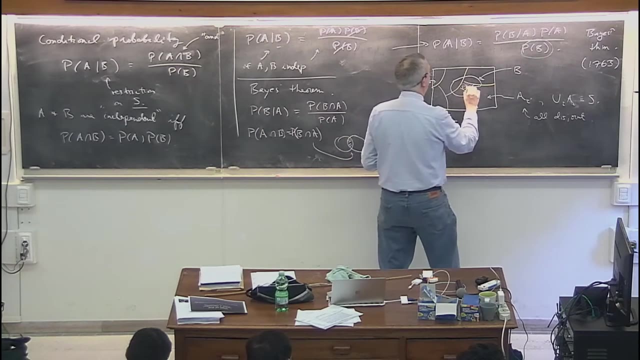 Basically, if all of these A sub i's are disjoint, then this thing here, that, what is that? That is, simply make sure I say this right: that's the intersection of A, i and B. So that guy, there is B intersect A- i. 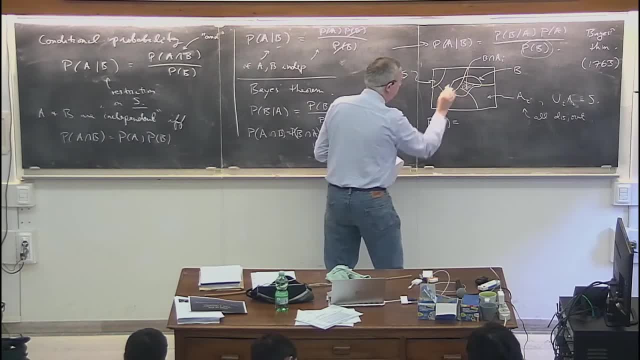 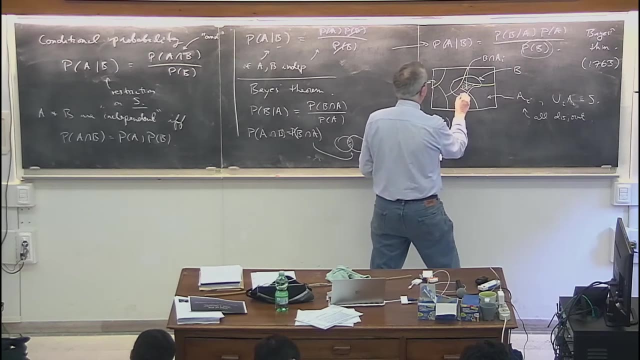 And those chunks inside B are also disjoint. So therefore, if I say that B is simply the union of these guys, how do I want to write this? That P of B is simply going to be B is the union of these subsets here. 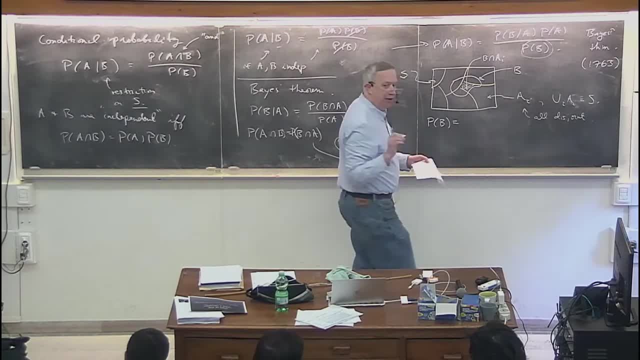 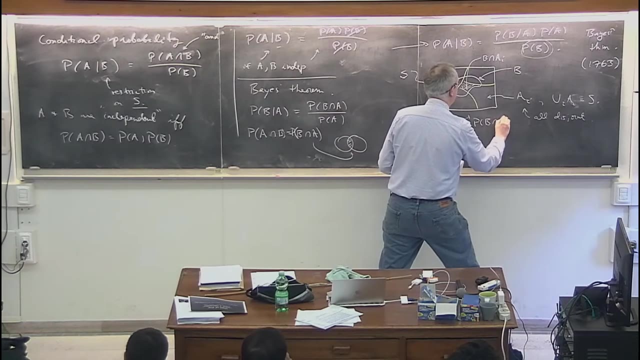 and because they're disjoint according to the third axiom of Kolmogorov, their probabilities add, And so, therefore, this probability is simply the sum over i of the probability of B intersect A, i. And then, if I go back to the definition of, 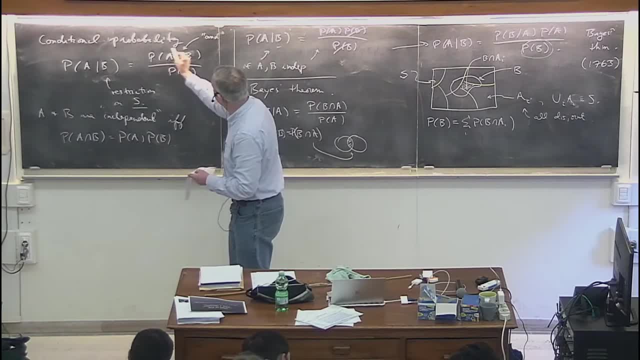 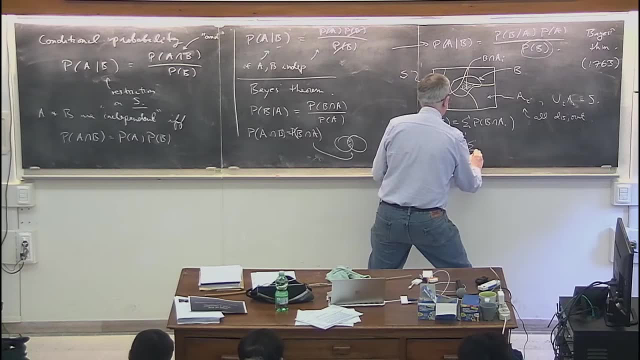 conditional probability, and if you would just solve it for, say, the probability of A intersect B, you'll see that I could rewrite this expression here as the sum over i P of B, given A, i P of A, i, And so that is what's called the law of total probability. 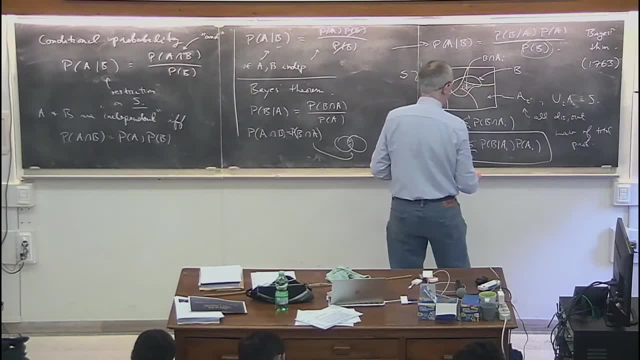 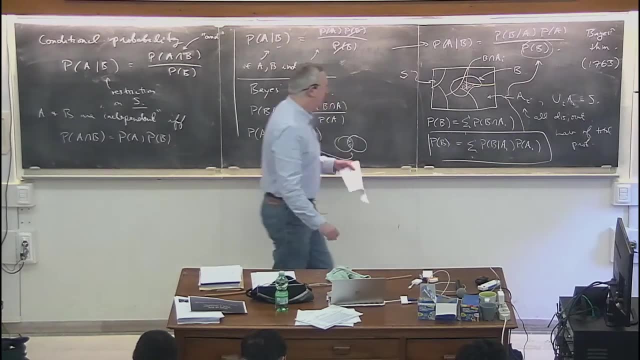 And it's very often used with Bayes' Theorem. Actually, I've got too many arrows here. It's used with Bayes' Theorem to replace the P of B that you see in the denominator there, So let me just rewrite Bayes' Theorem. 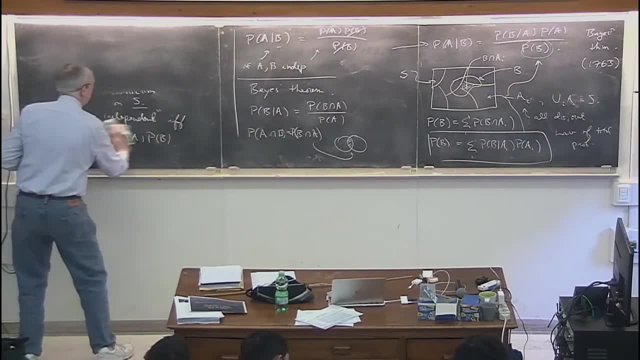 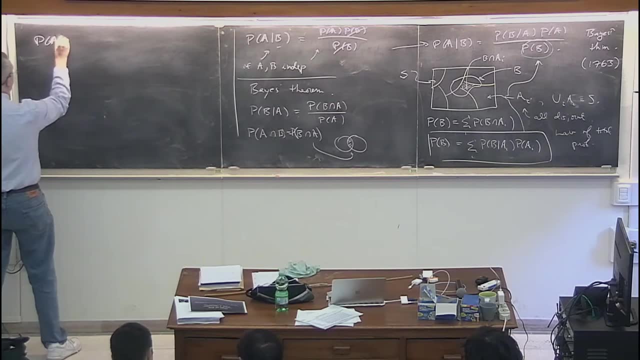 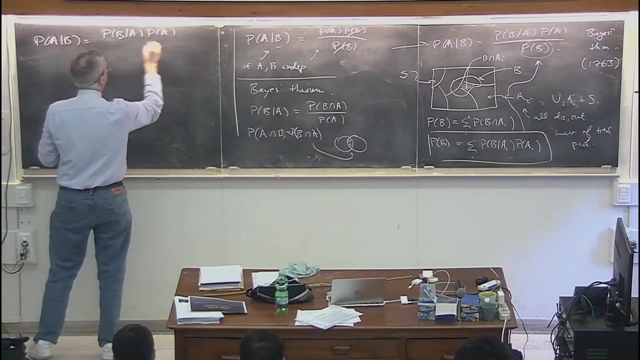 in the form that we will actually use it, And there is a homework problem that applies this. on your problem sheet for this afternoon, P of A given B is equal to P of B given A. P of A then divided by this thing in the denominator: 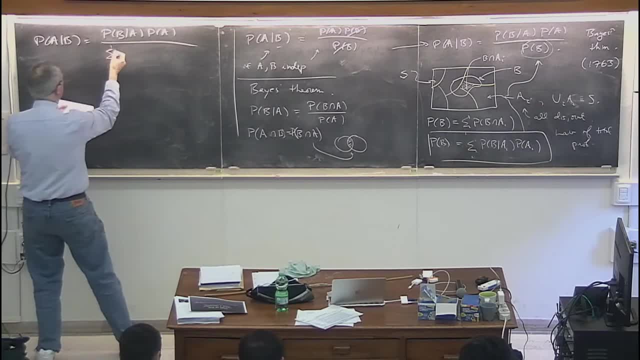 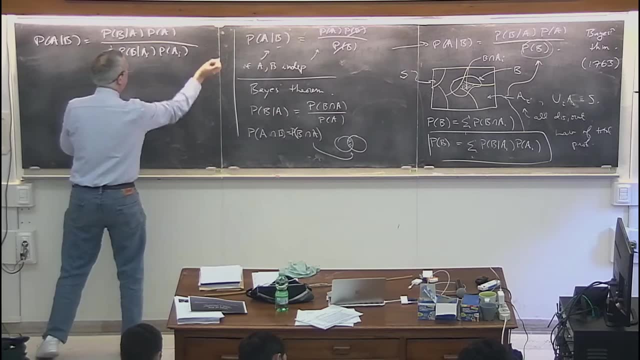 appears just as a normalization constant, if you will. P of B, given A i, P of A i, Voilà, Okay, so that's the version of Bayes' Theorem that we will come to know and love and actually use. 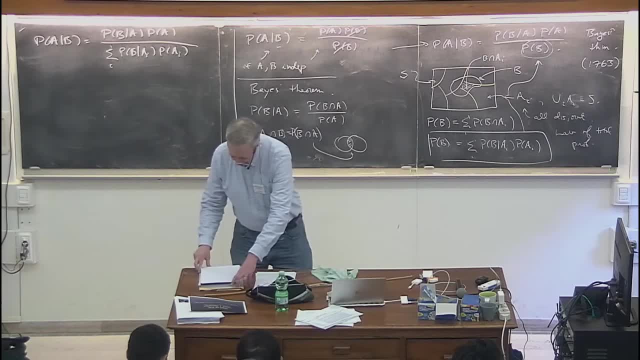 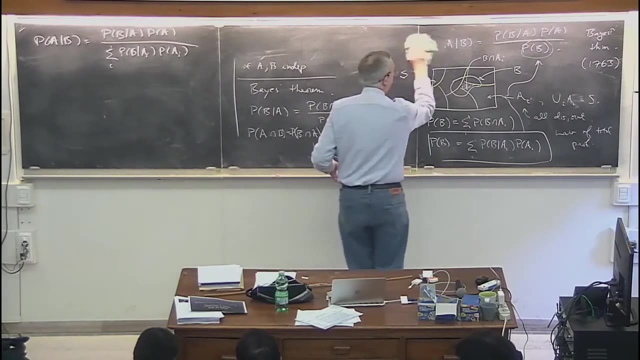 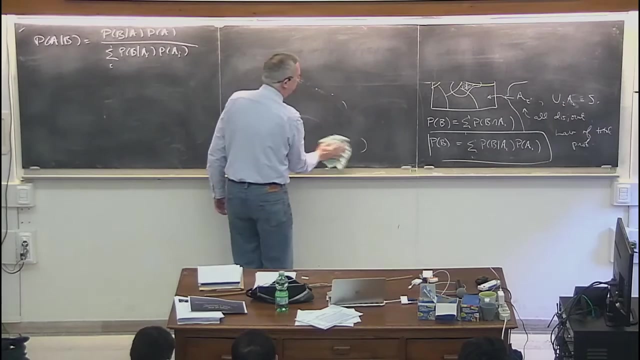 Alright, so before we get into the more the meat of things, I want to just spend one more blackboard of description of these two main schools of statistical inference, Because there's certainly a lot of confusion that emerges from discussions of statistical data analysis, And a lot of it has. 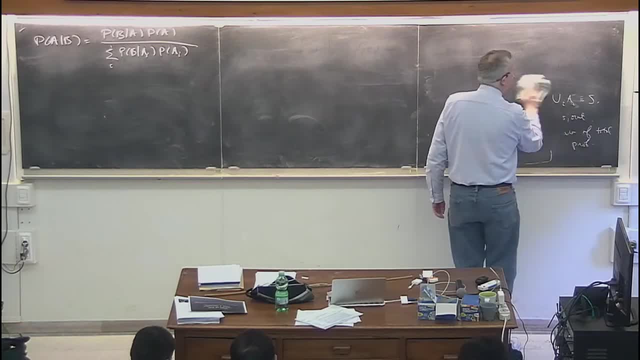 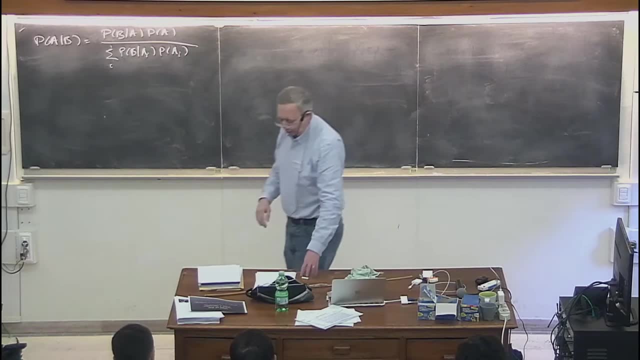 to do with starting off talking about a frequentist analysis and then getting confused and switching midway. So I want to make it clear as to what we're doing in a frequentist statistical analysis And what we're doing in a Bayesian statistical analysis. So 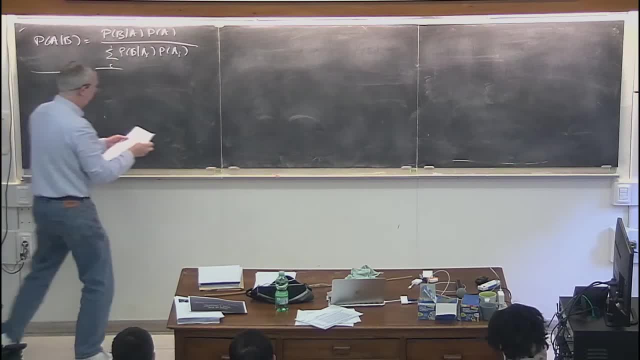 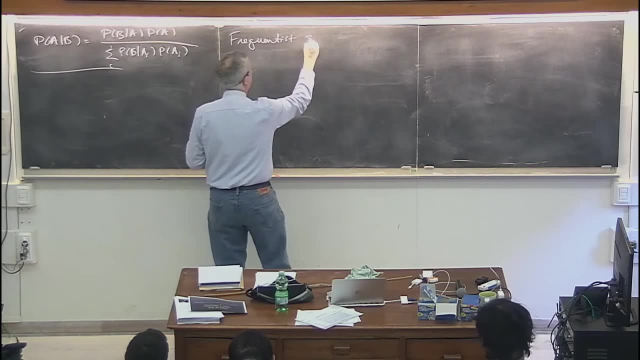 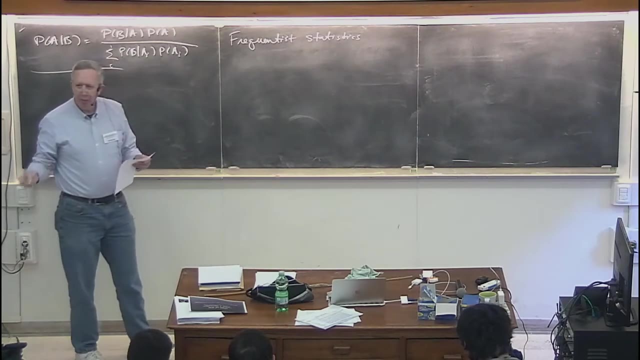 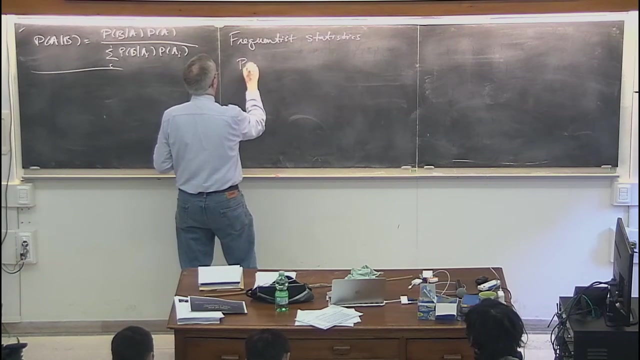 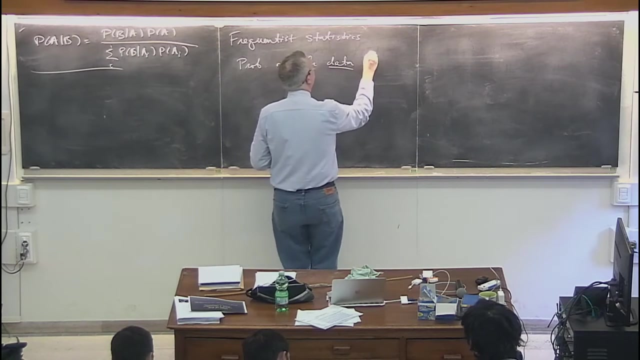 in frequentist statistics. I'll just say it here. I guess You only associate probabilities with the data, with the outcomes of repeatable experiments. So probability only for data, So outcomes of repeatable measurements, Alright. And so we define that using this. 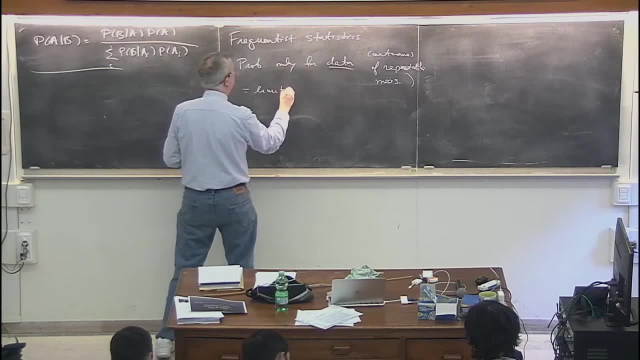 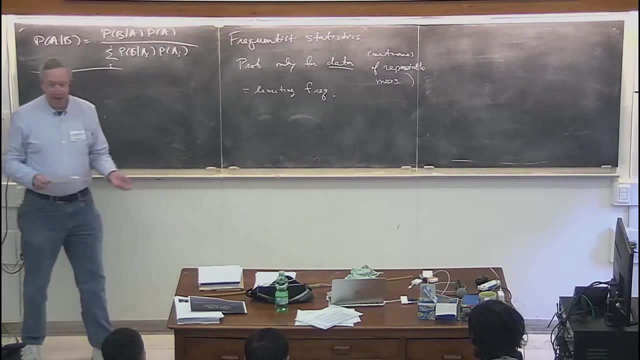 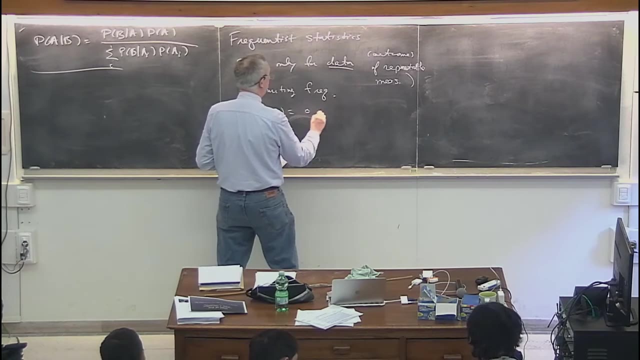 limiting frequency, definition that I had, interpretation that I had on the board Limiting frequency, And so that means that we're not allowed to say things like the probability of Susie being true that was equal to either zero or one, but we don't know which. 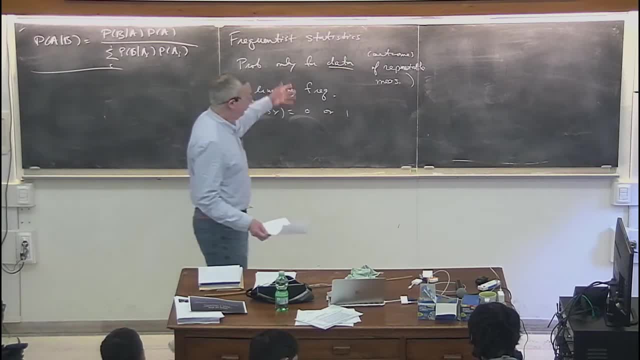 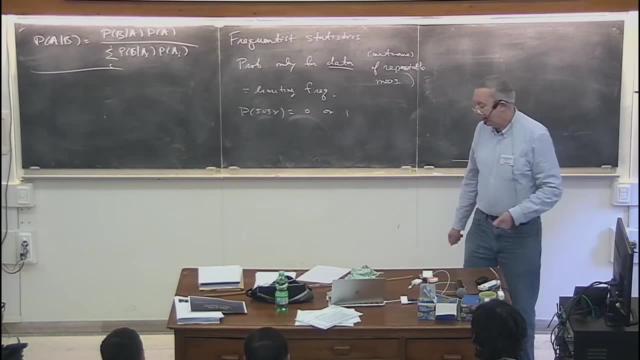 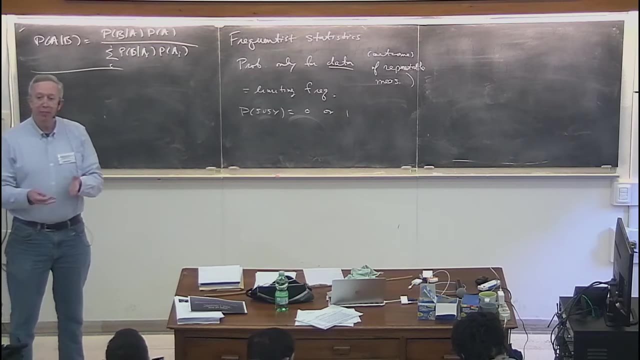 And so you might wonder: well, how, in frequentist statistics, are you going to address the question of whether a particular theory is preferred or not preferred? And it's going to boil down to saying that if a model is preferred, it means that that model predicts. 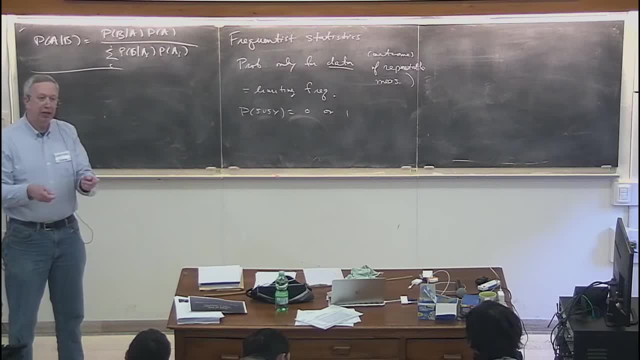 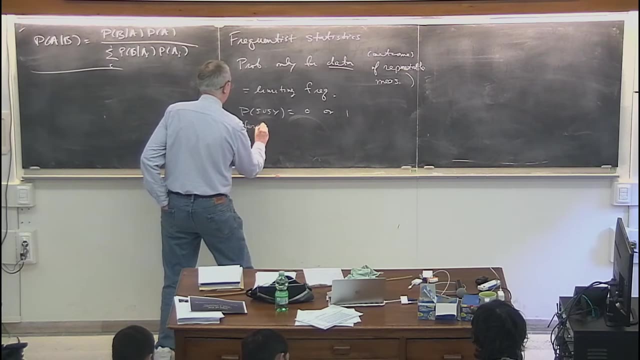 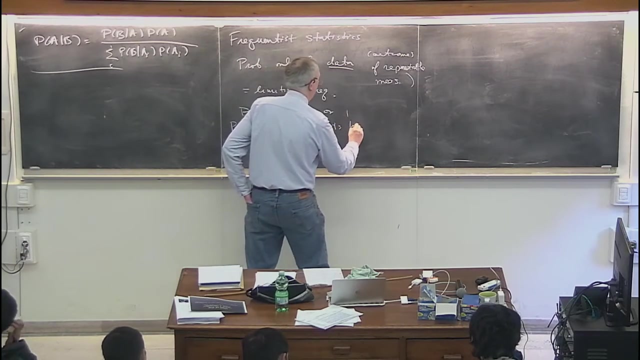 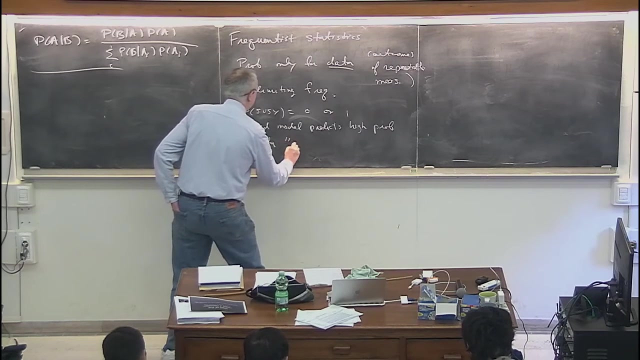 data that has a. it predicts a high probability for data that are similar to the data that you got. That seems like a very convoluted sentence. I better write that down. A preferred model predicts a high probability of for data like, in quotes, the data that you got. 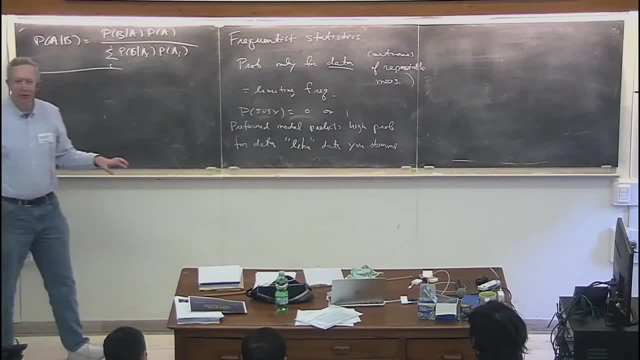 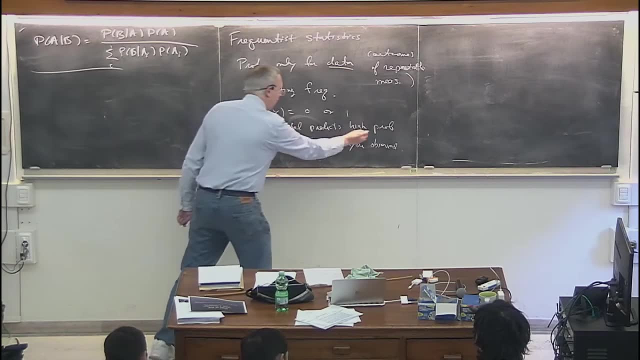 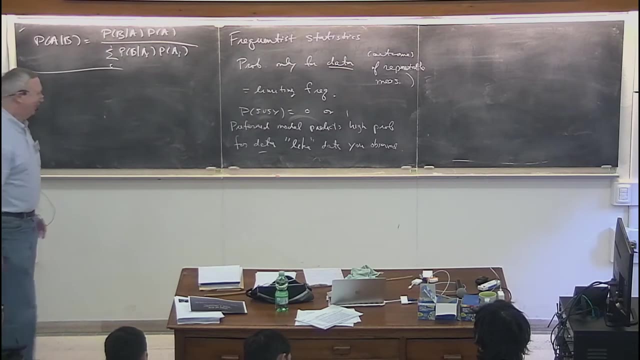 But notice, in making that somewhat convoluted sounding statement, I still only associate probability with the data Right. The preferred model predicts a high probability for data which is similar to the data that we found in our experiments. Immediately you might think: oh, that's. 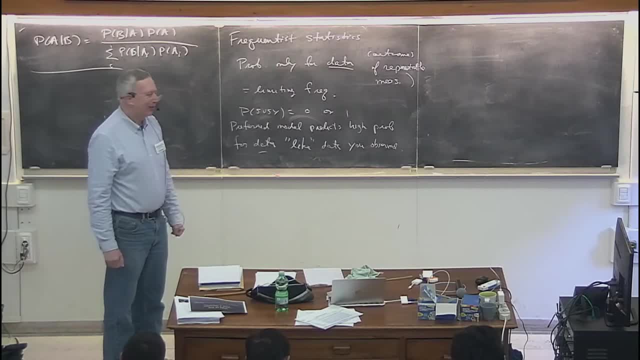 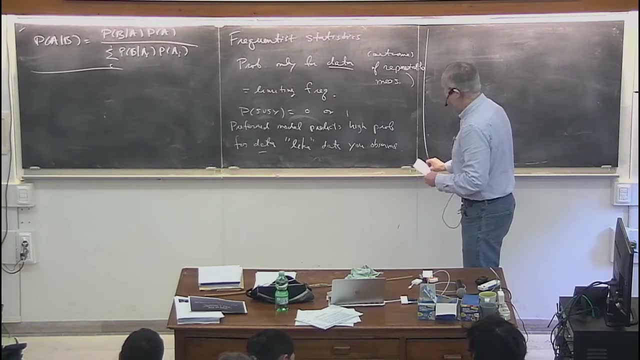 such a contorted way of having to phrase it. Surely we can do better. That is what most people who prefer Bayesian statistics would immediately say: Alright, this is no good. We would like to use Bayesian statistics, And in Bayesian statistics we extend probability. 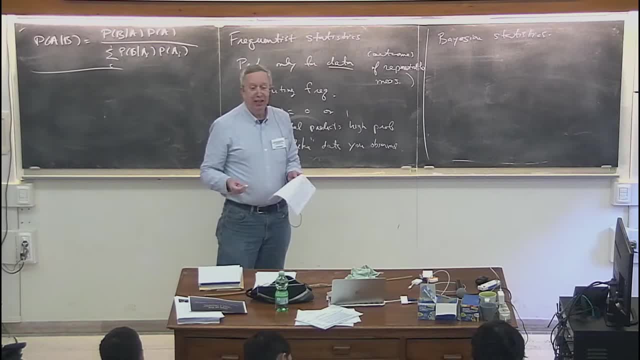 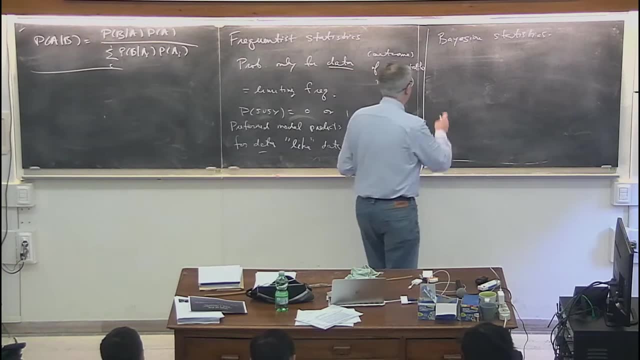 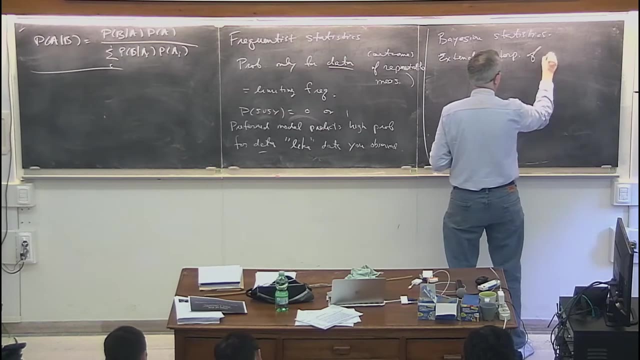 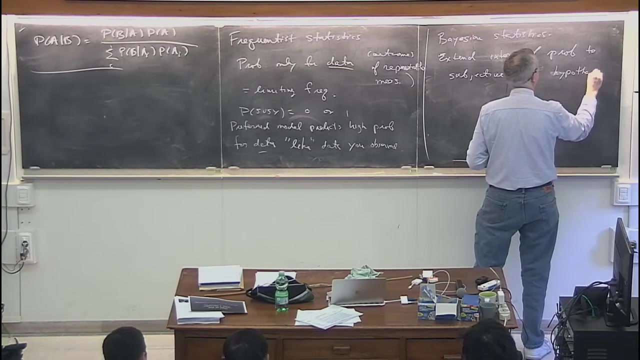 the interpretation of probability to include this subjective interpretation that I introduced And you can use that for your theories. So we extend the interpretation probability to include subjective probability for models, for hypotheses, And so let's see, here I'm going to use a kind of a notation. 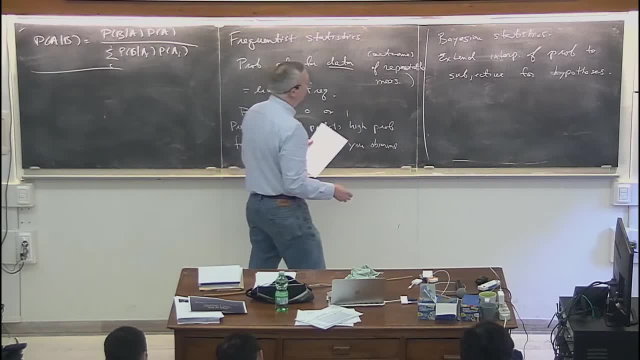 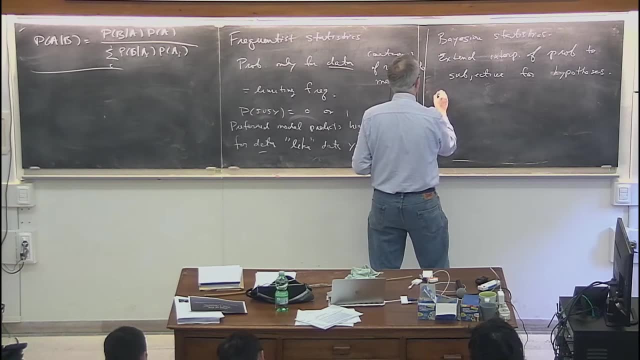 that for the data I will usually use some Latin letter like the letter X. So let me suppose that what you would want to get in Bayesian statistics. at the end of the day, you would like to know what is the probability that my hypothesis H is true. So this is: 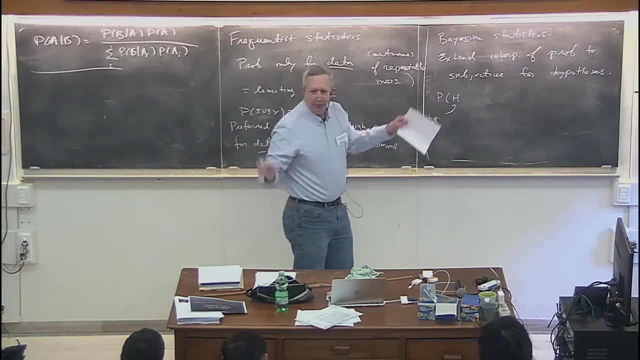 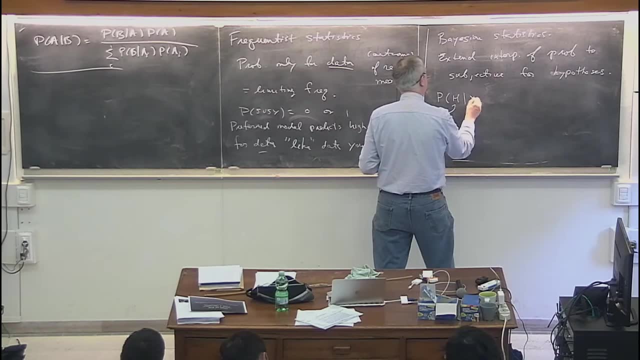 some hypothesis like supersymmetry or or technisprions or whatever, But I want the conditional probability, given that I observed a certain vector of data, a certain set of data from my experiment, Maybe I write an X with a vector Just to symbolize the collection. 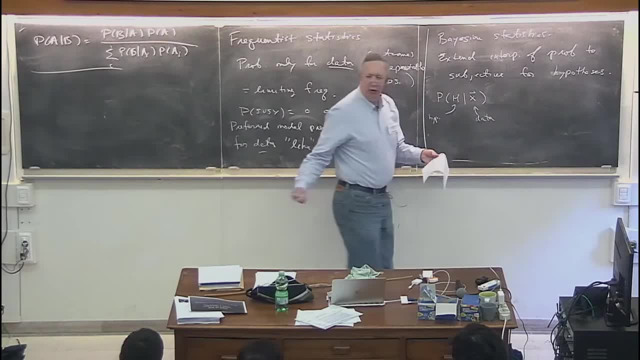 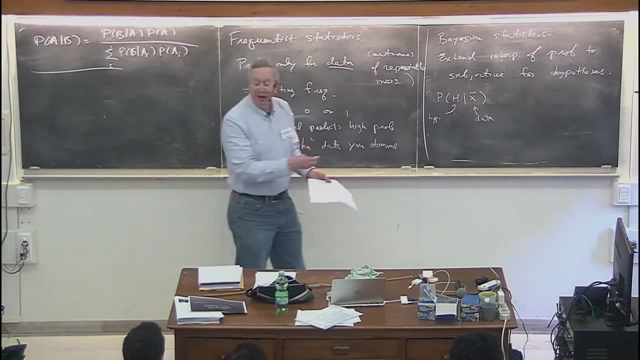 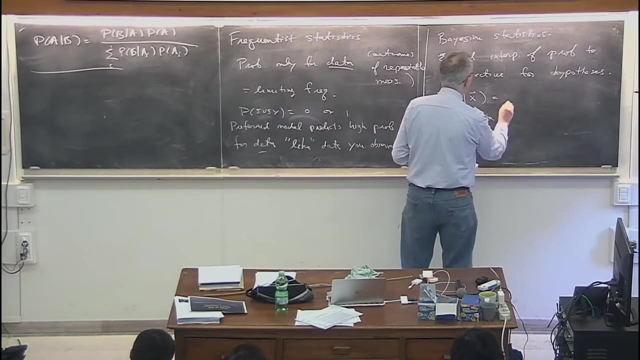 of numbers. that characterizes my experiment, So you usually use an X or something for that. That's what you want. That would be the final answer of your Bayesian statistical analysis: High probability, low probability, whatever. How do you get that? 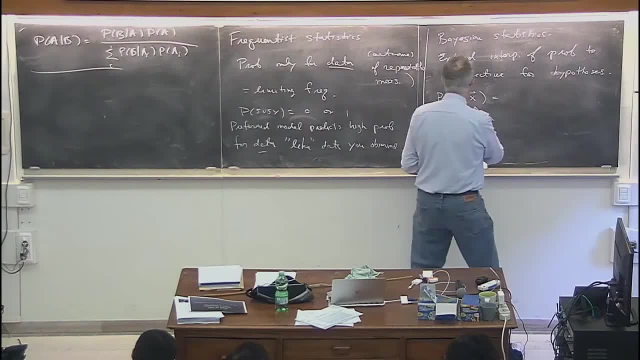 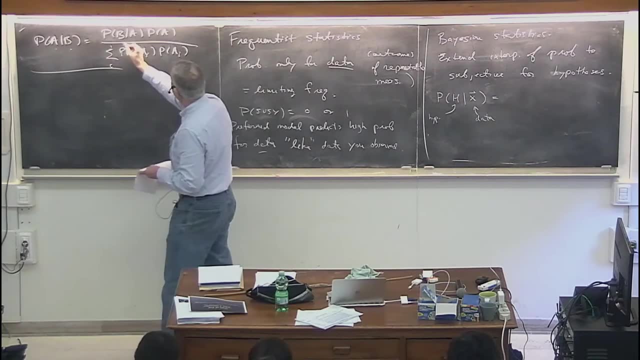 Of course, you use Bayes' theorem. We turn this around. What Bayes' theorem does, of course, is to relate the conditional probability of A given B to the conditional probability of B given A. It switches the two guys around, And so this tells me that 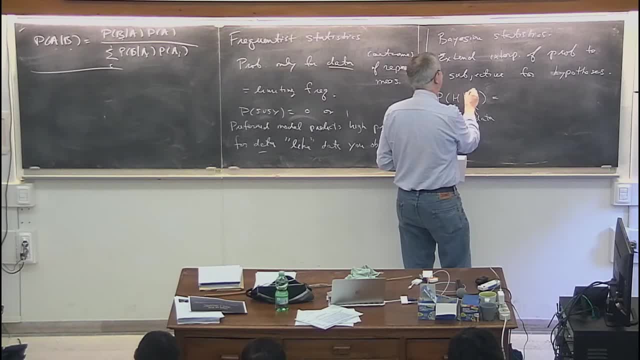 the conditional probability of my hypothesis, given that I got a certain set of data, is equal to the probability to get those data, given that the hypothesis is true. But now I need to multiply by the probability of the hypothesis, And I'm going to use here traditional. 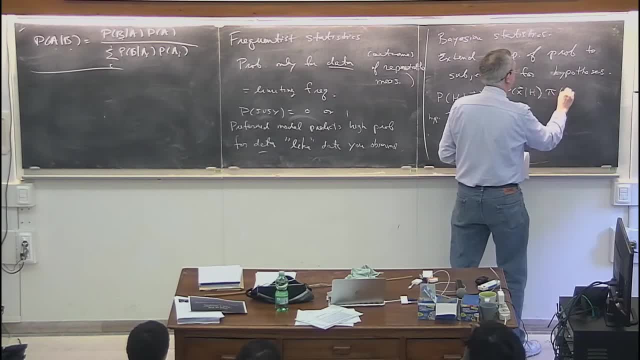 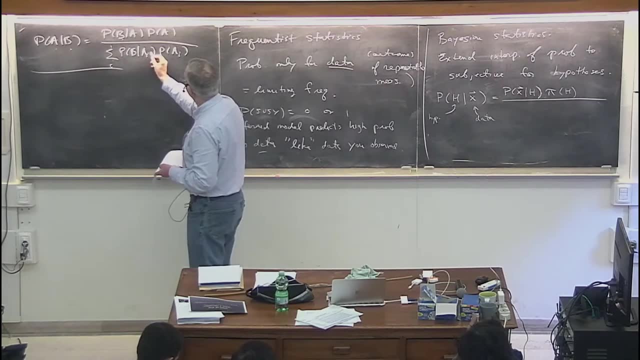 I'll just use a different letter. I'm going to use a pi for that, And then in the denominator I want to assume that I can break this hypothesis space into some subsets, And so I'll write it in the following way: Sum over. 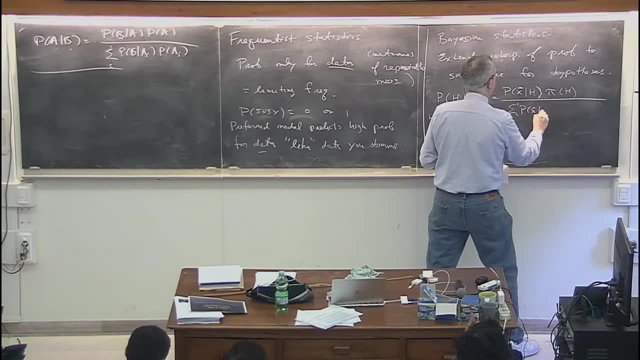 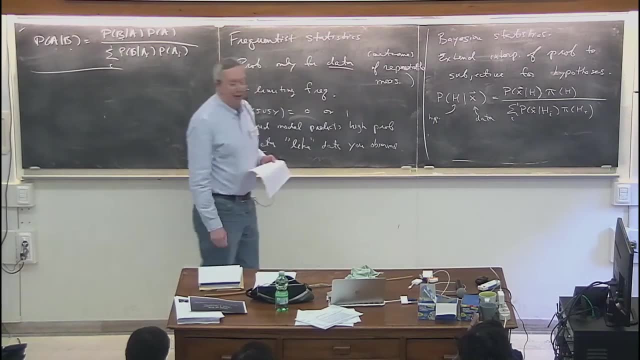 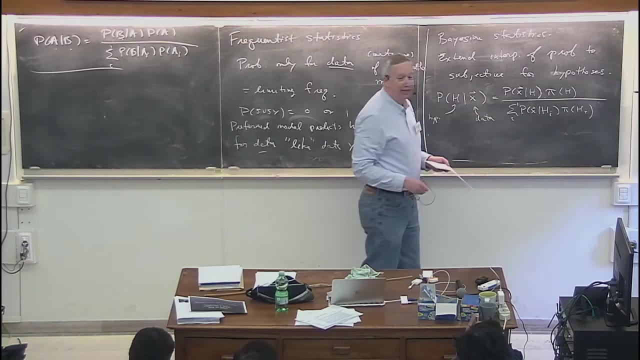 i p of x given h sub i pi of h i. Alright, so that's Bayes' theorem and that forms the basis of Bayesian statistics. Now I want to discuss some of the ingredients in this expression. First of all, what is this? 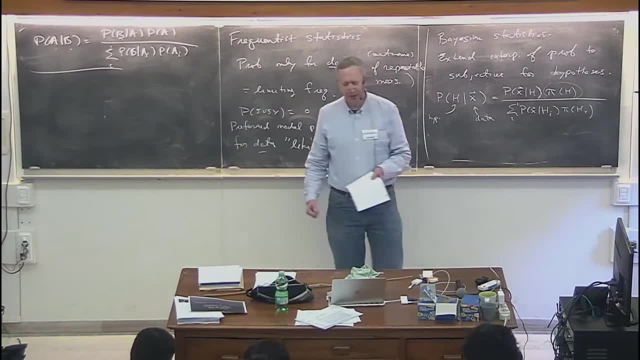 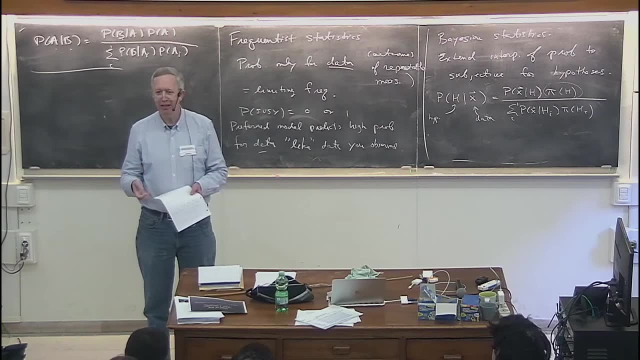 guy represent Pi of h. That's just the probability of the hypothesis, but without the condition imposed that you saw certain data in your measurement. So it's the probability of the hypothesis before you did the experiment. So we call that the prior probability. 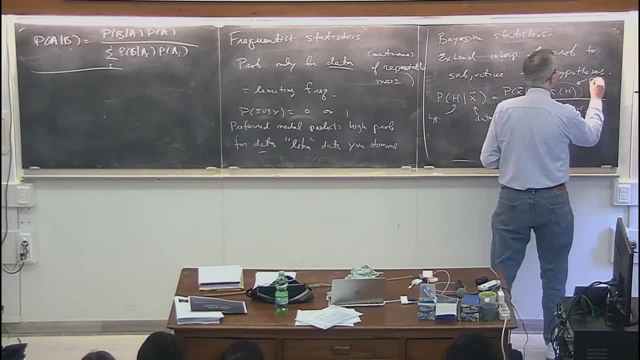 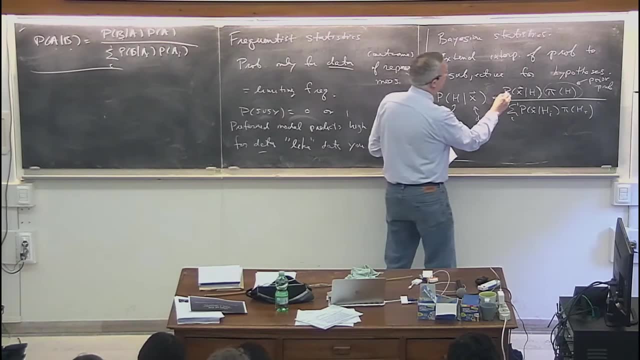 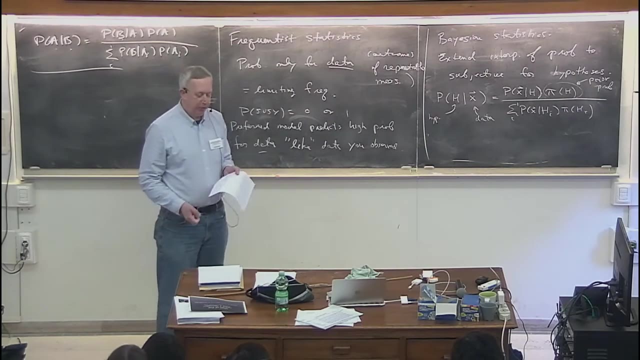 So this is the prior probability, The probability for the data given the hypothesis. that's what you compute, That's somehow the result of your. you say I want to consider a certain model and the result of your quantum mechanical calculation is the prediction for the probabilities for 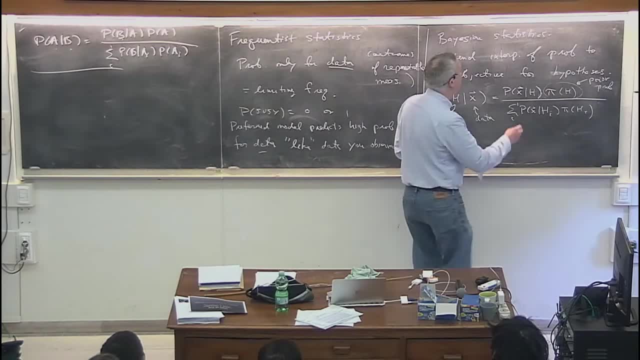 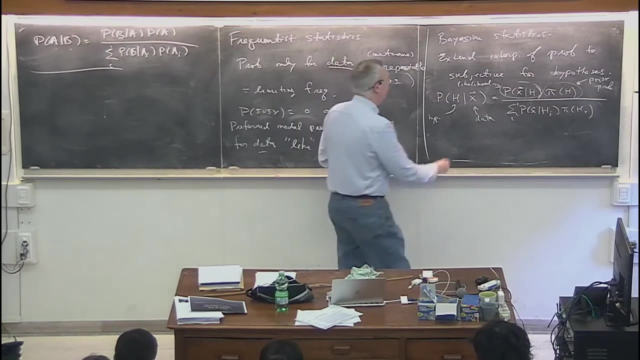 observable outcomes, And in this context, this term here is what we call the likelihood. So sorry, I sneaked that word in here. Likelihood- Alright, This guy here you can guess- is the probability of the hypothesis after having seen the data. And so that's the posterior. 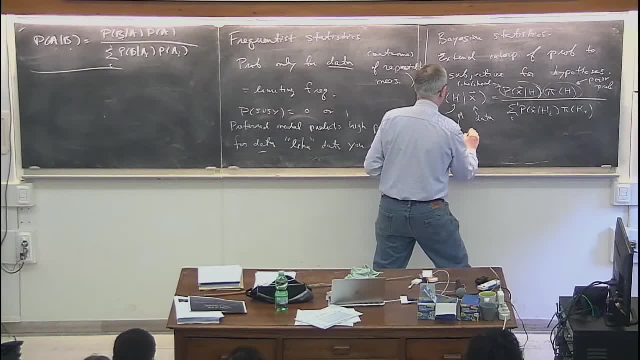 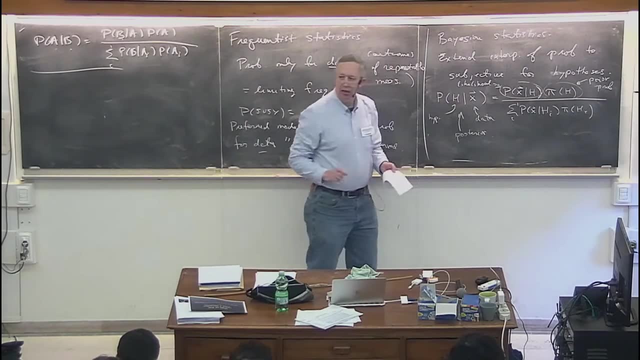 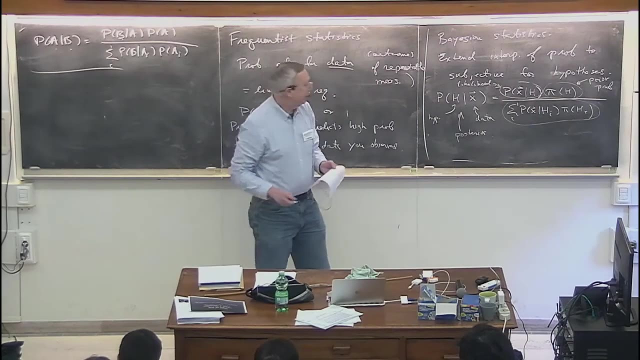 probability. And so those are the three important ingredients: Posterior likelihood, prior. This fourth guy in the bottom, if you think about it, just plays the role of a normalization constant. It means, for example, that if I were to take the left hand side and 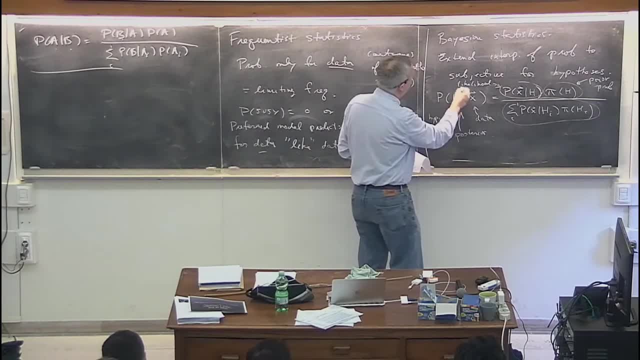 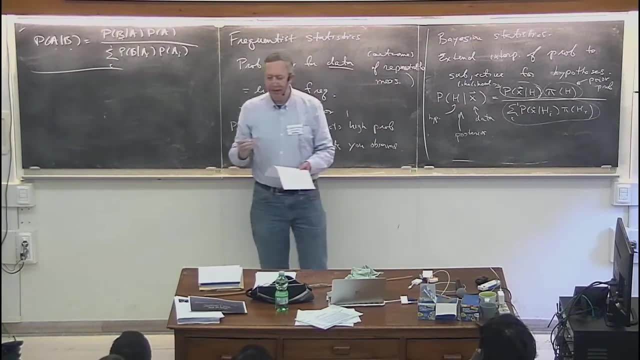 say that this is for one of the h i's and then I were to sum it over all possible hypotheses, then you would get the same thing in the numerator as in the denominator, And that simply tells you that if you sum your probability over all possible hypotheses, 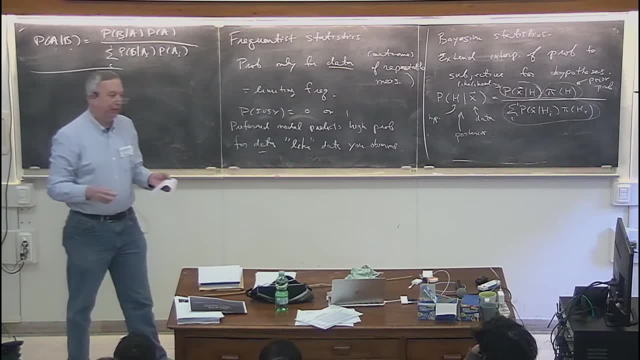 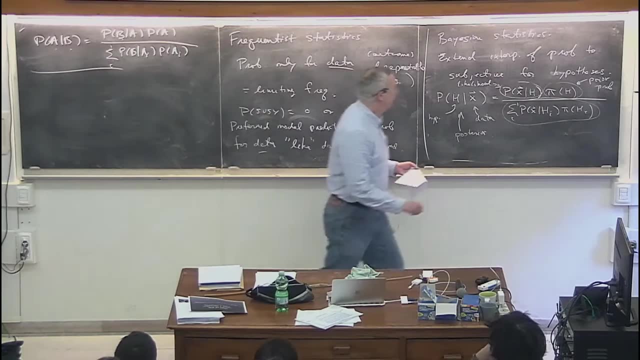 you get one To the extent that your hypothesis space includes one of them. that's true. Usually set it up so that by construction that has to be the case. So this thing here, I will say, plays the role of a normalization constant. 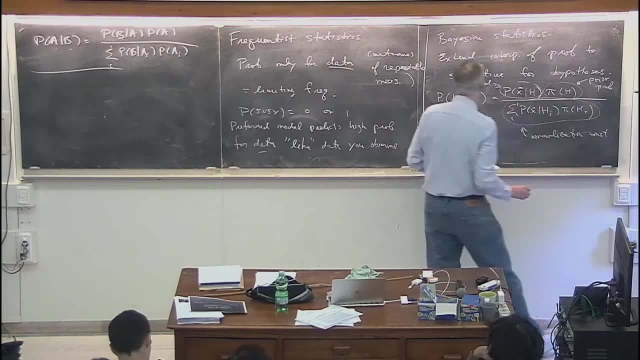 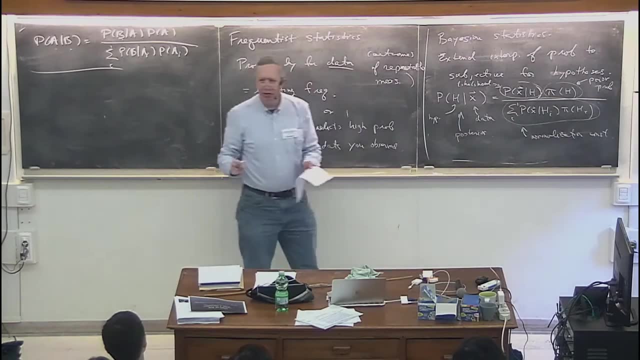 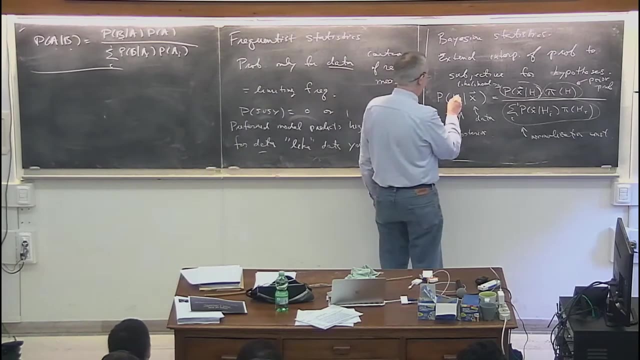 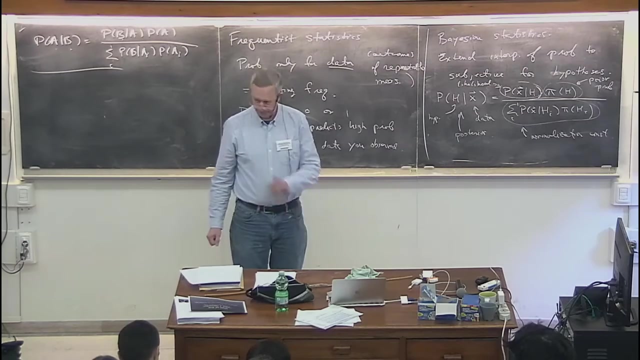 And there are many applications of Bayesian statistics where we just write this expression down as a proportionality. Sometimes we need the proportionality constant, sometimes we don't. I say that proportional to that. So let me give an example. Very often we would label the height of 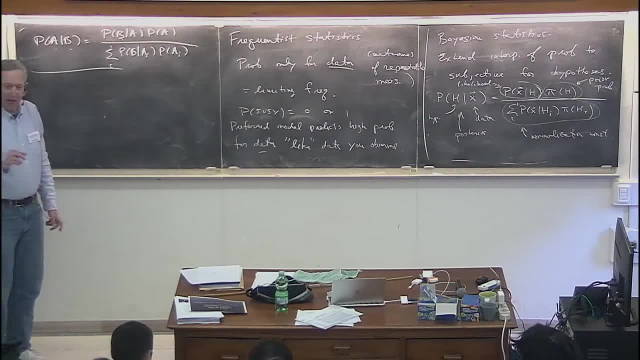 the hypothesis by means of some continuous parameter, And so we would say something like the probability for that parameter to take on a certain value, given the data, would be proportional to the probability for the data given. the parameter times the prior for the parameter. Alright, And so then? 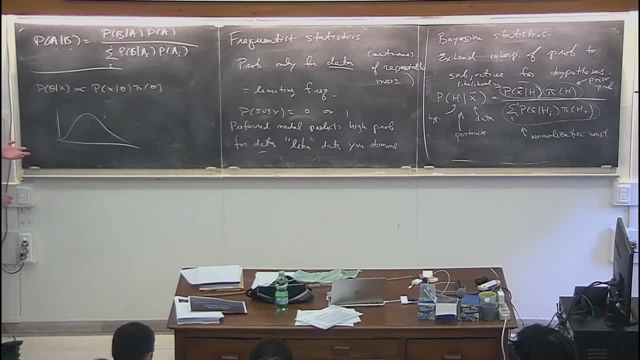 if I don't, I would get some curve like that, And if I wanted to know what is the mode of this distribution, I could just say, alright, well, it's here. That's somehow my preferred value of theta And that's. 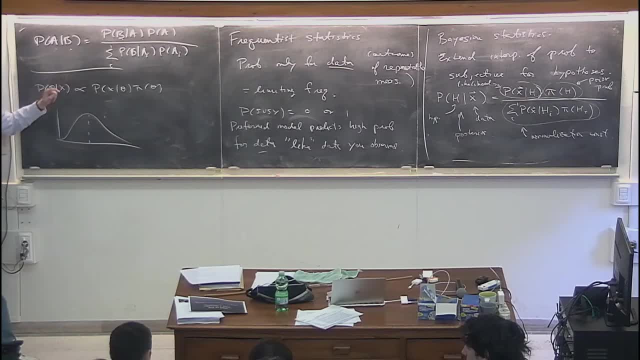 independent of scaling this up or down. On the other hand, hold that question if you wanted to know, for example, what is the value of the parameter theta, such that I have, say, a 95% probability that the true value is less. 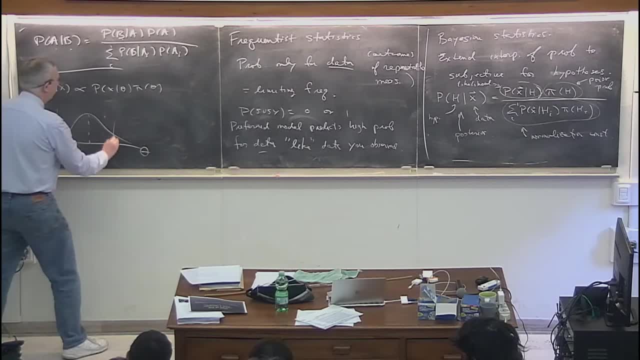 than that limit, then what you would do, of course, is you would say: alright, let me integrate this distribution to the point where I have, say, 95% of the area to the left, and that would then be some sort of 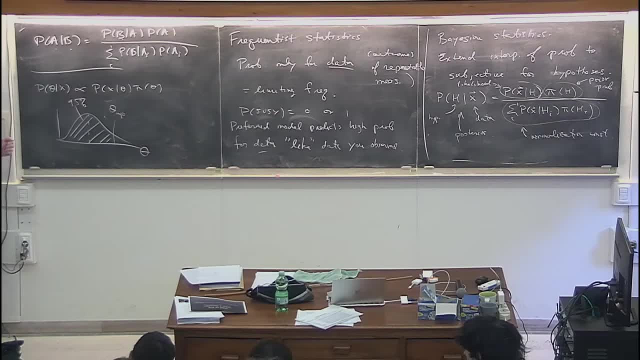 upper limit. So again there what you're really doing there. essentially, you are computing the proportionality constant in the sense that you're saying: give me 95% of the area. So for some types of calculations you need. 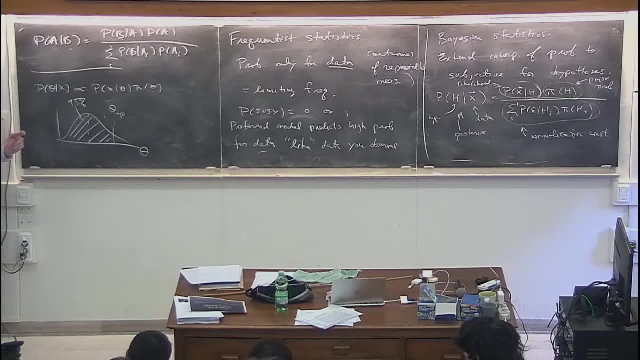 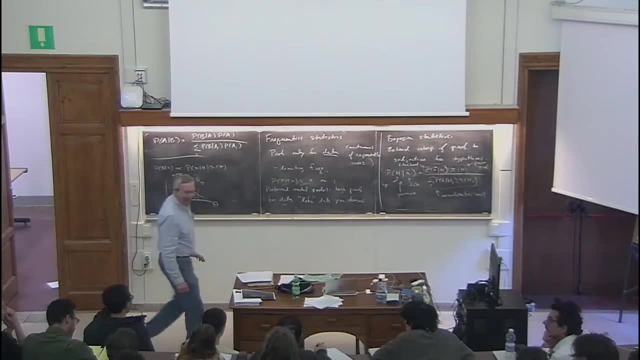 to normalize the thing In other types you don't. So sorry, there was another question here. That's the big question. yes, I'm getting to that. Yes, yes, exactly Because I had to make this very vague here. 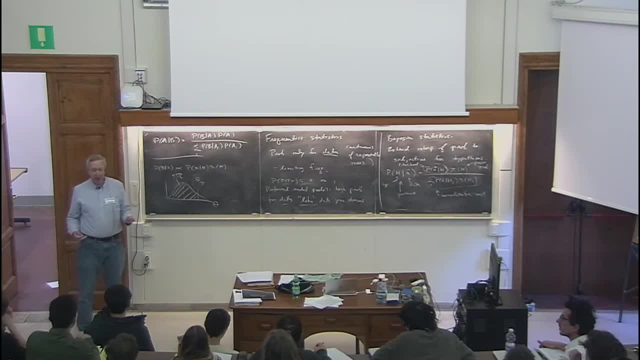 What does it mean to have a high probability for data which is like the data you got? I'm going to, when we discuss the method of maximum likelihood, which is hopefully coming up in an hour. I'm going to give an example for that And also tomorrow. 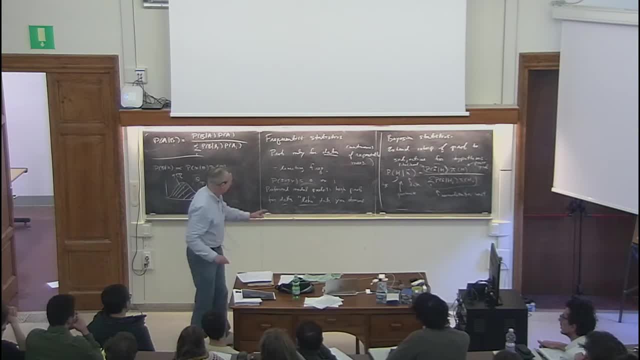 when we talk about statistical tests, I will say precisely what I mean by data, like the data that we observe. So that's a longer discussion, But the discussion about the prior probabilities is what I wanted to address just next. Yes, yes, so in other. 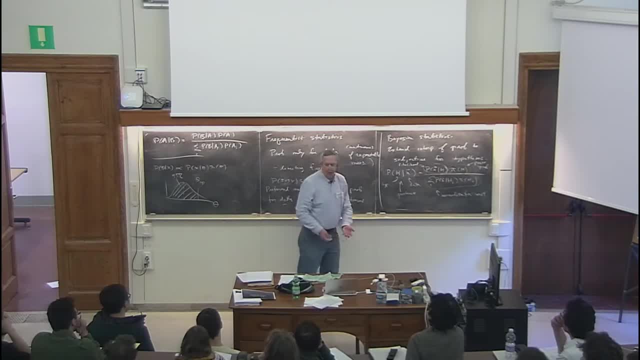 words that you would set up some sort of set of theories and you would say: give that one of them in this set is true. you could then come up with a set of posterior probabilities If you then want to enlarge that set to include. 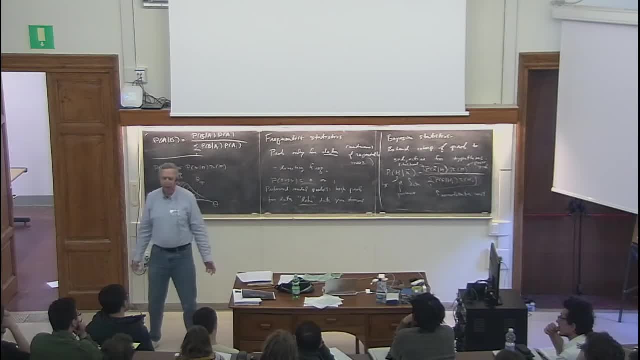 even further hypotheses, all of those probabilities would change. So what is statistics? Statistics is the branch of applied mathematics that allows you to decide between theories. If the theory that you want to decide between is not on the table, statistics can't help you. 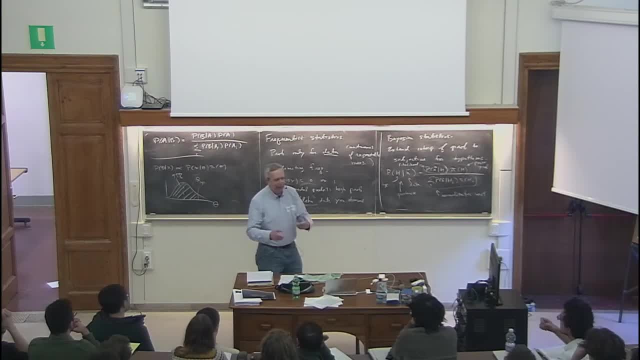 So that's a good point, Because you might think that somehow the statistical tool is going to lead you to say that, ah, there must be a theory which is not amongst the one I'm considering, but no, It doesn't work that way. 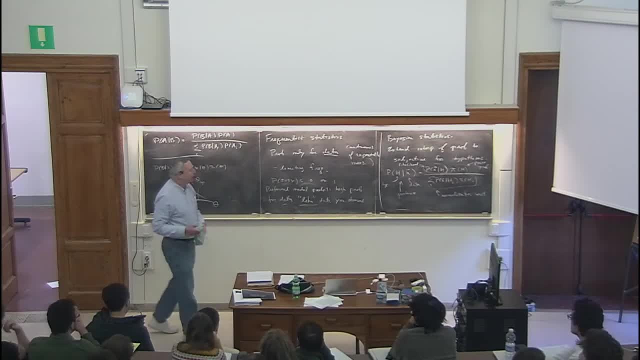 Okay, but no, this is a very good point about. I've been very vague. how are you going to get the probability that your hypothesis is true before you do the measurement? And that's one of the big sticking points behind Bayesian statistics. 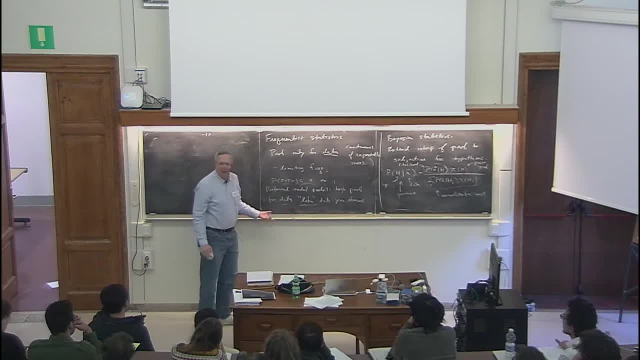 I started off by saying, oh, this phrase sounds so convoluted. certainly now everybody becomes a fan of Bayesian statistics. And then you look and say, uh, oh, I need this guy. So then maybe you bounce back. Let me just leave that on the board. 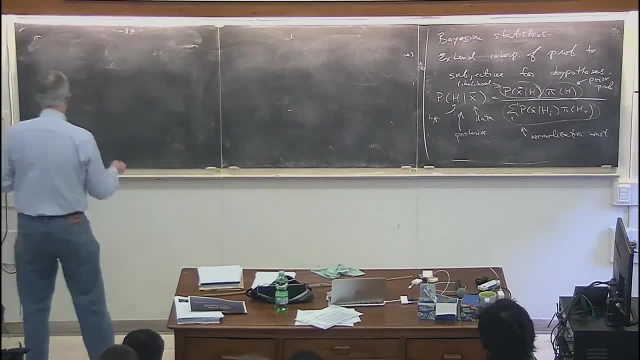 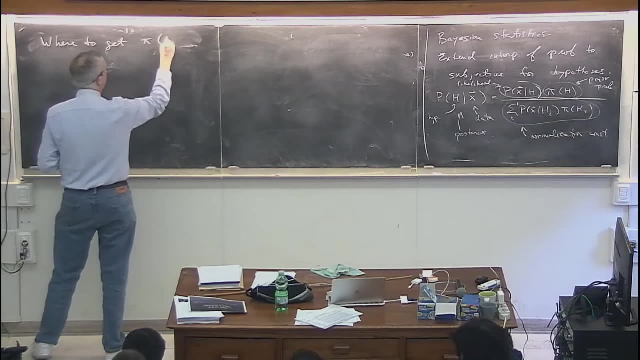 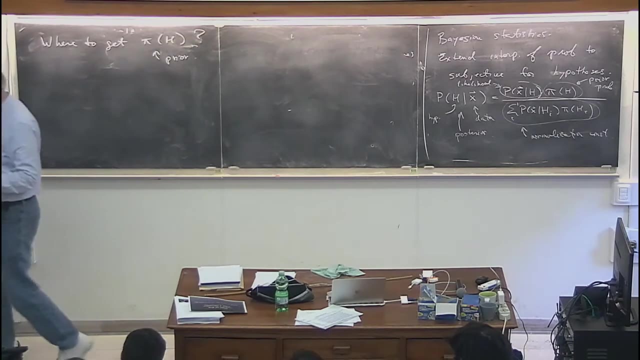 And write down this very important question as to where do we get the prior Alright? this is the song. I'll usually just call it the prior alright, the prior probability, And the answer is that, at least within the framework of Bayesian statistics, there is no golden 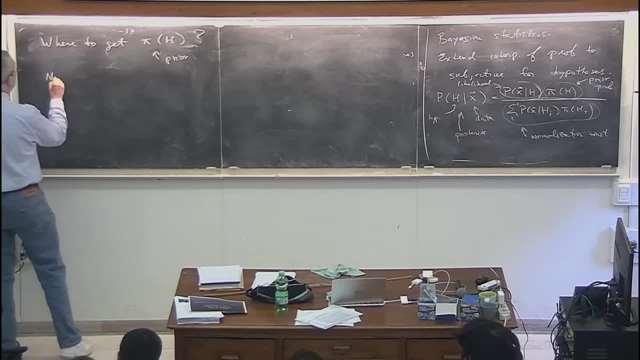 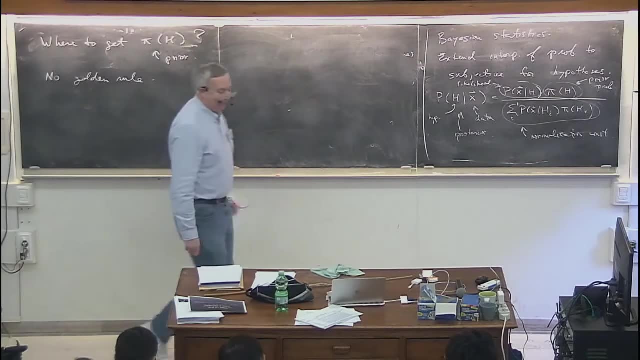 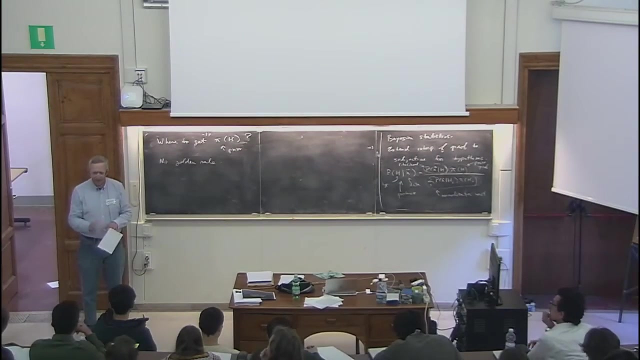 rule. There's no unique rule. I've sometimes. yes, you need either another mathematical formalism that will lead you to a choice of the prior, or you need subjective input, And so there are different branches of Bayesian statistics. One of them is called. 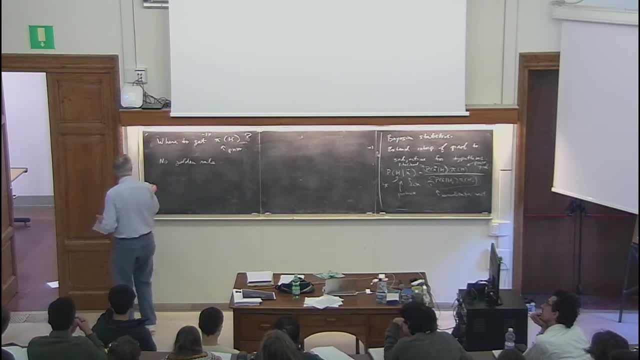 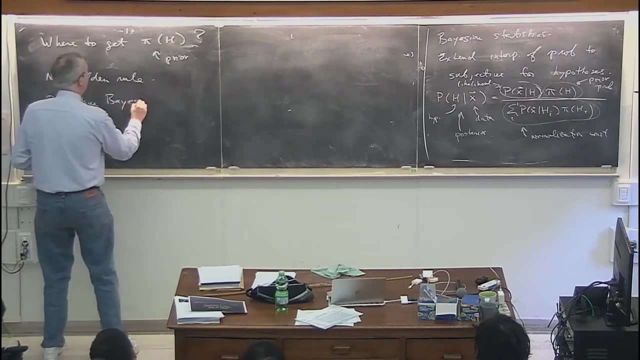 objective Bayesian statistics. It's just the name that they use for the collection of techniques that they've come up with, And I wasn't actually going to go into this in much detail, but the idea is to come up with some sort of formal rules which will lead 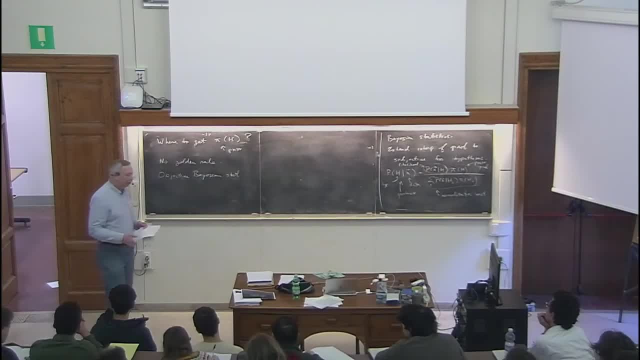 to a particular prior, And so those formal rules might be sorts of invariance principles. So let me give an example. We'll come back to this later. I said that very often what we're doing is we're labeling hypotheses by a continuous parameter. 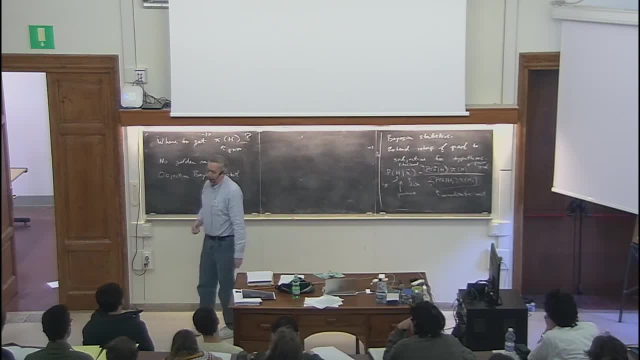 Alright, so I label the hypothesis by a parameter, beta, which is a ratio of vacuum expectation values of some particles in my theory. And then I say: well, before I've done the experiment, I know nothing about this ratio, So I've got this ratio. 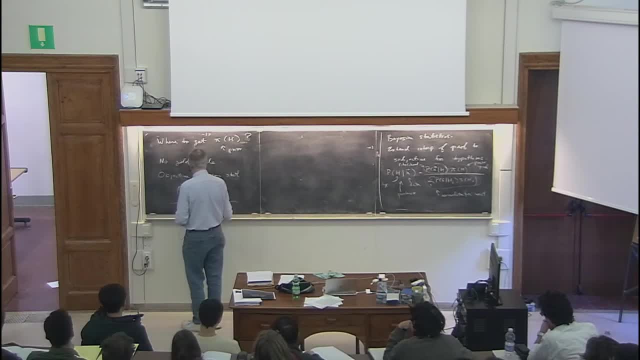 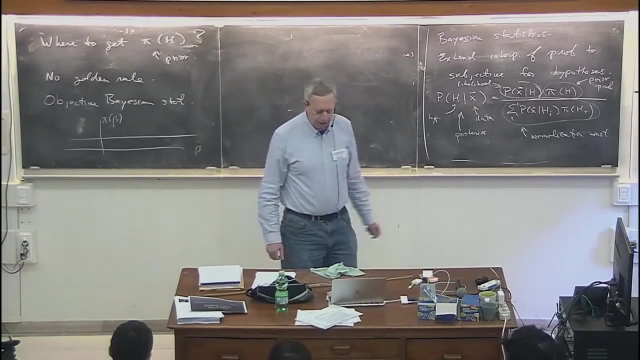 beta and I know nothing about it. so therefore, maybe I assign a very broad distribution to it. Sorry, this axis is beta, right, And I would say something like pi of beta is very broad, or maybe it's just a constant. 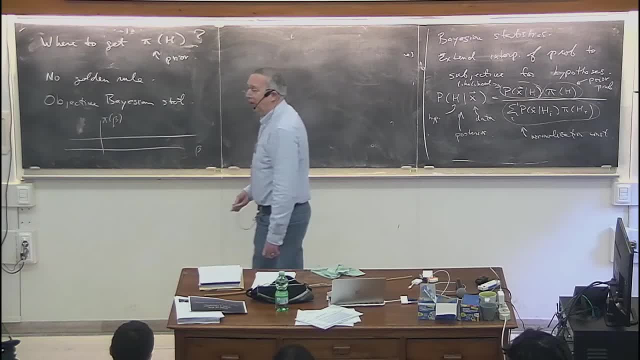 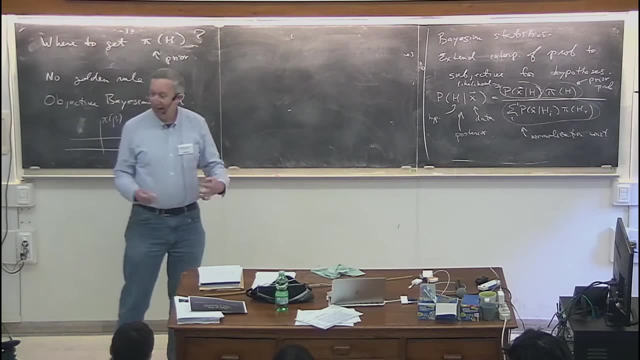 On the other hand, if somebody then comes back and says: well, no, I've formulated my version of the theory in terms of tan beta instead of beta, and I don't know anything about tan beta, so I would say that no, I want to. 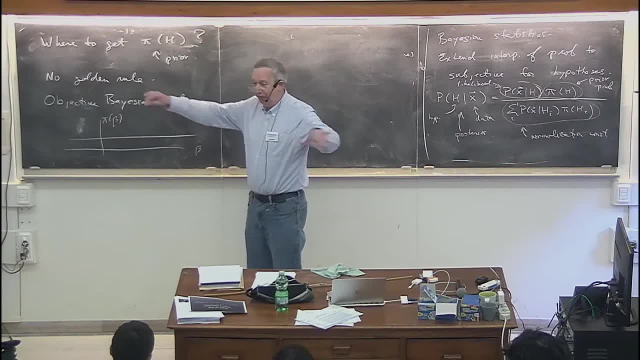 write down a prior which is constant in tan beta. Well, if it's constant in beta, it's not constant in tan beta, and vice versa. And so you run immediately into this idea that if you want to write down a prior that reflects 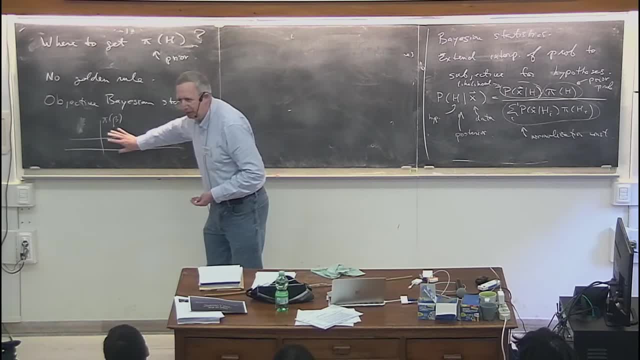 complete ignorance or complete ambivalence towards all possible hypotheses. that is not uniquely defined, So you can write down certain types of priors, however, which are invariant under parameter transformations, And that's one of the principles that can be imposed to determine a 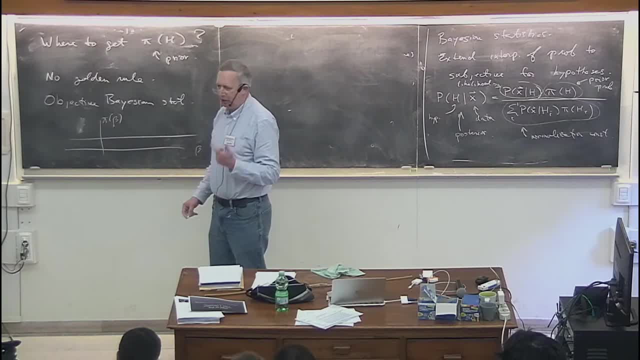 prior. If you do that, though, what you're really doing is you're choosing the prior to satisfy that particular invariance principle, and the prior is no longer actually reflecting your subjective degree of belief as to where the parameter lies, So 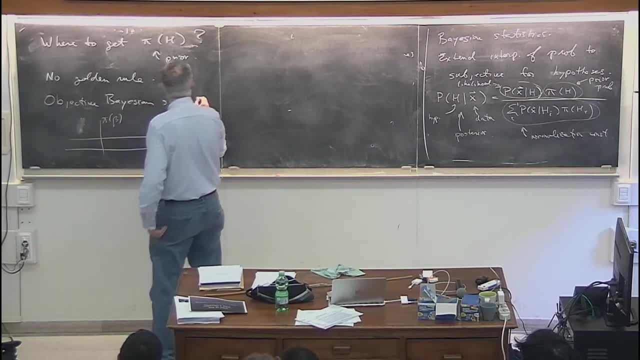 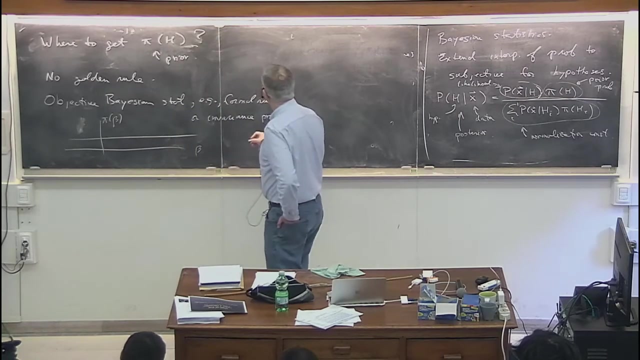 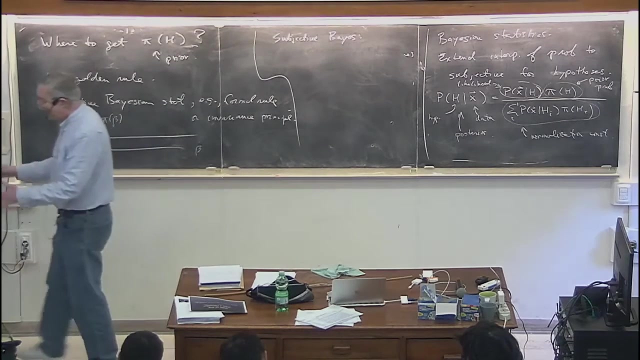 the objective Bayesian statistics would say: use an invariance principle or a formal rule, invariance principle, and then the other competitor in that game would be subjective Bayesian statistics. And so there, the prior is supposed to represent an individual's subjective degree of belief. 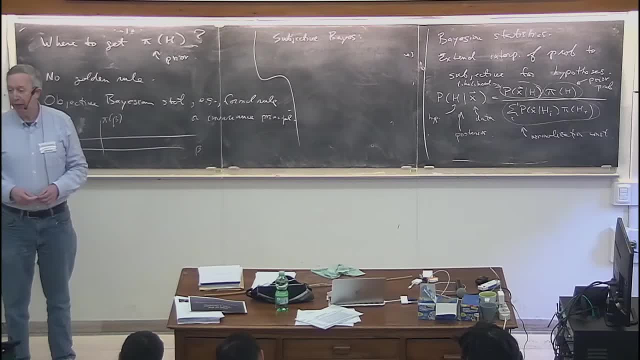 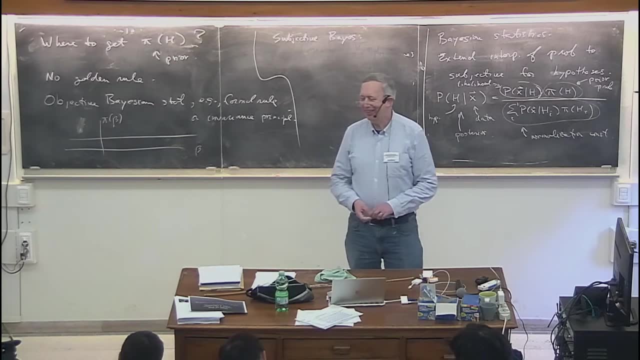 as to whether or not this theory is correct, And there is a formal procedure in the context of subjective Bayesian statistics, which is called elicitation of expert opinion. And the way that you do that is the following: You take a chair and you sit the 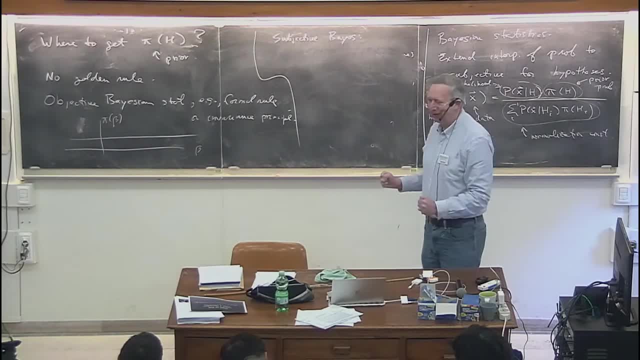 expert down in the chair. Maybe you tie the expert to the chair And then you interrogate this person to try to say, well, is this theory right or is that theory right? Or you know which value of beta is preferred. 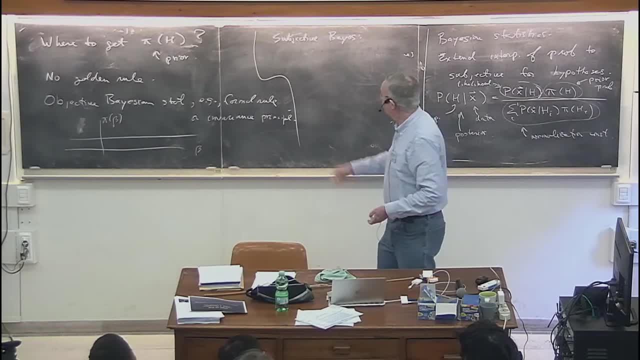 As a result of that elicitation of expert opinion, you write down some curve. I've had this type of conversation many times with, for example, theorists who are computing perturbation series, And let's suppose that they've only computed up to third order. 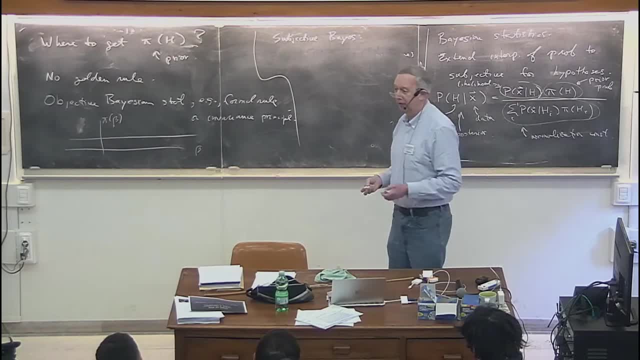 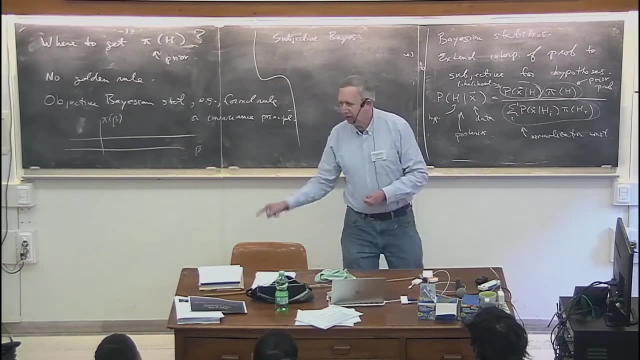 and the fourth order coefficient is not known. Let's suppose that that fourth order coefficient is called beta. And so I ask the person: how big do you think that fourth order coefficient is? And they would say: until I've computed it, I know nothing. That's baloney. 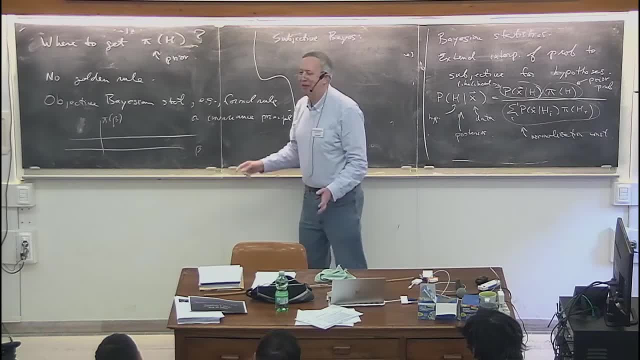 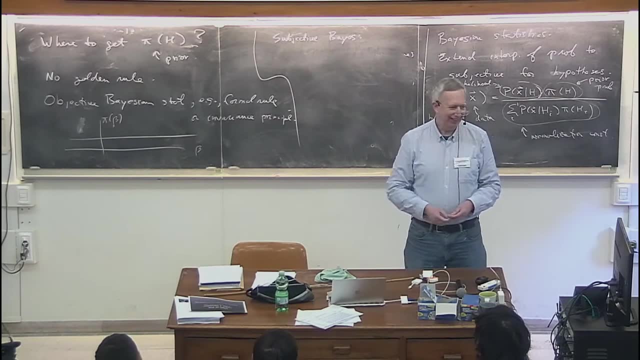 They obviously know something Because they've computed the first three orders, And so they have some idea of what they will be doing when they compute the fourth order. You know it will contain square root of pi and zeta of three. It's not going to come out to be ten to the fortieth. alright. 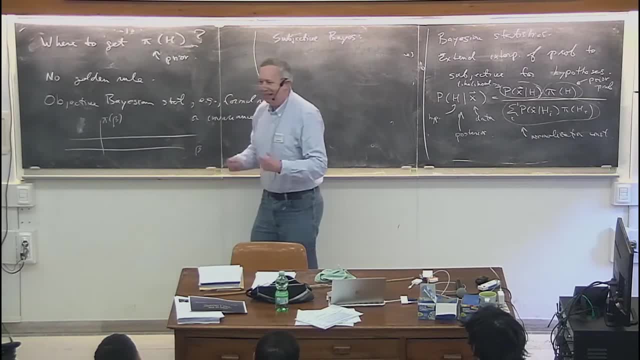 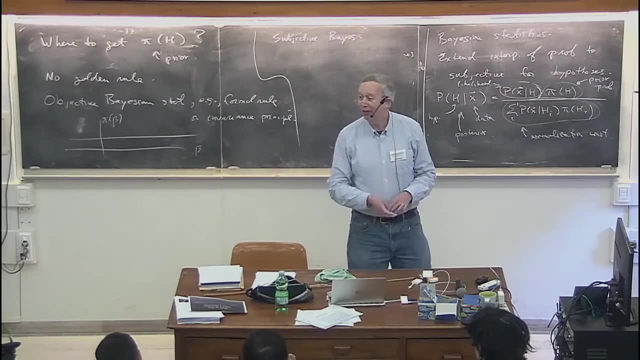 So the point is that, even in that type of a context, a theorist could write down a subjective degree of belief as to where a particular constant is going to lie, And then, a hundred years later, when it's actually been computed, you could check. 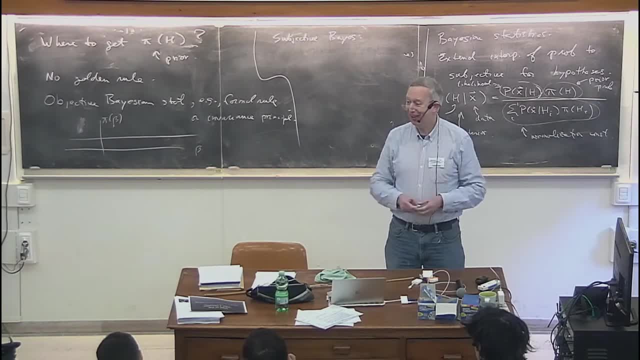 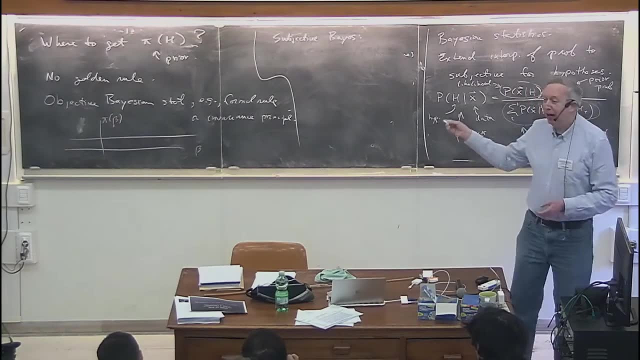 You could go back and see what fraction of theorists got it right. You could try to calibrate their degrees of belief. So this whole question of how to establish the prior for a Bayesian calculation is a long and complicated one, and that's what's led to this sort of two hundred years of. 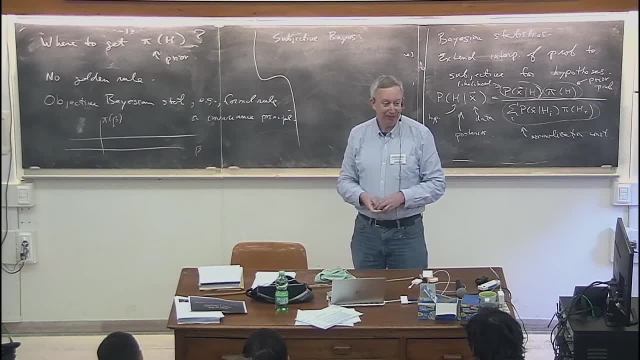 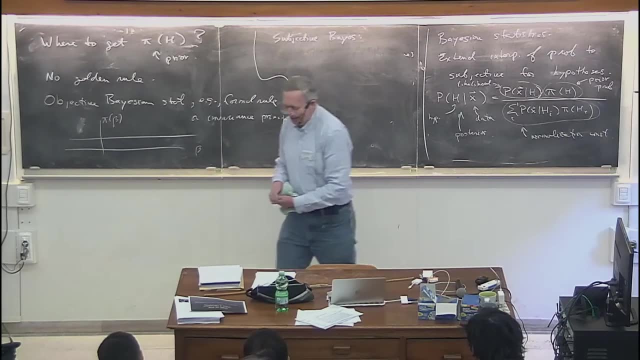 debate between the two schools. We should go on. I could finish the rest of the three days only talking about this, but we should go on to some more practical matters. I do want to make- sorry- the final statement concerning where to get the. 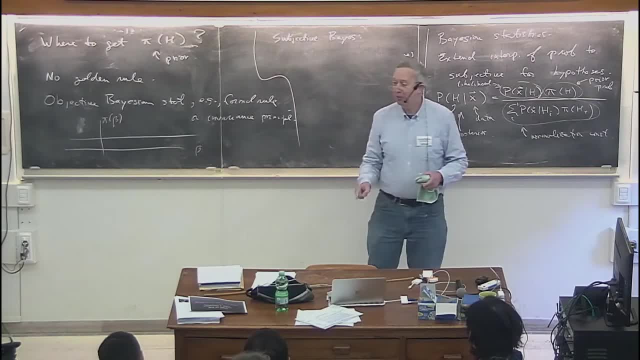 prior, When you do the solicitation of expert opinion, to reassure the person that you're not going to hold them responsible for whatever probabilities they say, you should point out the if-then nature of Bayes' theorem. Okay, So how should I say this Bayes' theorem? 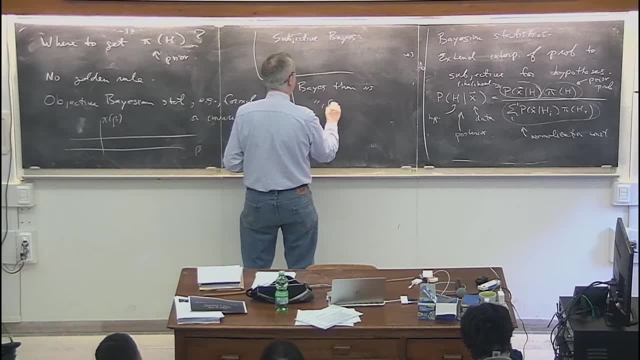 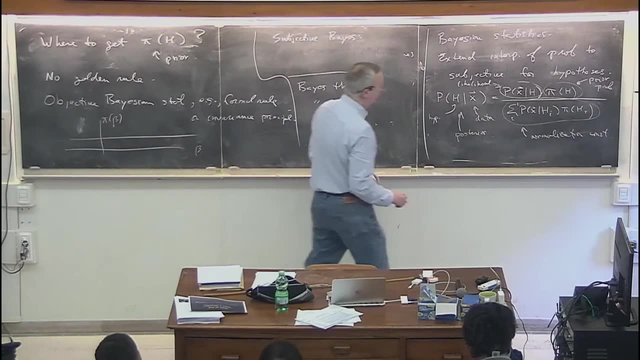 Bayes' theorem is an if-then statement. What it's saying is that if your prior probabilities are given by a certain prior pi of h, then in the light of the data, those degrees of belief should be updated according to Bayes' theorem. to give you that: 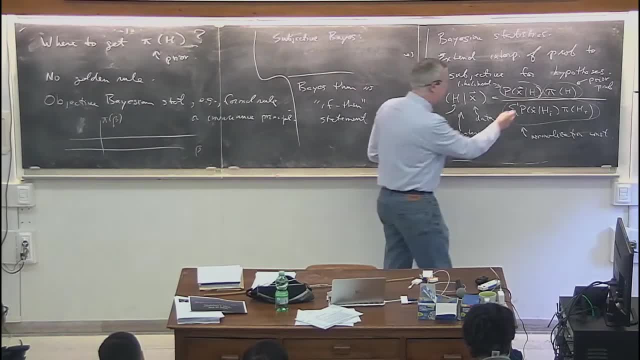 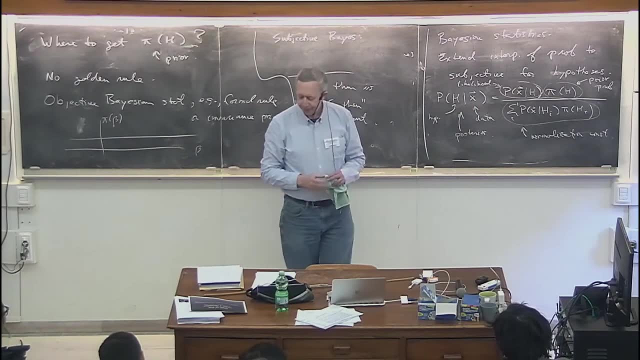 So it's really an if-then statement. It's not giving you a golden rule to determine what the priors are. It's only telling you uniquely how to update them in the light of the data. Okay, Let's go on. 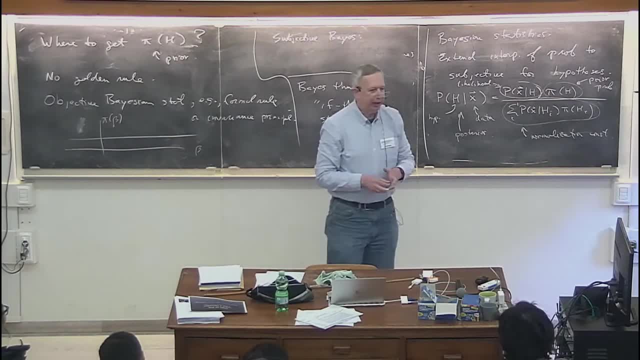 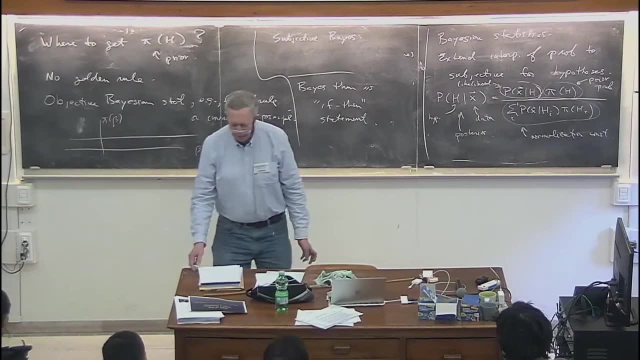 By the way, I should. I'm supposed to take a break at some point. Is that right, As I like? No, it's as you like, But if I take a break, can we make it just five minutes or so? And if it's five minutes, is that meaningful? 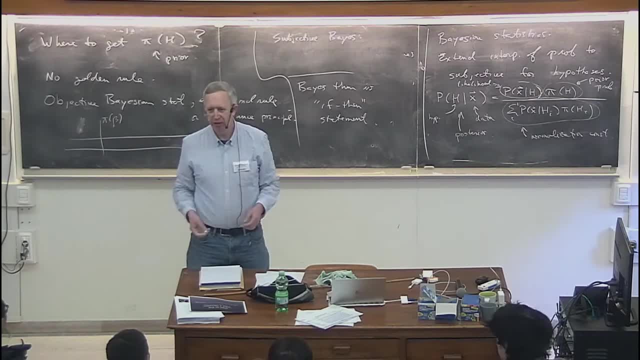 Does it have to be ten to be meaningful? What do you think? I would just assume, move on. If you guys can hold out for an hour and a half, we just plow through. Is that okay? Okay, Yes, Yes. So, for example, 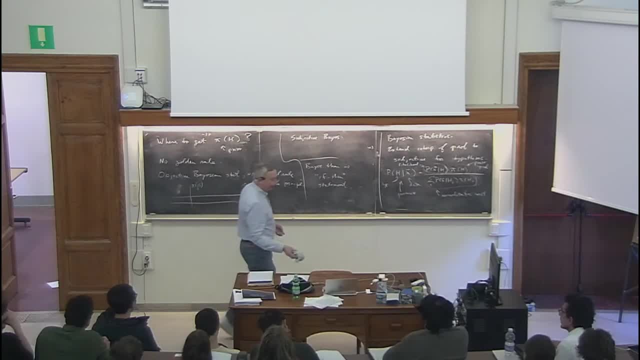 one of the common applications of Bayesian statistics in the context of LHC analyses is to set upper limits for parameters, And so there you would do exactly the game. that I said is that you would get a posterior which would have some shape like that: 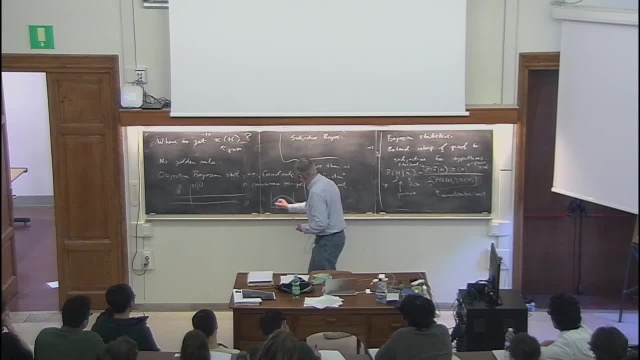 for the parameter. Let's call the parameter theta- And you would integrate it until you get 95% of the area and you would say that that's your upper limit. And very often what this parameter represents in that context is the cross-section of a process. 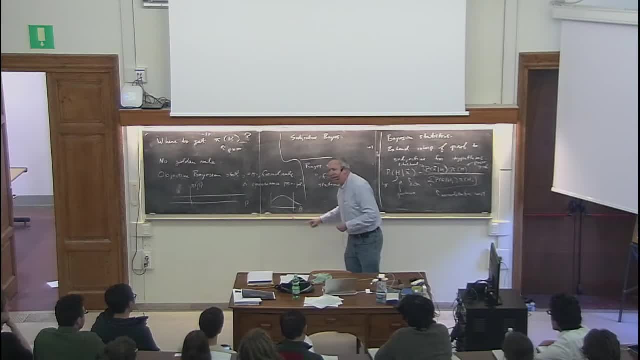 And that's going to be proportional to the mean of a Poisson distributed variable. So that's the one example where we would very often use this: flat prior is for the mean of a Poisson variable, But then the mean of the Poisson variable. 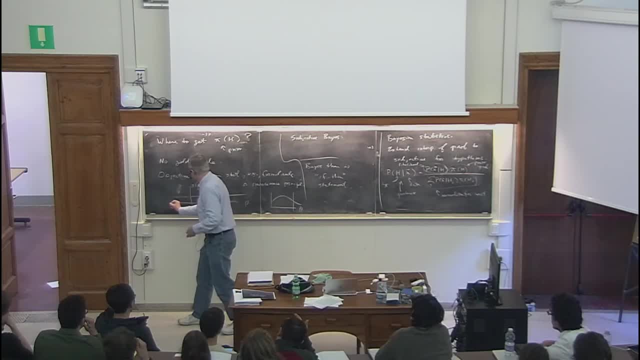 has to be positive, so you chop it off like that. So that's a common example And there are problems with that procedure which I hope I have time to go into tomorrow or the next day. So the convention, which is very often used in particle, 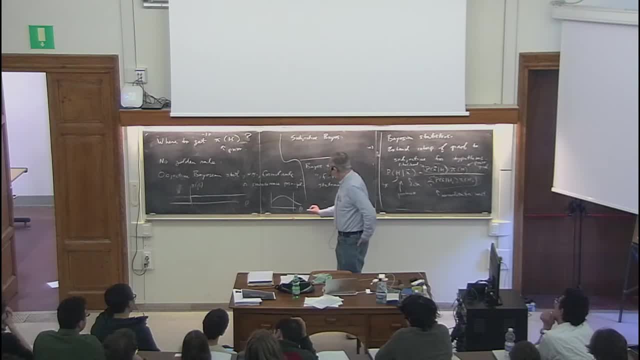 physics is. the variable that you would choose is the one that's proportional to the cross-section of the process you're looking for. So, for example, suppose you were looking for a manifestation of a new theory, and so you take that prior to be constant. 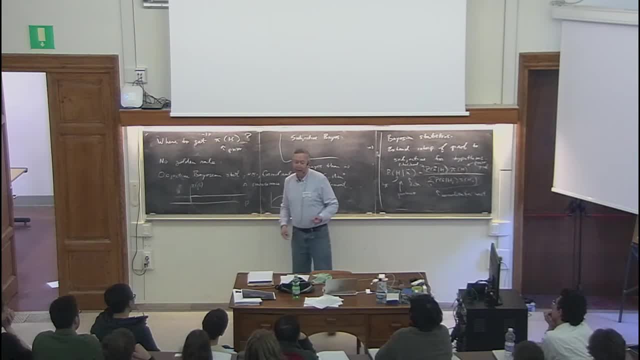 in the cross-section for that theory. On the other hand, that theory probably contains some particle of a certain mass and the relationship between the rate of the process, the cross-section of the process and the mass of the particle involved is going to be some complicated non-linear function. 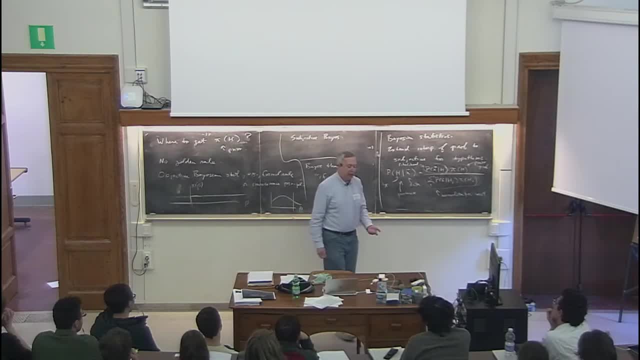 So you could have taken a step back and said: oh well, really, the thing I know nothing about is the mass of this mysterious particle, and I should take it to be flat, But that would lead to a different answer. So this business about taking the mean of a Poisson, 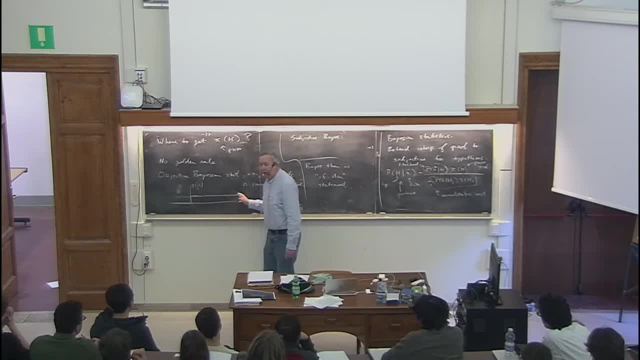 variable to be flat for positive is kind of a convention that has often been used. That's a convention, Furthermore, that doesn't really correspond to anybody's rational degree of belief. If I take this to be completely flat out to infinity, that means that I have equal probability. 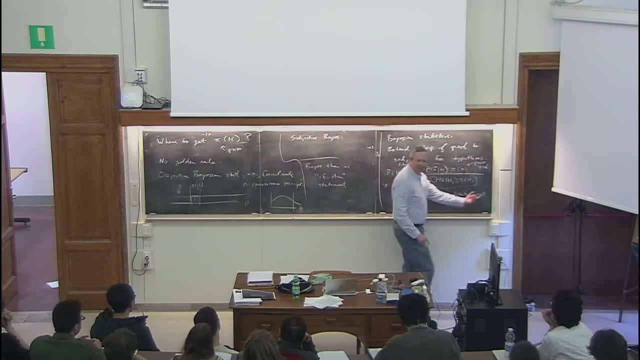 I say here between 10 to the 40th and 10 to the 40th plus epsilon. So that's not really corresponding to anyone's rational degree of belief. Yes, that's right. Yeah, Okay, Let's keep going. Yes. 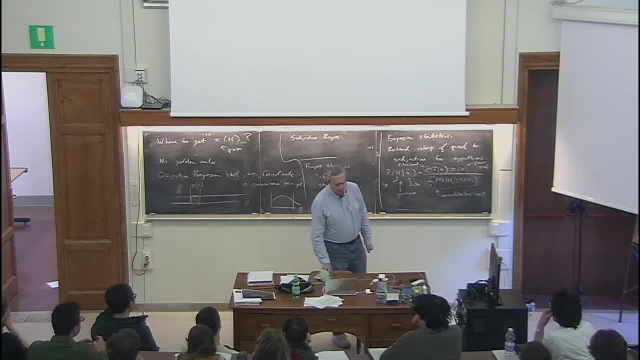 No, the prior is a quantity which we associate not to a theory but to a set of theories. Right, Yeah, no, if I assign a prior, for example, very often the case I'm considering is it's not labeled by an index, but it's labeled by a 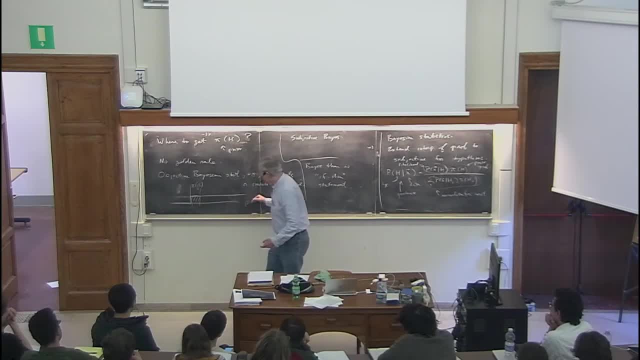 continuous parameter, And so then I have this type of a probability density. I'm not sure what you meant by consistent in the sense of. does consistent mean that the result that I get shouldn't depend on the prior? If you meant that, then the answer is no. 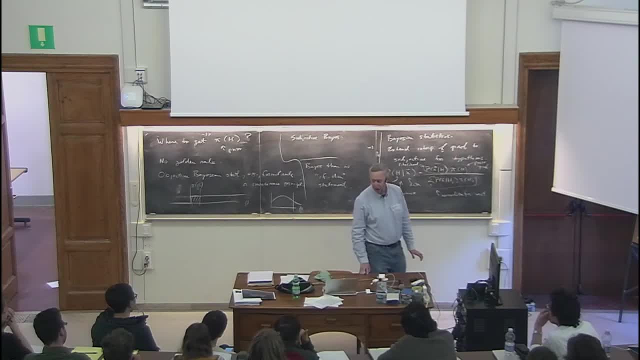 You can't do that, because the answer will definitely depend on your choice of prior. Yeah, There is a situation that I should mention while we're on the topic, and that is that, if you look at how Bayes' Theorem works, 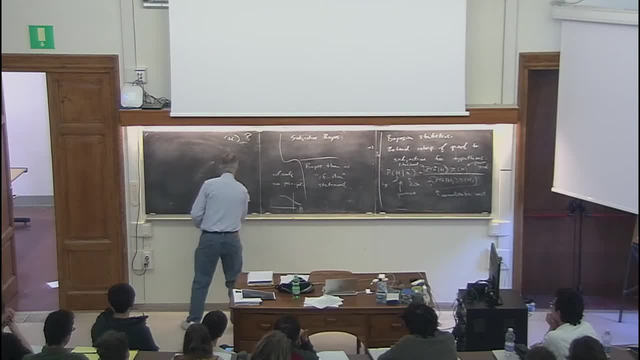 the posterior probability always depends on the product of the likelihood. with the prior. They always appear together as a product, And so very often what you can have is if we label again the hypothesis by a continuous parameter, it can be that the likelihood 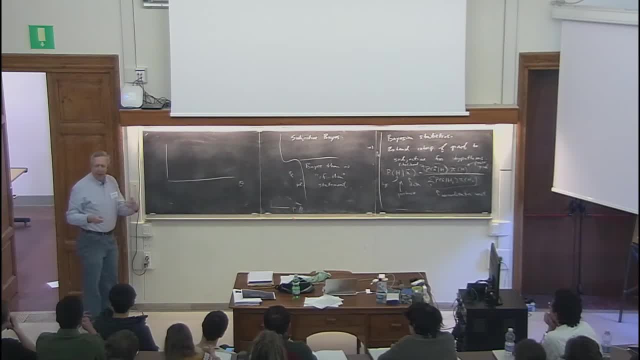 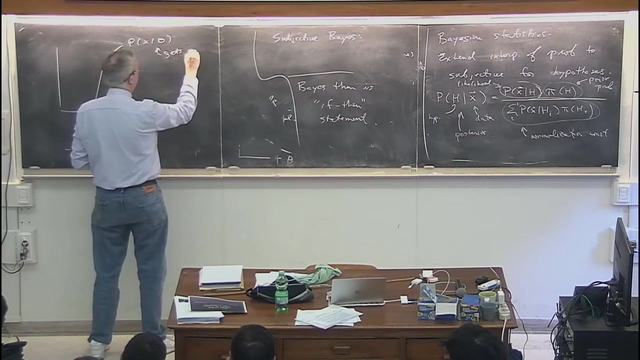 let's call this the probability for the data given by a continuous parameter. it can be that the likelihood theta, so that's the likelihood. it gets narrower and narrower as the accuracy of the data increases, improves, So it gets narrower as data. 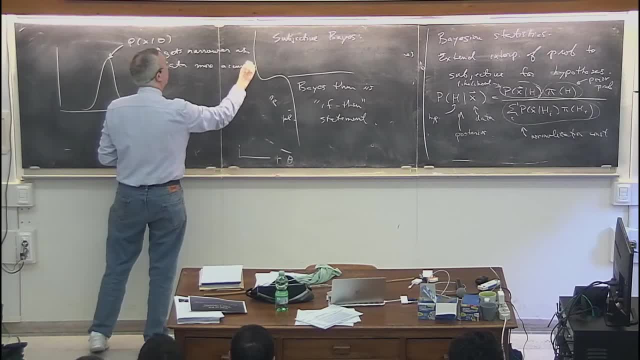 more accurate. In the context of a particle physics analysis, that would mean in the limit that you collect more data, in the limit that your data sample gets larger, And so what happens is that, if your prior degree of belief was represented by a curve, 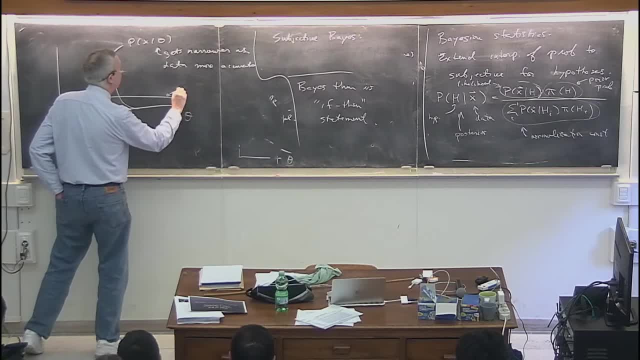 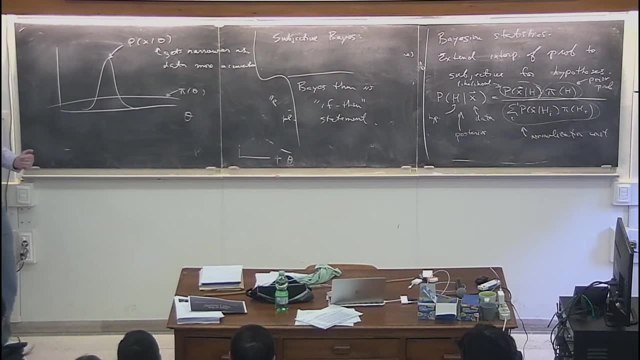 which was, say, very broad. you can see that the product of these two things is roughly going to follow the likelihood, Whereas, on the other hand, suppose that your prior degree of belief was over here and it was very narrow. So, if you consider, 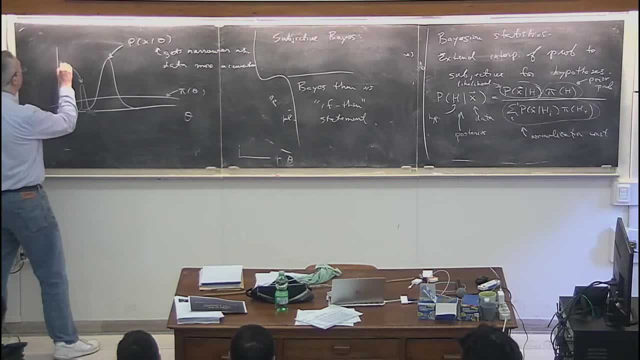 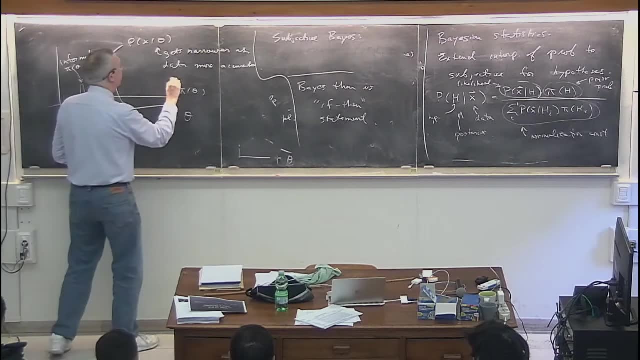 this would be a very informative prior and this would be an uninformative prior. So in this case you would say a priori you had very little knowledge about where the parameter is, and here you had a priori a very definite knowledge as to where it is. 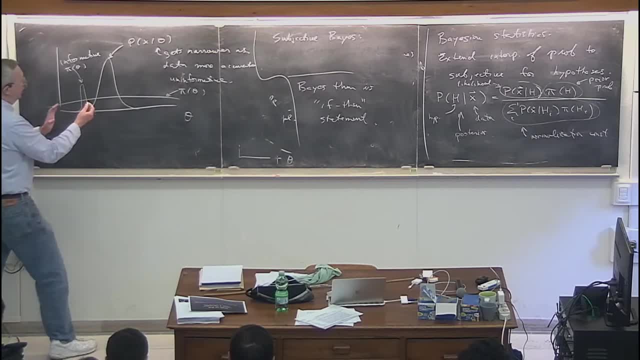 In the limit that your data gets more and more accurate. it's always then the likelihood that dominates in that product, And the posterior then more often follows, roughly speaking, the likelihood. You find yourself in a situation where you're taking the product between the likelihood. 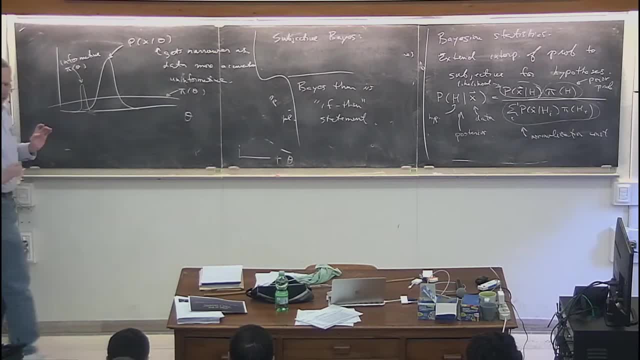 and something which is much broader than the likelihood, And in that limit you become insensitive to the exact nature of the prior. So it's important to mention that that at least in this limiting case, where your data is very accurate, you have a very large data sample. 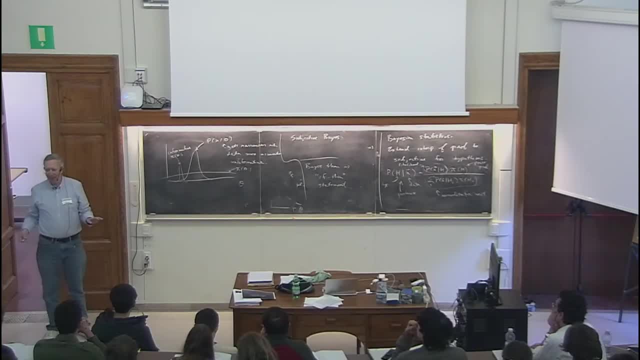 then everybody should agree. As long as you start with a sufficiently broad prior, you can imagine a situation where I say: well, here's the likelihood, and as I collect more and more data it gets narrower and narrower. But suppose a priori, 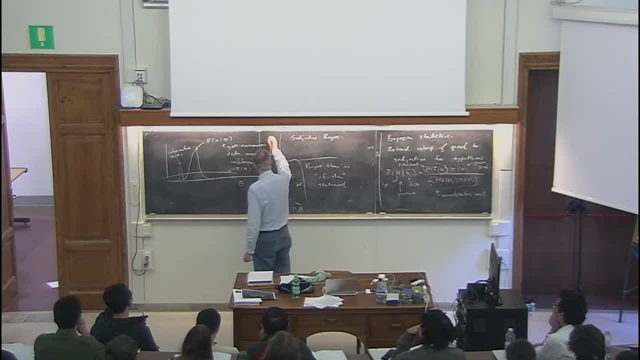 I said: that's where I know the data is. It's a delta function right there. Well then, the product of this, and that always gives you still a spike here. So you have to start with an open mind, You have to start with a sufficiently 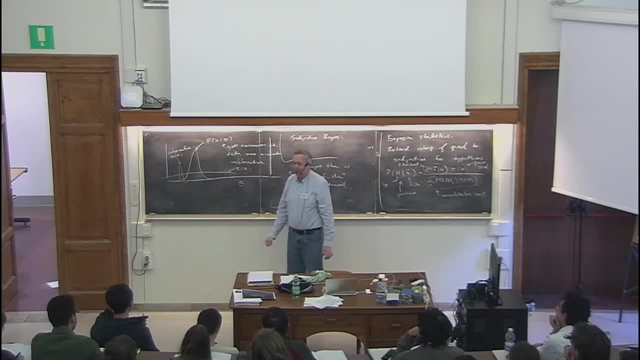 large, broad, prior: Yes, I see this discussion is going to go on. That's good. If it's an independent experiment, yes, you can do that. But here's what you can't do. You could say: well, the prior is some degree of belief that it would. 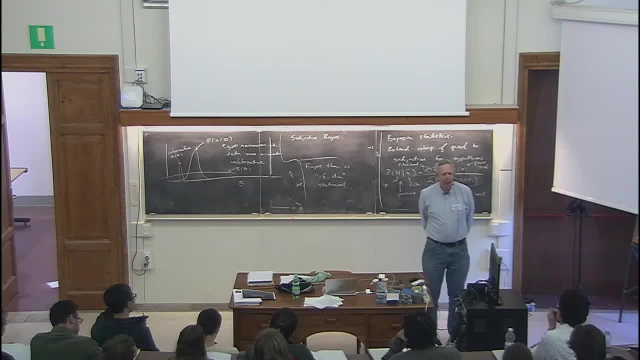 be appropriate to have before doing the experiment. And so you take that prior, you multiply it by the likelihood, you get the posterior And you say, ah, that's what I now believe after doing the experiment. And then you can sort of think: well, 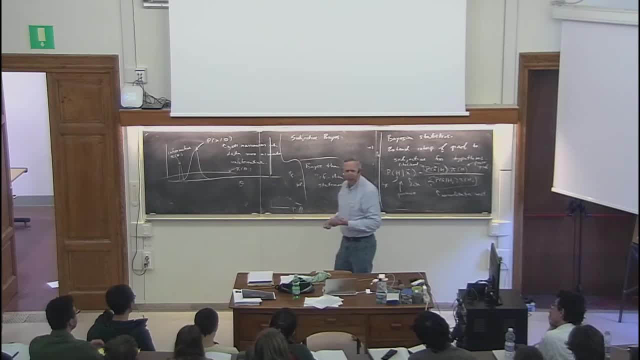 if it's okay to believe that after doing the experiment, surely it would have also been okay to believe that before doing the experiment, Why not? And so you say I should have taken that as my prior, And you put that back in and you iterate. 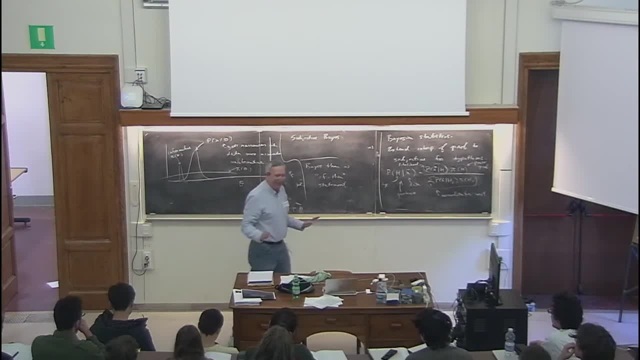 and that's wrong. That's not what Bayes' theorem says to do. Okay, But if you actually combine experiments, new experiments, then that's absolutely correct what you say. Repeating an experiment with independent data with new data, yes. 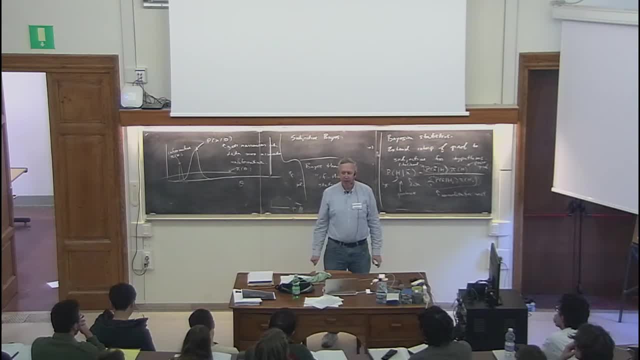 It will the new prior that you would use, that is to say it's after having done the initial measurement before doing the subsequent measurement. yes, it would be narrower in the sense that it would contain more information already about the parameter than you had before. 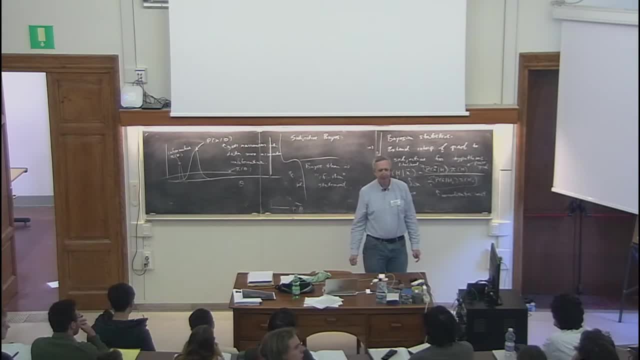 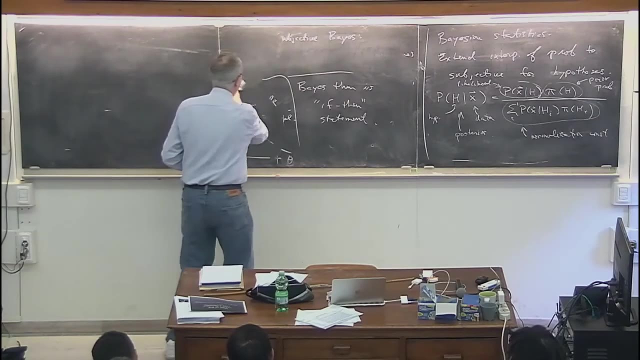 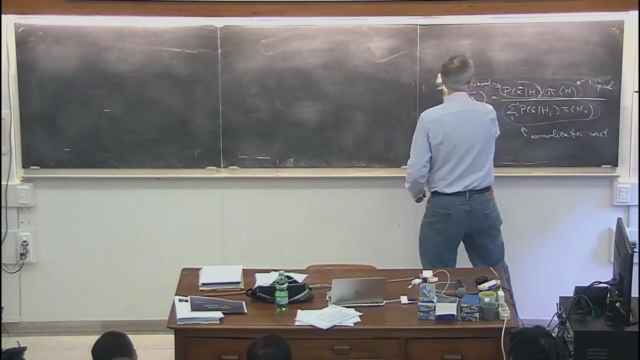 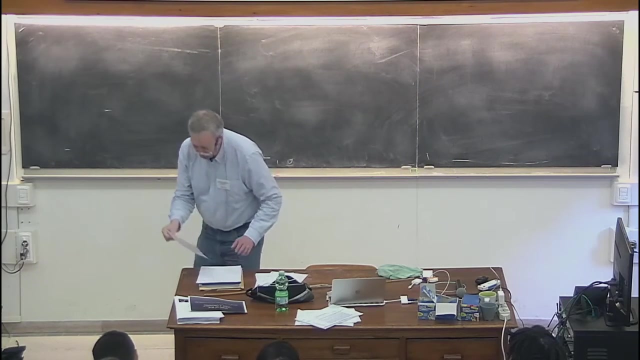 Yeah, Narrower. Yes, Yes, that's correct. Okay, Let's go on. I just want to introduce quickly some vocabulary and notation that I'm going to be using in the following lectures, And this concerns random variables and expectation values. 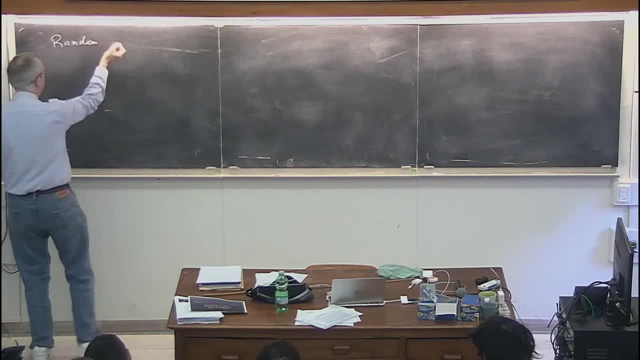 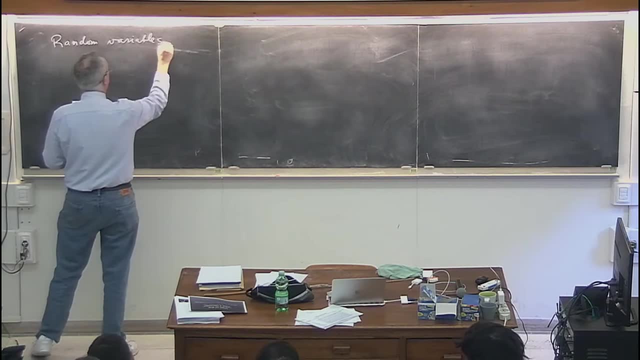 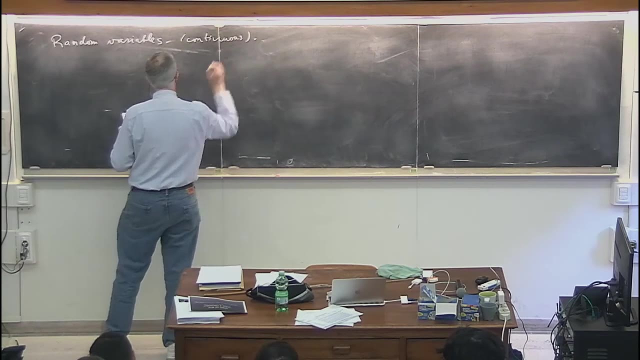 So this is. everybody knows this. I just want to put this on the board to solidify my notation. I'm going to do this first for continuous random variables. So first of all I should say what I mean by a random variable is a numerical label. 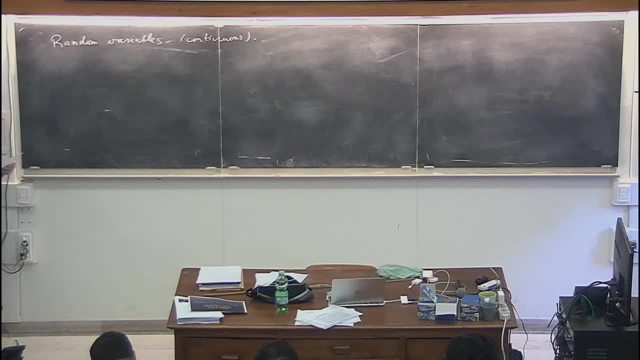 for any element in the sample space or any element in the hypothesis space, if we're doing Bayesian statistics, And so the most important function we have is the probability density function, And I will usually just say something like f of x, And so by that I mean 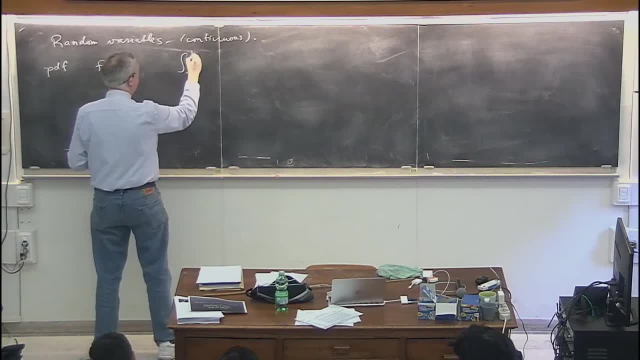 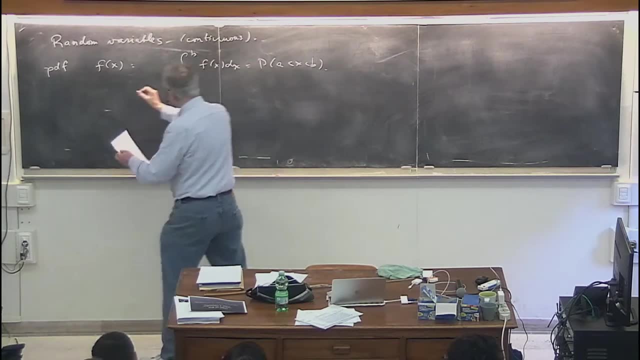 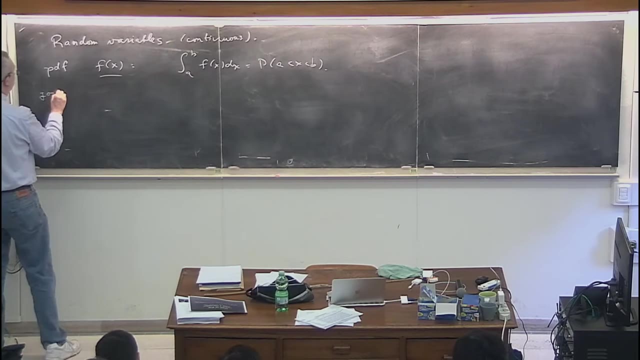 something that you can integrate between two limits to get the probability that the random variable lies between the limits. So I'll use the letters pdf for that. So I will use the phrase joint pdf if this thing has more than one argument. So x, y and so forth. 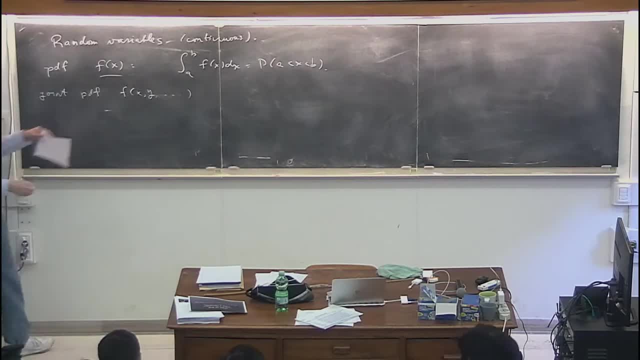 So really I could just still call that a pdf, but I always stick in the word joint if it has more than one random variable. If you have a joint pdf but you're only interested, say, in the pdf of one of the variables or some subset of those variables, 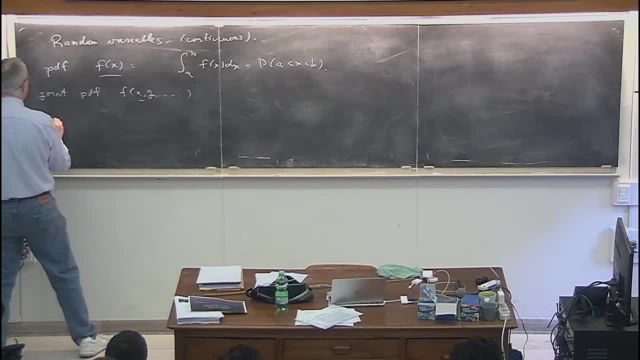 then of course what you do is you integrate over the unwanted variables And that gives you what we call the marginal pdf. So let's suppose you wanted the pdf of x and what you had was the pdf of x and y. then of course you just integrate. 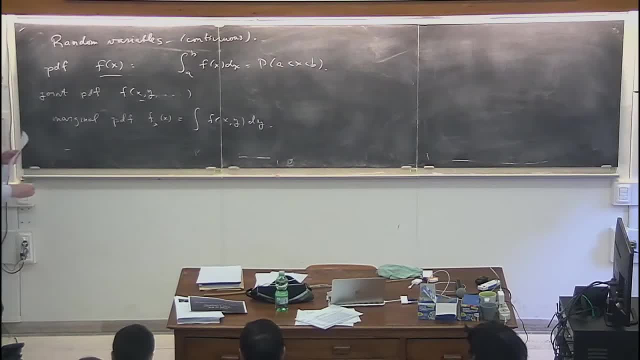 over the unwanted variable, And so I call that the marginal pdf. Sometimes I will be labeling these pdfs just by their arguments and I'll use the same letter. So the way that you know that that's not the same function as that, even though it has the same letter, is just by the argument list. 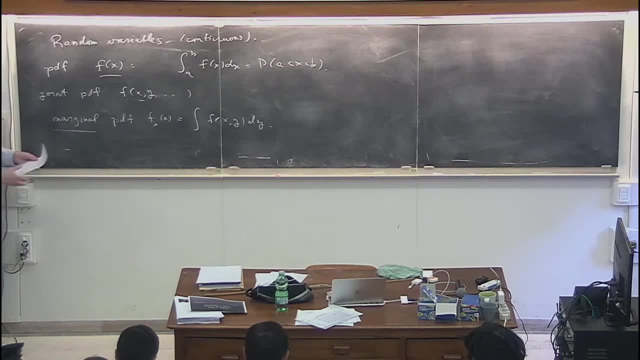 Sometimes, to avoid confusion, I'll put a subscript or use a different letter. And then, of course, if you want to know the pdf of, say, x, given that y is held to a fixed value, then of course that's what we call the conditional pdf, And the conditional pdfs would. 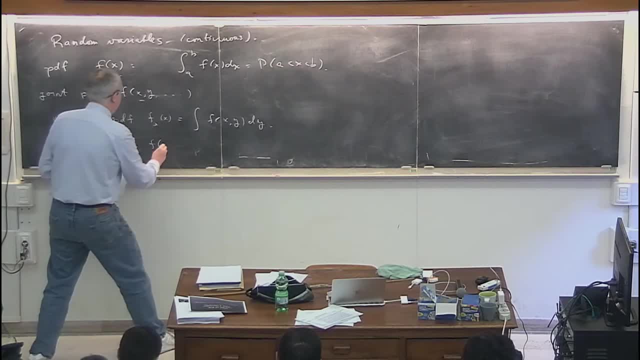 obey Bayes' theorem in a manner analogous to the way I had it written previously with the set theory language. So we would say conditional pdf of x, given y is the joint pdf of x and y. That would correspond to the intersection operation Divided by the pdf of the. 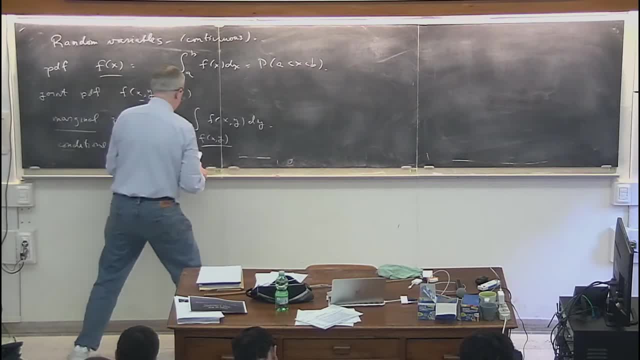 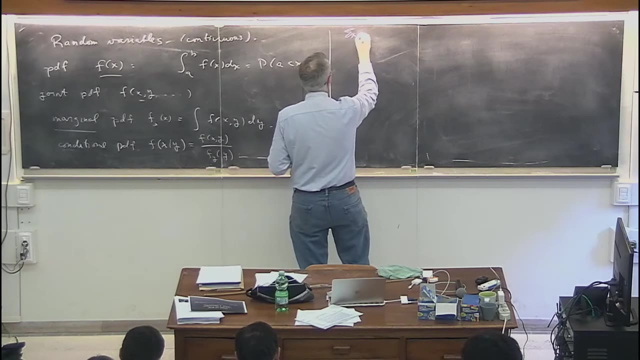 condition you impose. So in that case, that's going to be the marginal pdf of y. Okay, so I just wanted to make sure I got the basic vocabulary down And then, similarly, my notation for expectation values is the one that is standard in statistics but not so standard. 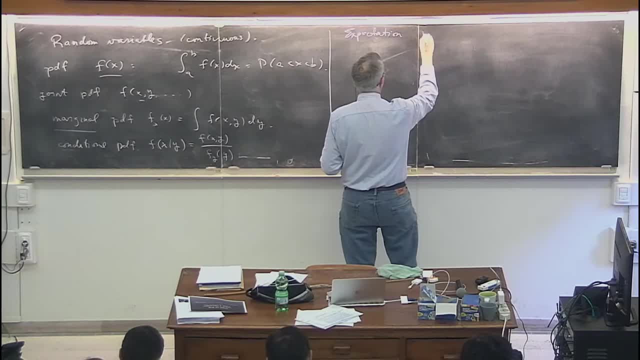 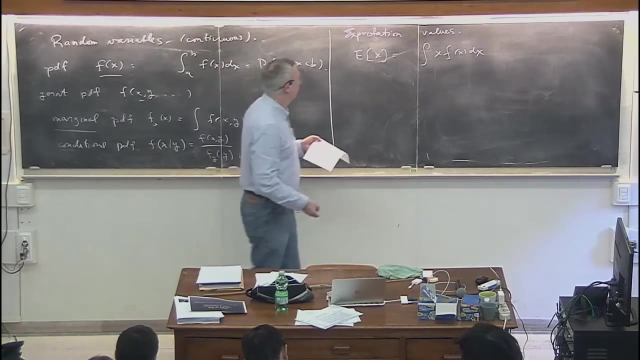 in physics maybe, So expectation values. I will use this e with square brackets. Okay, so that's for a random variable x that follows a pdf f of x. that's what I would mean by the expectation value. Obviously, I'm showing these formulas for 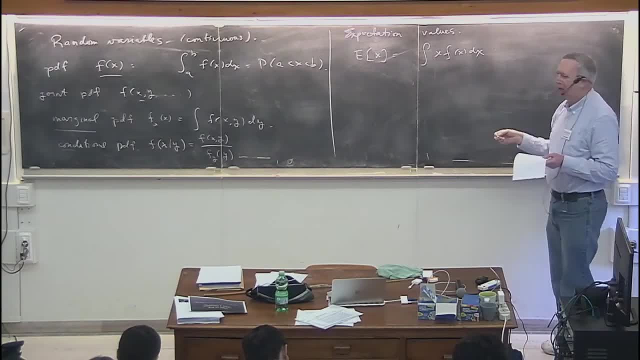 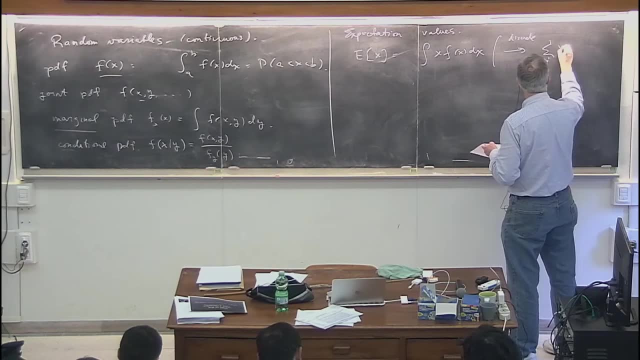 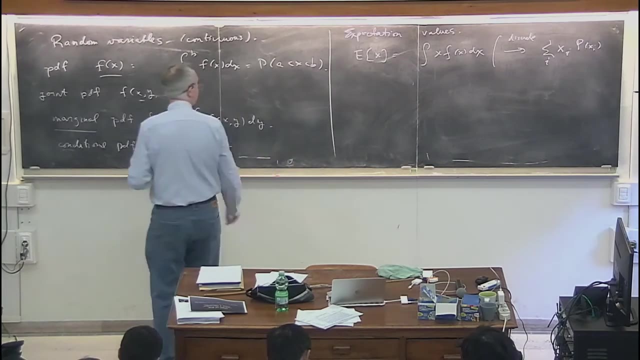 continuous random variables, and so if you had a discrete random variable, then you would replace this by the sum of xip of xi, something like that. So integrals just become sums, and so forth. One piece of notation that I will very often use is: I'll use: 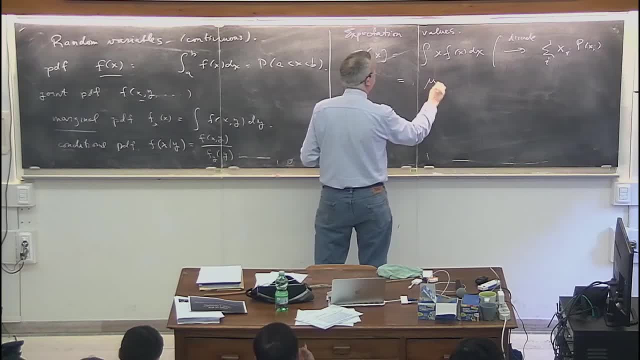 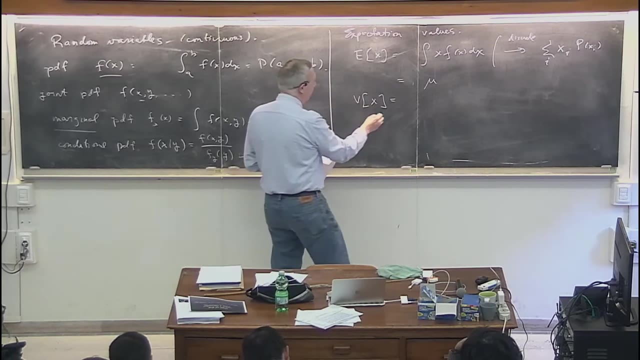 some Greek letter like the letter mu for the expectation value, And so just to warn you that that's very often used. I define the variance of a random variable using this capital V operator, and that's just the expectation value of x minus mu, The quantity squared. 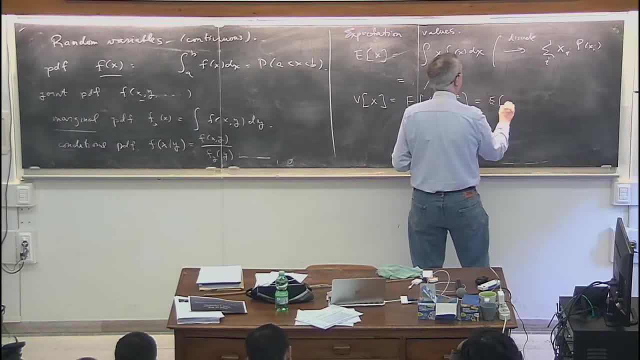 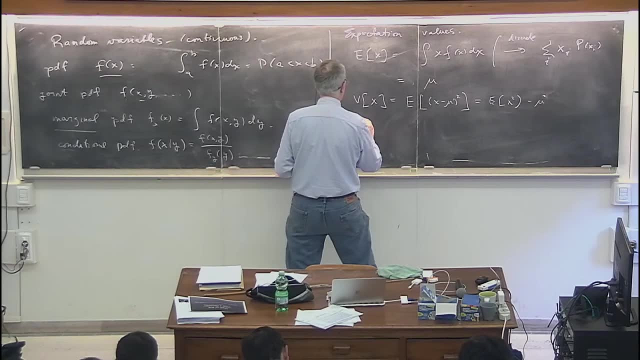 and of course that's just the expectation value of x squared minus mu squared. And then, very often as well, if we have two random variables, I can talk about their covariance, Covariance of x and y, And that is just the expectation value of their product. 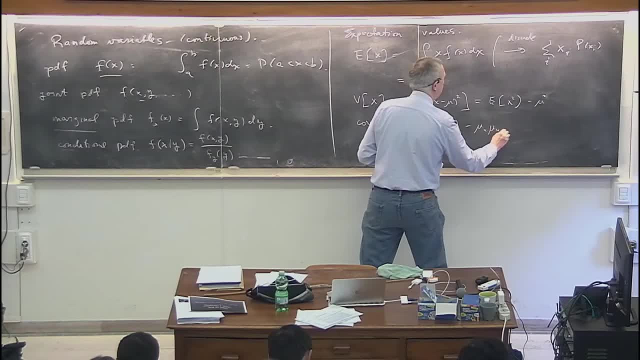 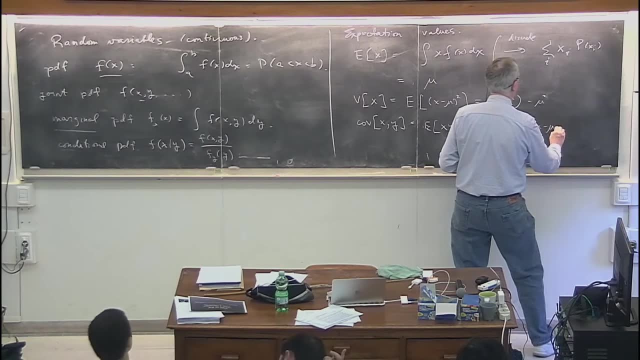 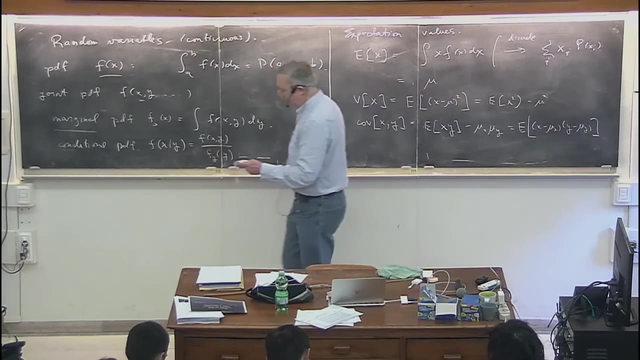 minus the product of their two expectation values. You can write that in an equivalent way. You can write that as the expectation value of x minus mu, x minus mu y. Right, So I'm out of board space, I'm going to write it here. 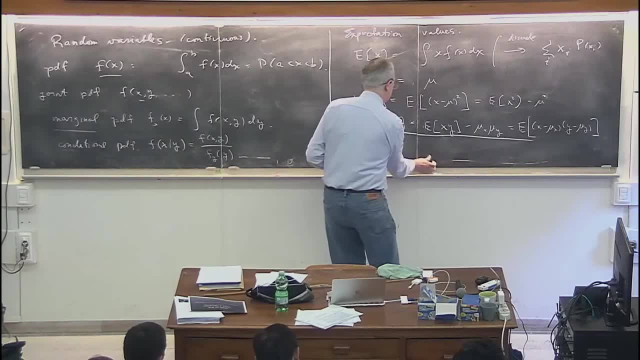 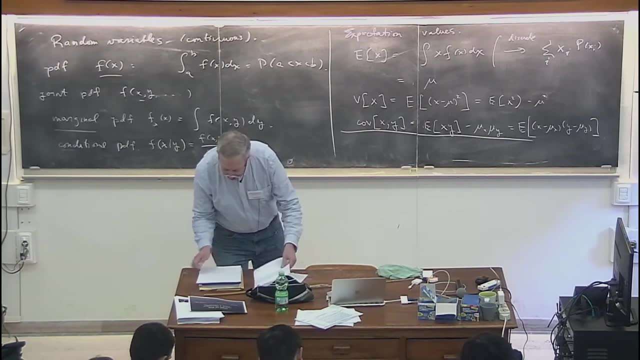 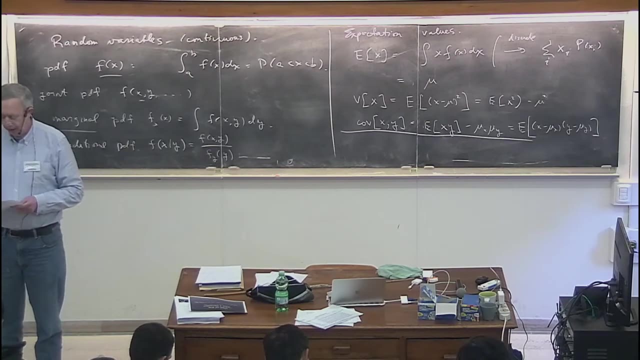 I just wanted to. well, that's enough. So that's just my notation for there. I'm going to assume that you're familiar with most of the probability distributions that I'll be discussing, like the Gaussian distribution and the exponential distribution, Poisson, And I'll write those down as we need them. 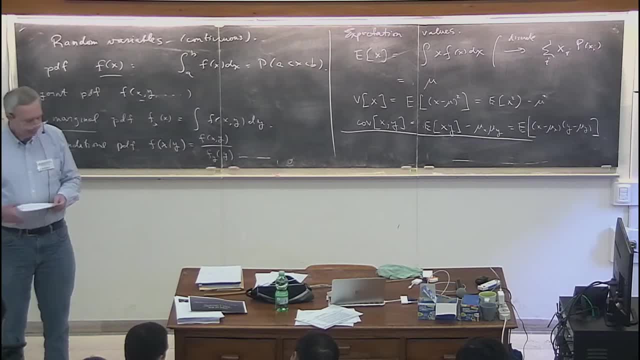 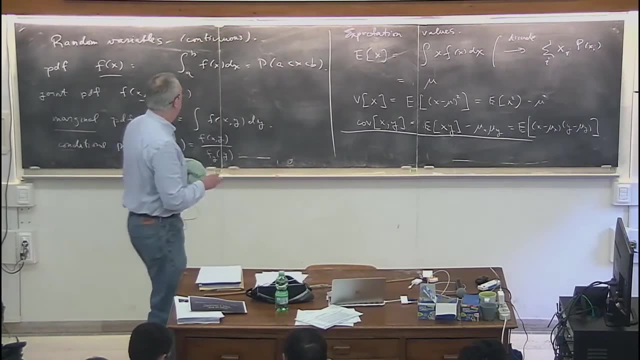 But let's not waste time writing those down here, Okay? So very often, the PDF that I might be using to model my data would contain some unknown parameter, And what I want to talk about now is a way to use the data to estimate the values of the parameters. 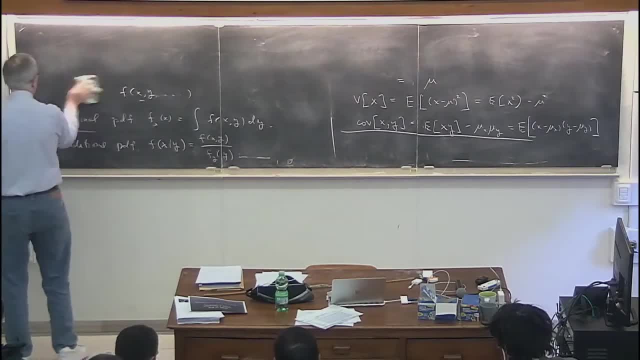 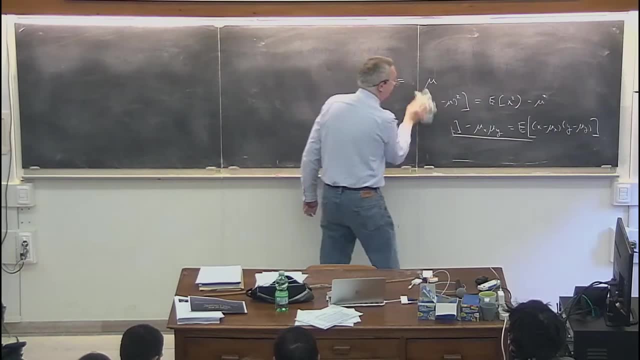 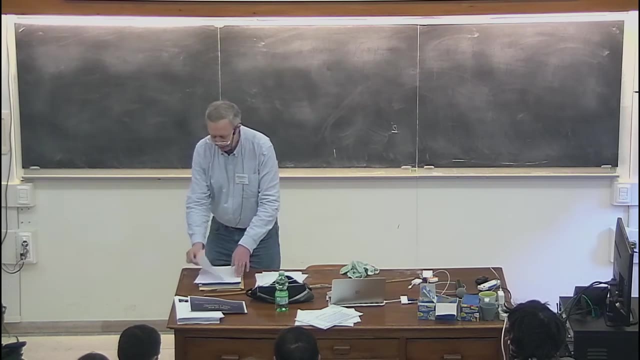 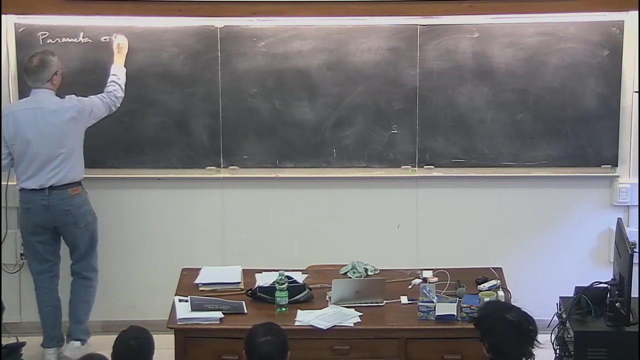 So that's an important task in statistics. That was my bullet point number one that I had in the first list, And so let's go through that. So, parameter estimation: How am I doing for time, by the way, When should I stop? 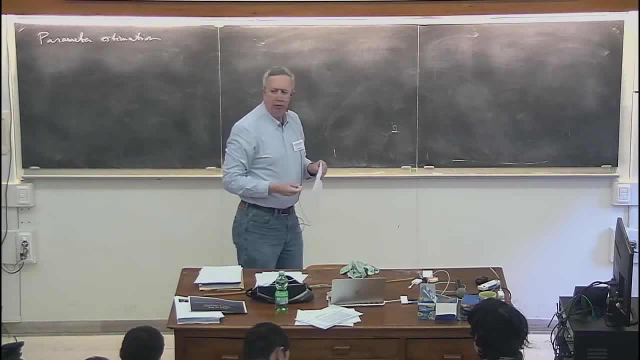 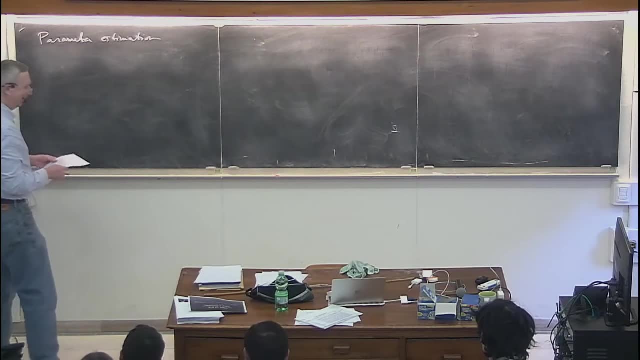 Okay, That's good. Okay, Alright. So let's suppose that I have a random variable x and then it follows: I'll use that symbol, the tilde, to indicate that the random variable x is sampled from a PDF f of x, and then I'll write here a semicolon: 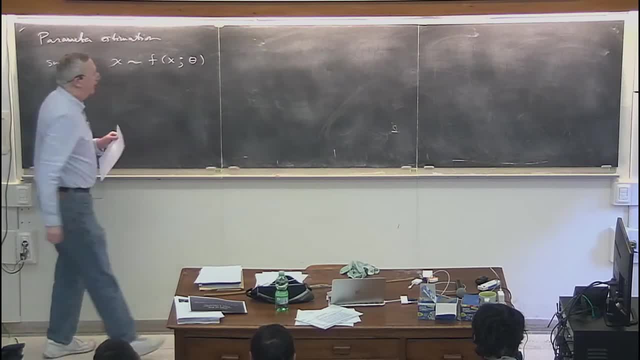 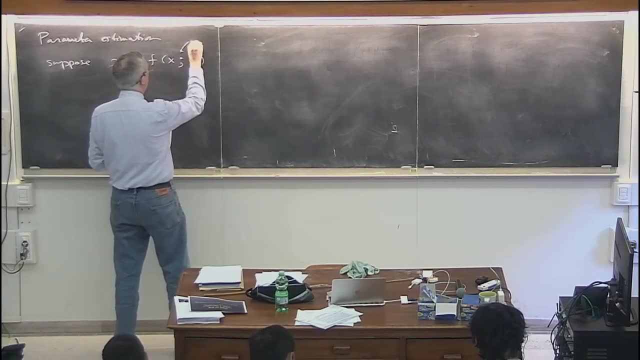 and indicate that this functional form for the PDF is going to contain some unknown parameter. Sometimes, instead of the semicolon, I'll just use a vertical bar, and that would be the same language as the language of conditional probability. That would be like f of x, given theta. 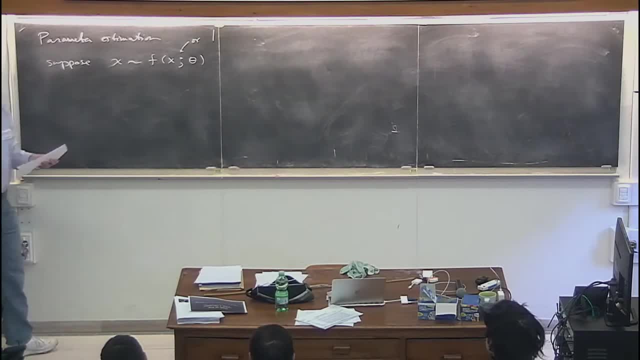 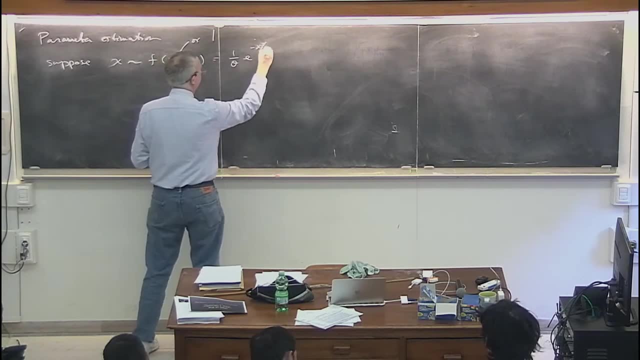 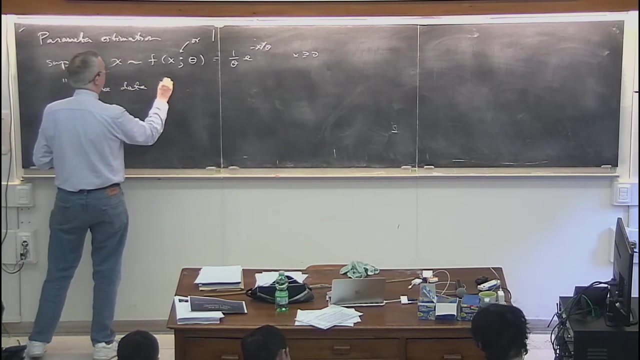 It's essentially the same thing in this regard, And so let's suppose it's an exponential distribution And let's suppose that we have data. I'll put a vector over the x, because maybe it's more than one x value, maybe I've sampled n values. 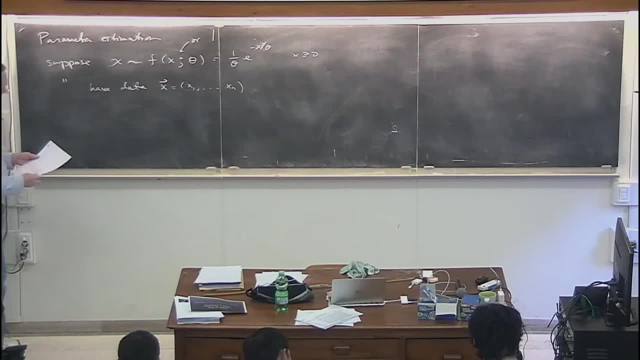 Alright, And what I want to do now? my goal is to construct a function- I'll call this theta hat- and it's a function of the data. Alright, And the goal of this function is to estimate theta. So whenever I have a hat, this is what I mean by an estimator. 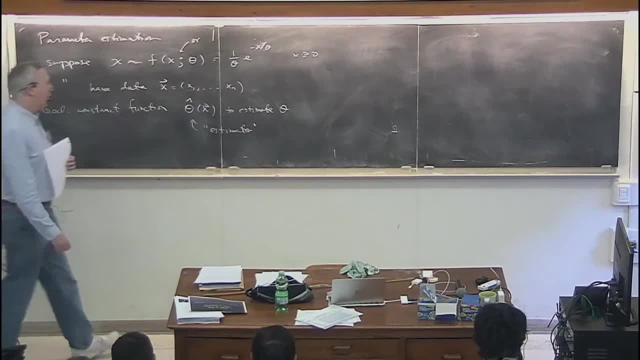 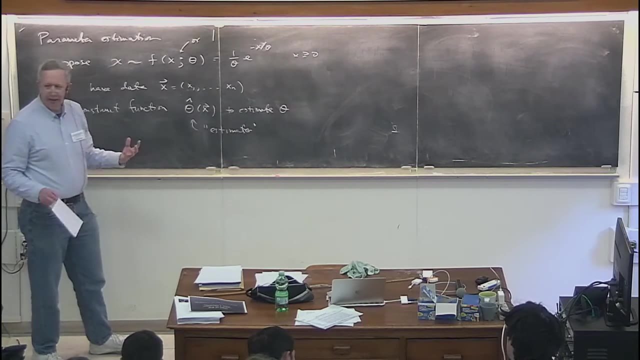 So physicists are not great at distinguishing between a function as a mapping and the value of that function when you evaluate it with a particular data set. So sometimes I'll say estimator if I want to insist on the function and I'll say estimate if I mean the value. 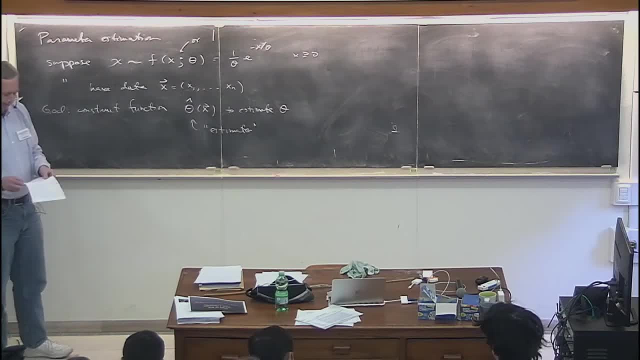 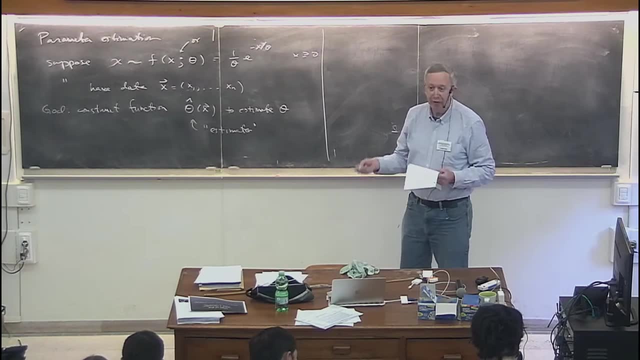 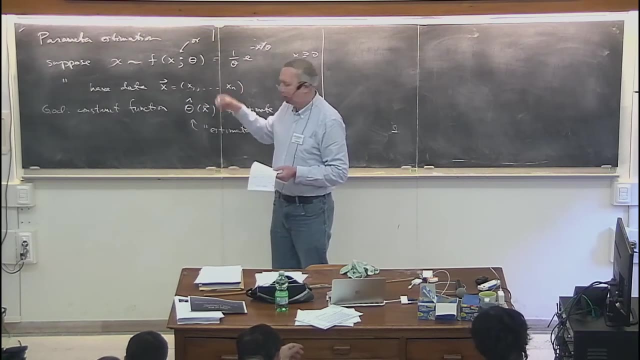 of that function, But because the estimator is a function of a random variable, it itself must be a random variable. If you were to repeat the entire experiment with new data- independently sampled data- you get a different value for theta hat, and so you could do that many times. 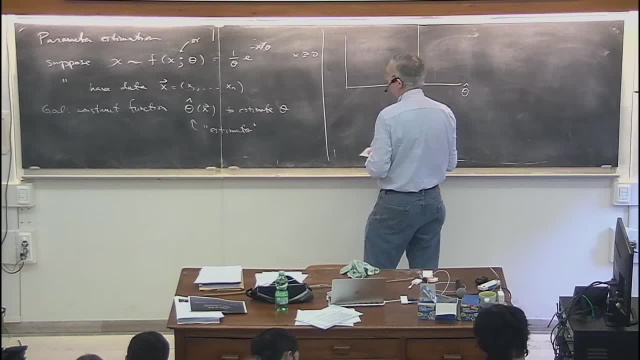 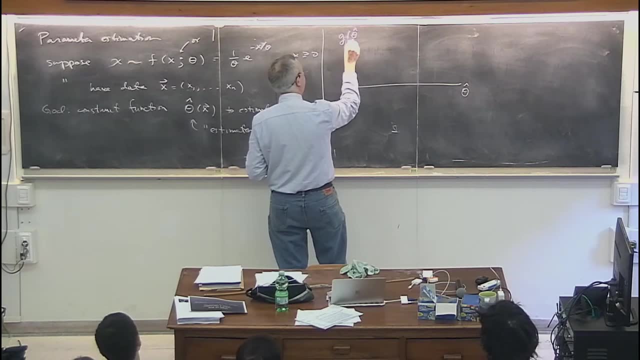 You could imagine making a distribution, a histogram, of the values of theta hat, and this would correspond to a new PDF. I'll use a different letter, g, because it's the PDF now of theta hat. That PDF, of course, depends as well on the true value of theta. 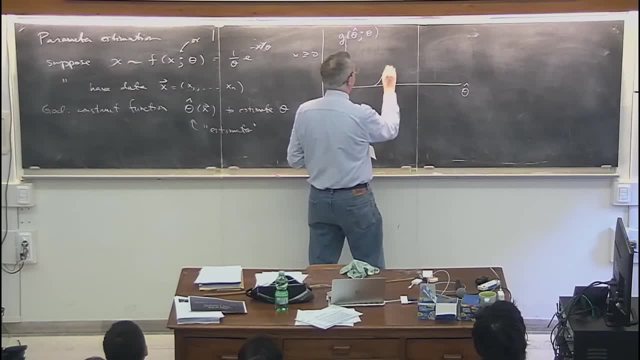 So I can imagine that this PDF maybe looks something like that. It might look like that if the true value of theta were somewhere there and if the true value of theta were over here, then it would be in a different place. Now, why am I going into this? 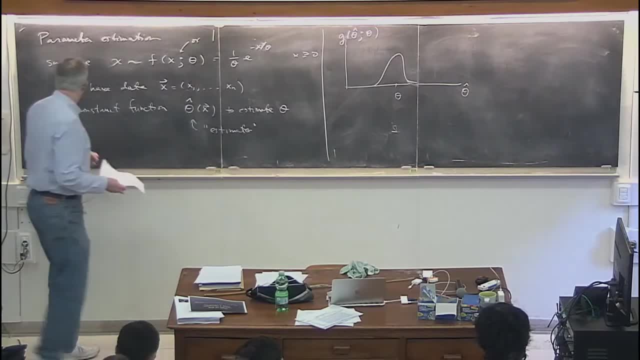 I should have stopped here and said: look, if this is the goal to construct that function, why don't I just write down the right answer? And the answer is that there is no unique recipe. There is no unique best estimator in general In certain specific cases. 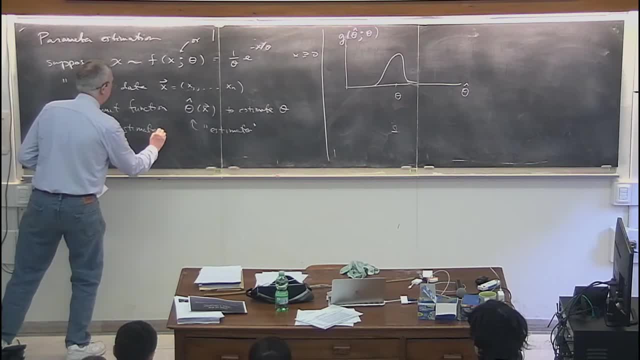 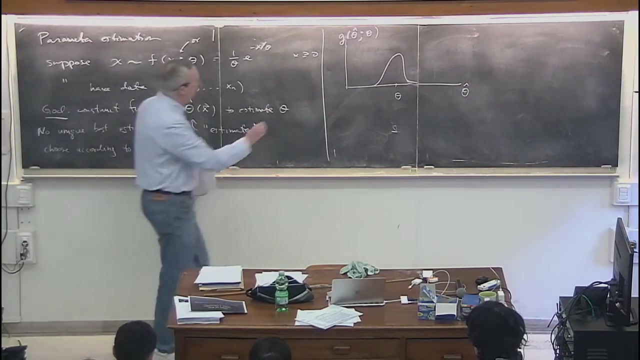 you can point to one which is better than others, but there is no unique best estimator. We have to choose amongst possible estimators according to their properties, And the properties that I am referring to are going to be the properties of this sampling distribution, The distribution that you would get. 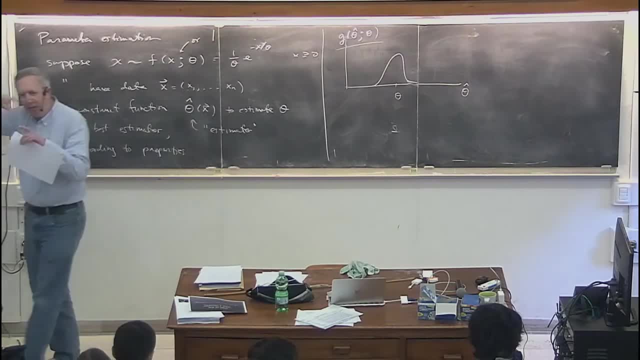 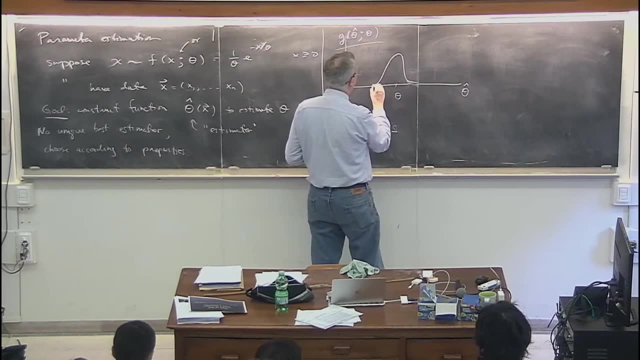 if you were to repeat the entire measurement many times. So let's suppose that this is the result from a particular estimator. it had this sampling distribution. I could construct the estimator in a different way, such that the sampling distribution might be over here And the distribution of estimates. 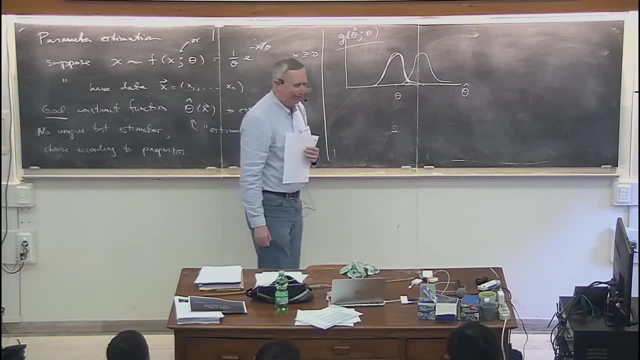 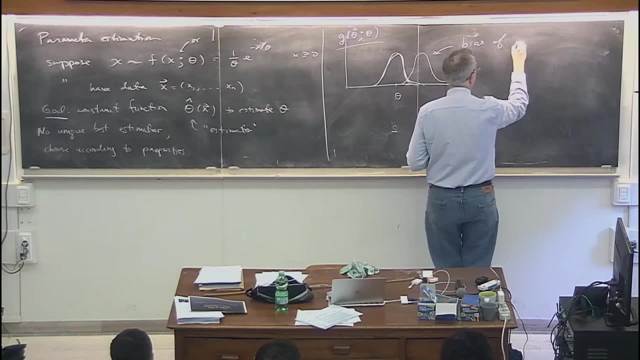 is over there, So that is less good. So one of the properties that we would look at is what is called the bias of an estimator. B is defined as the expectation value of the estimator minus the true value. So the way I have drawn it here, 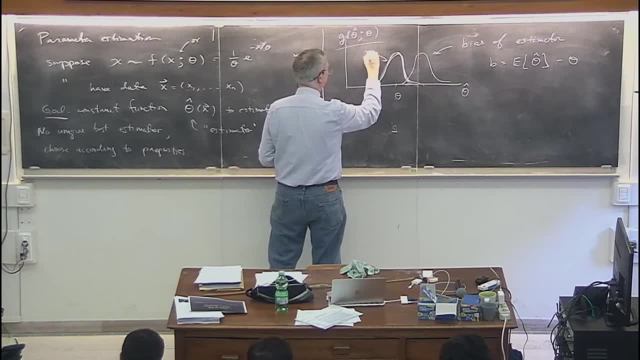 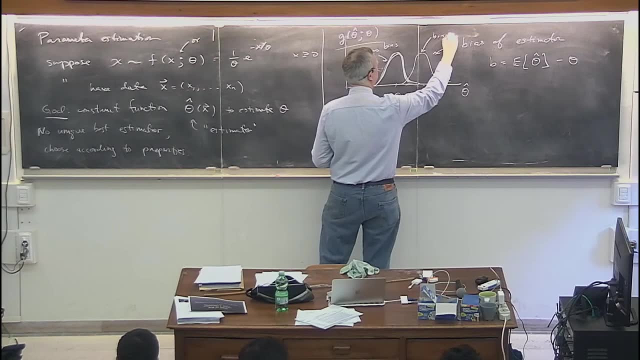 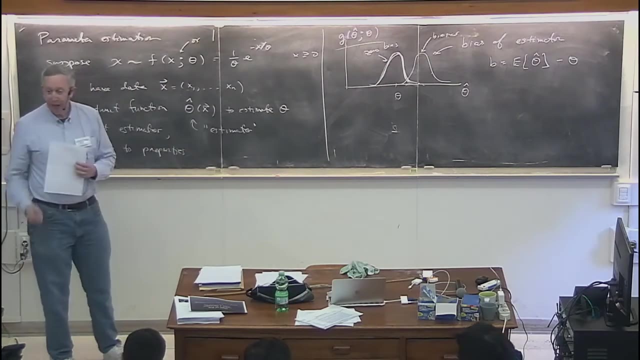 is that this estimator would have zero bias And this one here would be biased 1s, 2s, I don't know. Okay, so that is one of the properties: You would choose an estimator that minimizes the bias. 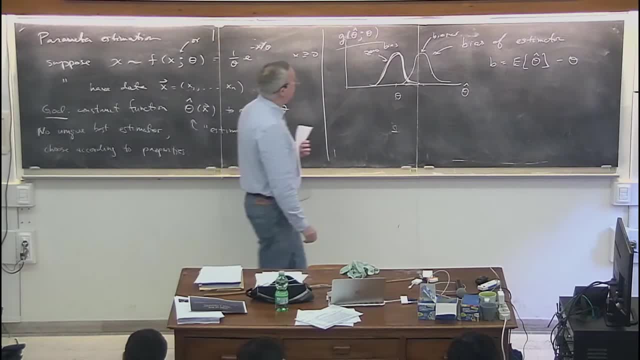 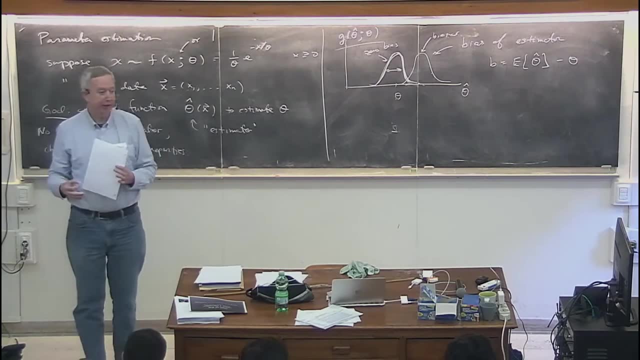 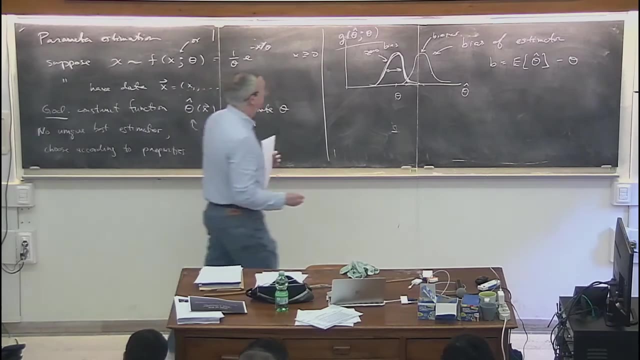 On the other hand, what is the width of this distribution? of course represents how reproducible the measurement of theta is in an experiment of that type And obviously if that distribution was narrower it would be better. The width of this distribution represents the statistical error. 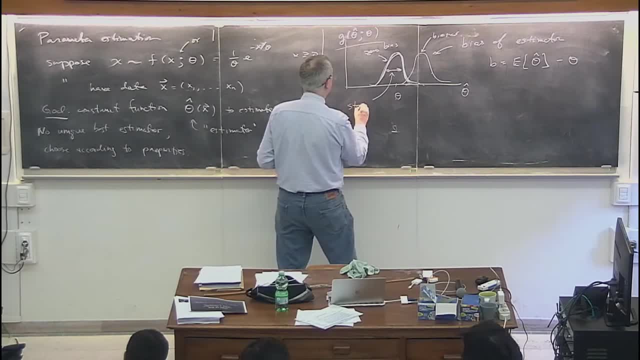 So I will say that sigma, the standard deviation of theta hat, is the statistical error of theta hat, And we want that to be small. So, for example, if I had another estimator that led to a sampling distribution that looked like this, it would also be unbiased. 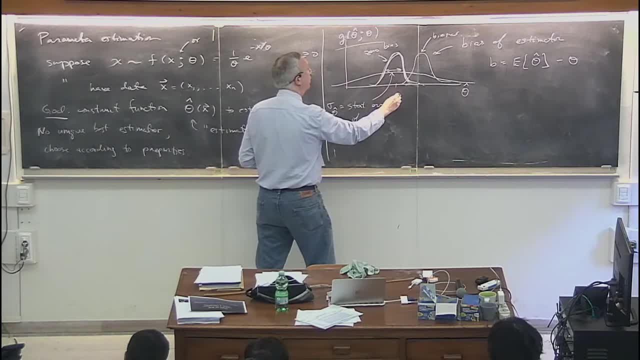 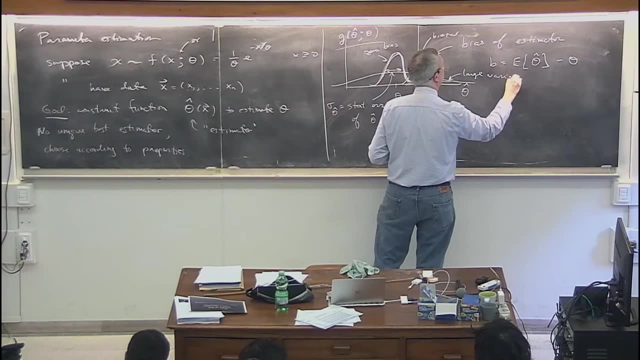 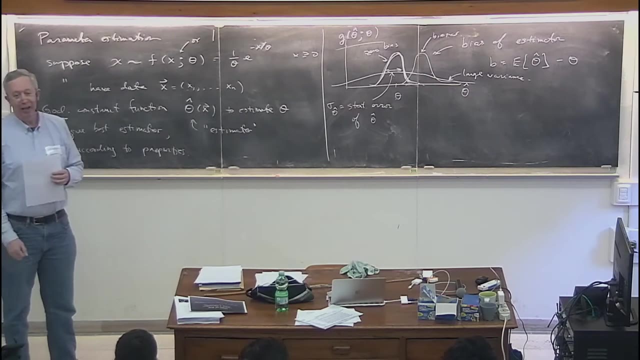 because its expectation value is equal to the true value. So that is another criterion. A second one: We want the smallest possible variance. And so now you might be thinking it is very simple: We have to choose the estimator that gives us the smallest bias. 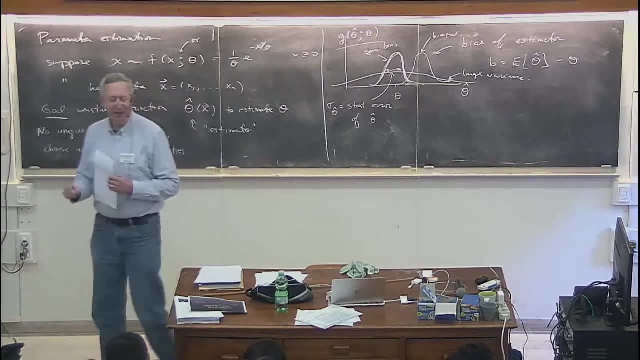 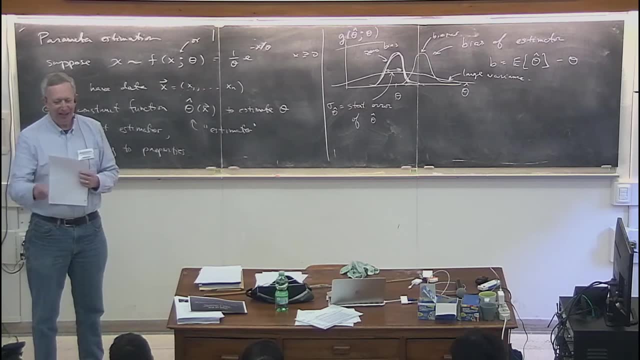 and the smallest variance. You can't do that. They are conflicting criteria. in general, In general, you can't optimize the highest, longest bridge in the world. You can't optimize with respect to more than one criterion. You can't have the estimator. 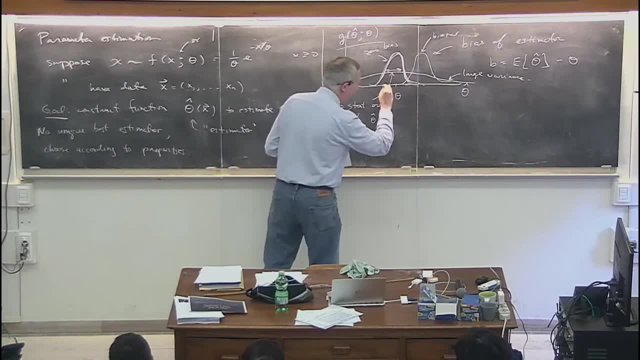 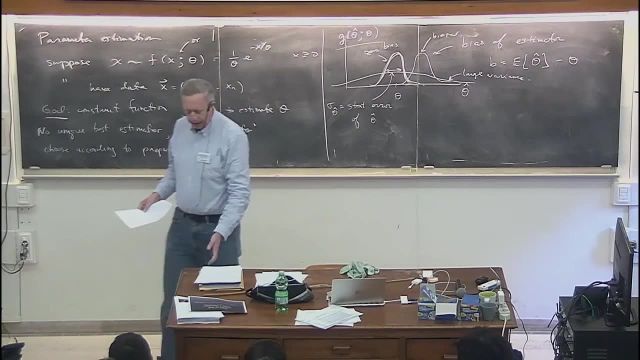 that has the smallest bias and the smallest variance in general. And there are other criteria that we could list, But those are the two important ones, So let's stop there. Robustness, consistency, blah, blah, blah, But these are in general. 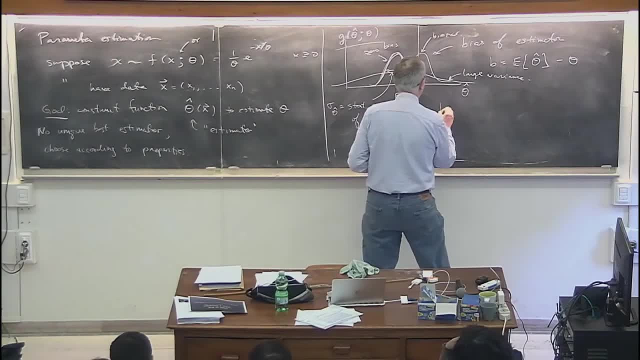 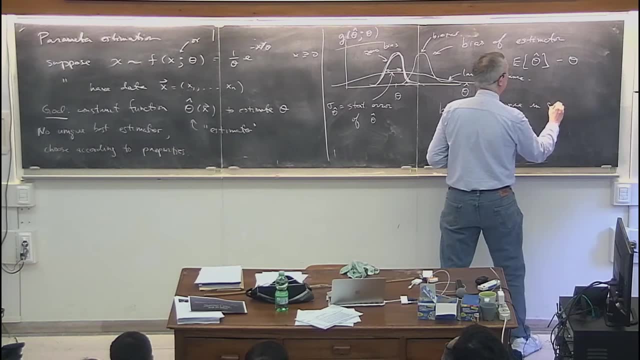 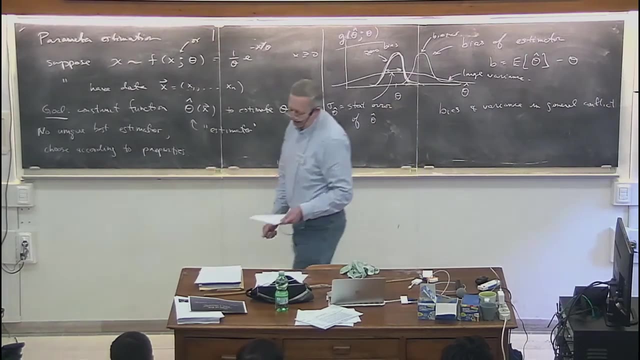 conflicting Bias and variance In general Conflict. And so now you might be thinking: well, to my mind, bias sounds worse, Because bias sounds something like scientific dishonesty or something like that. 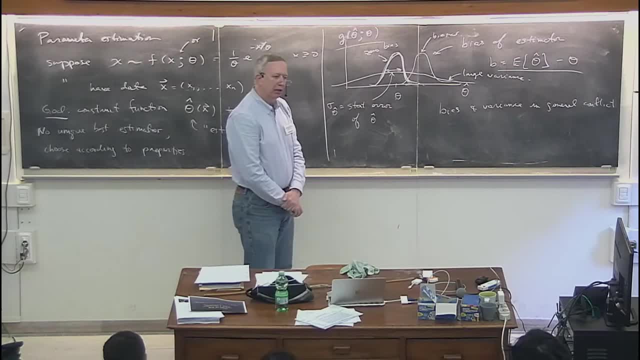 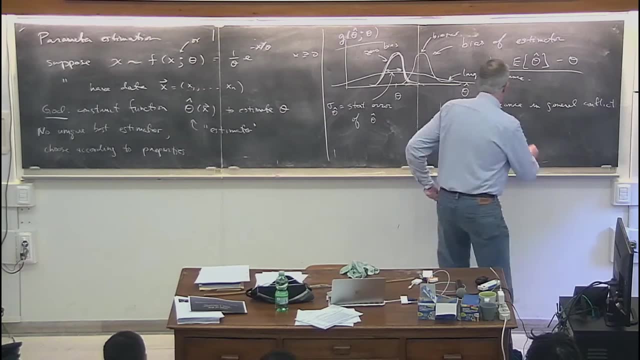 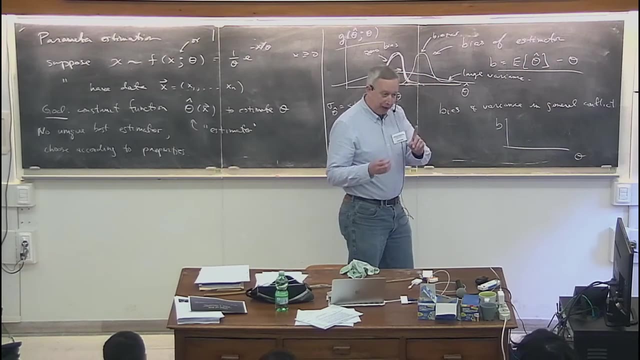 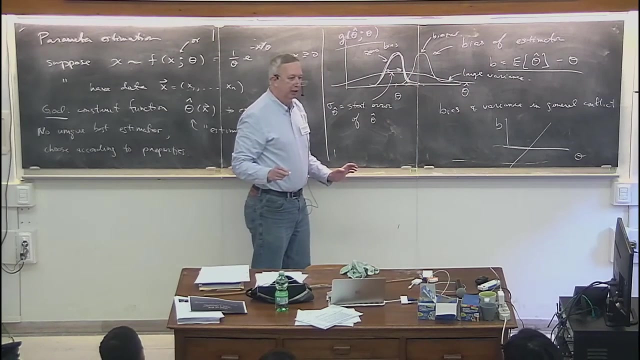 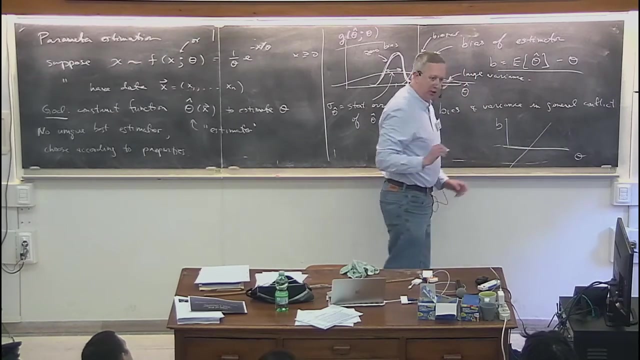 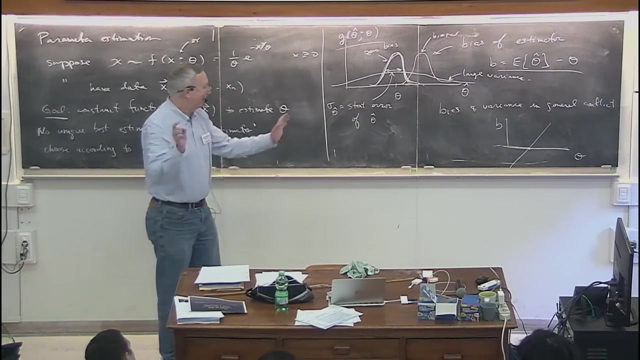 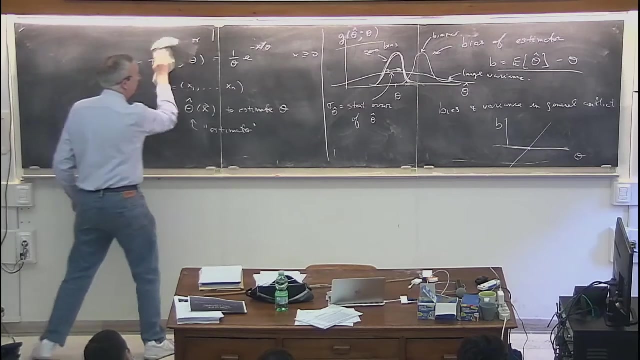 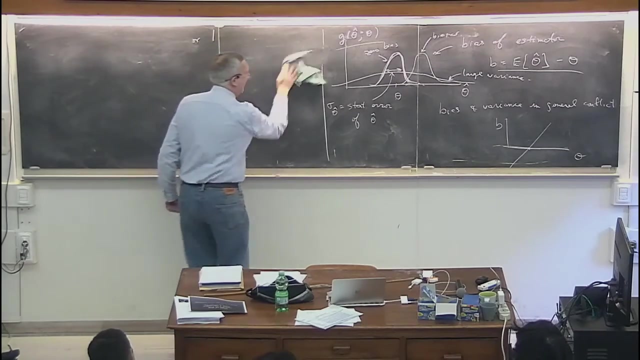 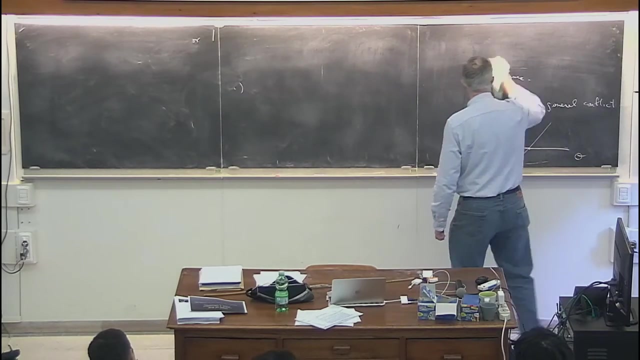 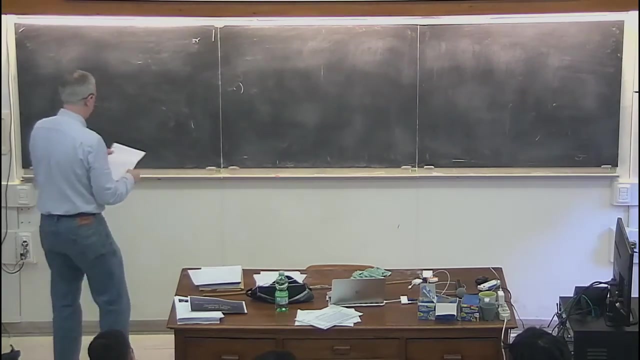 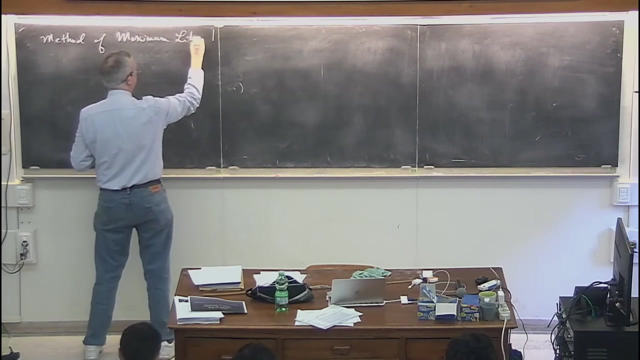 The method that I want to introduce is what's called the method of maximum likelihood. I'll very often just use the abbreviation ML for maximum likelihood. 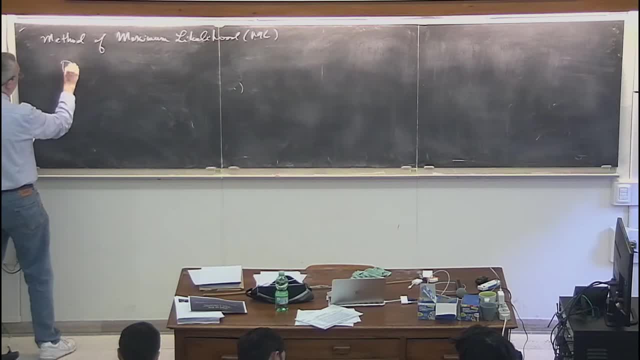 The idea is that if I have a measurement that produces some data and it contains a parameter, and that function is what I will refer to as the model or the hypothesis. but the model or the hypothesis means the rule, The rule that assigns the probability for data for every point in the parameter space. 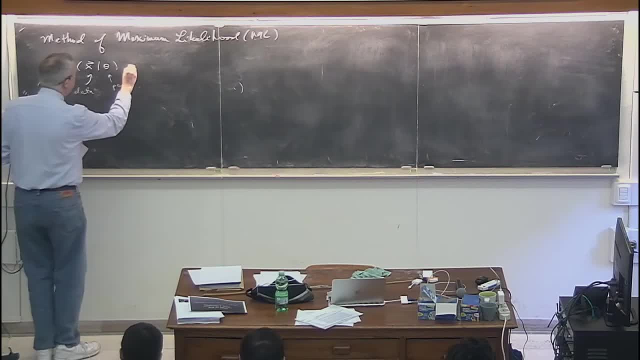 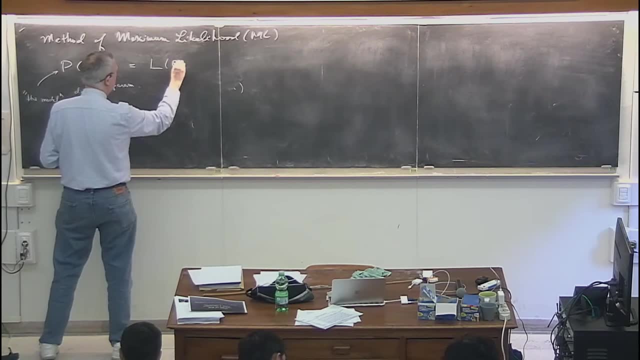 If I regard this thing just as a function of theta or just as a function of the label of the hypothesis, I call that the likelihood. So here I suppress the notation, I suppress the x. x is still in there, the data is still. 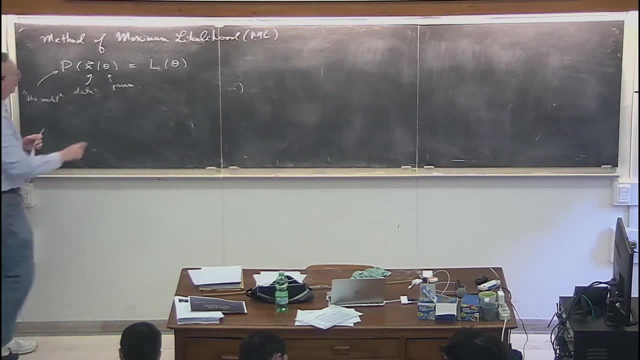 in there. but if I only look at the dependence of this quantity on the hypothesis or the hypothesized parameter, I call that the likelihood. Okay, You'll notice, in Bayes' theorem I used the same thing, but in Bayes' theorem I didn't. 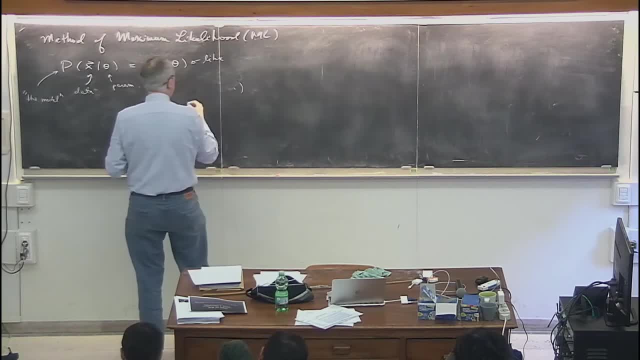 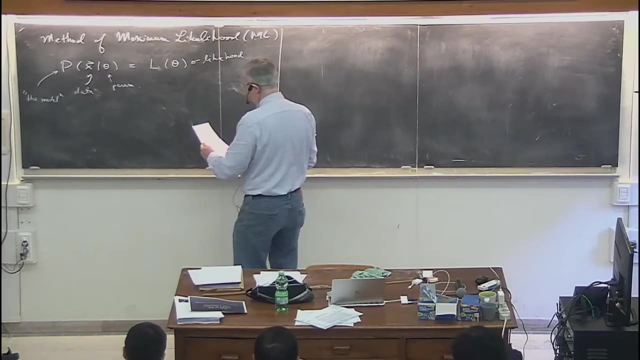 suppress the x. But here, in this context, I want to use the notation L of theta for the likelihood, And so let's suppose that we have. I'm going to skip this and go here. So here's the method. The method says that the maximum likelihood estimate 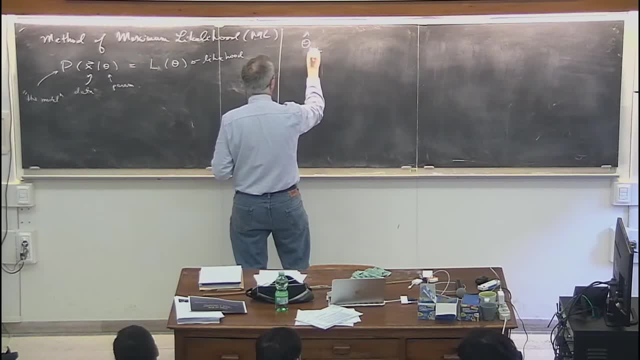 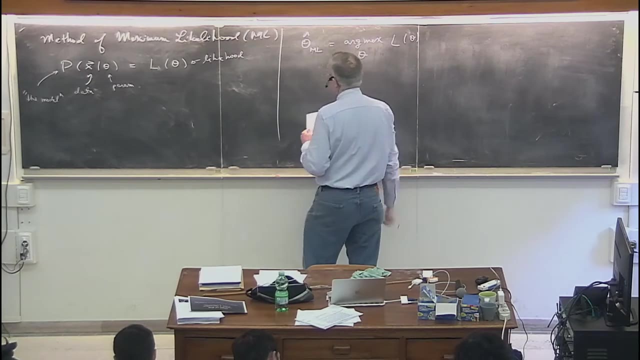 Usually in the subsequently. I won't put the ML as a subscript, but it'd just be. the maximum likelihood estimator is equal to the value of theta, which maximizes the likelihood. So that's easy, And so you might. that sounds so natural, that sounds so obvious, that clearly that's. 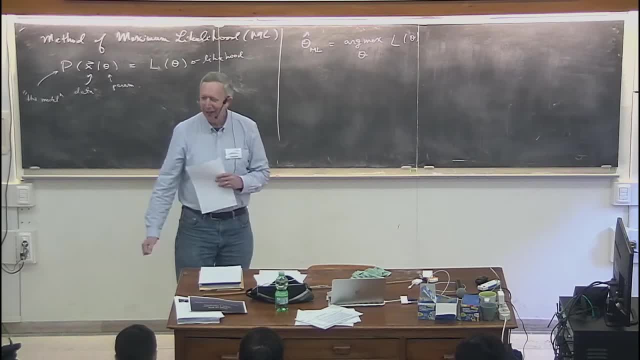 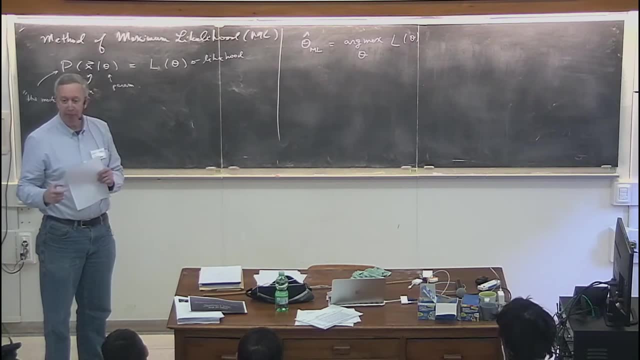 the right answer, but that's just my definition of the maximum likelihood estimator and we need to estimate, we need to investigate the proper properties of the ML estimators with respect to bias, variance and so forth, And very often we will find that maximum likelihood estimators have a non-zero bias. 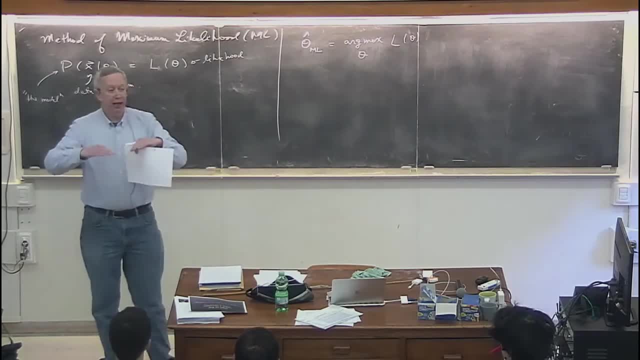 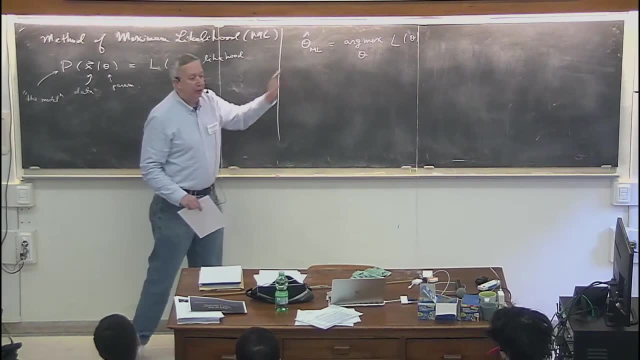 For any estimator that you write down, there will be a certain trade-off between the variance and the bias and you might, in certain circumstances, come to the conclusion that the maximum likelihood estimator doesn't give you the desired trade-off between those two, those two quantities. 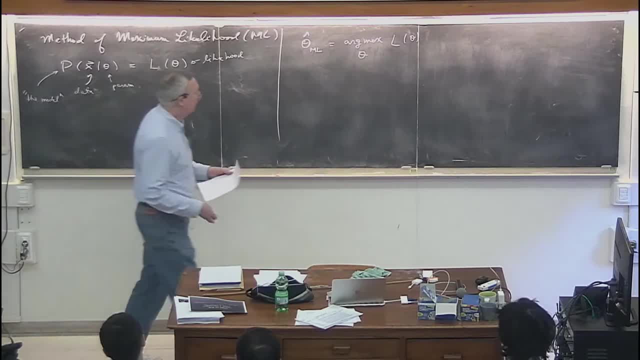 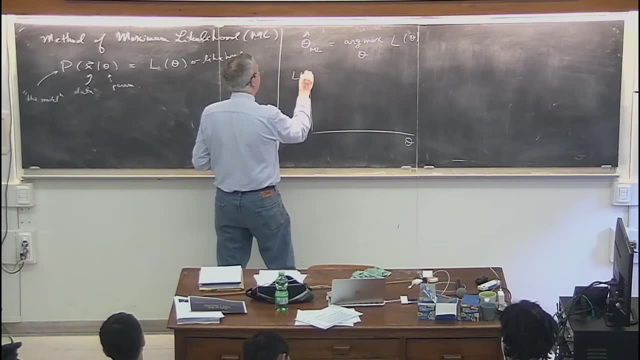 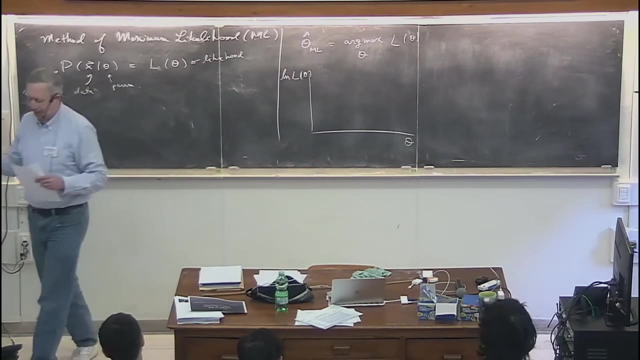 And hopefully get time to go into that later. So here's the basic idea is that I want to find now the value of theta that maximizes the likelihood, but now it's equivalent to find the value of the parameter that maximizes the log of the likelihood, because logarithm, of course, is a monotonic function. 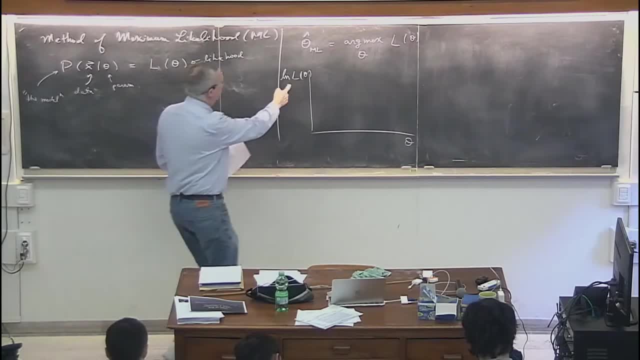 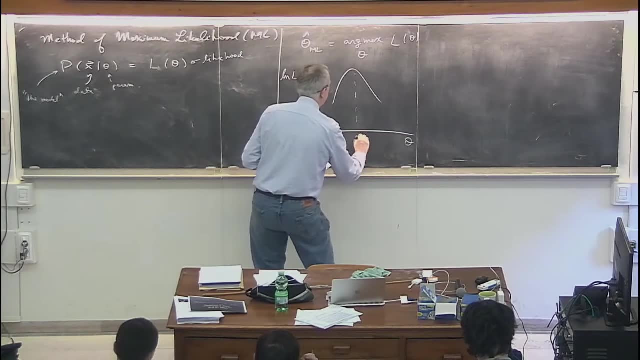 And so this is equivalent and it's usually much easier to work with the log, And so you have something that comes up and goes down and so you would say: there we are, Maximum likelihood estimator. In general, this thing could have wobbles. 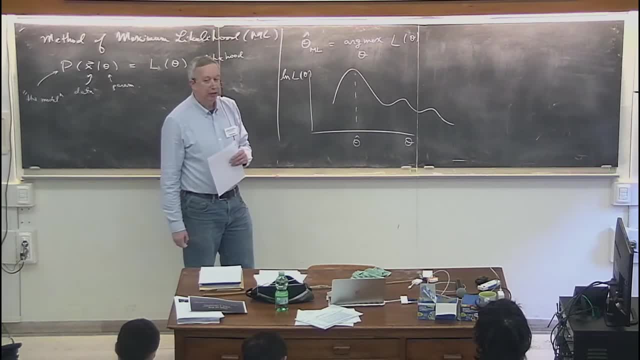 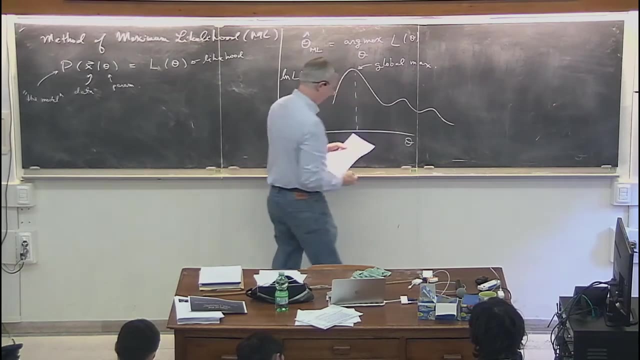 There could be multiple local maxima, in which case I mean by the maximum likelihood estimator to take the global maximum, global max. All right, So let's do a quick example. I think I just have time for that. It's going to take the full board. 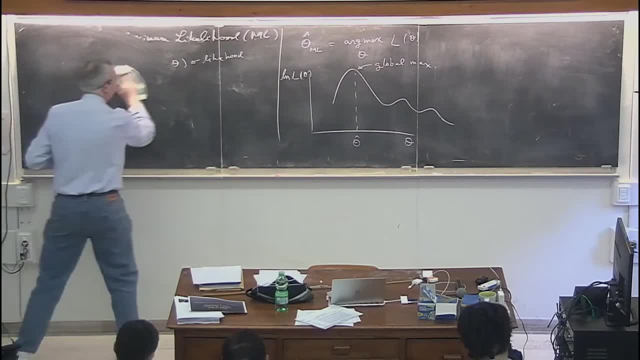 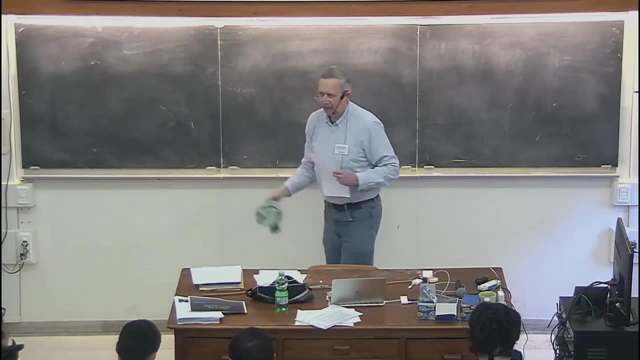 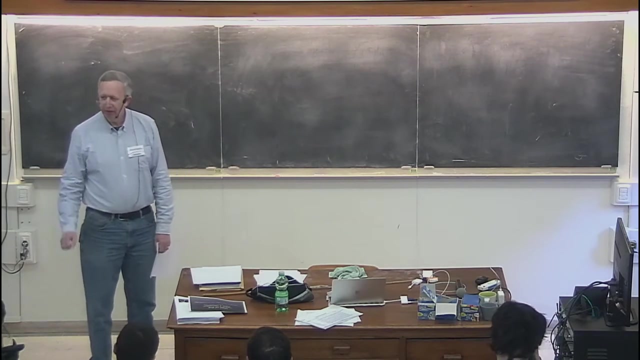 So I'm going to Let me see here That can be very difficult, Yeah. No, There can be cases where numerically that might be arbitrarily difficult or impossible, But in most cases of practical interest that's not the biggest headache. 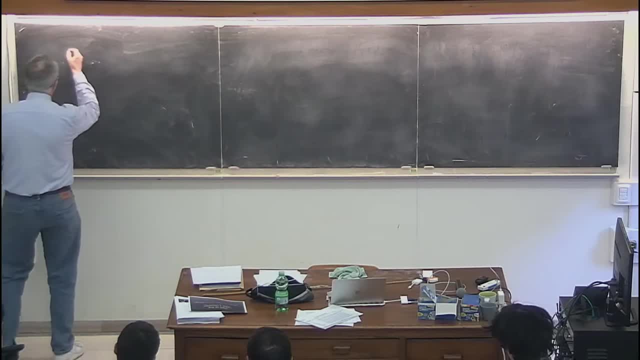 Let's suppose that I have a PDF, So here's an example. Okay, Let me suppose that the PDF is a function of a random variable that I'll call t, and it has as a parameter tau and it is an exponential distribution. 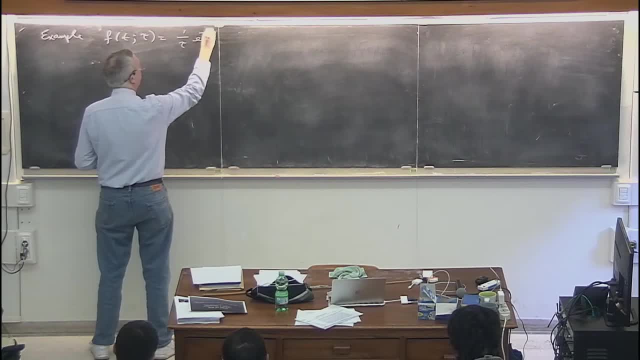 And so that follows the standard convention, that I'll say that t represents maybe a decay time and I'll use the corresponding Greek letter to correspond to the mean decay time. Okay, So in this particular example, the expectation value of t is equal to tau. 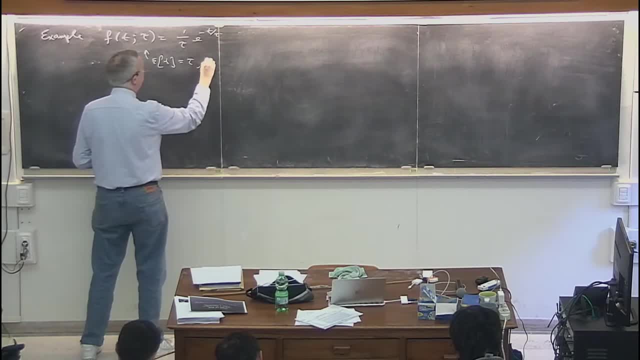 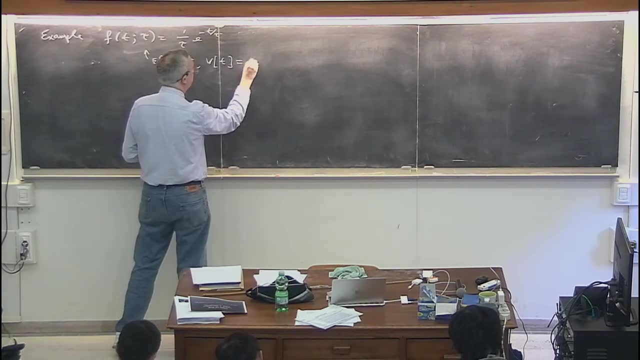 Right, And the variance of t. you can work out from the formulas that I had on the board previously that the variance of an exponential distribution is equal to the square of its mean. So that's the model. And now suppose that I have data. 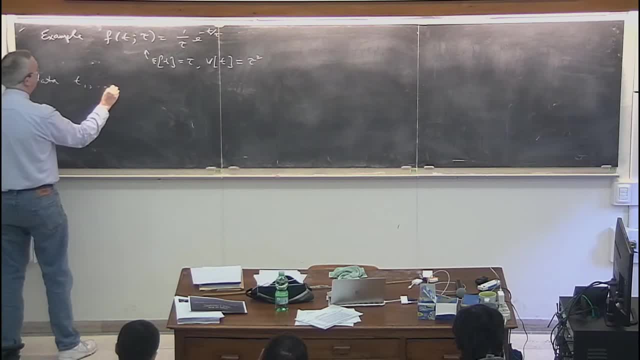 So I've observed, say, 10 n particle decays and for each one I measure the proper decay time, And let me suppose that they are all independent. Okay, Okay, Okay, Okay. If I've observed n independent particle decays, then that would be the case. 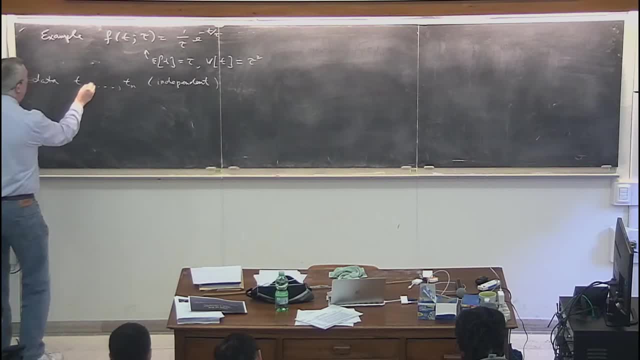 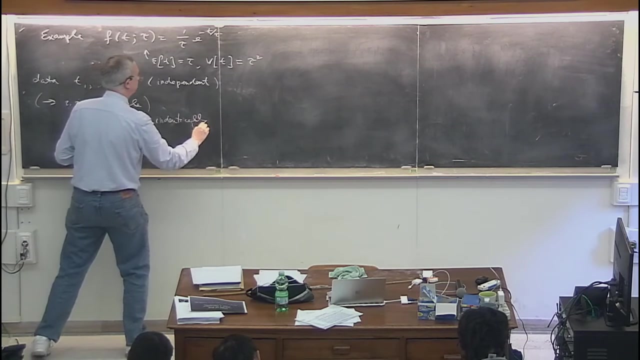 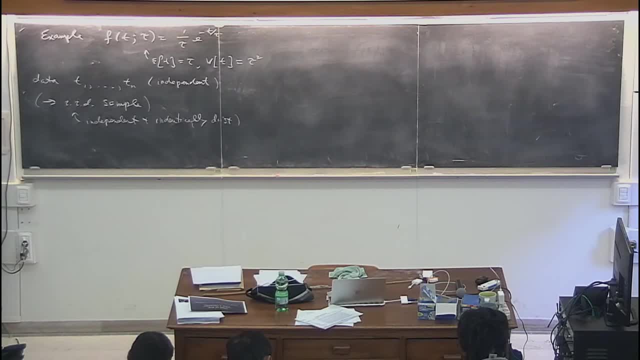 Okay, Okay, Okay, Okay, Okay, Okay, Okay. So if we have an IID sample, what is then the joint PDF for this entire set of data? So, remember, I said the definition of independent events is the two events were independent if 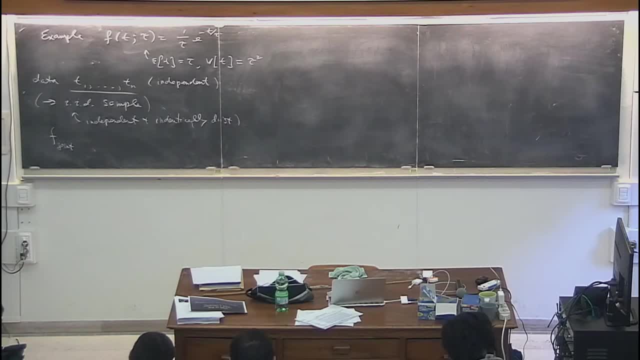 the probability for two of them was equal to the product of the corresponding probabilities. And so that's what we would have here. We would say the joint probability for the whole sample would just equal to t. Okay, Okay, would just be the product of f of t. sub i tau. 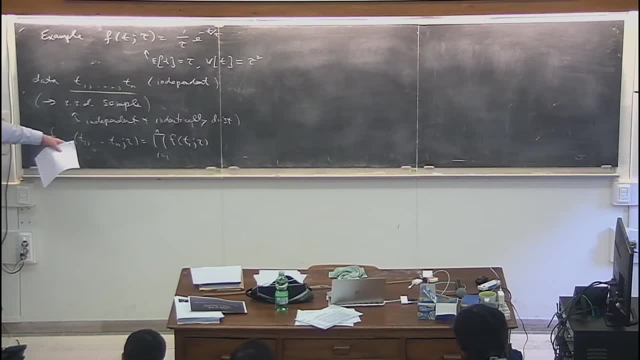 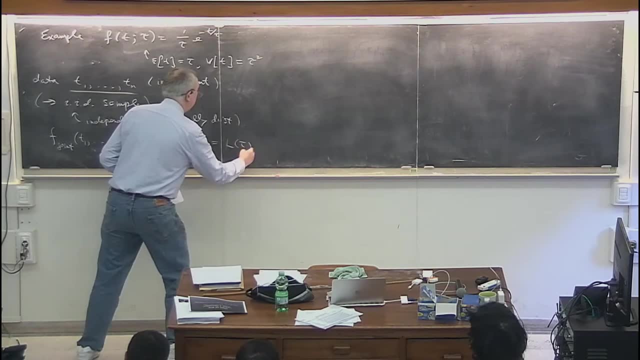 And then, if I take this joint probability and view it only as a function of the parameter tau, I would say that this is equal to my likelihood, And so now it is a simple matter of finding the value of tau that maximizes the likelihood. 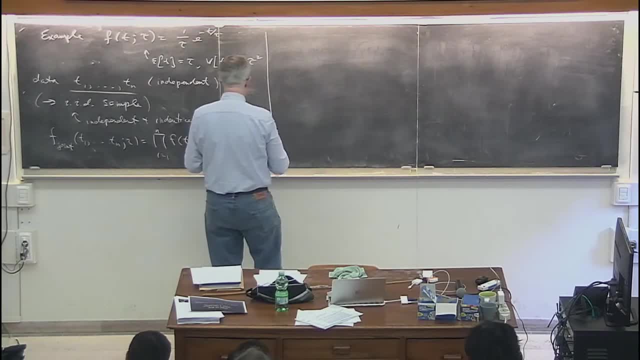 And, as I mentioned earlier, it's easier to work with the log of the likelihood and so that converts the product into a sum, which is very handy, And it converts any exponential factors here into it gets rid of the exponential. So this is just going to be log one over tau. 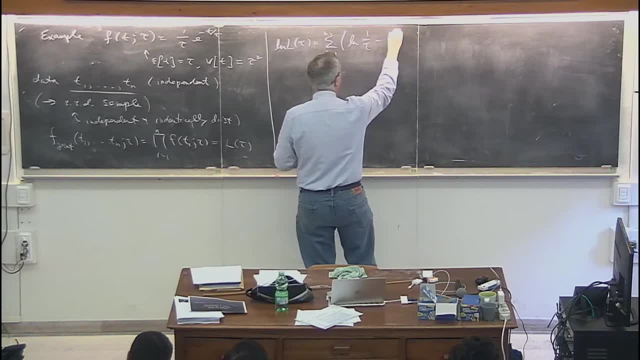 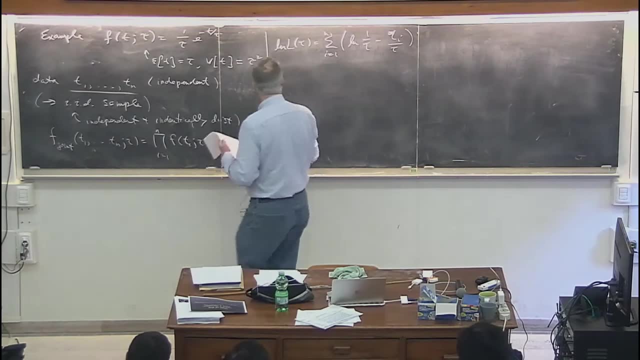 minus t, sub i over tau. Voila, All right. so now I simply have to differentiate this guy with respect to tau, And so this is going to be the sum. So that gives me minus one over tau right, Plus t i over tau, squared. 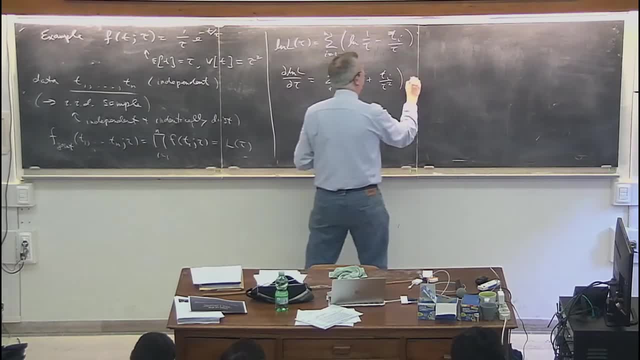 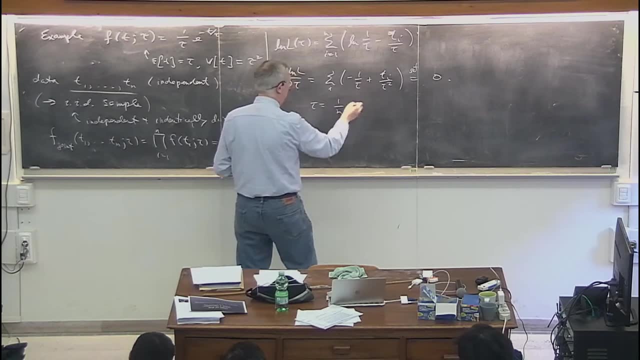 And then I just set that equal to zero and I solve for tau And that gives me- I skipped the math, but it's easy- That just gives me the arithmetic average of the t sub i, which is kind of interesting. So there, I've constructed my function. 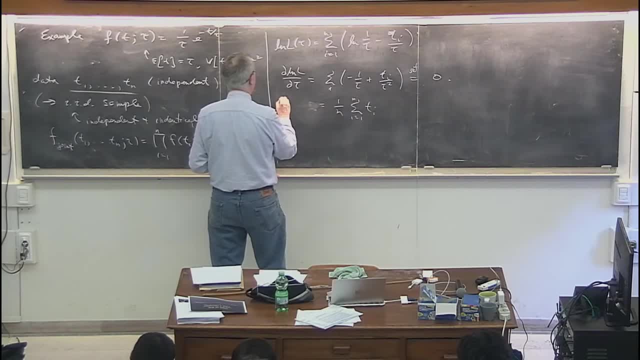 I said tau. I'm going to write it with a hat because that's my estimate And that is a function of the data. It's a function of t1 through tn. I usually will suppress that part of the notation, but keep in mind that the estimator 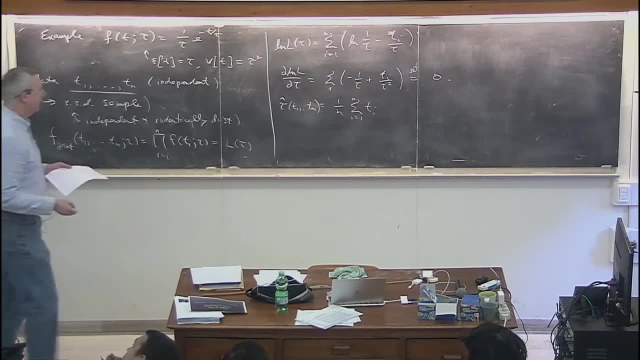 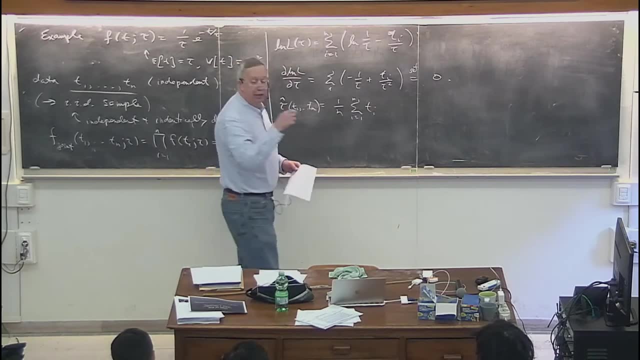 is always a function of the data. Okay, good. So if you look in the notes from the course page, there's like a little Monte Carlo thing where I took a Monte Carlo generator and I generated, say, 50 values of t. 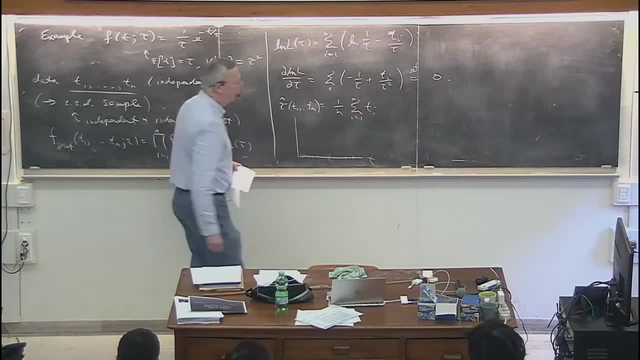 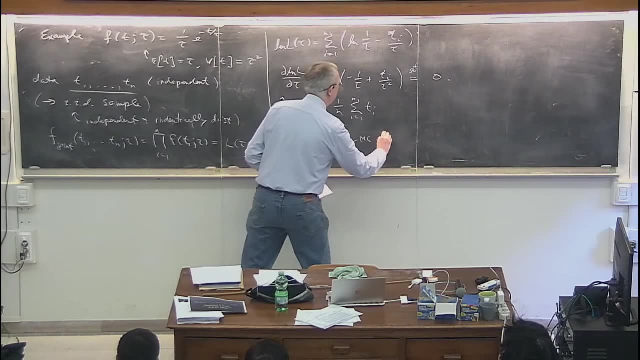 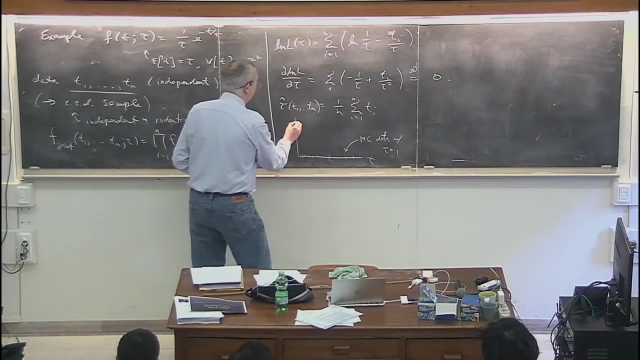 According to an exponential distribution that used tau equals one. So this is MC data, with tau equals one, And then you generate these t sub i values And then if you were to plot the result, the result would correspond to some other value of tau. 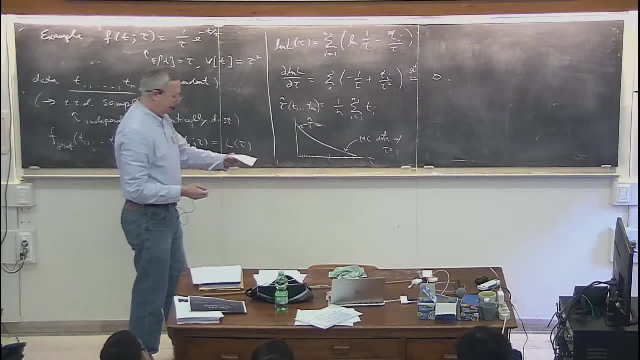 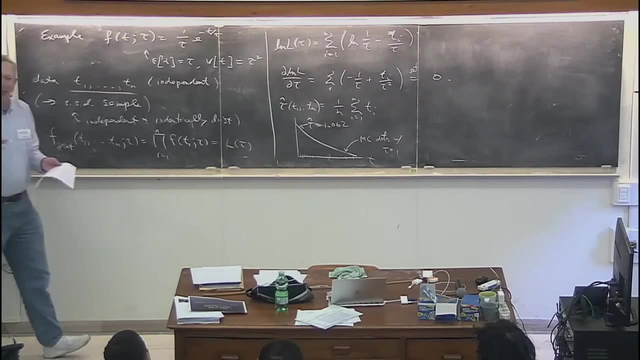 And did I write it down? Yes, It obviously will be some other value. It turned out to be 1.06.. Because of the statistical fluctuations in the data, Now we want to check the properties of this estimator. We want to check: is it biased? 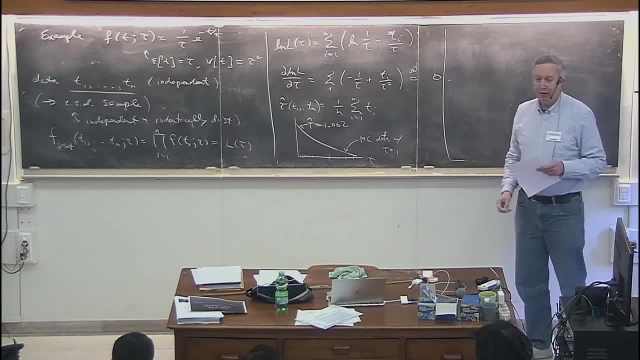 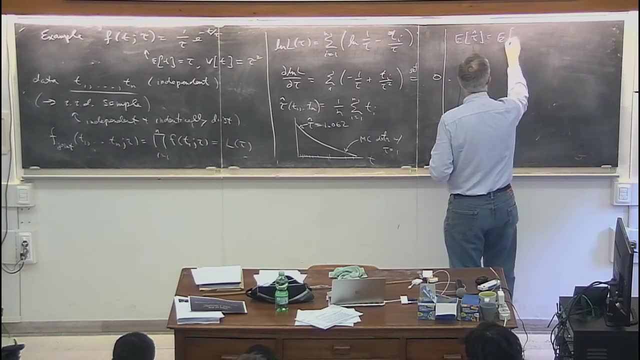 And what is its variance. So let's just work out really quickly the expectation value of tau hat, And so that's the expectation value of this, And one of the things that's obvious from the definition of the expectation value is that it's a linear. 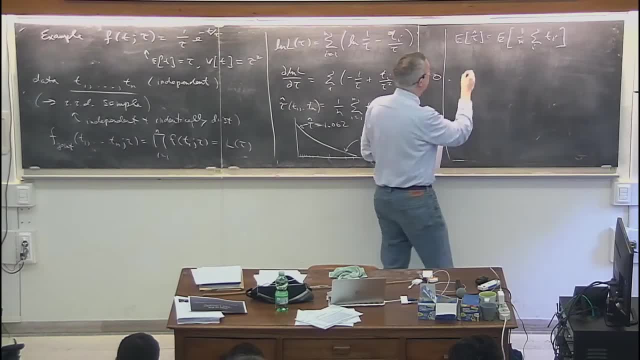 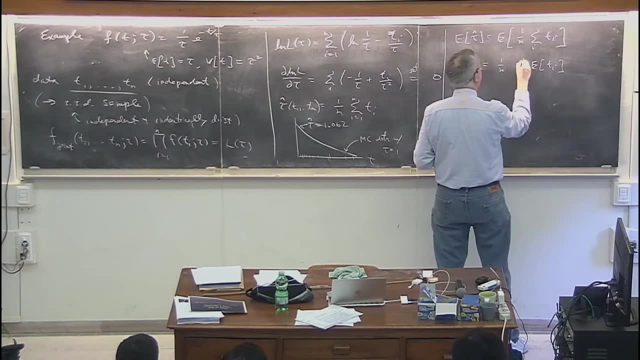 It's a linear. It's a linear operator. So this is just one over n times the sum of the expectation values. There's n terms in the sum And each of those guys is equal to tau, And so it's one over n times n times tau. 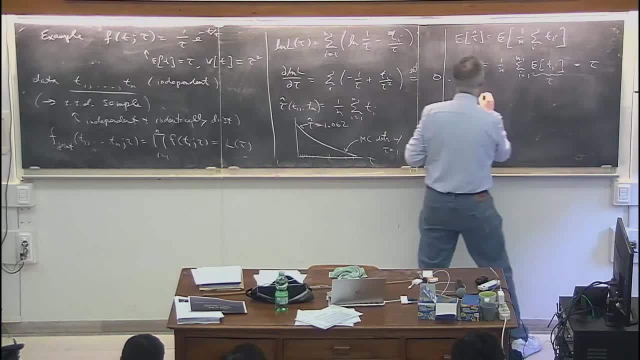 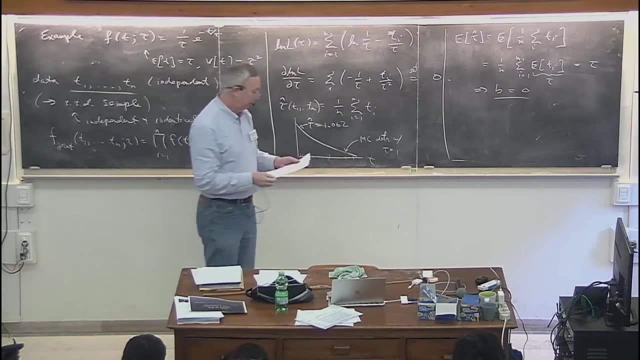 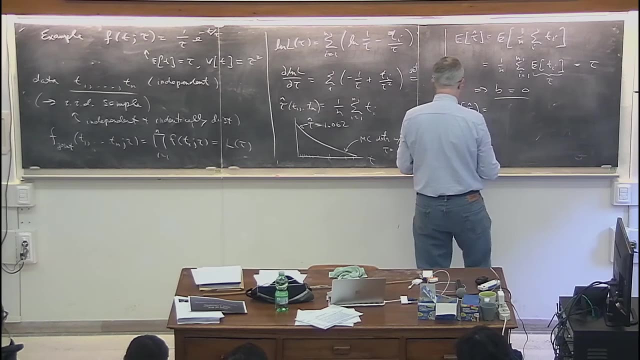 It's tau, And so therefore we come to the conclusion that this bias is identically zero for all values of tau. So that's a special example. So we can now work out also the variance of tau hat, And this is equal to the variance. 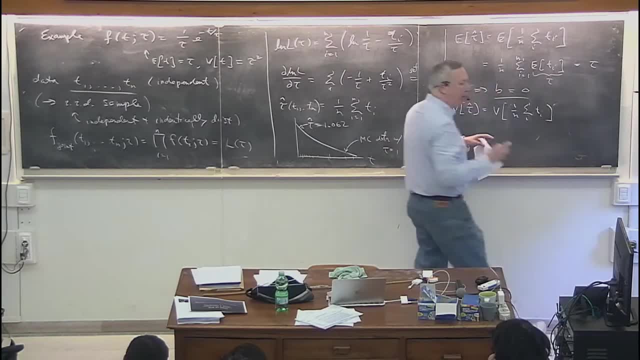 Now again, if you go back to look at the definition of the variance, you'll see it's not a linear operator because it's the expectation value of a product. So when you pull out this constant here it actually gets squared. And then if the ti's are all independent, 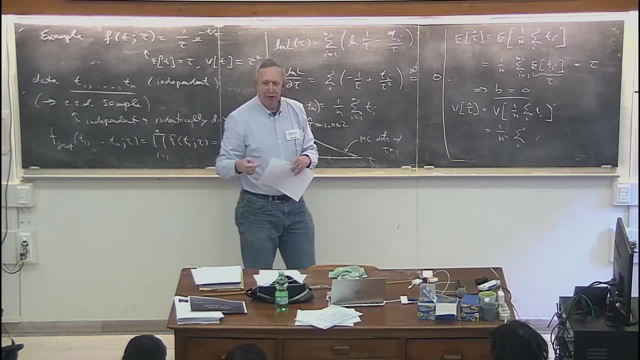 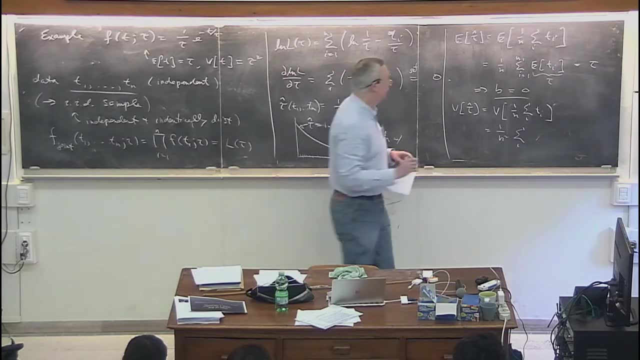 that what? one of the consequences of that is that the variance of the sum is the sum of variances. If the ti's are independent, that's true. So it's just going to be the variance of the ti's. That's tau squared. 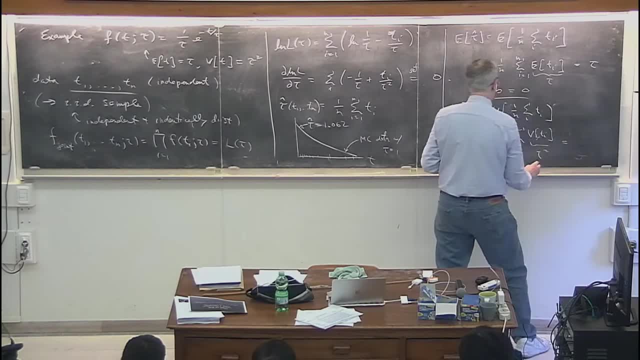 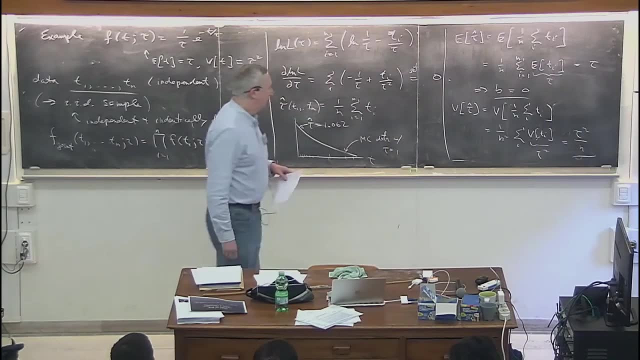 And so we get. let's see, there's n terms in the sum. So this is going to give me tau squared over n Right? Or I could say that the standard deviation of tau hat, that's just the square root of the variance, is tau over. 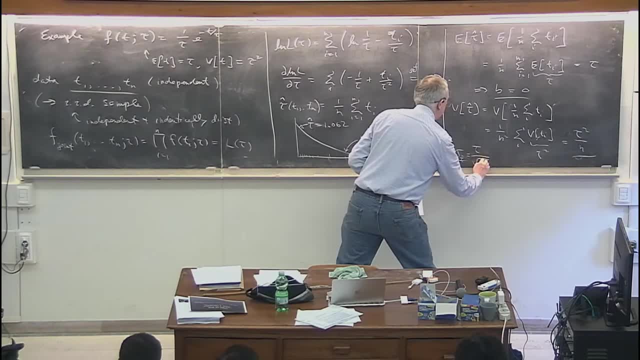 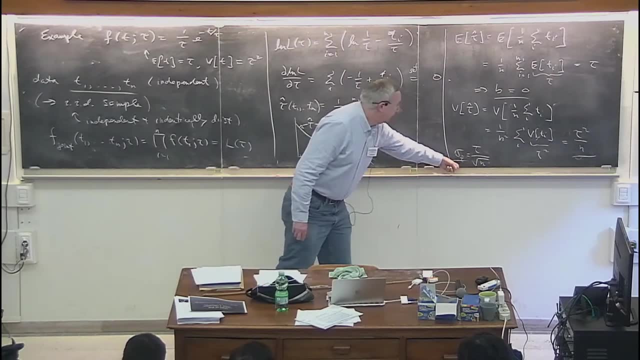 the square root of n. That gives you the well-known property of the statistical errors. So that's the number that you would report as the statistical error. That's the statistical error of your measurement And you see that that decreases inversely as the square root of the number of measurements. 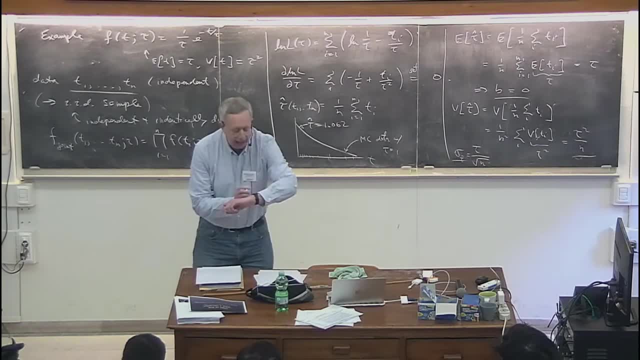 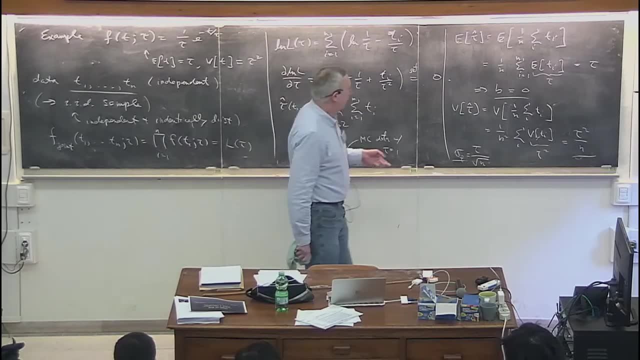 Now I'm going to do this very quickly because I want to show you another way of getting the variance in problems where it's not so easy. So in this particular case, in three lines of mathematics we could work out the bias and the variance. 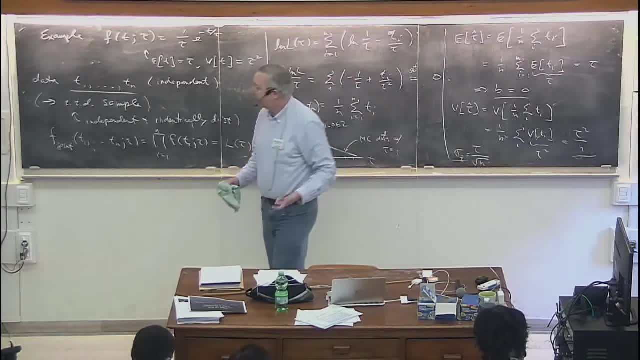 But in general, you're not going to be able to do it in closed form, And so what I want to show is a shortcut. It's an approximate. It's an approximate shortcut which will allow you to compute the variance of an estimator in general. 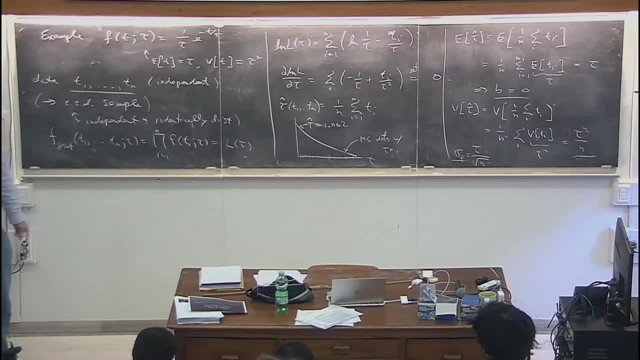 Yeah, Yeah. no, it's not completely obvious, But actually let's do that in the discussion session. That is a good question, But if you look back at the definition of the variance and you see what would happen if I multiplied, 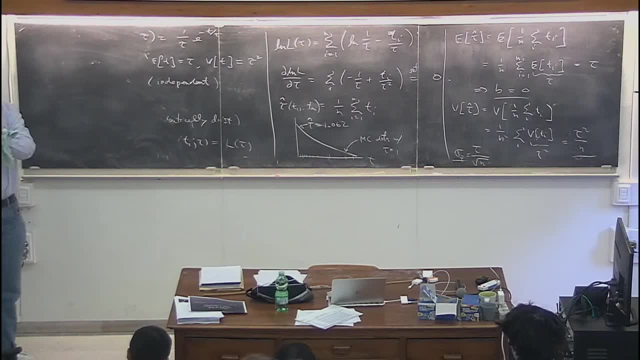 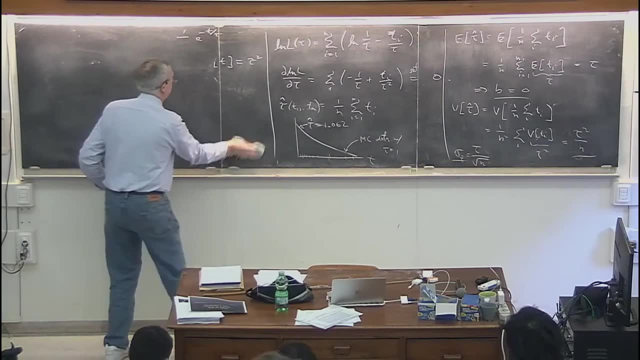 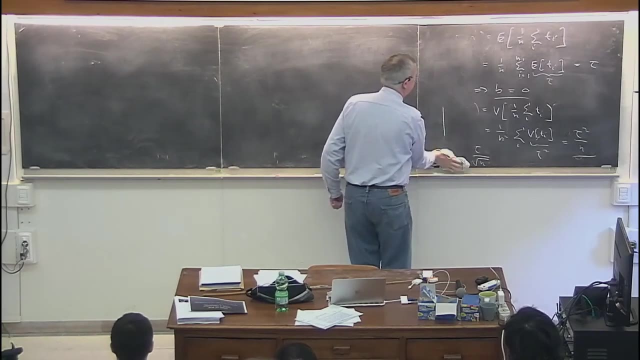 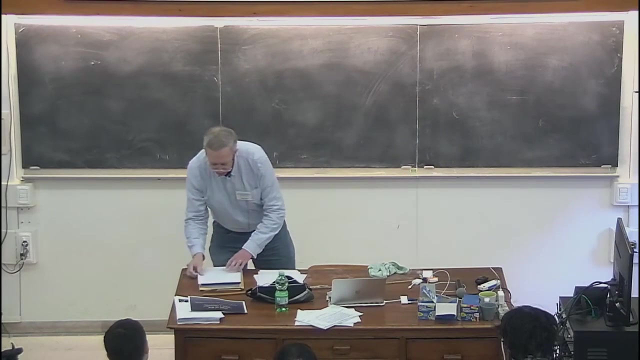 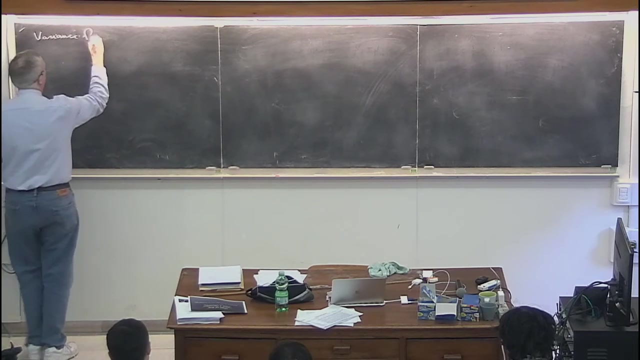 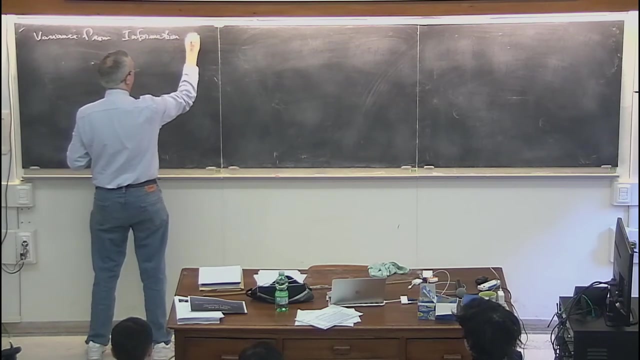 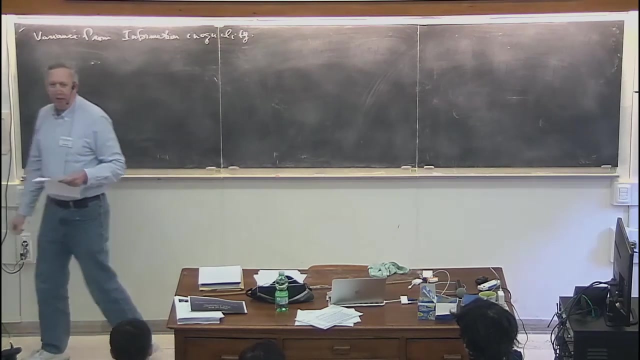 with a constant, it's obvious that it gets squared, But let's talk about that in the discussion session. So here is a way to estimate the variance from something called the information inequality. It's sometimes called the RCF inequality or the Rao-Kramer-Fresche inequality. 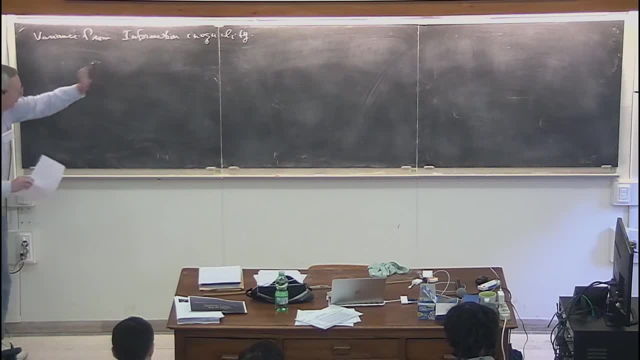 So let's just call it the information inequality, And what that says is that the variance of any estimator- not only estimators- from the method of maximum likelihood. but however I've constructed my function of the data, however I've constructed my estimator. 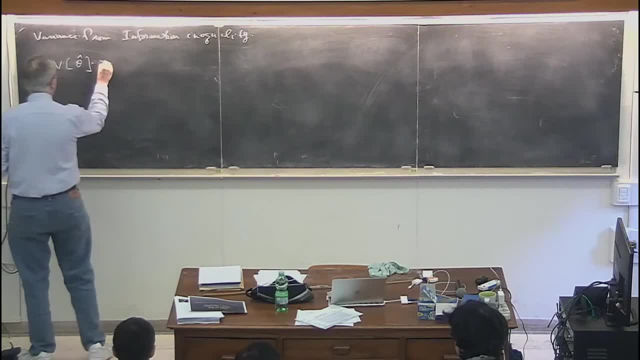 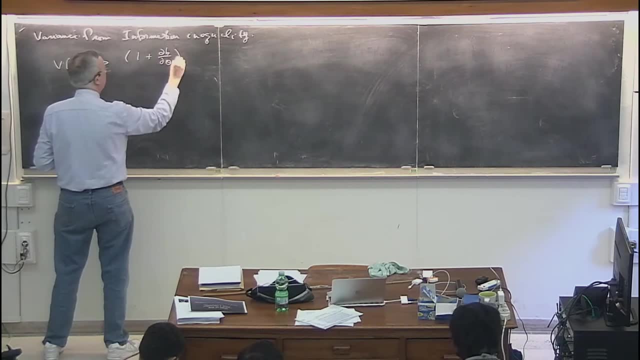 its variance has to be greater than or equal to this quantity, which I'll write down here. put a minus sign there. I'm writing down the version of the inequality for a single parameter. We can generalize this later to the case of multiple parameters. 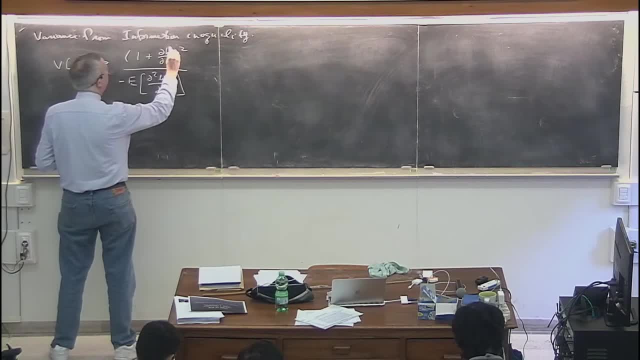 So that quantity, there is the bias as I've defined it previously, And here I've got the likelihood function. even though I might not be talking about the maximum likelihood estimator, I can always talk about the likelihood. So that's an inequality. 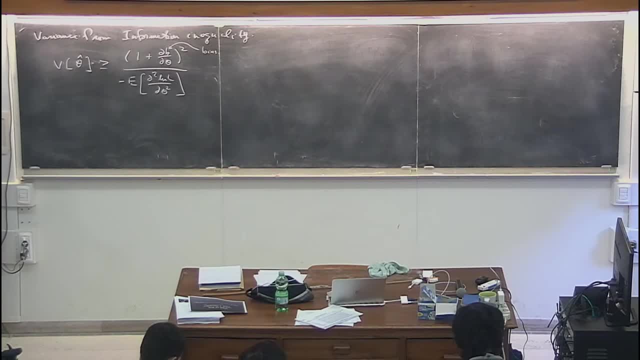 One of the homework problems that I stuck on the first problem sheet is to prove this, And actually I just thought of this yesterday evening. It's been years since I've gone through the proof myself, but the way I've structured the problem kind of walks you through it. 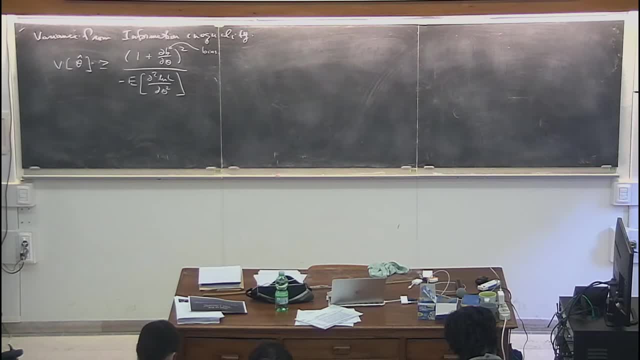 So maybe we can go through that together this afternoon. So I should say that this expectation value here means with respect to the data. so the expectation value of this guy means minus integral of the second derivative of log L, So this expectation value is over the data space. 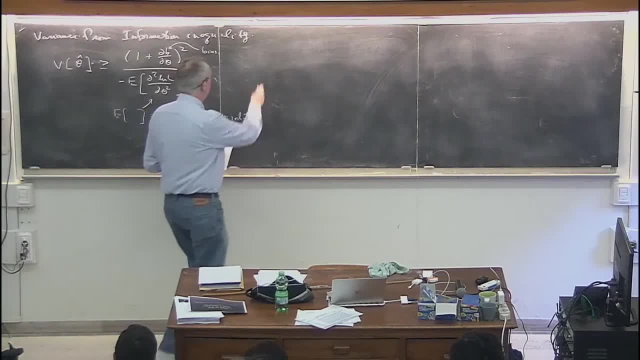 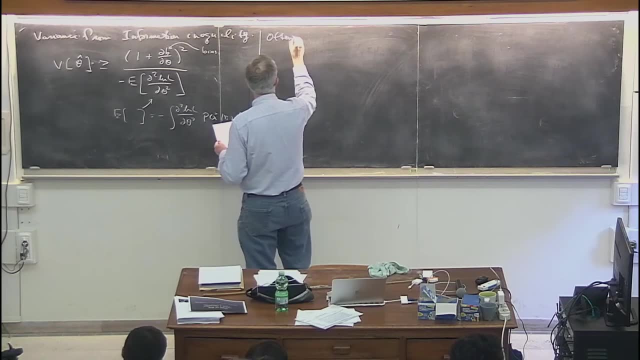 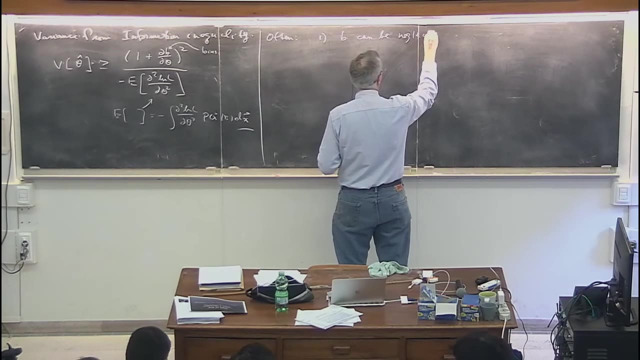 Now often I can make the following two statements. Often one, the bias can be neglected. I showed you that the statistical error goes as one over root n. Very often the bias, if it's nonzero, drops off as one over n. 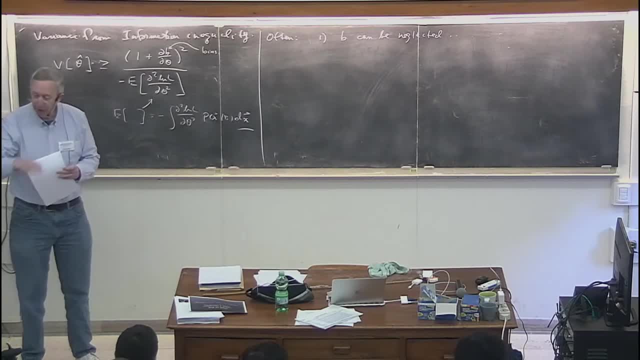 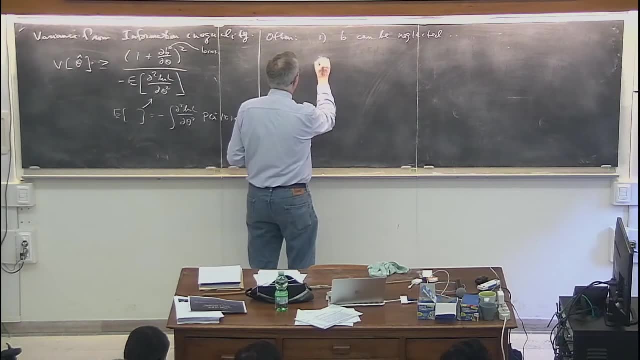 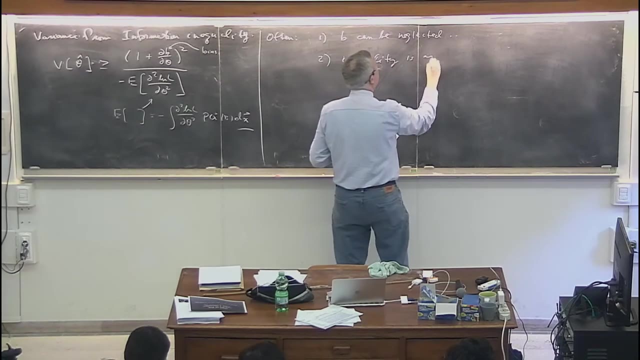 So it drops off much faster. So in many problems of practical interest the bias can be neglected. Or maybe it's identically zero, And then, second, the inequality is an approximate equality, And so then what I can do is I can say: 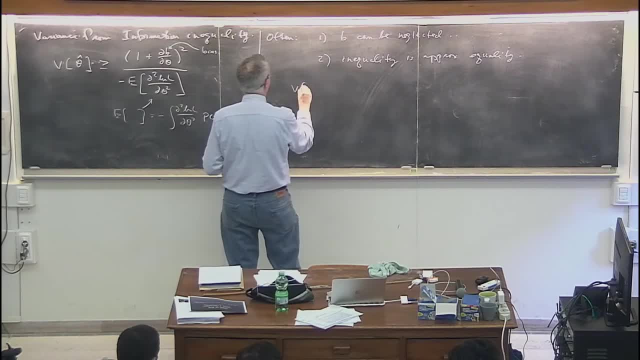 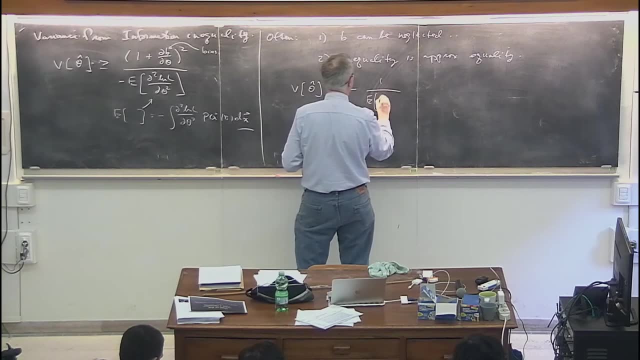 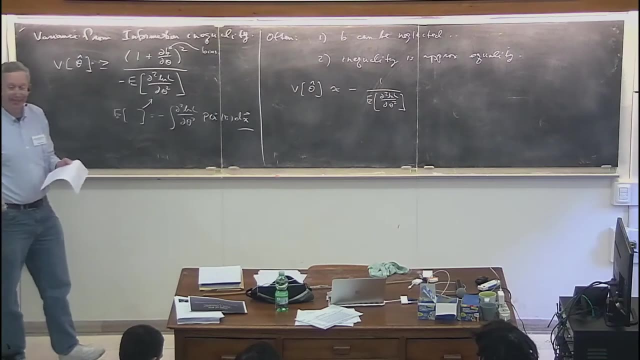 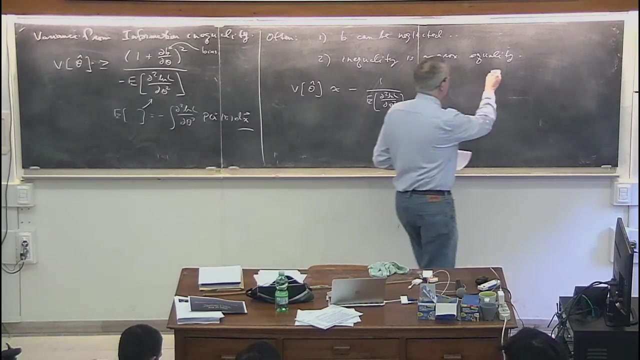 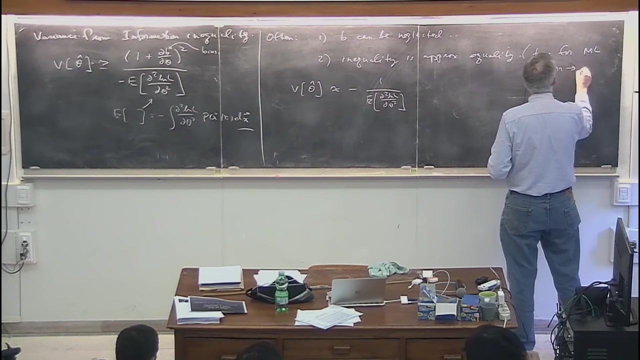 that the variance of my estimator is approximately equal to minus one over the expectation value of the second derivative of log L. All right, so that's the basis of this approach. This second thing I should say will be true for maximum likelihood in the limit where the data sample is very large. 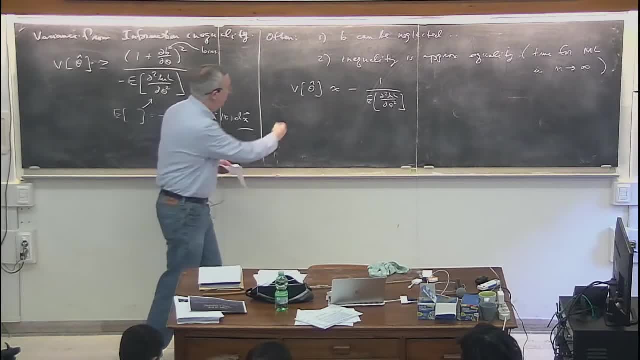 Okay, so then we get this expression here. Now keep in mind that the bias and the variance of estimators are functions of the true and unknown parameters, So strictly speaking, this would be some function of theta. But I want a number. 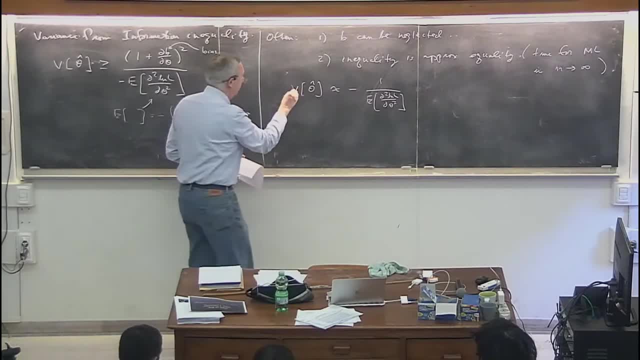 What I want is an estimate of the variance of the estimate of the parameter. Notice two occurrences of the word estimate in that phrase. All right, what I want is the estimate of the variance of the estimate of the parameter. So what you can very often do is simply take. 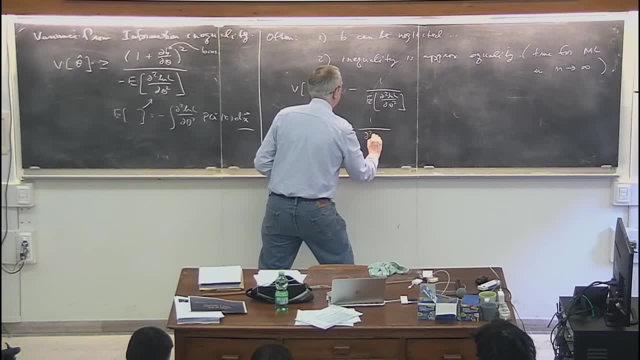 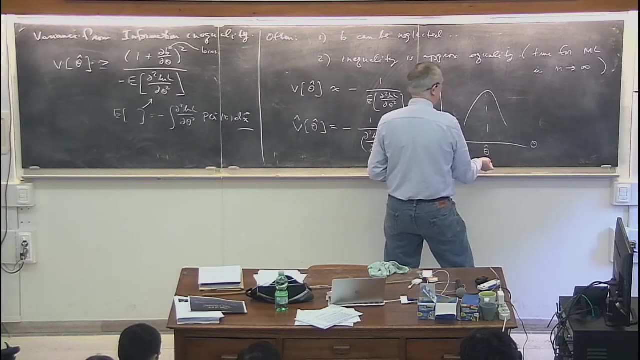 the second derivative of the log likelihood function evaluated at the estimator. So if you look at log L versus theta, it's someplace here where the estimate is, And what you're looking at here is essentially the curvature of the log likelihood function. That's what the second derivative gives. 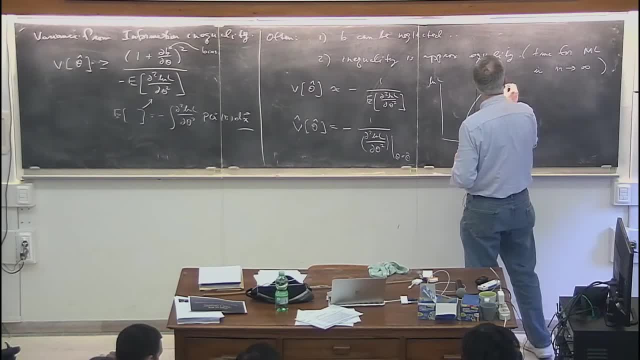 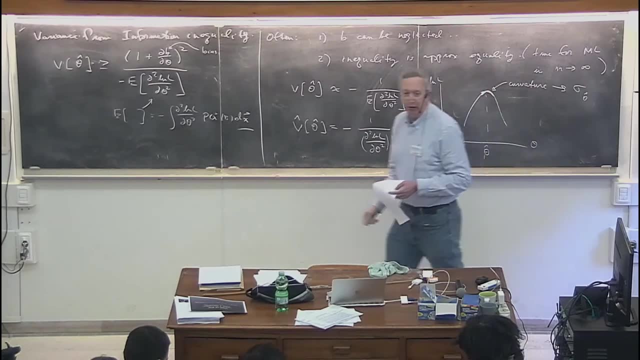 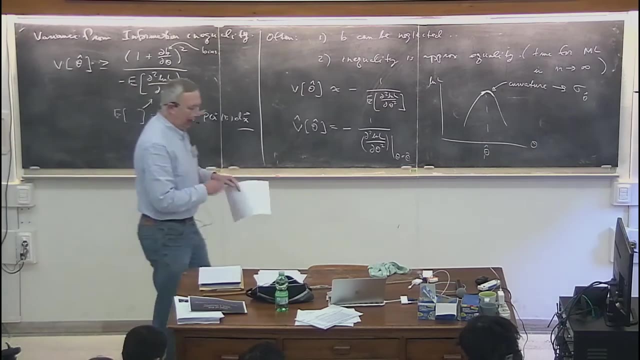 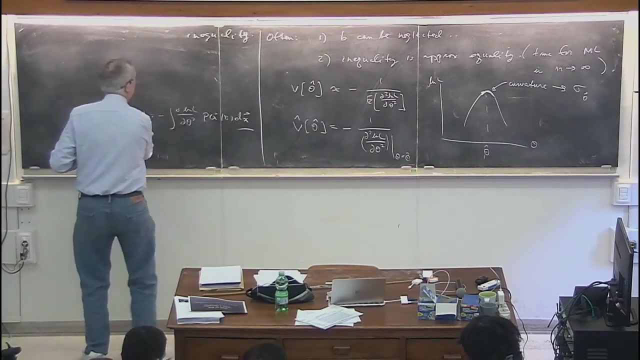 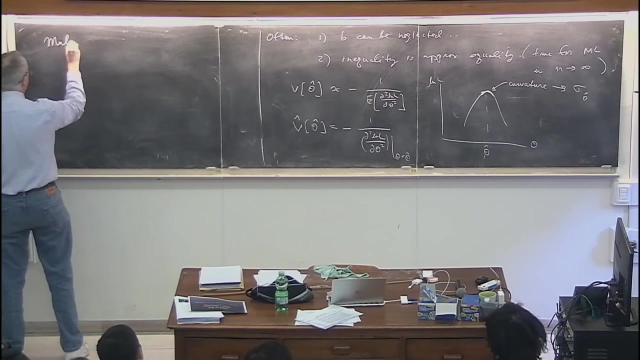 So the curvature here gives you the standard deviation of the estimator. So the standard deviation, of course, is always just the square root of the variance. I just want to mention really quickly the multidimensional generalization of that. So if I have a problem that has more than one parameter, 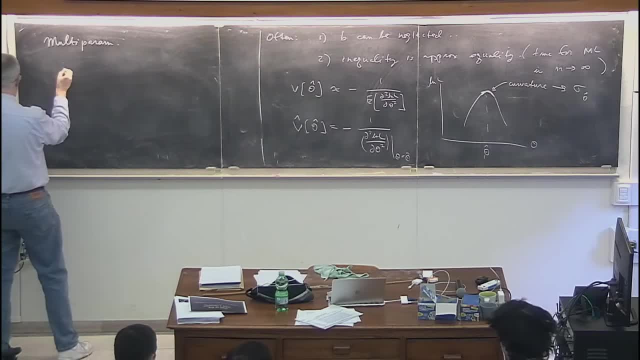 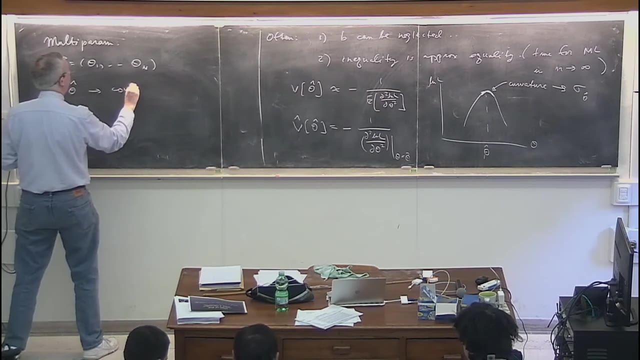 we would say that first. so let me say that suppose I have a vector of parameters, theta one through theta n, And let me suppose that I have constructed estimators And I have the covariance of each pair of estimators. So the covariance of theta i hat and theta j hat. 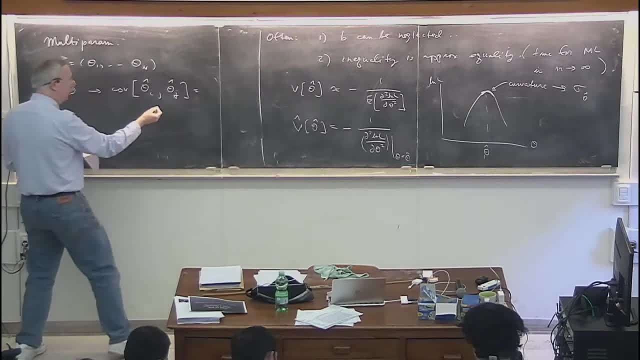 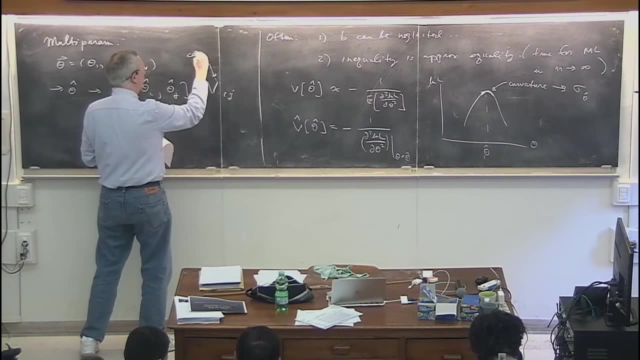 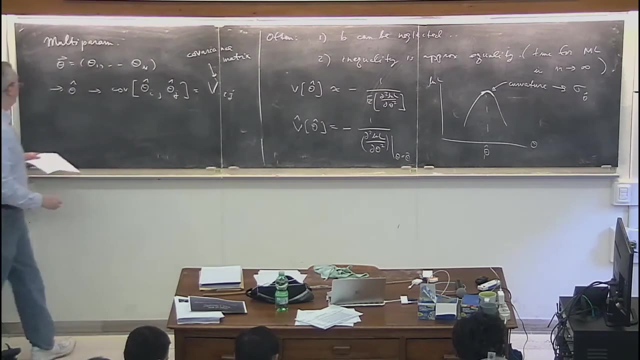 And I have that for all pairs, And so therefore I can put that into a matrix. I'll call it vij, And so that's obviously what I call the covariance matrix. So let me suppose that I have constructed the estimators And I have the, and what I want to do is to 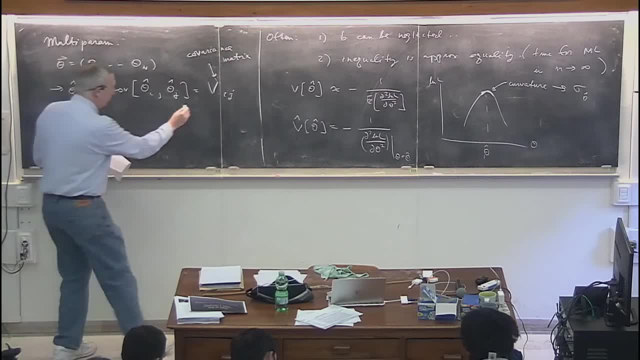 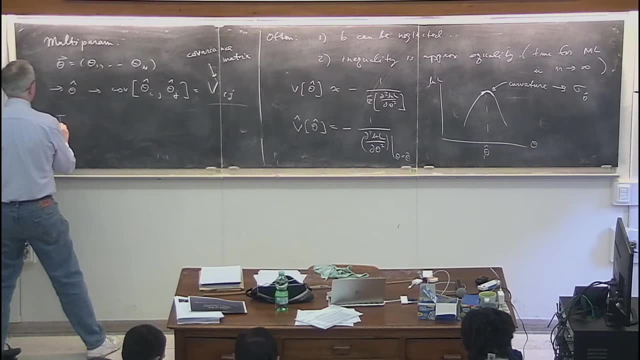 try to obtain an estimate of that matrix of covariances. So what you do is the following: is I define the matrix capital Iij as the negative expectation value of the second derivative of the log likelihood function with respect to parameters i and j? 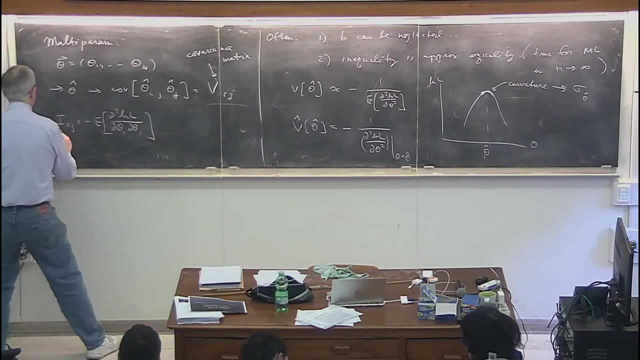 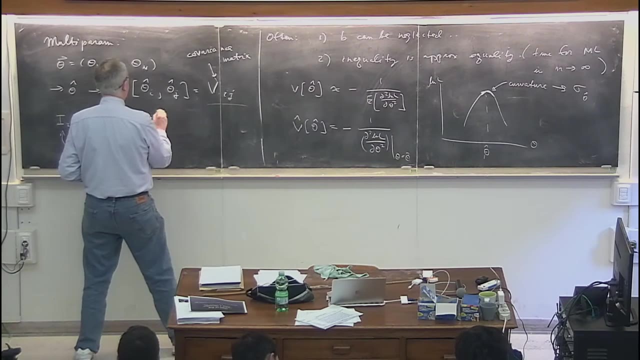 And that is what's called the Fisher information matrix Matrix, And this multi-parameter version of the information inequality so says the following- Sorry, I'm running out of space. So the information inequality becomes now the statement that the difference between the matrix v 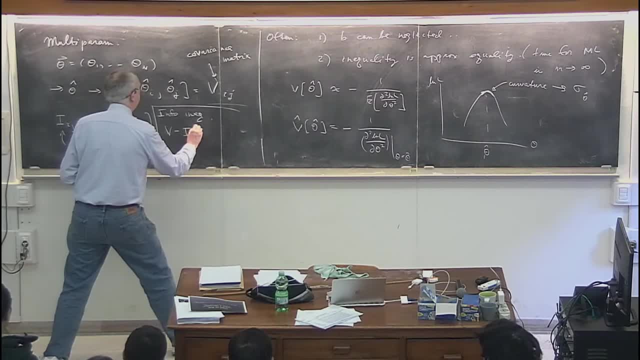 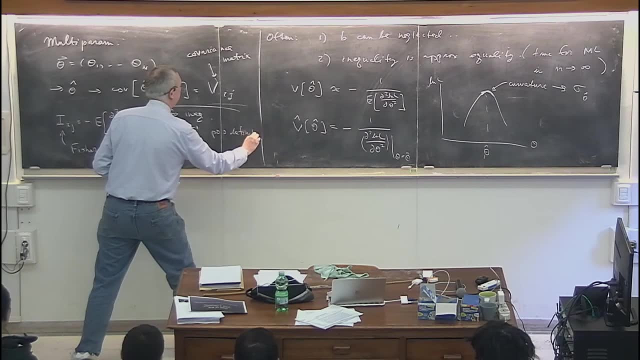 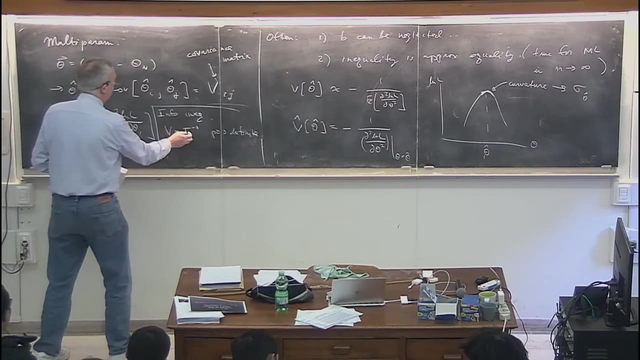 and the inverse of the matrix i. that difference is a positive, definite matrix. In particular, that means that the diagonal values are positive, And so you could use that to get a corresponding lower bound on the variances. But what's done in this multi-parameter approach? 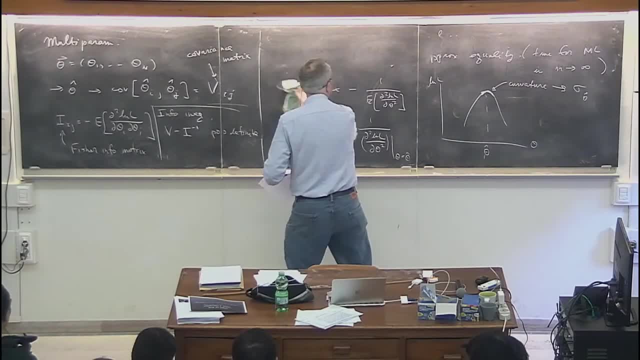 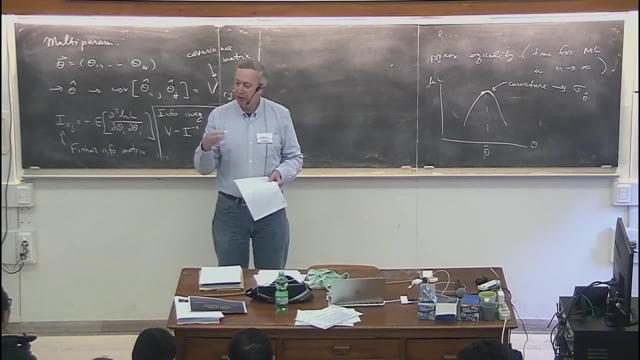 more frequently is analogous to what I just said before. That is to say, if you assume that the inequality is an approximate equality and if we neglect the biases, what we do is we say we approximate this covariance matrix. That's the thing we really want to get. 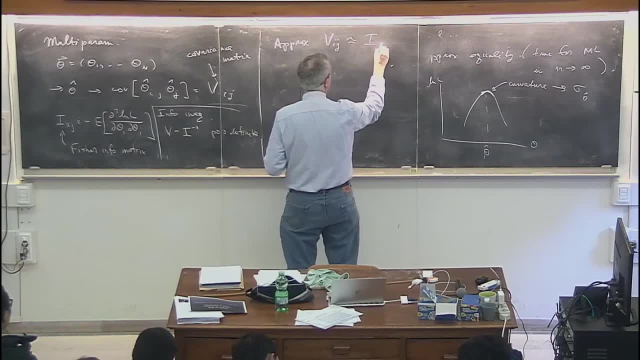 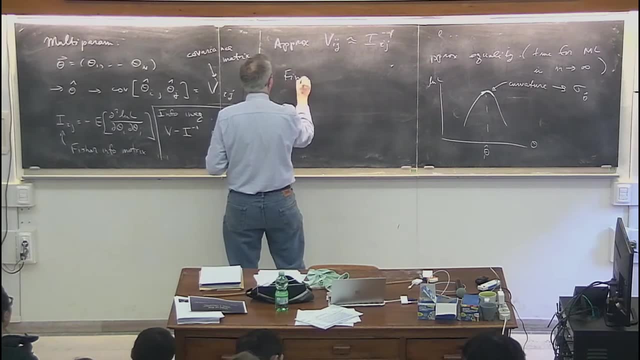 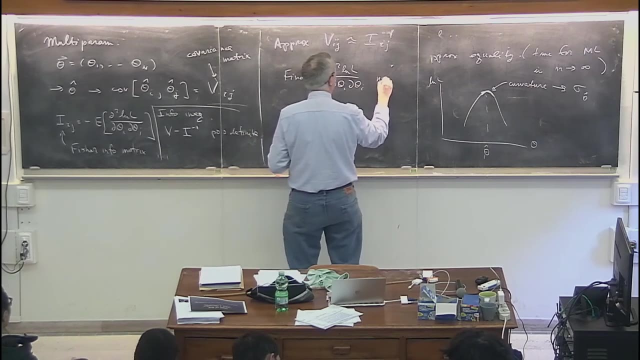 We say that it's just approximately equal to the inverse Of this Fisher information matrix. And so what you do is that you find this matrix of second derivatives numerically at theta equals theta hat and then invert to get the covariance matrix. So some of you have probably played with software. 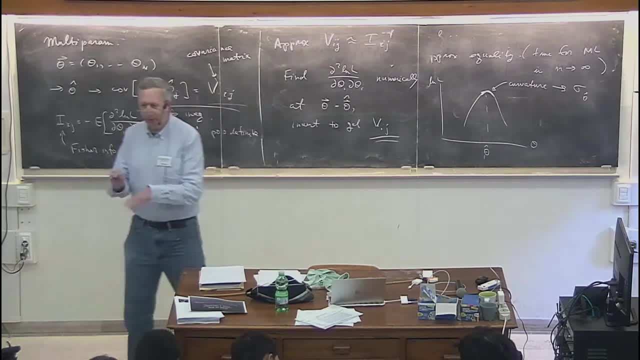 for fitting program for fitting data where you have more than one parameter, Like in Python. it's called curve, fit or whatever, And you execute the command to do the fit. It prints the fitted values and it prints a covariance matrix. And you might have wondered: what is it doing? 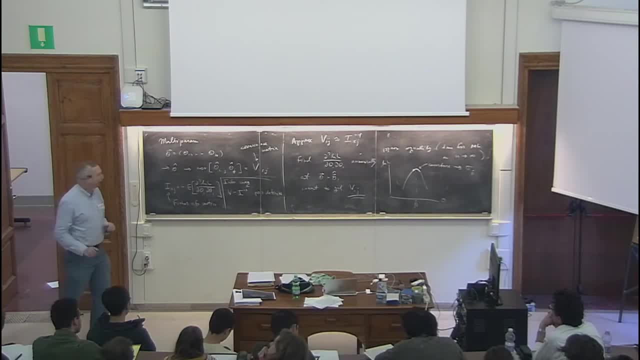 behind the scenes And what it's doing is this: It's numerically computing the matrix of second derivatives with finite differences, Inverting it, Making the various assumptions that I said, but not telling you Alright. So it's neglecting the bias. 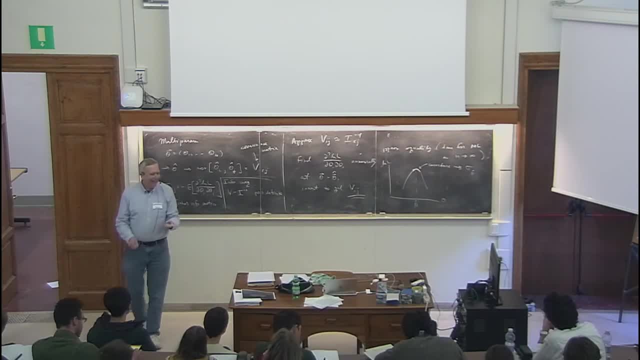 It's approximating the inequality as an equality And it's spitting out this matrix of numbers as your covariance matrix. So we'll have some practice with that later this afternoon And I propose that I stop now. So there are questions. 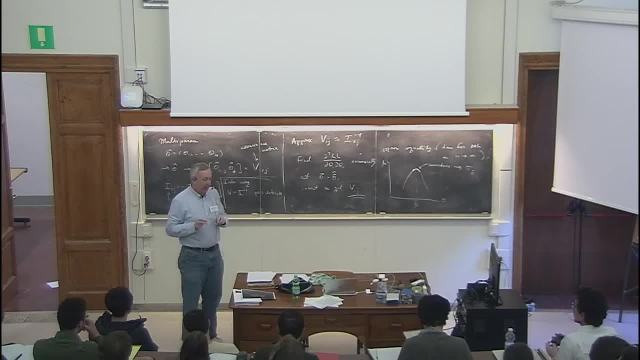 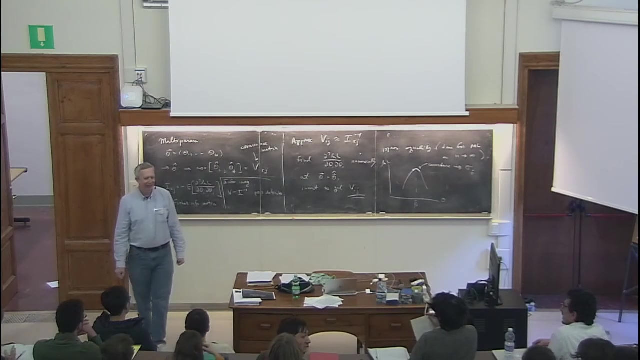 It's not too hard in the homework problem you were going to do this afternoon, But in general, that's exactly correct. So Well, No, no, You invert the matrix numerically as well. Inverting the matrix means pushing a button. 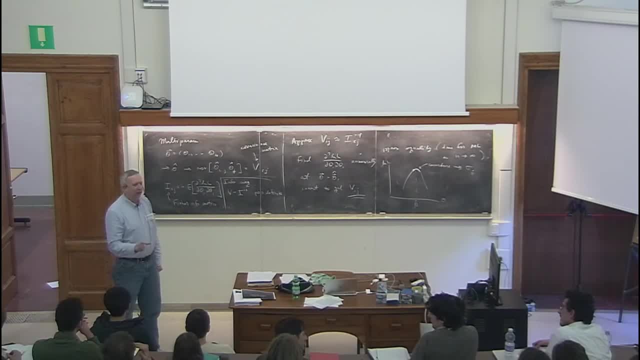 So there are certainly problems where we can work out the covariance matrix in closed form, Either with or without use of this information inequality, And so we'll explore some of those later in the afternoon. Yes, So Yes, By comparing its properties. 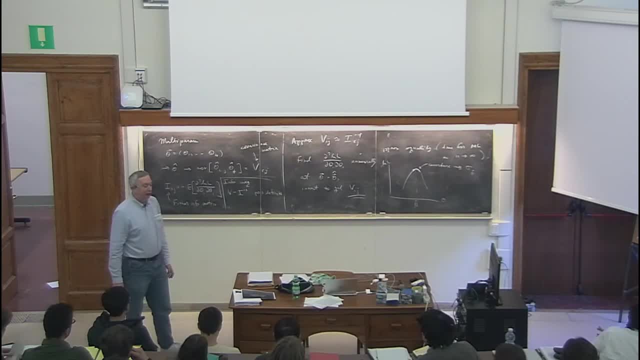 By saying, for example, the maximum likelihood estimator might have a zero bias but a certain variance, And some other estimator might have a small bias but a much smaller variance. And so then you have to ask about the trade-off. You have to say, all right. 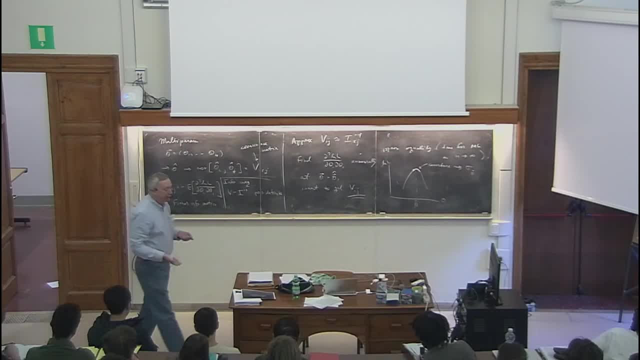 the bias. if you think about it, the bias is like a systematic error, And the square root of variance is like your statistical error, And so what you might care about is something like the quadratic sum of the two. And so if you had zero systematic error, 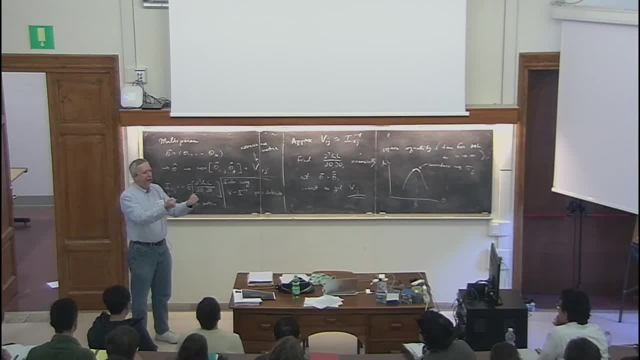 but a large statistical error. compare that to a situation where you had a small systematic error and a much smaller statistical error. So when we talk about deconvolution or unfolding problems, very often the maximum likelihood solution has a catastrophically large statistical error. 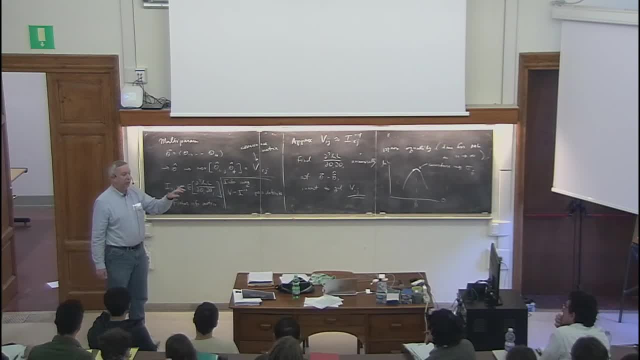 but zero bias, And what we do is we go away from the maximum likelihood solution a little bit, And what we do in that way is to introduce necessarily a small systematic error in exchange for a huge reduction in the statistical error. So that's one of the games. 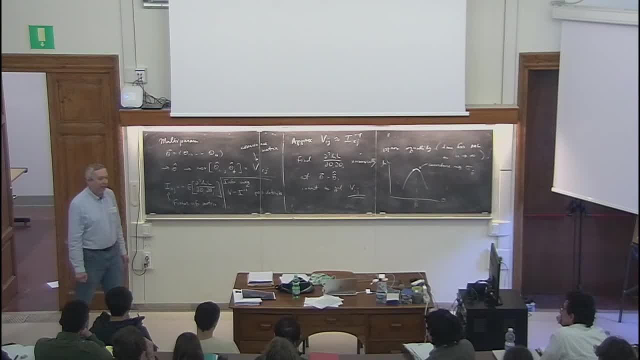 that somehow sometimes is played Okay, No, no, no. So the famous example which I didn't have time to show is if you consider the two parameters of a Gaussian, So the Gaussian has a, has a mean mu and a variance sigma squared. 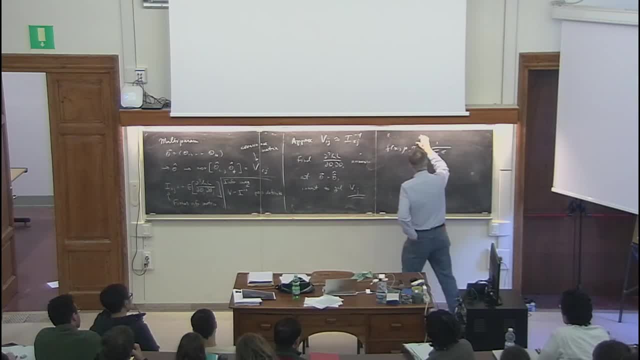 I could take the parameter to be sigma or sigma squared, It doesn't matter, Let me take it to be sigma squared, All right. So I write it that way. So what you can do is you can construct the maximum likelihood estimator for the mean. 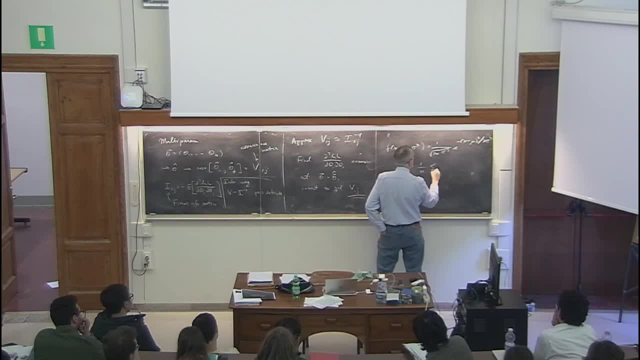 And, interestingly, that just turns out to be the arithmetic average And you can construct the maximum likelihood estimator for the variance And that turns out to be the following: Where the mu hat is that guy, All right, And what you can show is that 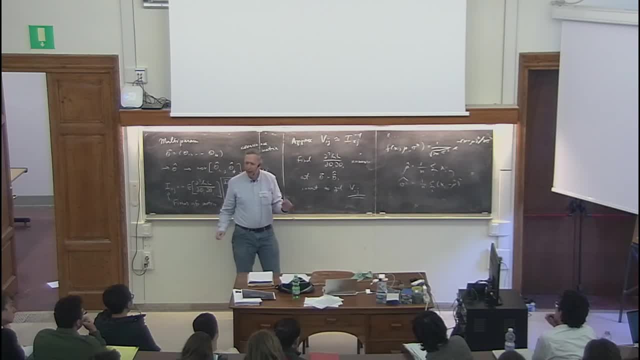 that estimator actually has a bias, All right, But there's another estimator for the variance, which sometimes is called s squared, which you've probably seen on the keyboards of old calculators. which is this? All right, And you might have wondered. 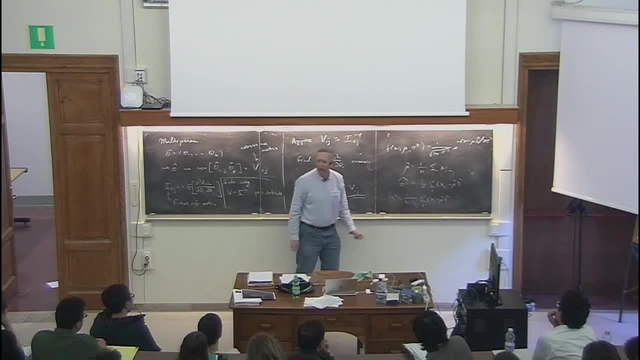 what's this minus one doing here? And so somebody might have told you: oh, that has something to do with losing a degree of freedom. when you compute the mean, What is that? I don't know what that means. what a degree of freedom? 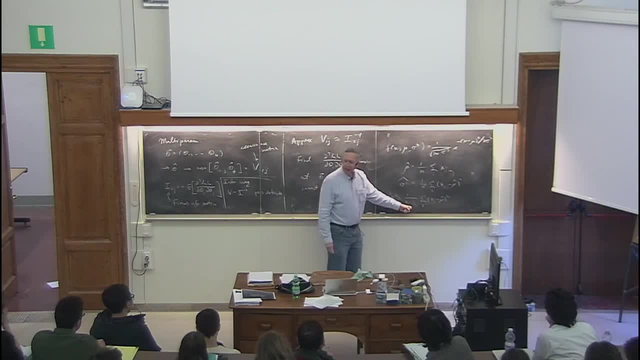 The reason this minus one is there is to give this estimator zero bias. It's there by construction to give you zero bias. You could consider estimating how? about one over n plus 17? That works, It's a function of the data. 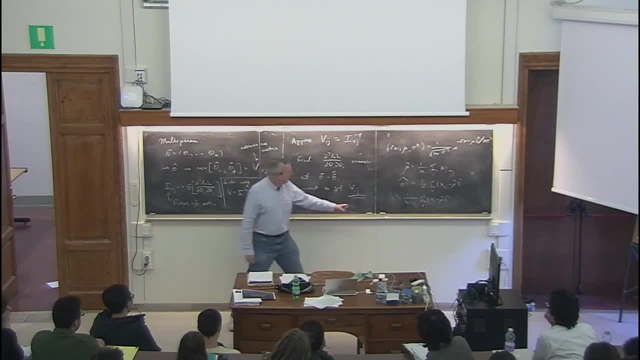 But the reason for the minus one is that this estimator has zero bias. We should have lunch, I think. Sorry, Yes, Yes. Well, what that says, for example, is that vii minus i inverse ii is greater than or equal to zero. 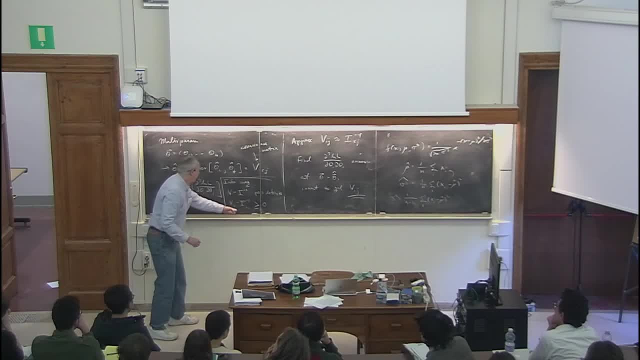 All right. So you can see that if I interpret this inequality as approximate equality, but then for the diagonal elements, it's a more sophisticated argument that I don't think I could reproduce. Small, Small, That's correct. That's correct, yeah. 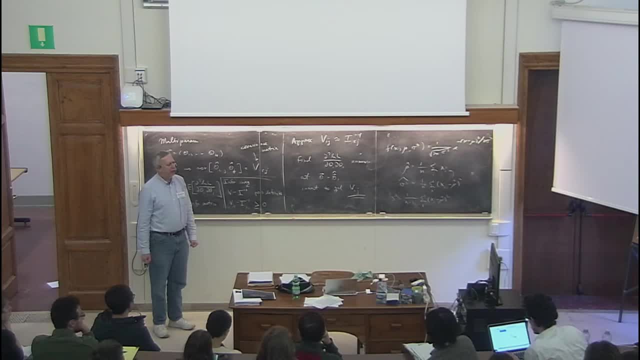 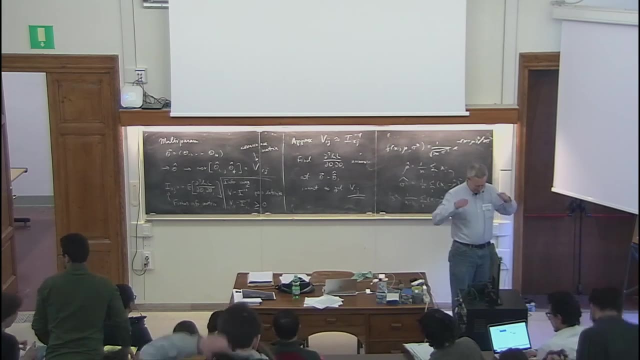 What time do we start with the discussion sessions? Oh, plenty of time. Yeah, okay, I'm sorry. I hear I was rushing because I thought you were going to have to swallow your lunch in two seconds flat. Okay, good, All right. Thank you.